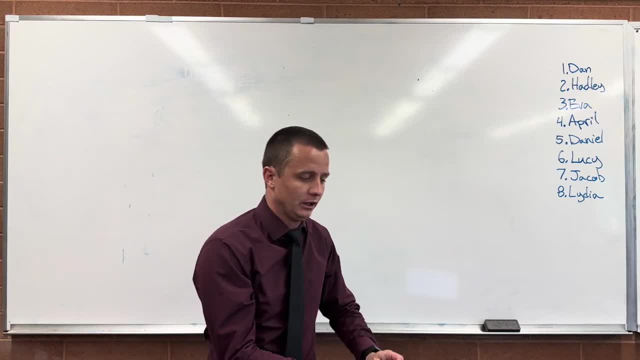 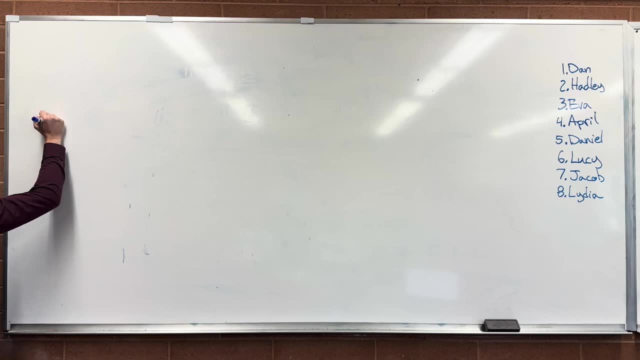 denominator. You want nothing but regular whole numbers in the denominator. So, starting out with the example, his first example says: uh, radicalize the denominator. and it has root 3 minus 9, all over 2 square root of 6.. When we say radicalize the denominator, what we mean is we do not want. 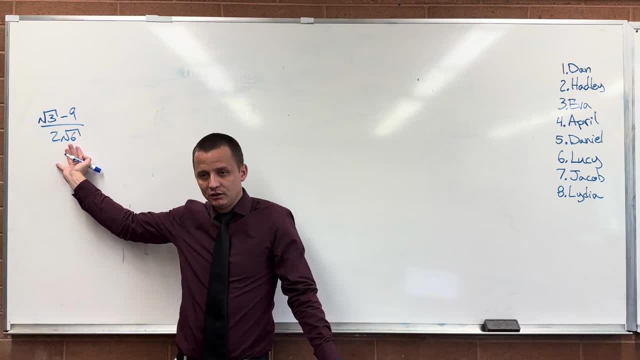 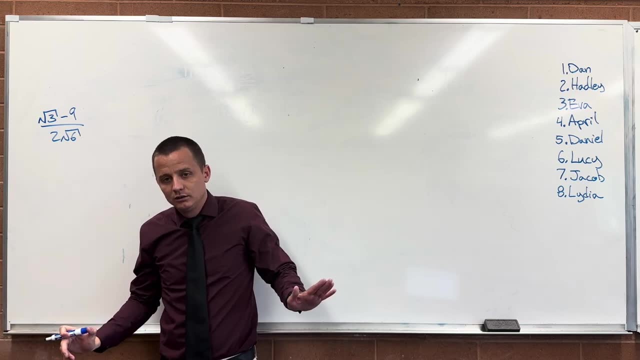 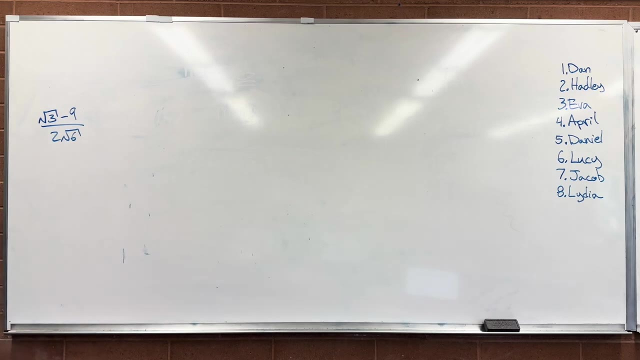 there to be any roots in the denominator. So what can I multiply square root of 6 by to get rid of it from the denominator 3? Huh, 3? 3? What's the square root of 6 times the square root of 6?? What's the square root of 6 times the square 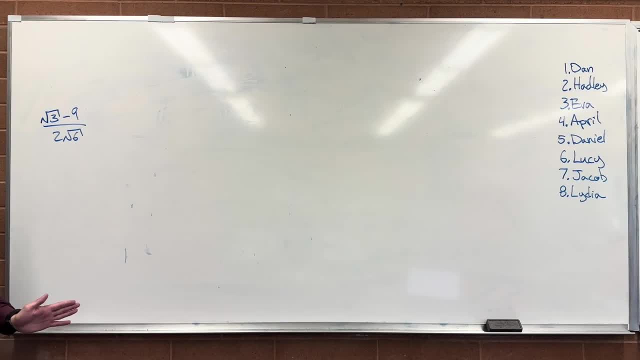 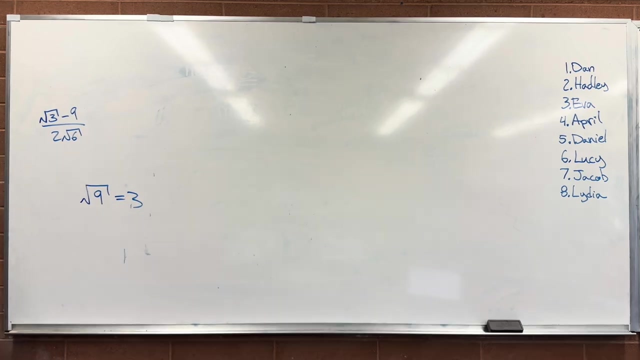 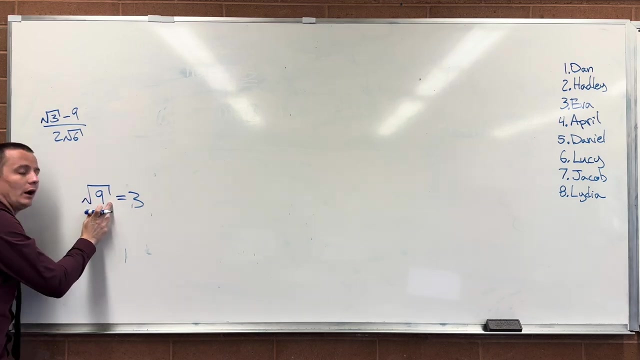 root of 6?. Let me ask you: let's reset, Let's pick a different number that is easy for us to work with. What is the square root of 9?? 3. How do you know that the square root of 9 is 3? Because 3 times 3 is 9.. So when we say what is the square root of 9?, We're saying: 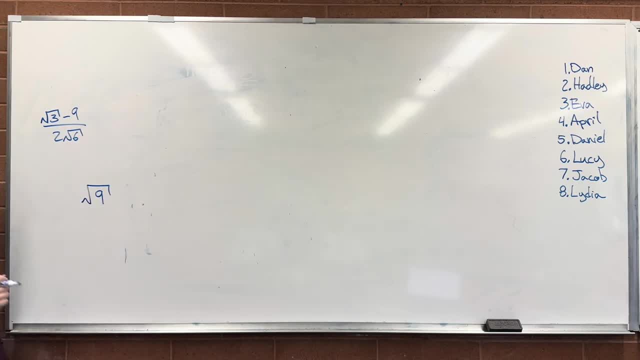 what times itself gives us 9?. Oh, So what is the square root of 9 times the square root of 9? 9. It's 9! Or in other words, 3 times 3 is 9.. That's what we mean by the square root of. 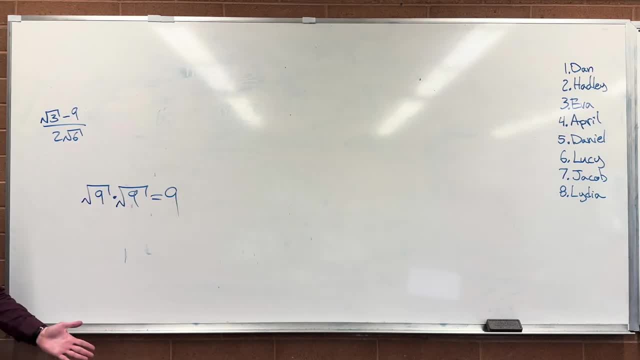 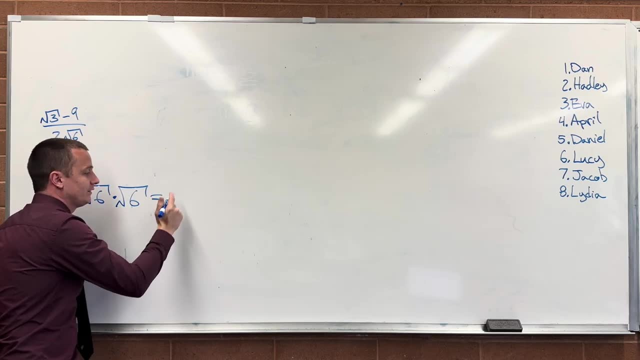 9.. We mean the number such that when you multiply it by itself, you get 9.. Alright, reset. What's the square root of 6 times the square root of 6? 6.. There it is, it's 6.. And in general, what's the square root of any number times the square? 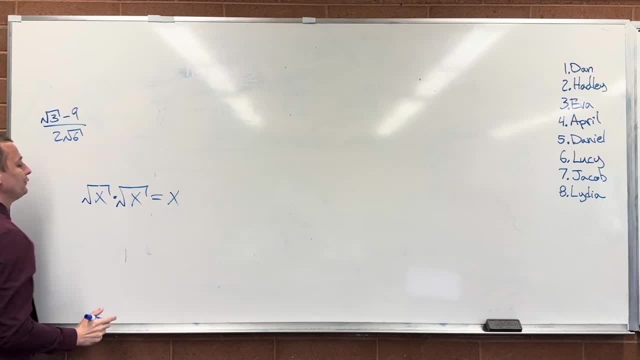 root of itself, again Itself Itself. And if we were talking about the cubed root of x, then 3 cubed over x is 9.. The cubed root of x gives you back x. If we were talking about the fourth root of x, 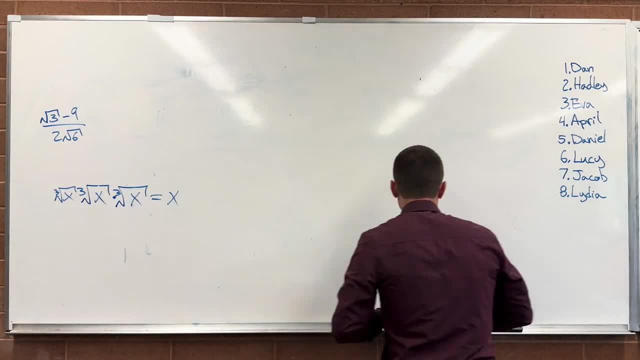 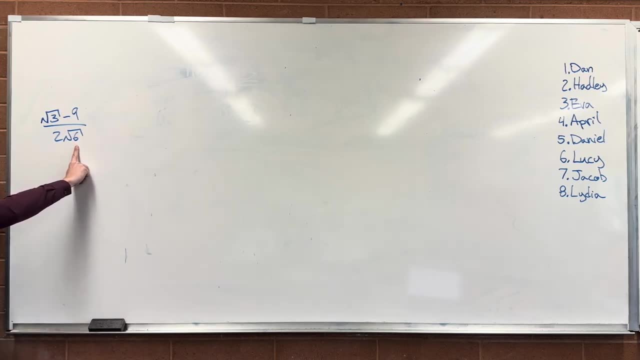 4 of them gives you back x, Etc. Okay, so back to our initial question: What can I multiply the square root of 6 by to get rid of the square root? Square root of 6.. Square root of 6.. Because square root of 6 times square root of 6 gives me just 6, and 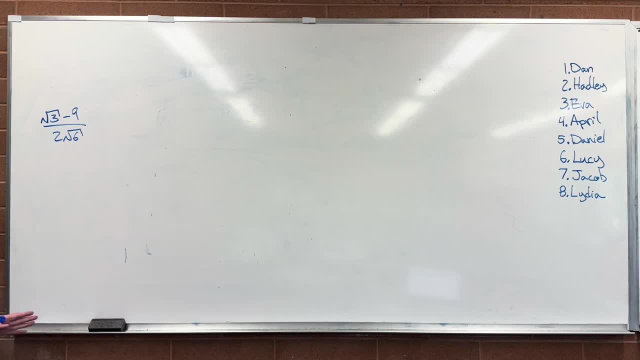 it gets rid of the square root, So we don't have a radical anymore. Good, Now I can't just multiply this number by the square root of 6.. That changes the number. I have to multiply it by 1.. I have to multiply it by 1 where I get a square root of 6 in the denominator. 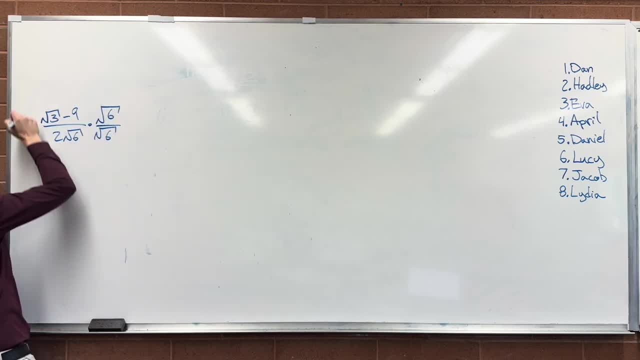 So I multiply it by square root of 6 over square root of 6.. So I didn't change the whole number. It's still the exact same number we were talking about before. I just multiplied it by 1, but I multiplied it by this clever one That makes it so that in the denominator we get rid. 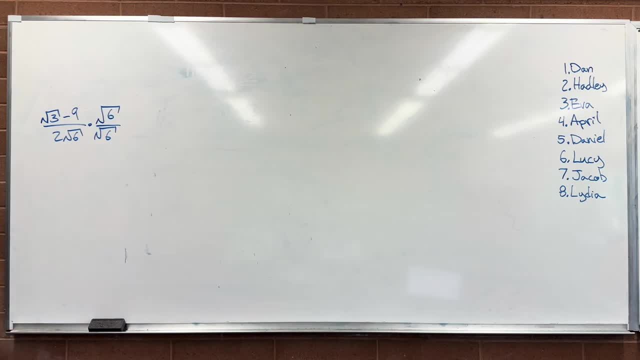 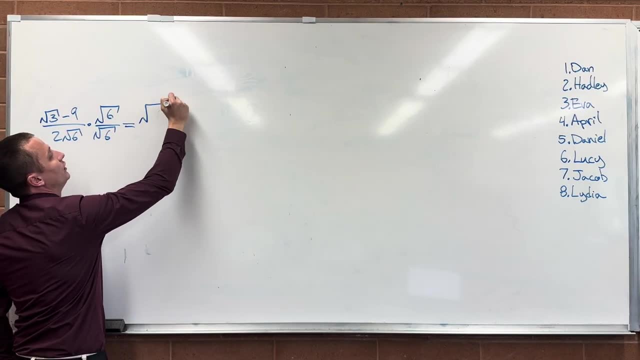 of our square root. That's what we mean by radicalize the denominator. So we multiply this through Square root of 6 times square root of 3 is square root of 18.. We'll deal with that more here in a sec. 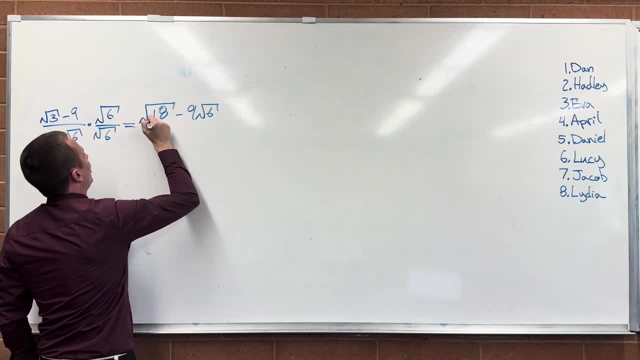 Minus 9, square root of 6.. But now it's all over. Square root of 6 times square root of 6 is 6 times 2 is 12.. There we go, So it's over 12.. Okay, now we're just simplifying. 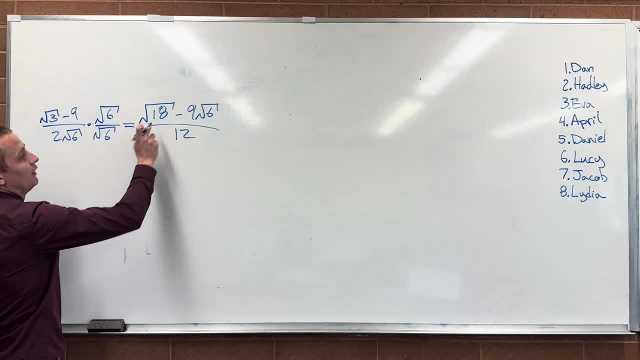 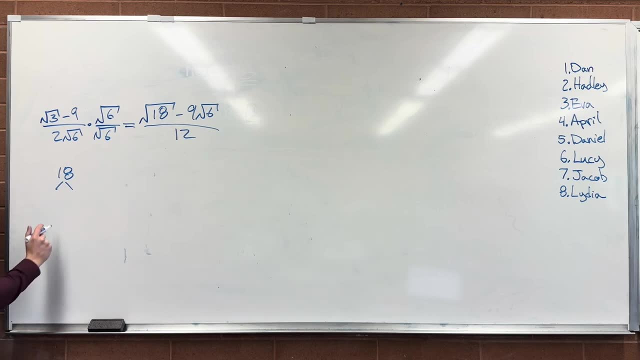 the way we know a lot. So square root of 18, what can we break that up into? Can you get a perfect square root of 18? It's 3 and 6.. 3 and 6, neither of those are perfect squares. 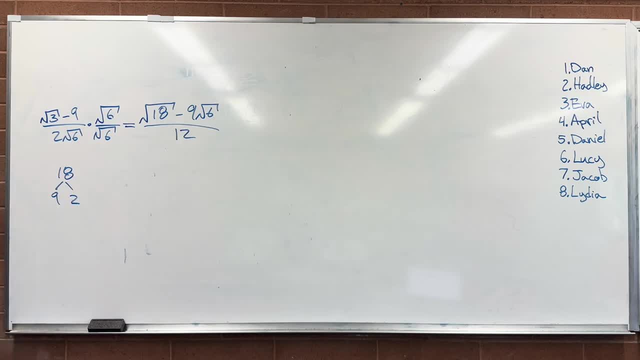 9 and 2.. We can break it up into 9. and 2. Remember 9 is the same thing as what: 3 times 3.. Yeah, 3 squared. So when we say square root of 18, that's the same thing as the square root of 3 squared times 2.. Breaking. 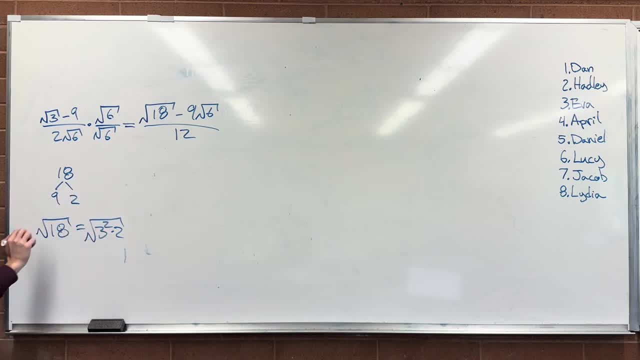 it up And now we can pull the 3 out, getting rid of the square. So it's going to give me 3 e-squares of 2.. You remember doing this. You should have just done a bunch of this on your homework. You should be fairly competent at this process by now. Okay, so this is now. 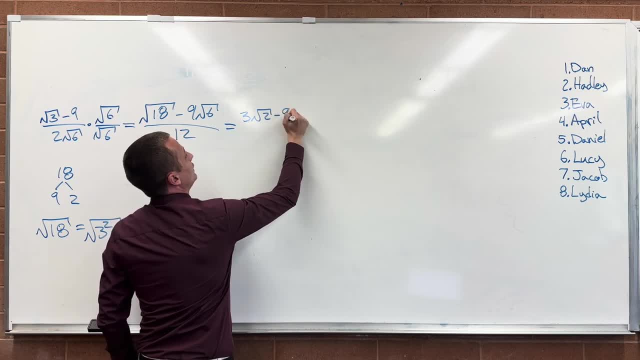 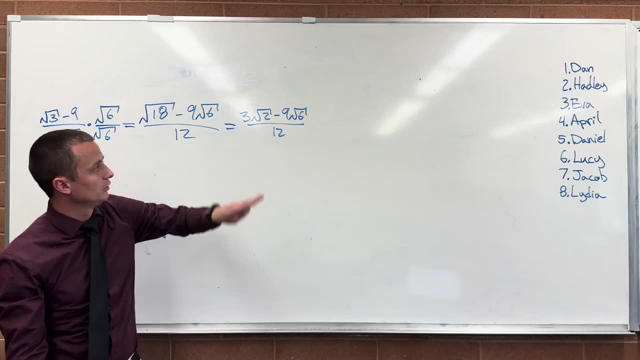 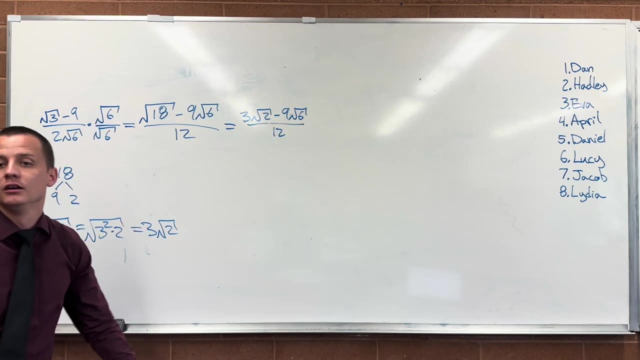 equal to 3 squared of 2 minus 9 squared of 6, all over 12.. Now the only question is: can we factor something out of these two numbers? Is there anything that goes into this number? and this number 3 goes into those. So pull the 3 out and what are we left with? 3 times. 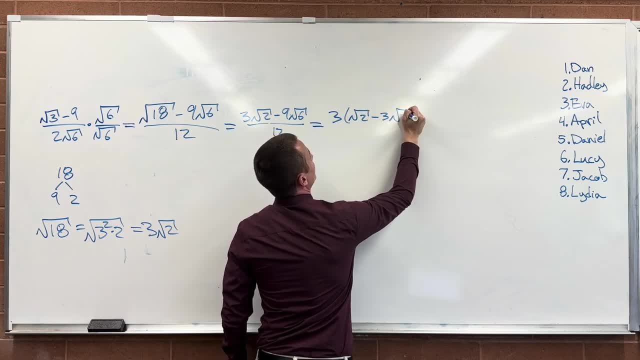 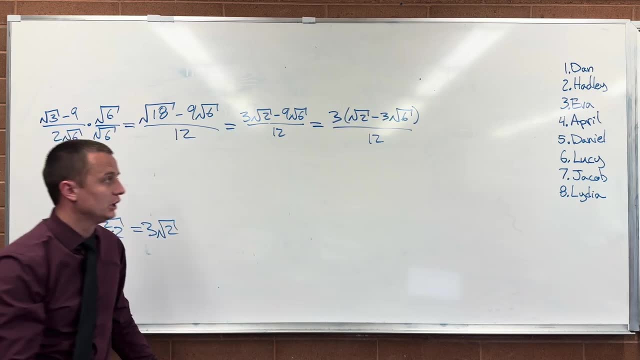 the square root of 2 minus 3, squared of 6, all over 12.. And now that we have two factors here, we can cancel a factor from top to bottom, Because 12 is really the same thing as 3 times 4, and so we can cancel the 3 top and bottom. 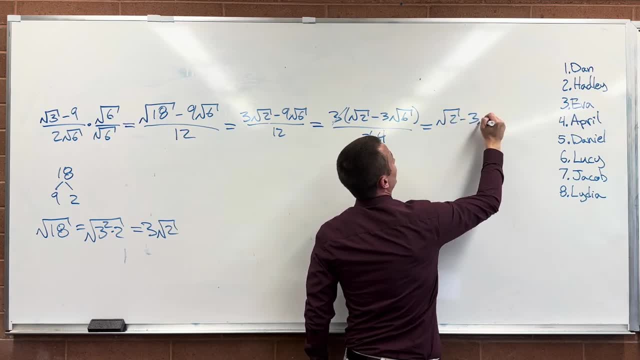 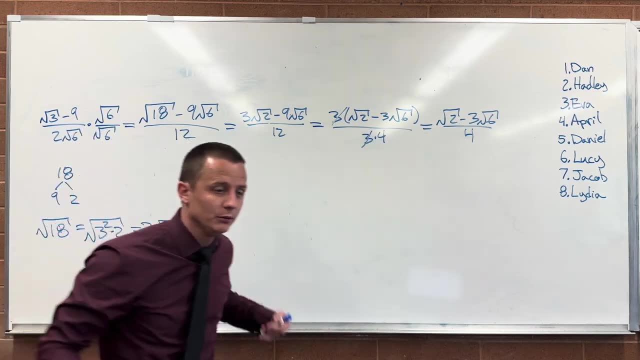 And that's as reduced as we're going to get. So it's root 2 minus 3, root 6, all over 4. And we can't get more reduced than that. Coming back to you, the stuff you've been doing. 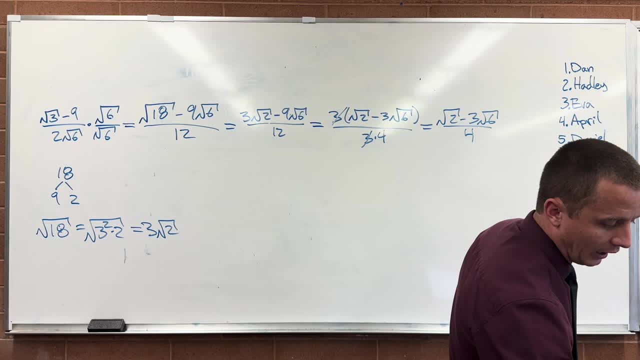 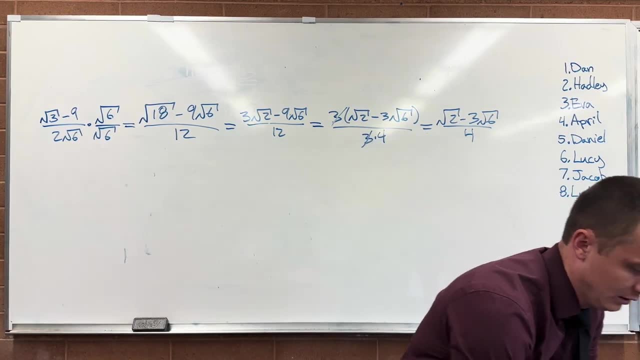 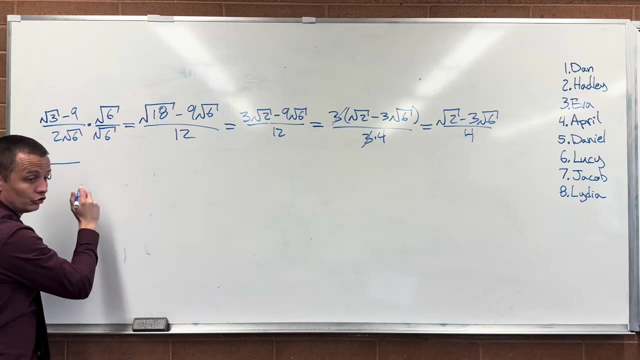 Root 2 minus 3, squared to 6, all over 4.. Okay, same thing. All right, let's try a bit more convoluted one. So his next one here that he has for us is 2 square roots, 2 square root of 20, x to the. 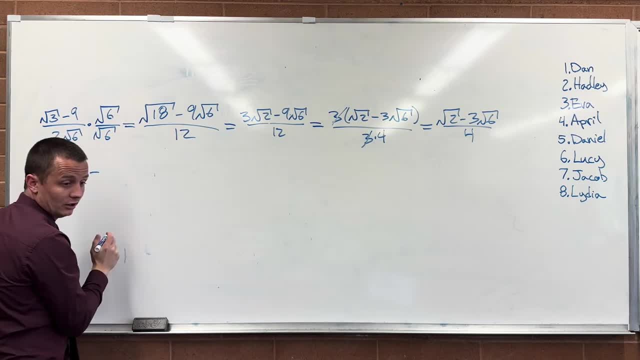 5, n, radical minus square root of 12 x squared. square root of 12 x squared, And we're going all over a square root of 18 x squared. All right, so first thing I'm going to do is try and simplify each of these the best I can. 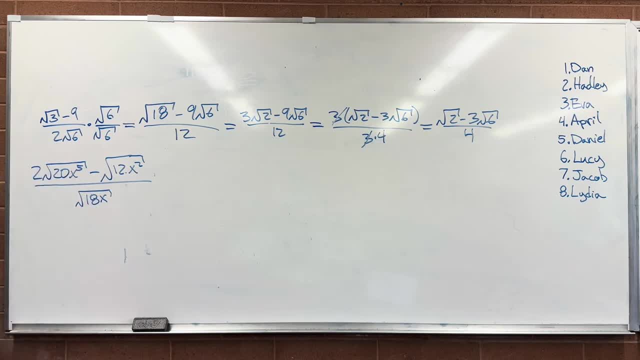 See if there's any perfect squares I can pull out of the number Just Daniel. Okay, oh, thank you. So we're going to take each one of these and see if there's any perfect squares we can pull out of it. Any perfect squares we can pull out of here- What? 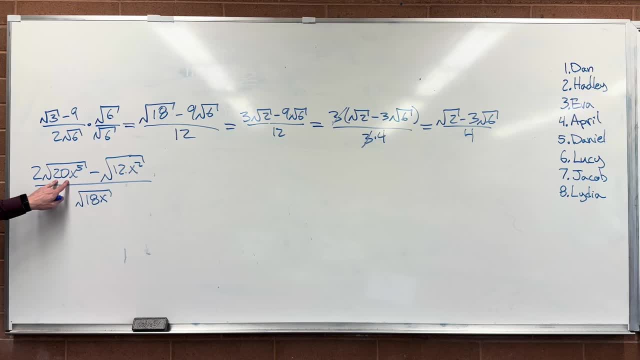 Huh, So 4, we can pull out of the 20.. What can we pull out of here, Out of the x to the 5.. Yeah, we can, Let me rewrite this expression. So, this expression, we can write this as rewriting. 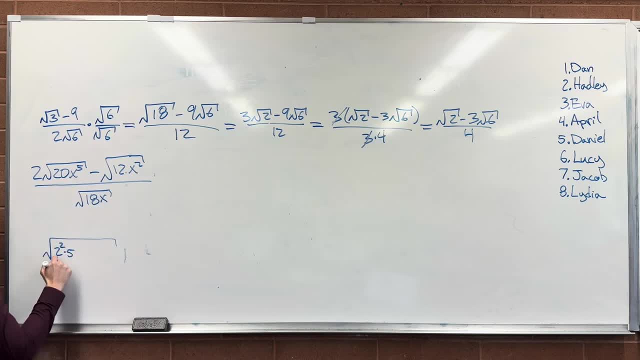 the 20, that's the same thing as 2 squared times 5, 4 times 5, here's a perfect square times x squared squared times x. So we can pull out 4 of our x's, leaving only 2 of them, and we can pull 4 out of the. 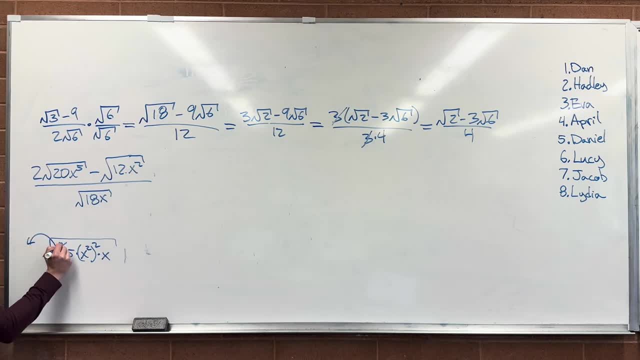 20, leaving only 2.. So if I pull the 2 out, it gets rid of the squared, and if I pull the x squared out, it gets rid of the squared, And so we're going to be left with 2 x squared. 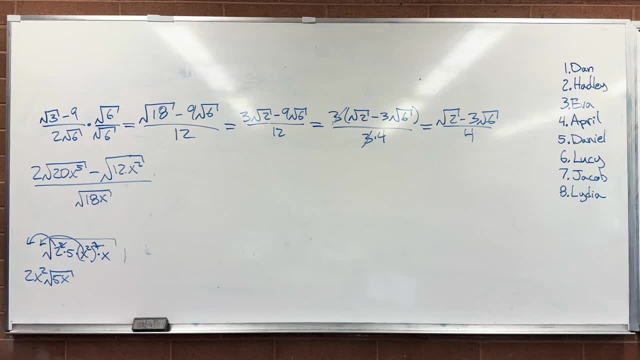 times the square root of 5 x. So we pulled the 4 out and we pulled an x to the 4 out, cutting each one in half. It's power Okay. So this first term we pulled this out, but we already had 2.. So it's going to be 4 x. 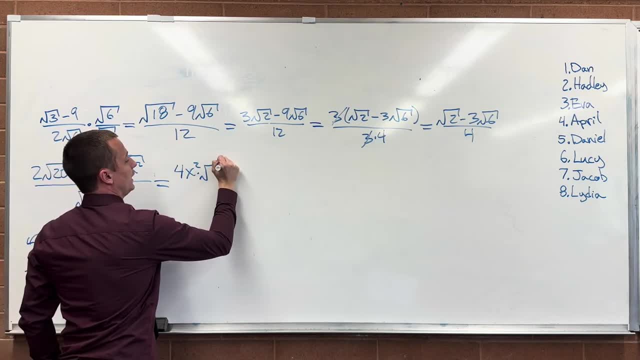 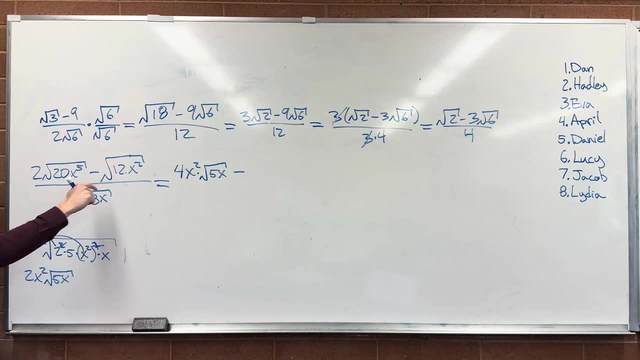 squared times the square root of 5 x. So there's our first term Minus. can we pull anything out of 12?? 3 and 4.. 3 and 4.. So I can pull the 4 out. If I take the square root of 4, it becomes a 2.. 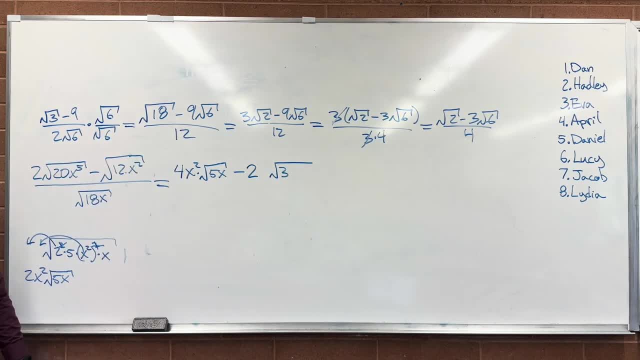 And we leave a square root of 3 on the inside. Because 12 is 3 times 4, we pull the 4 out. taking its square root gives us 2.. Leaving that, We have the x squared here, taking its square root to pull it out just. 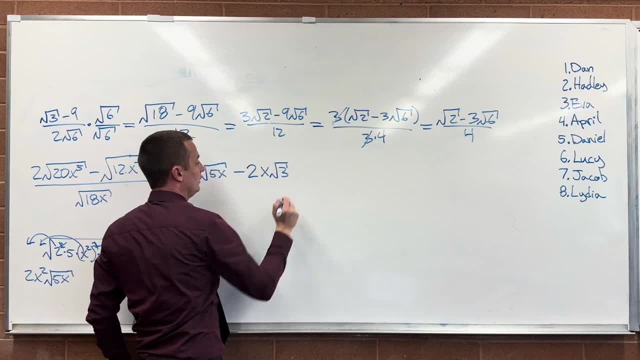 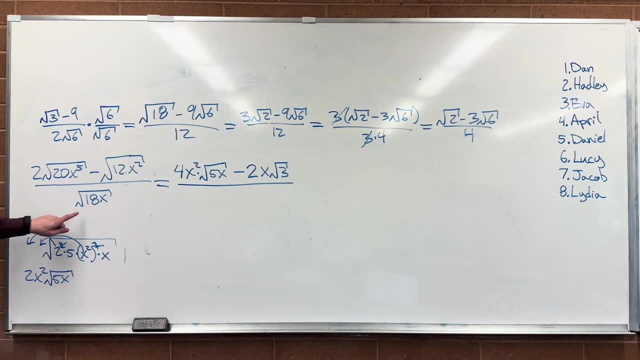 leaves us with x- x- The square root of x- squared just x. So we have minus 2 x squared, so 3 all over. Now finally, this one, 18.. What can we pull out of 18? 9.. 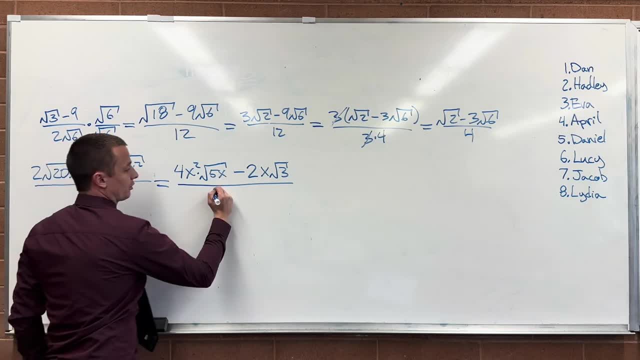 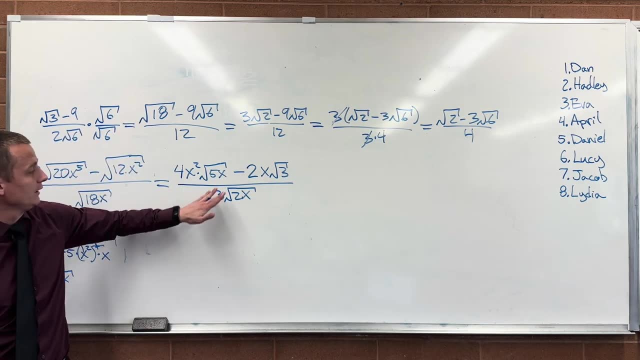 9 and 2.. Take the square root of 9, as we pull it out, gives us a 3, and we left 2 behind. Okay, Now I can't simplify these anymore. I need a radical. I can't simplify this, but. 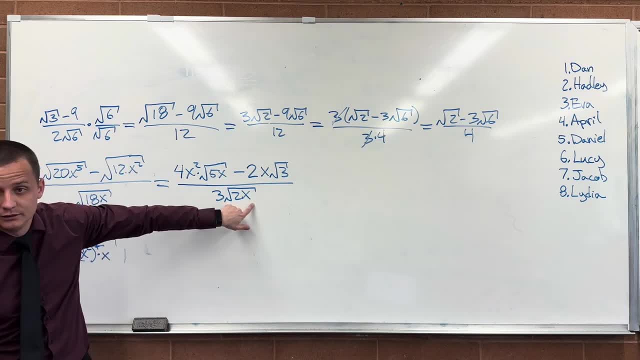 I can't simplify that. I can't simplify that. I can't simplify that. I can't simplify this. I can't simplify this, Radicalize my denominator, so I need to multiply by whatever its square root is: top and bottom. 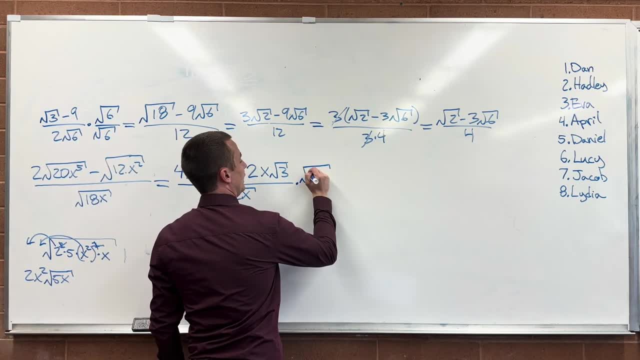 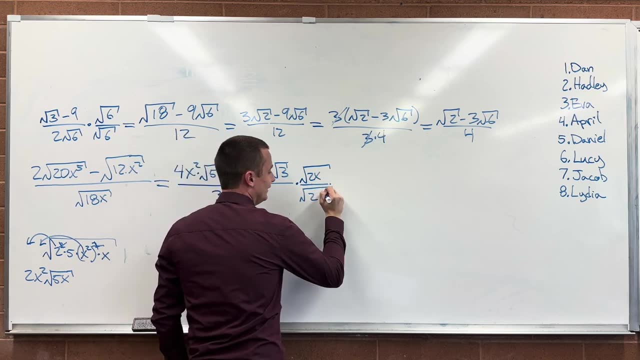 So now I'm going to take this: I'm going to multiply top and bottom by square root of 2x over square root of 2x. Sorry, no idea. Square root of 2x over square root of 2x. there we go. 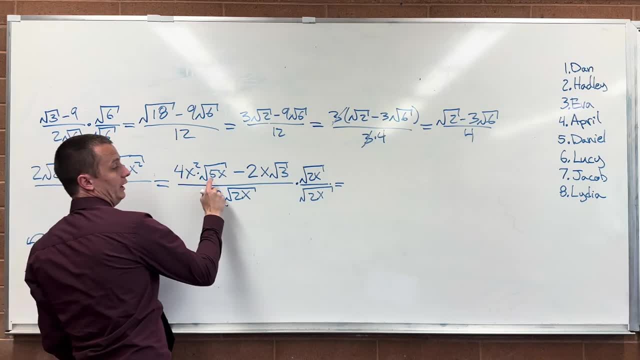 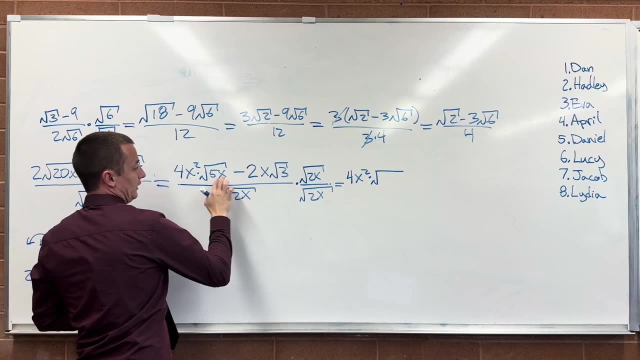 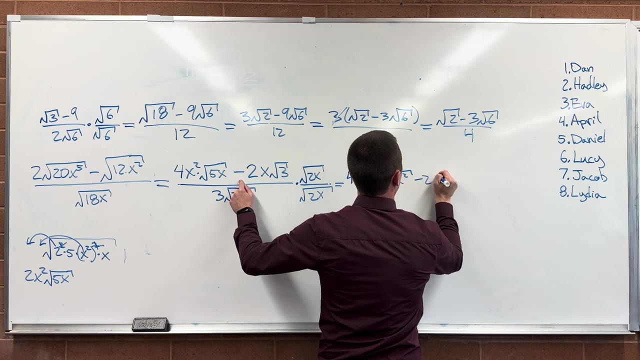 Alright, multiply this through to each term. So here we're going to get 4x squared times the square root of 2x 10x squared. thank you, 10x squared minus 2x times the square root of what? 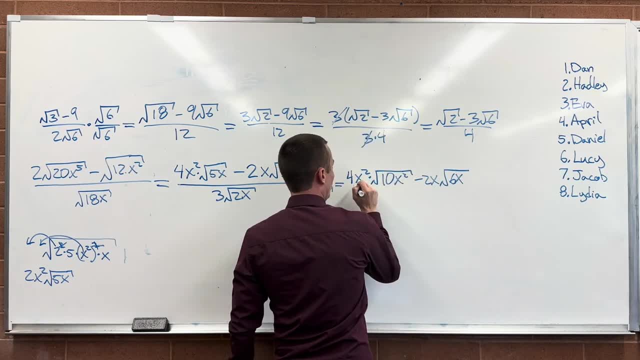 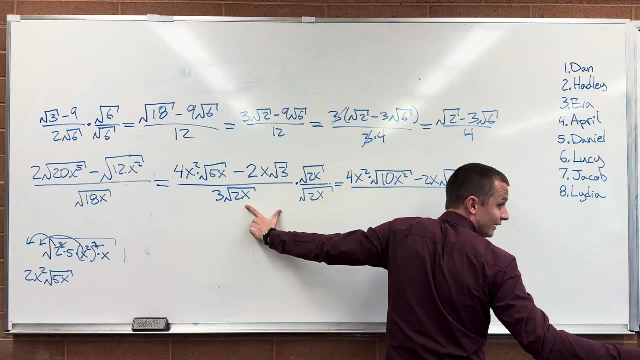 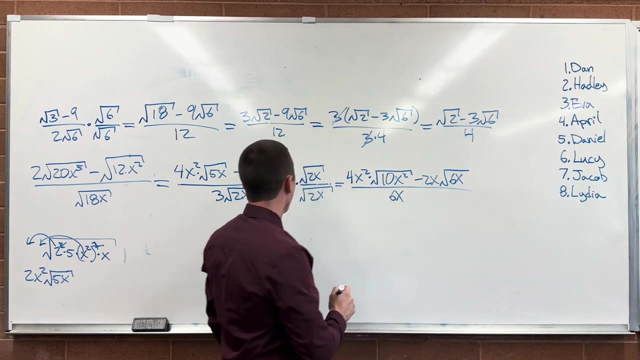 6x, Just 6x good, Alright, all over. tell me my denominator: 1x, 3x squared 3x squared 3x squared 6x, 6x, because the square root of 2x times the square root of 2x is just 2x times 3 gives us 6x good. 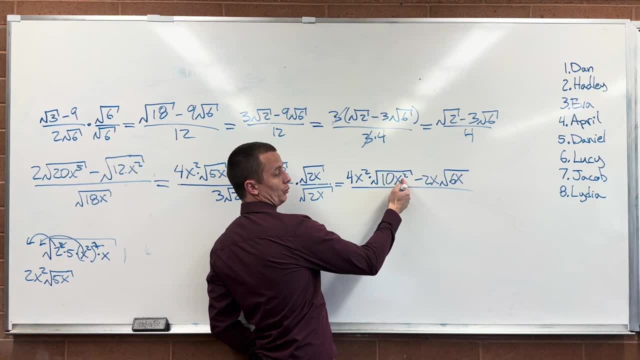 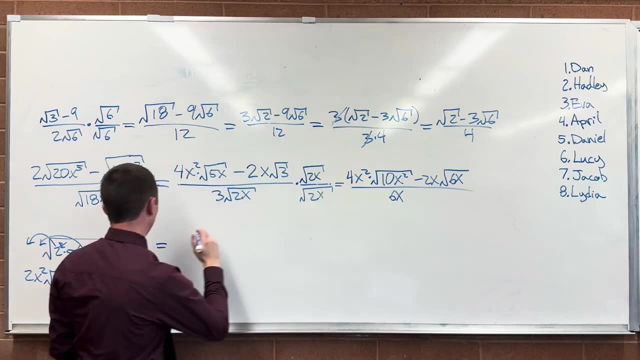 Now notice this one. I can take the square root of my x squared here. I can pull that x out. So this is going to be equal to: on this term, we're going to get a 4x cubed, 4x cubed times the square root of 10, nothing we can do with the square root of 10, minus 2x squared of 6x, all over 6x. 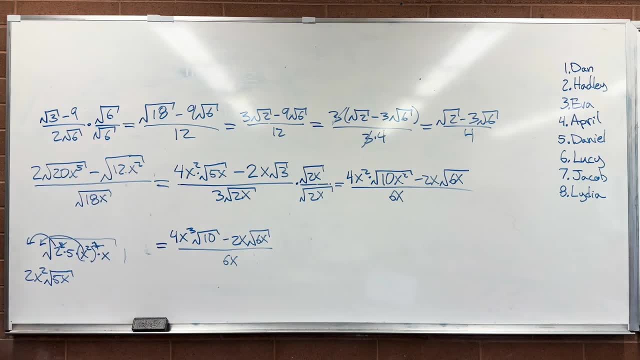 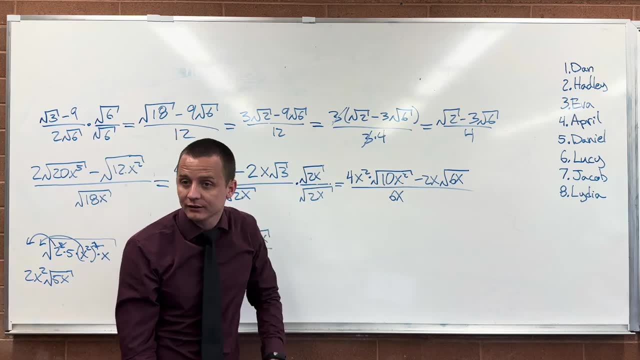 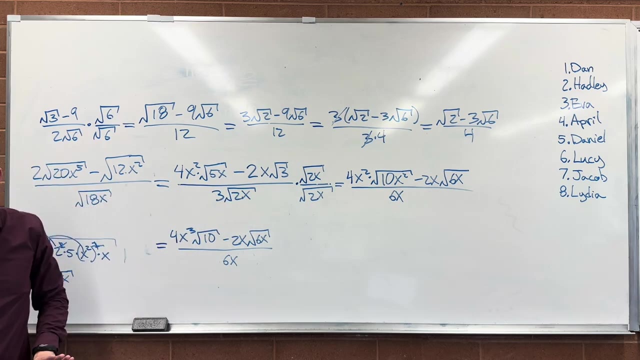 Why isn't it x to the 4?? When I take the square root of x squared, what do I get? Just x. So x squared times x gives me x cubed good. And now, finally, let's see if there's anything we can factor out of the top to cancel out with the bottom. 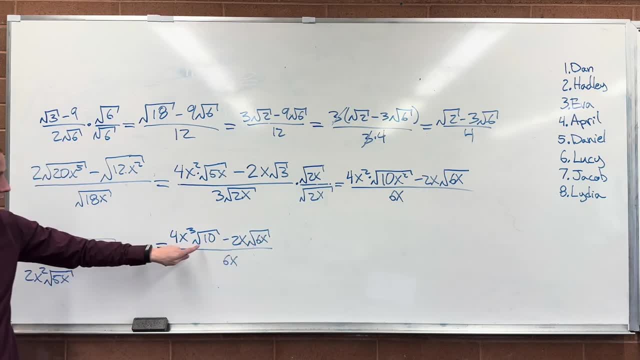 There's 6x, but Can I pull anything out of these two terms in the top 2.. 2,- we can pull a 2 out. We can also pull a 3.. No, An x, Oh. 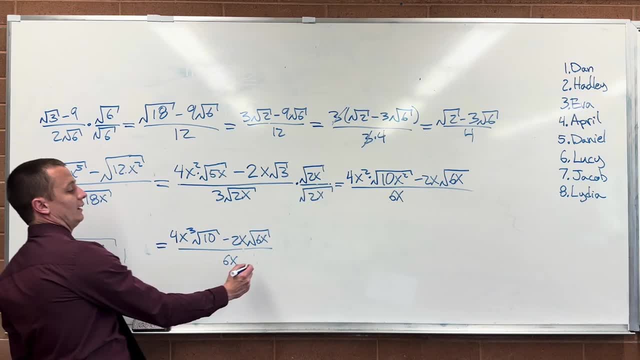 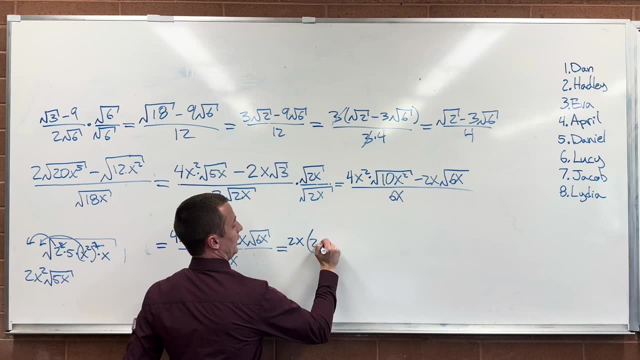 That has an x, that has an x, that has an x. So I'm going to pull a 2x out of the top, and so we're left with 2x times. when I pull it out of this term, I'm left with 2x squared square root of 10.. 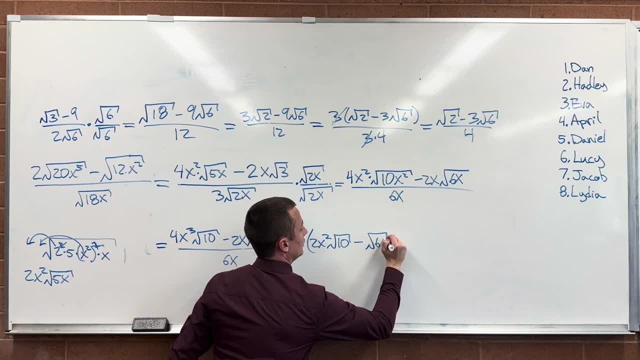 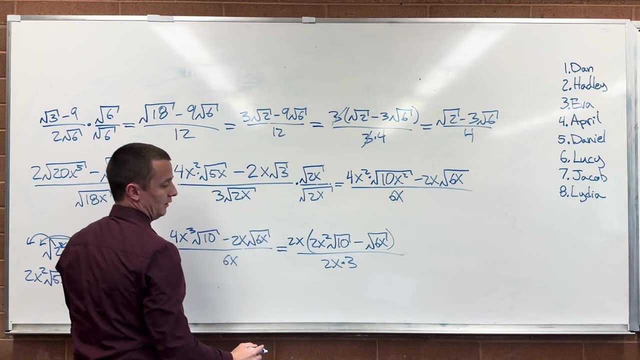 Minus square root of 6x all over, rewriting 6x. this is the same thing as 2x times 3. And we can cancel out 2x top and bottom, and so we're left with that over 3.. 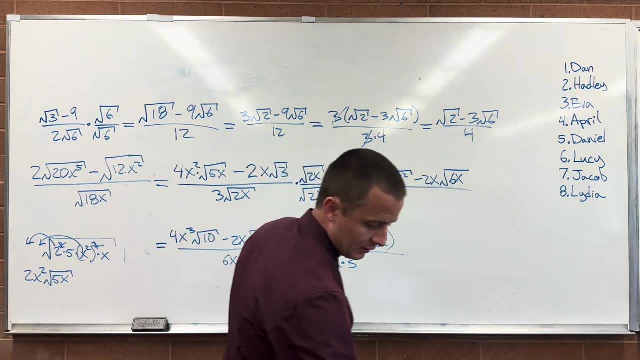 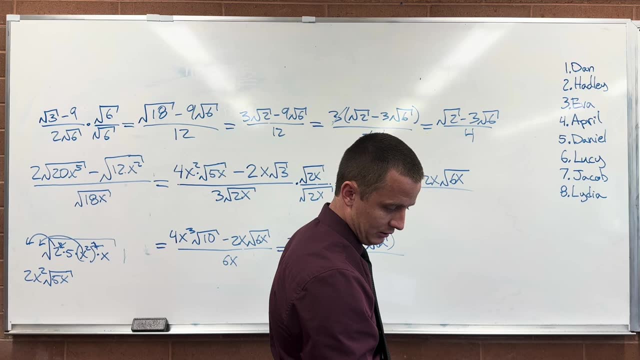 You see that. Okay, Let's double check. with his answer, He still had a 3x in the denominator, But he cancelled out an x, so that's a typo. It should just be 3.. Okay, Let's now get to the conjugate. 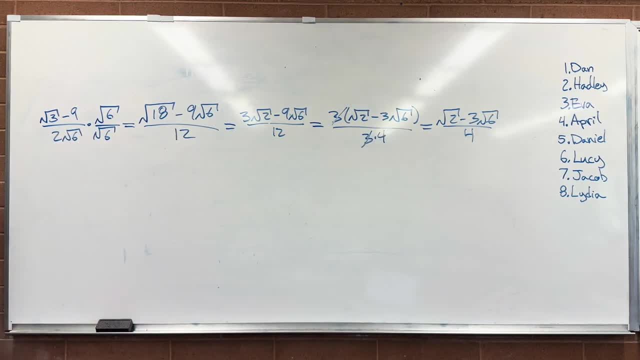 So sometimes radicalizing our denominator isn't so straightforward. Here's a good example: We have 2 over the square root of 3, minus 5.. What can I multiply my denominator by to get rid of the square root of 3?? 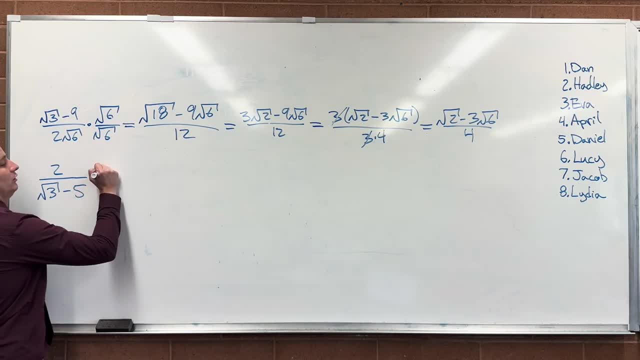 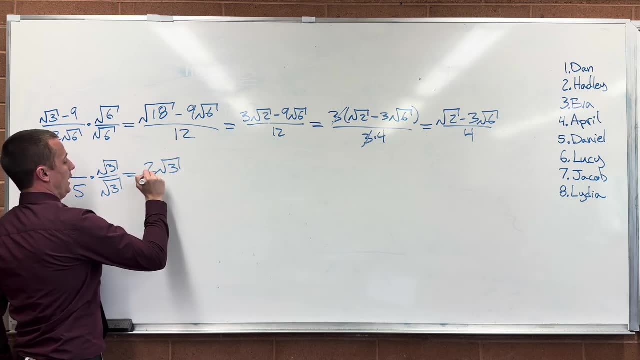 Your gut's going to say square root of 3, but see what that does to us. So I'm going to multiply his top and bottom by square root of 3, and what am I left with? In the top, we get 2 square root of 3, but look what happens in the bottom, because I have to distribute this to both. 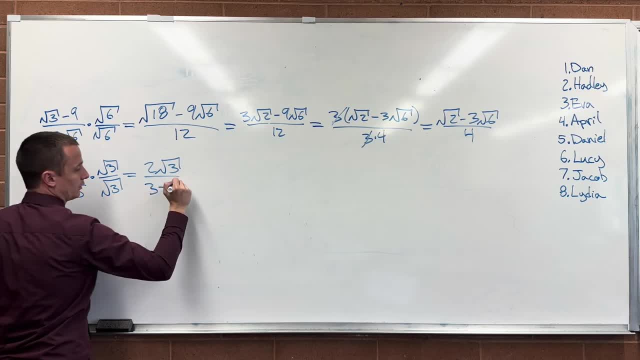 Square root of 3 times square root of 3, that's 3, but then we have minus 5 square root of 3.. And it's still there, And we still have the square root of 3 in the bottom. so we got nowhere. 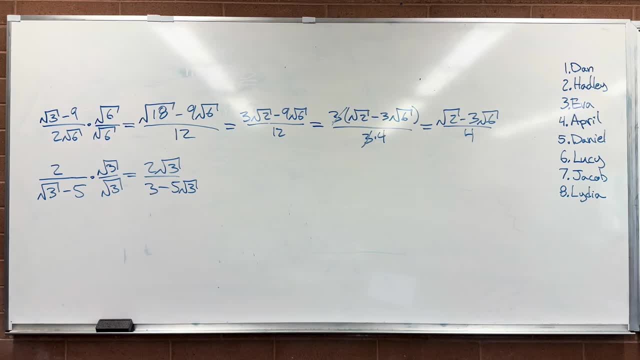 So you Yeah- kind of annoying huh- Can you do what you already have to do by the 9th of B? Yeah, I was going to say that. So what we want to multiply it by is what we call the conjugate of the number. 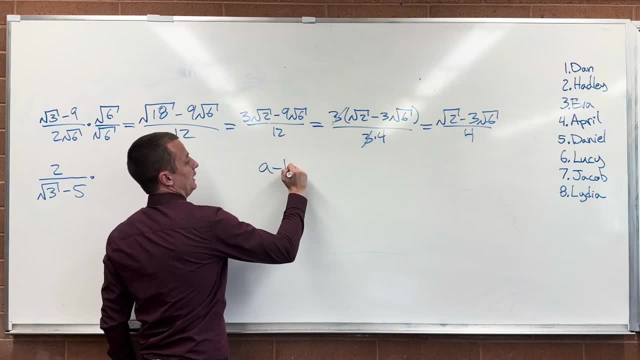 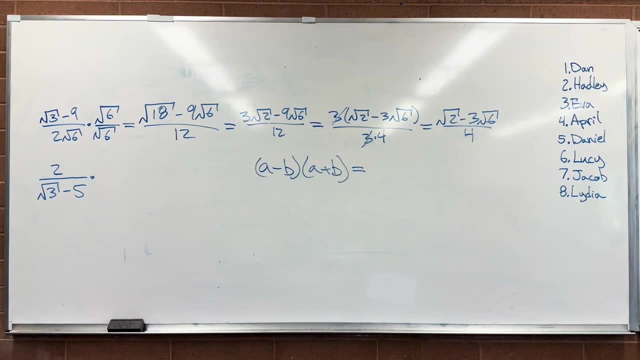 And we're essentially using the fact that A minus B times A plus B is equal to. will you remember what this is? This is our difference: of squares A squared minus B squared. Correct, This is our difference: of squares A squared minus B squared. 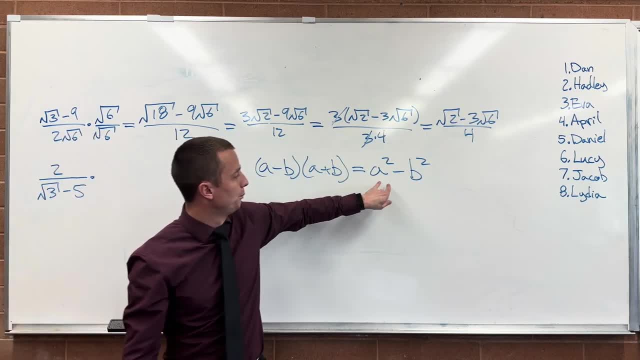 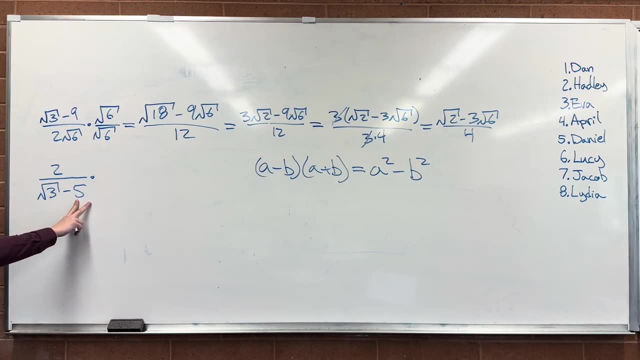 And notice that that squares both our terms, And so this is a way that if this had a square root, we're going to get rid of it, And if this had a square root, we're going to get rid of it. So here's what I'm doing. 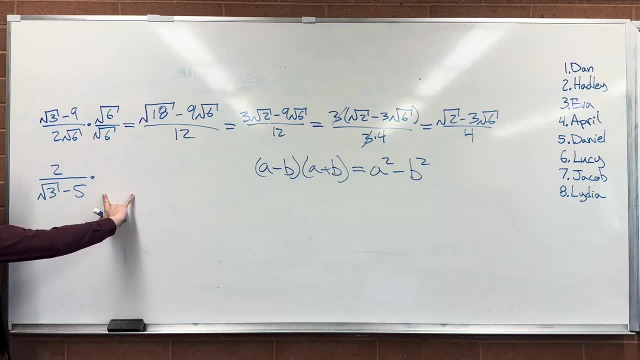 We think about this as our A minus B. I'm going to multiply it by A plus B and this is what's going to come out. So I'm going to multiply this top and bottom by A plus B. So we're going to multiply it by A plus B. 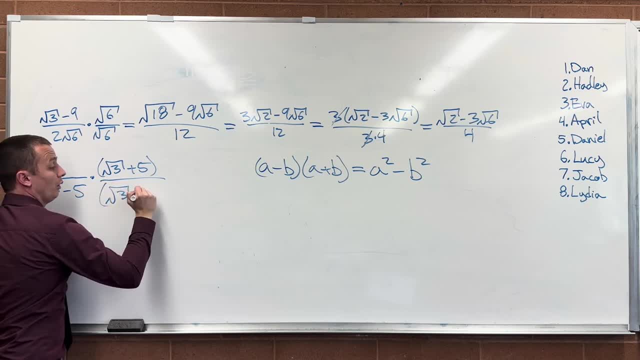 And we're going to multiply it by A: A minus B plus B. Remember, we've got to multiply it by 1. Otherwise we're changing the number. You can't do one thing to the bottom and one thing to the top. 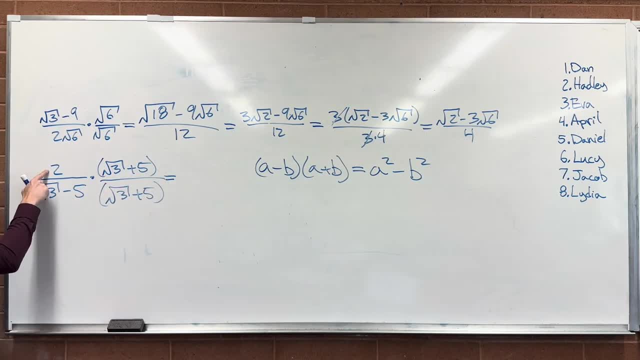 So now, when we multiply all this out, let's see what we get. In the top, we get 2 squared to 3 plus 10.. In the bottom, what did we get? Well, square root of 3 times square root of 3 gives me 3.. 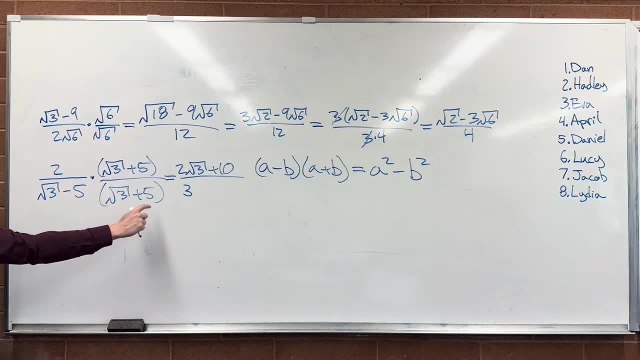 Negative 5 times square root of 3 gives me negative 5 squared to 3.. But positive 5 times square root of 3 gives me positive 5 squared to 3.. And those will cancel out, And so what I'm left with now is negative 5 times positive 5. 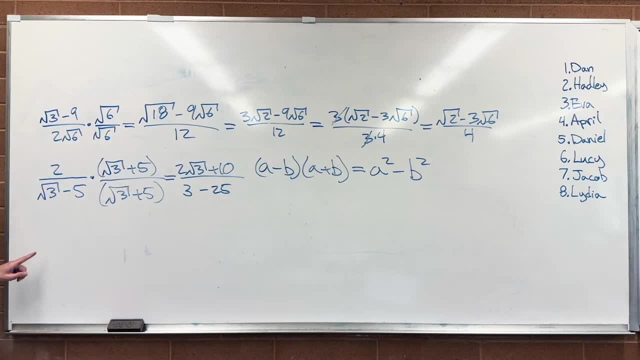 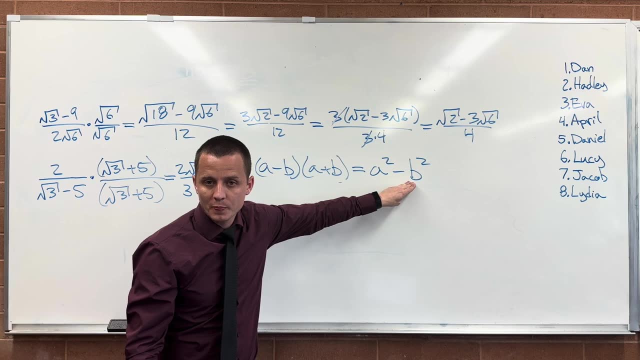 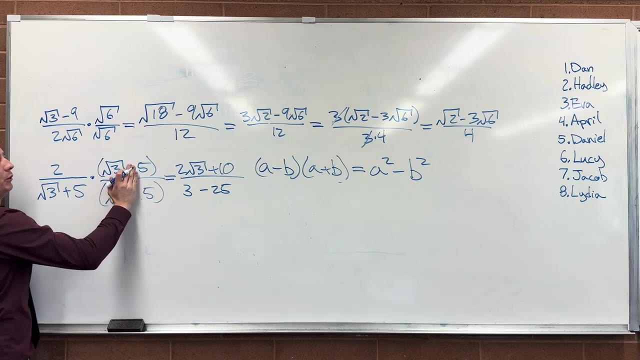 gives me minus 25.. And so notice what we're left with was A squared minus B squared. It's just the same thinking. If this had been plus, here we would have instead multiplied top and bottom by minus, minus. We call this the conjugate of this. 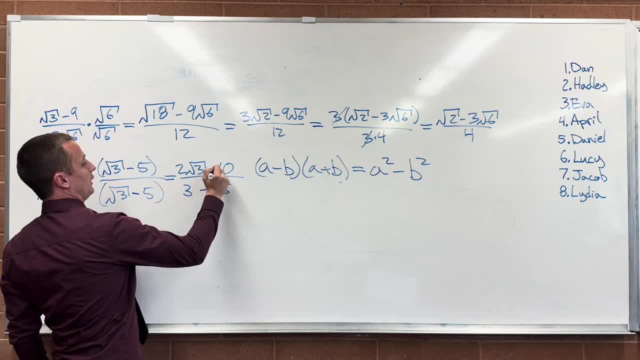 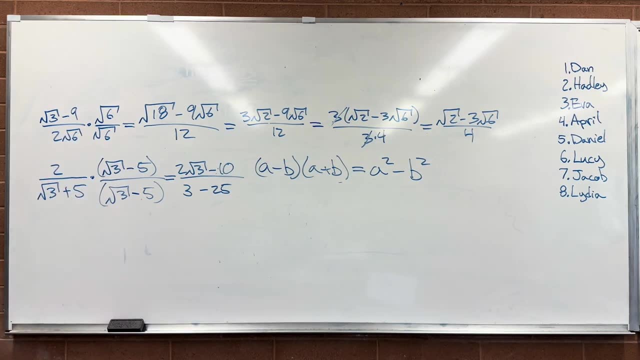 And so if you had worked out all like that, the only difference here is that we would have had a minus up there. Our denominator is still going to be the same thing. It's still going to be A squared minus B squared. Make sense. 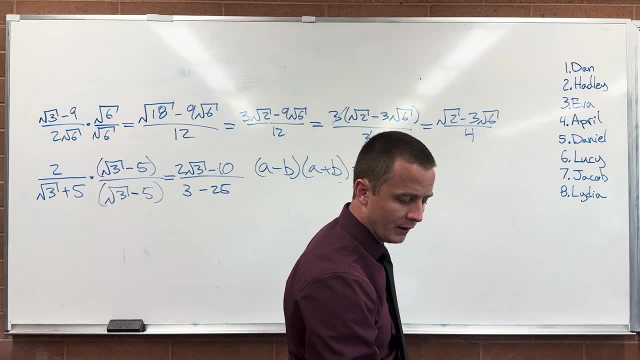 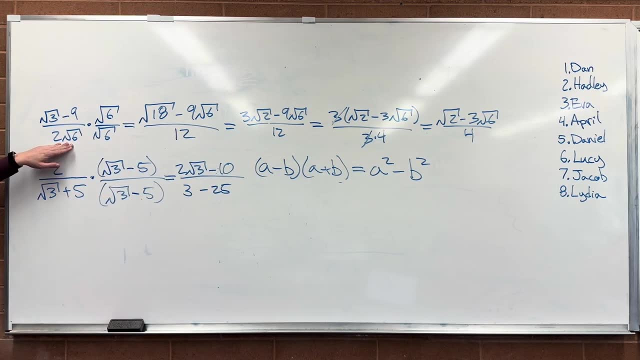 So that's what you do when you have two terms in a denominator. So that only happens when you have the square root plus something else, Because if it's like the top one you don't have to do it. Yeah, if it's like the top one, we hardly have to think about it. 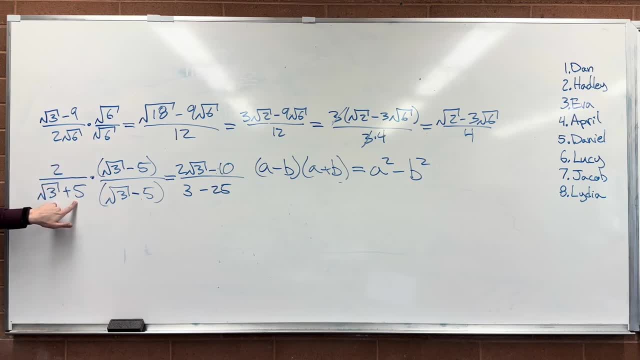 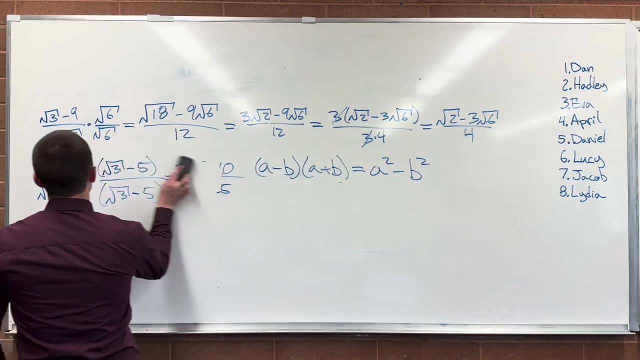 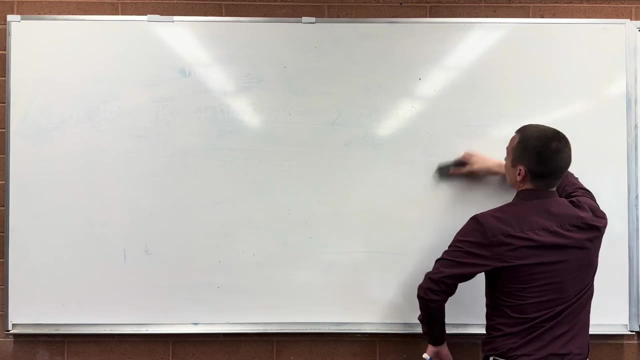 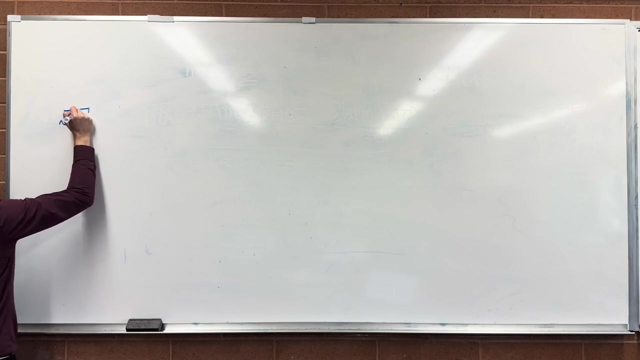 We just multiply by square root of 6. But when we have two terms now it's a bit harder. Good, OK, so let's work through a full example. OK, so this one: we have square root of 15 all over square root of 5. 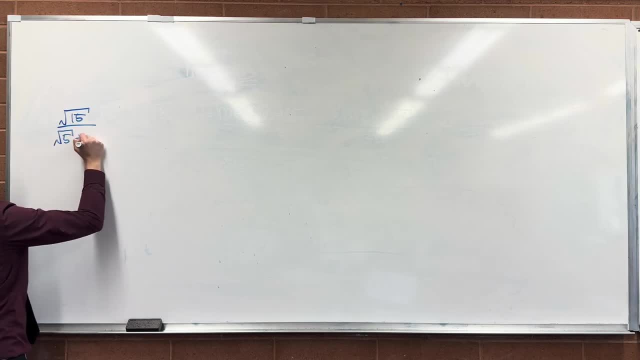 plus square root of 3.. All right, What am I going to? multiply by top and bottom Negatives: Square root of 5 minus the square root of 3.. Square root of 5 minus the square root of 3, just by the conjugate. 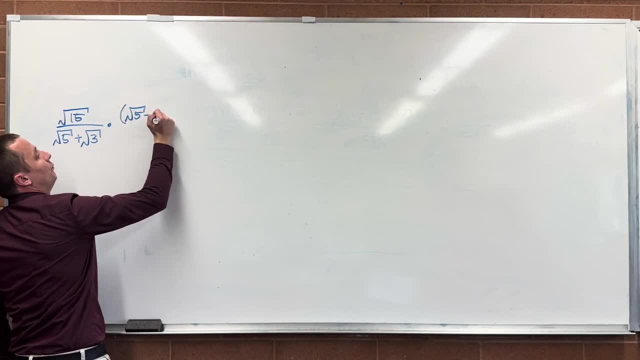 So we multiply by the conjugate top and bottom Square root of 5 minus square root of 3 and square root of 5 minus square root of 3.. All right, Let's see what that gives us In the top square root of 5 times square root of 15. gives me what. 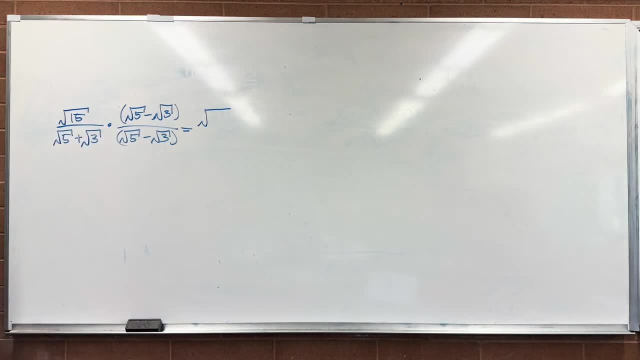 What's 5 times 15?? 5 times 15? 65.. 5 times 15? 65.. 65.. 65. 5 times 15.. This is recorded. People know you're taking this long. 5 times 15.. 75.. Thank goodness for calculators. 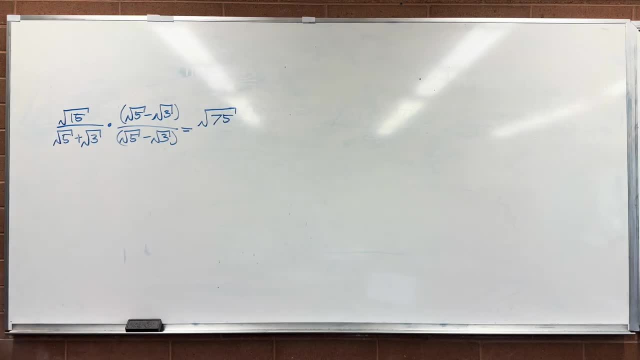 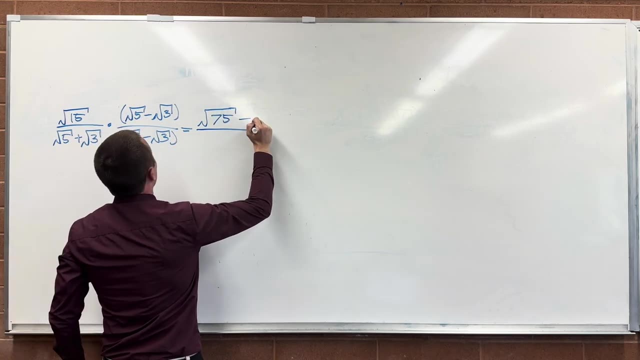 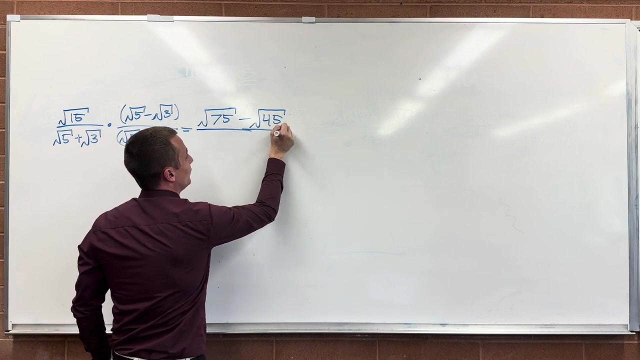 Alright, 5 times 15 is 75. All over in the denominator. Oh wait, That was only the first one. So minus 3 times 15.. 45. Much better, You can tell you didn't use the calculator on that one. 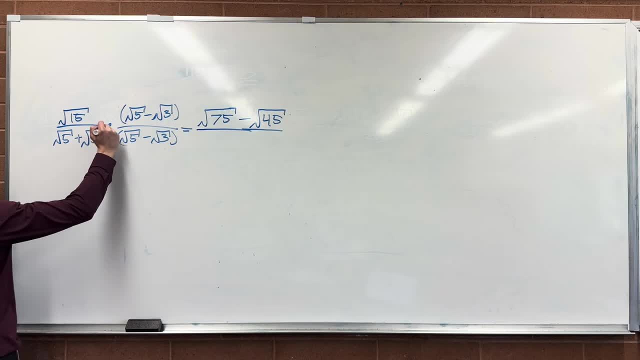 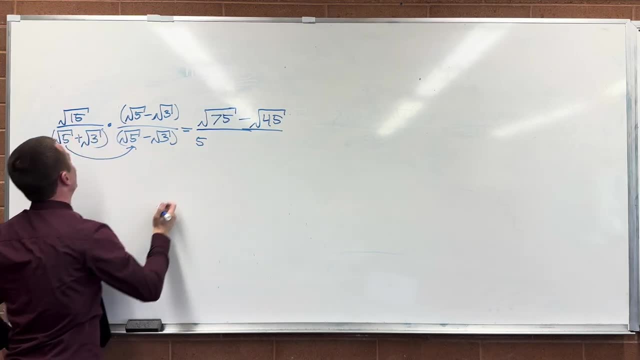 Okay, Now in the denominator we're multiplying this to this. So I've got to multiply root 5 to root 5.. What does that give me 5.. Good, Now I've got to multiply root 5 to minus root 3.. 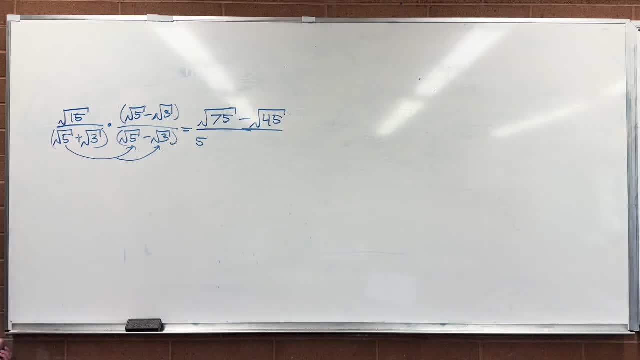 What does that give me? Negative square root of 15.. Good, Now I need to multiply square root of 3.. So I've multiplied that to both. Now I need to multiply. What Square root of 3 to square root of 5.. 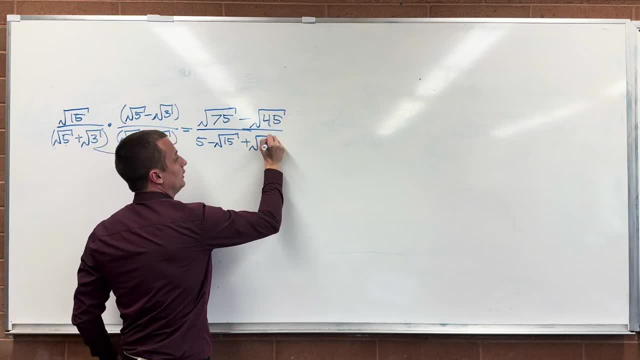 Positive square root of 15.. That's why we multiply by the conjugate. Those will always cancel out your square root terms And then finally root 3 times negative. root 3 gives me 3.. Negative 3., Negative 3.. 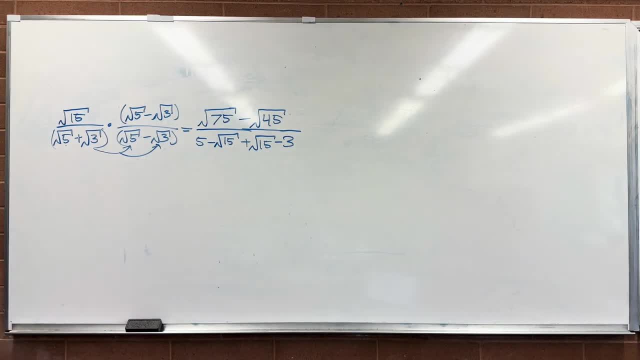 Negative square root of 9, but negative 3.. Same thing, Perfect. And so, as we wanted, our radical terms cancel out. That's why you multiply by the conjugate. That will always happen, Because a plus b times a minus b is always equal to a squared minus b squared. 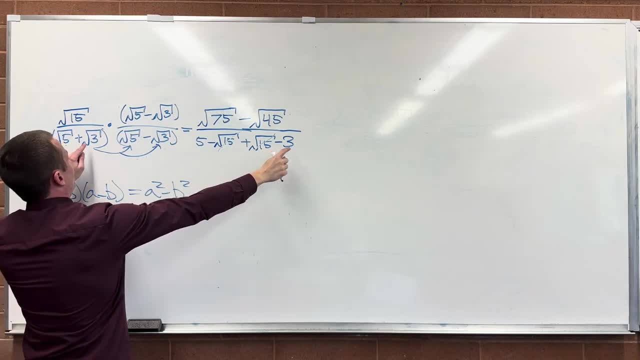 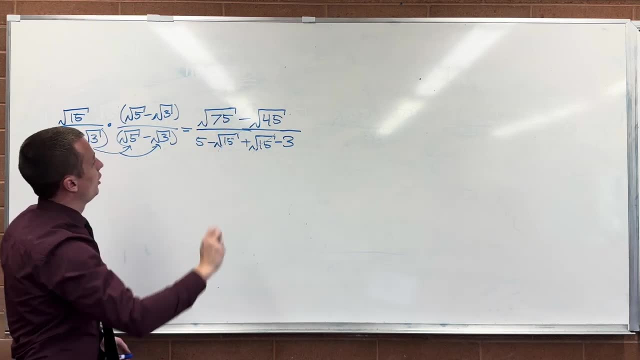 It's always going to happen. So we ended up with a squared minus b squared Every time. Okay, So now that we got it like that, let's just do all our reducing. What's a perfect square that goes into 75?? 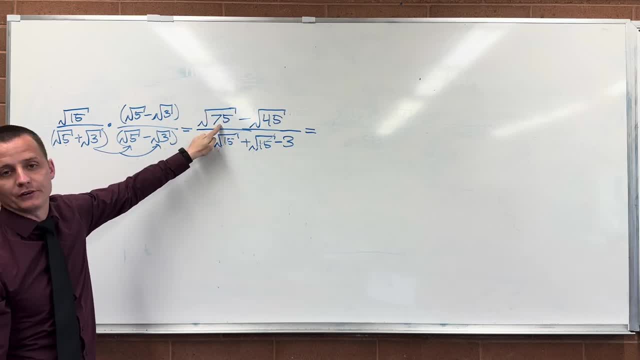 5.. Not 5.. 5 is not a perfect square. but what's a perfect square that you make with 5?? 5 times 5 is 25.. Does 25 go into 75?? Yes, So 25 is a perfect square. 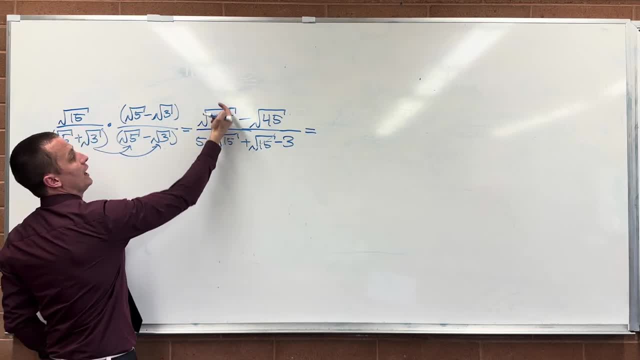 25 and 3.. So it's 25 and 3.. So we pull the 25 out. What's the square root of 25? 5.. So when we pull the 25 out, we're left with 5 squared to 3.. 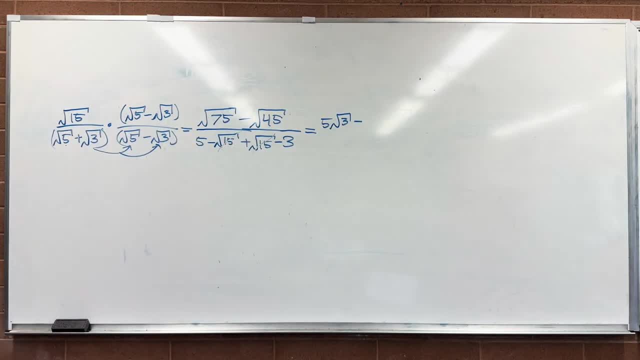 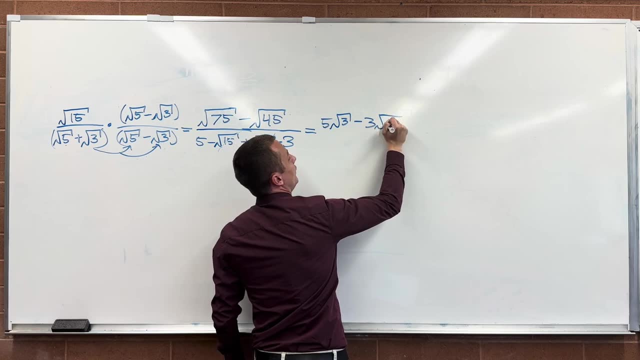 Minus. Do we have any perfect squares in that 9. 9. So when we pull it 9 out, we get a 3. And we're left with inside squared of 5. 5. Good. 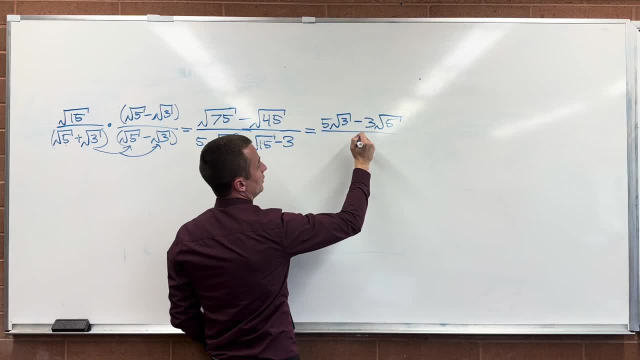 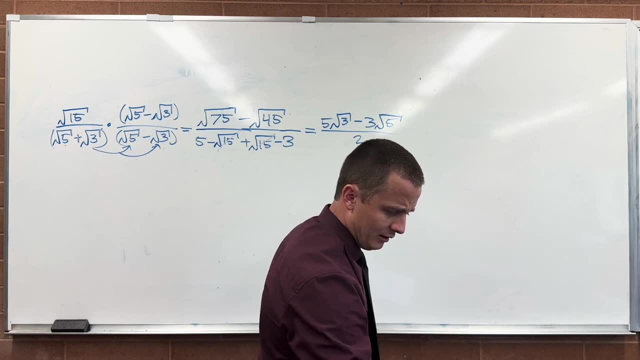 All over 5 minus 3.. 5 minus 3 is 2. 2. There, it is Not too bad, Okay. Okay, Trying to pick one that might get messier. Okay, This one looks messy. 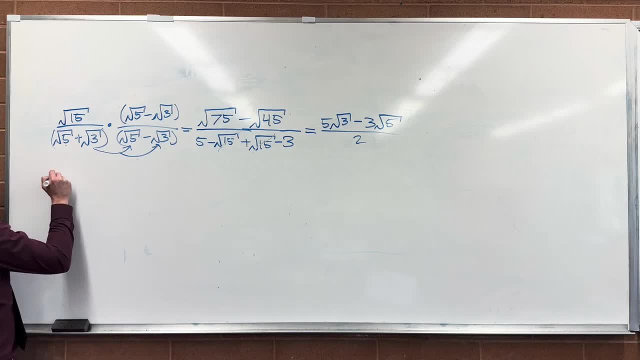 So Let's try this one. This one: we have 3x, square root of 2x plus square root of 4x, cubed all over 5x minus the square root of 3x. Okay, Looks busy, Looks like it has a lot going on. 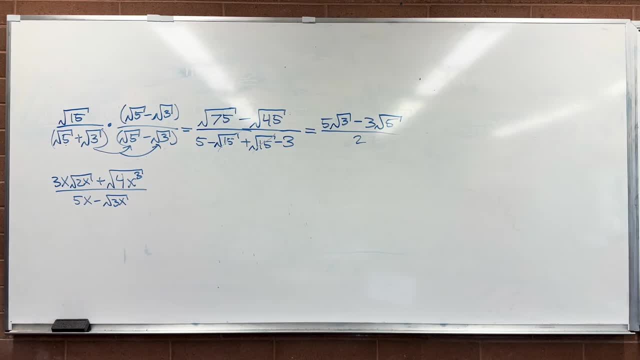 How on earth do we start this problem? What do we do? What do we do? Your conju Multiply by the conjugate Yeah, Yeah, It doesn't get any easier than that. We could, if we wanted to calculate some square roots first. 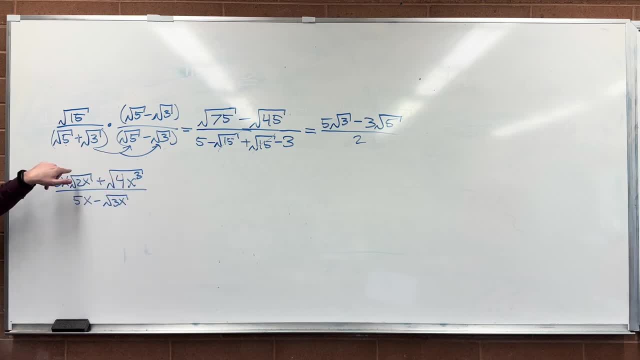 So we can look at each term and see if we can pull something out first That will makes up. when we're multiplying we don't get really big numbers. Could you hear x's? So looking at this one, we have 3x. 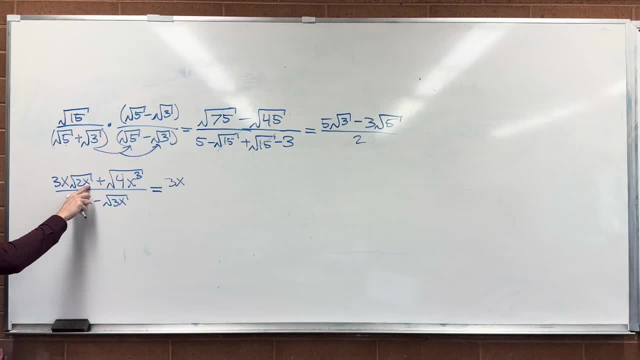 Can I pull anything out of 2?? No, Can I pull anything out of x? No, So that stays the same. So that's still square root of 2x, But look at this one. Can I pull anything out of 4?? 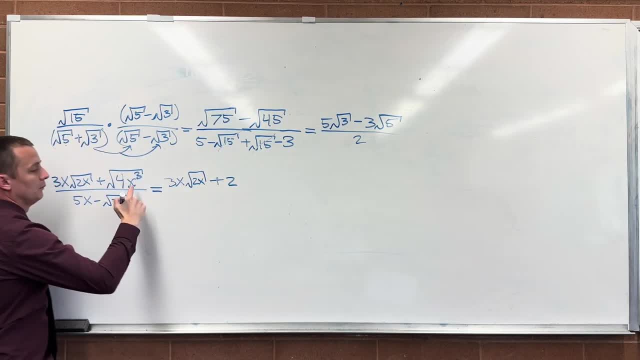 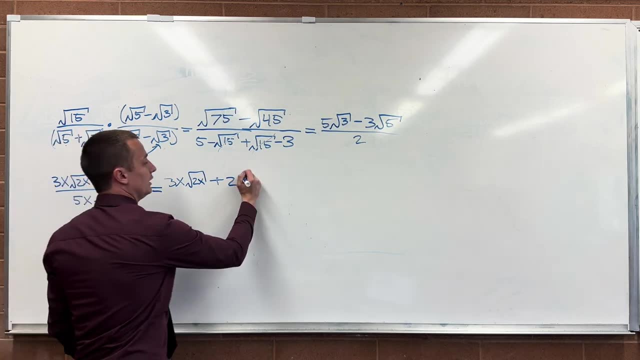 Yeah, I can pull the whole thing out, So that becomes 2.. Can I pull anything out of x cubed, x squared, x squared, pulling it out, leaving me an x, And so x square, root of x right. And then in the denominator, we're still stuck. 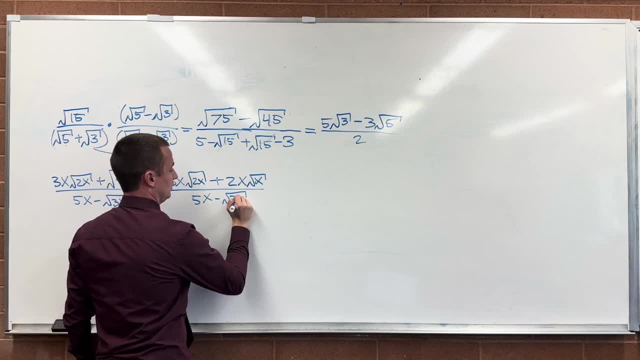 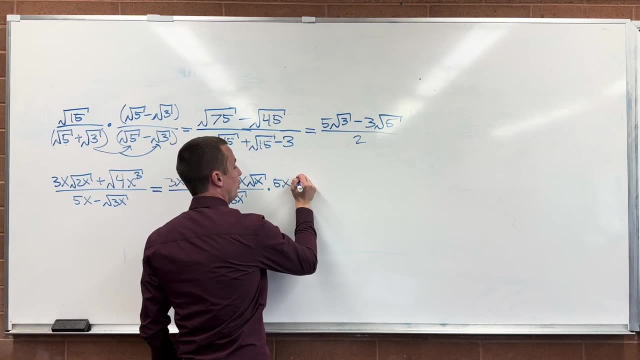 It's still 5x minus square root of 3x. So now we multiply by the conjugate top and bottom. We're going to multiply by 5x plus the square root of 3x And 5x plus the square root of 3x. 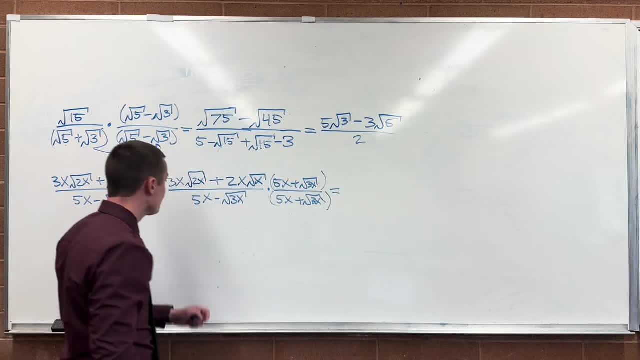 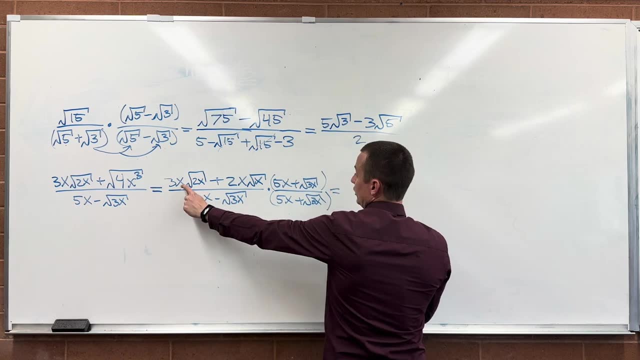 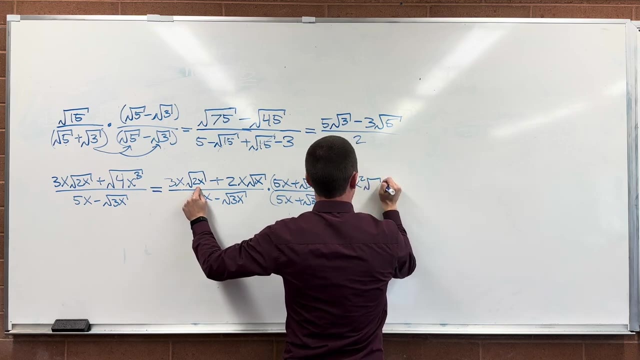 So multiply that top and bottom to both these and see what we get. All right, 5x to this: what do we get? So multiply the 5x to that, what do I get? 15x squared Root, Square, root of 2x. 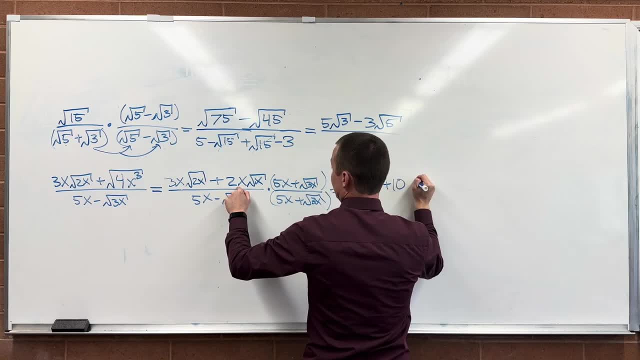 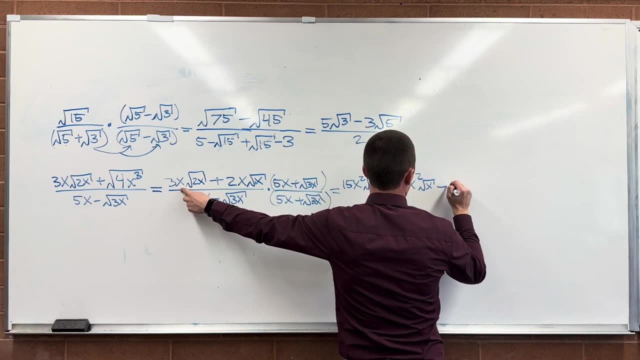 Multiply the 5x to this: what do I get? 10x squared- 10x squared square root of x. Multiply the square root of 3x to this, and what do I get? 9x squared? No, the square root plus the square root. 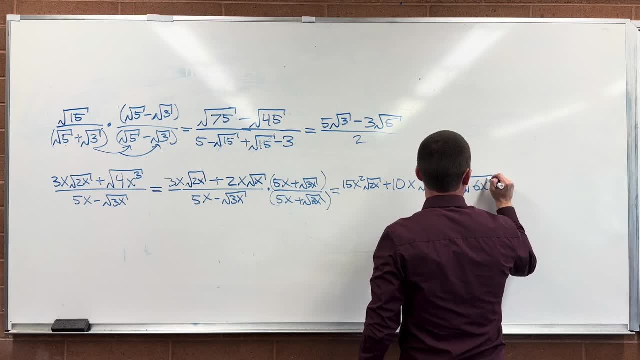 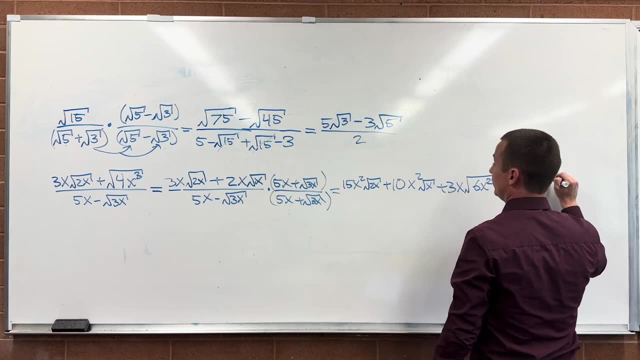 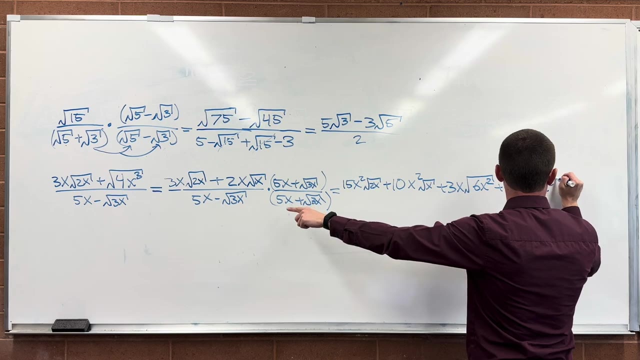 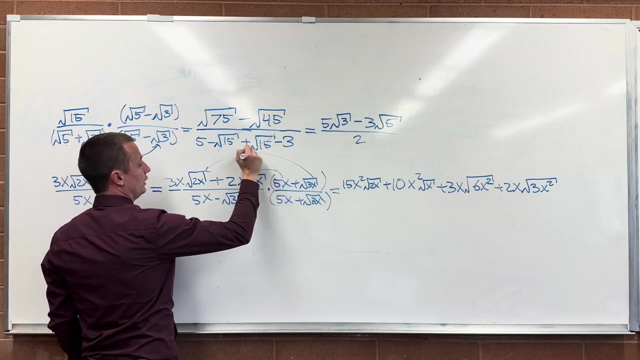 So 3x square root of 6x squared, right, Yeah, Okay. And then square root of 3x to this gives me plus 2x times the square root of 3x squared. Did I do that right? So I multiplied 5x to this, multiplied 5x to this and then multiplied root 3x to this. 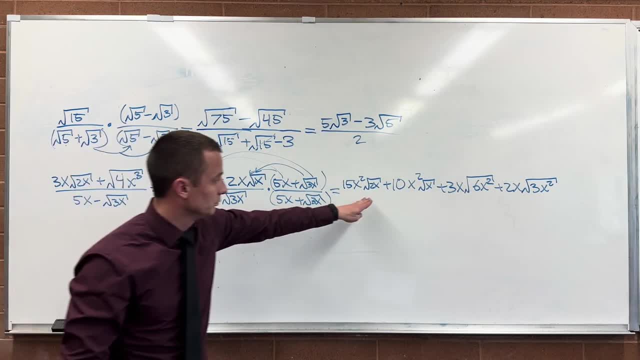 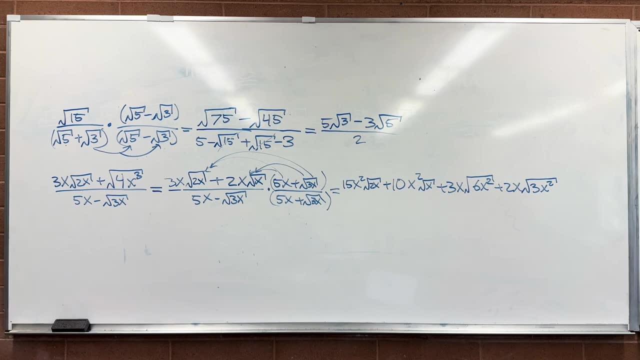 and then multiplied root 3x to this to get these four terms Good, Did I mess up any of them? 15x squared 2x 10x squared square root of x. 3x Square root of 6x squared. 2x square root of 3x squared. 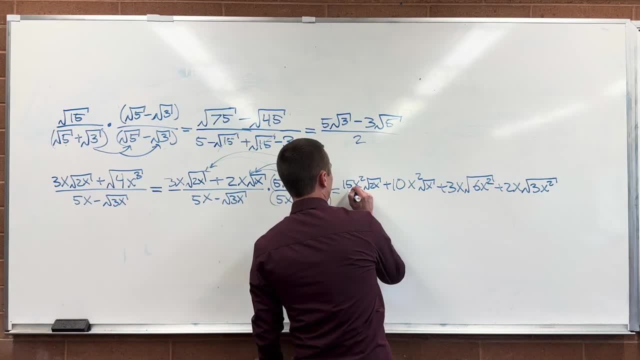 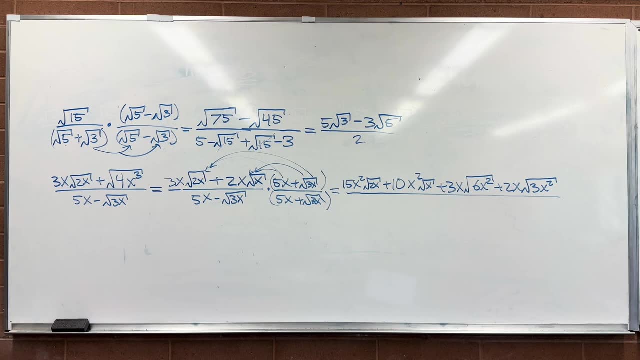 Okay, That is a wrong equation. Oh, I'm just writing bitch, Yeah. Yeah, it's got four terms. come on, Yeah, it's a small term though, Yeah, And now you can multiply out this whole thing and notice that things cancel. 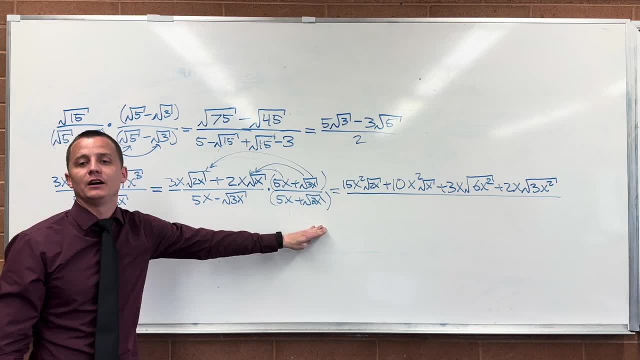 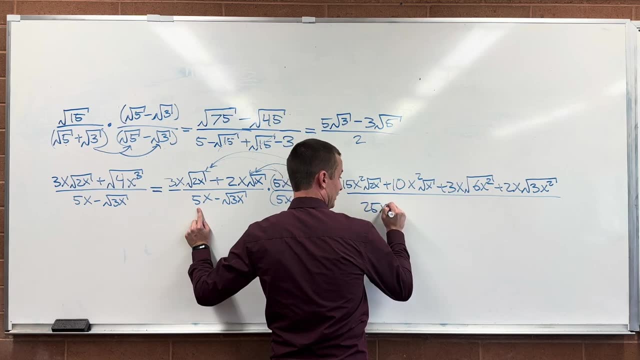 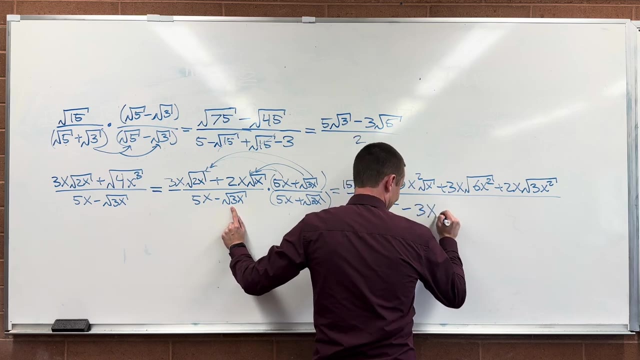 Or you can know that a minus b times a plus b, is always and forever a squared minus b squared. So it's just going to be a squared which is 25x squared. Good Yeah, Minus b squared Um 3x squared. 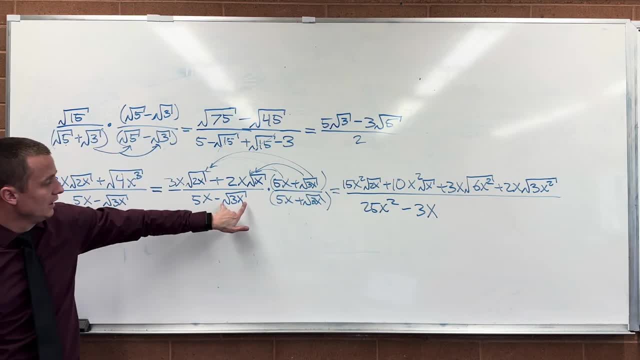 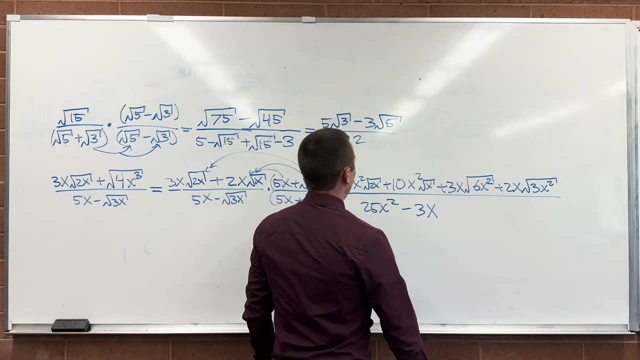 No, Ah, It's just 3x. It's just 3x. Yes, If you take something under a square root and multiply it by itself, you just get the thing under the square root. Yes, Okay, I always make a mistake. 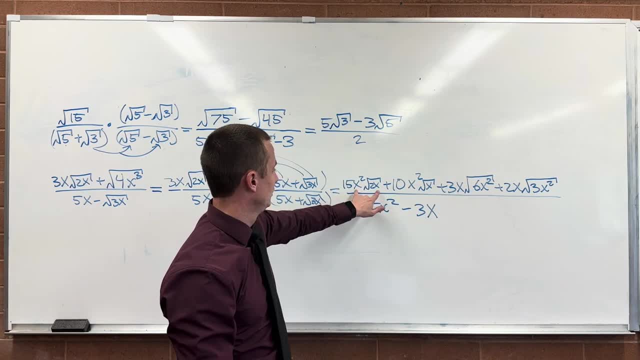 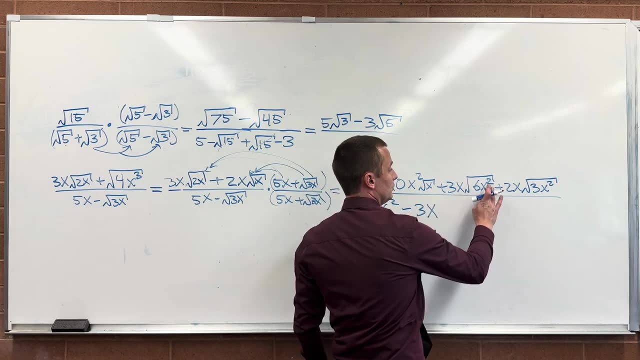 So now let's see what we can do with any of these That we can't do anything with. That. we can't do anything with This. we can pull out the x squared, X squared. Yeah, I'm just going to erase the x squared here and make that a squared. 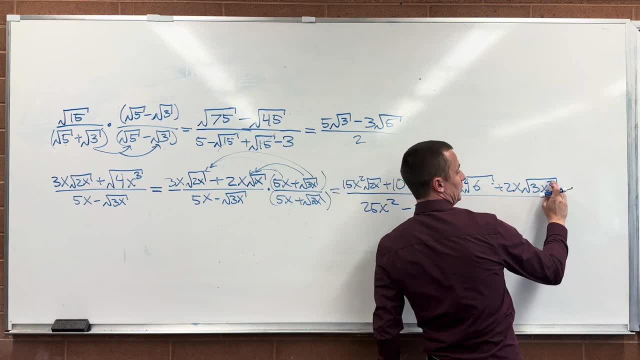 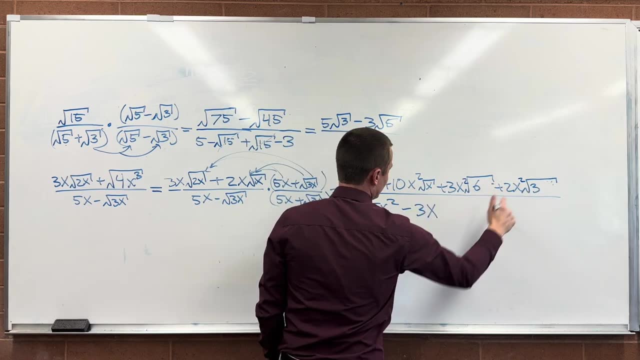 So I pulled an x out And this one. I can do the same thing. I can pull out the x squared and make that a squared. So I have a squared of 2x, a squared of x, a squared of 6, and a squared of 3.. 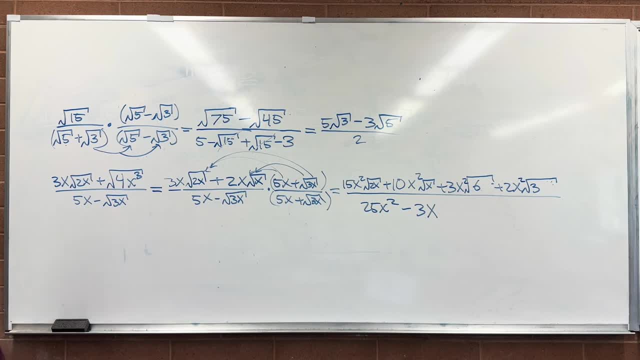 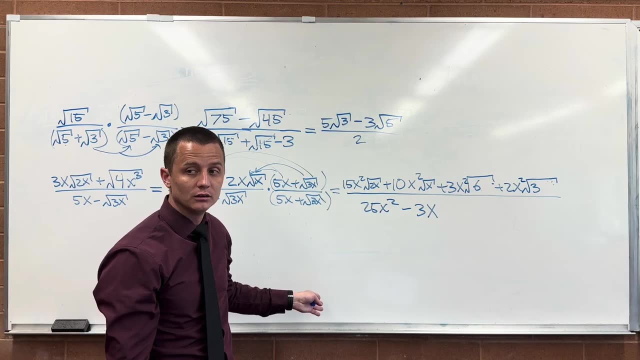 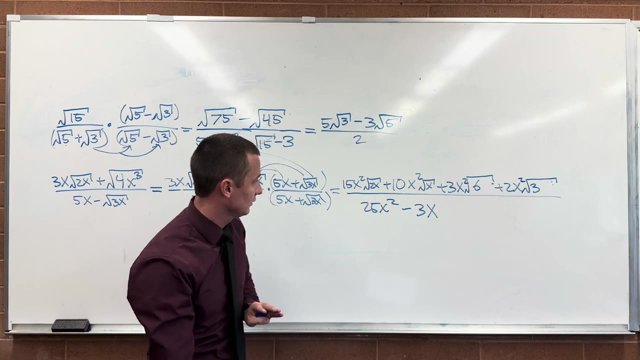 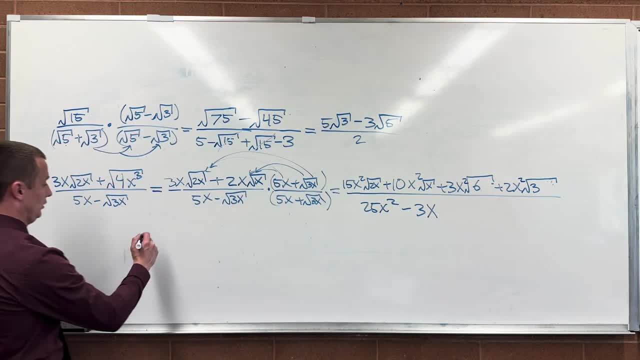 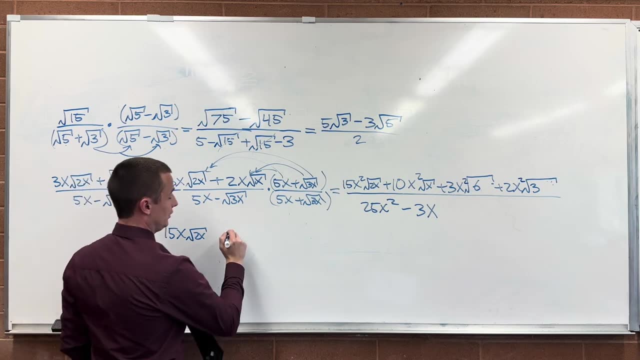 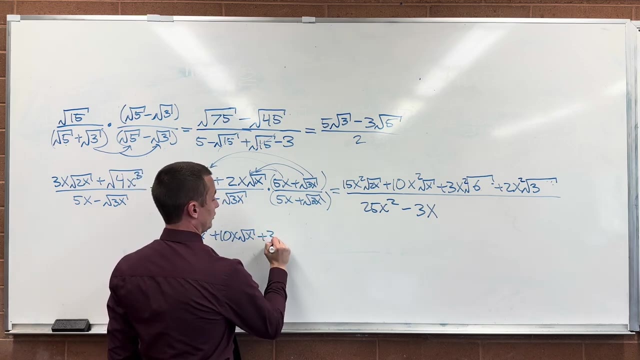 That has an x, That has an x, So I can pull an x out of everything And I don't see anything else I can do. So let's write that. So I see 15x square root of 2x plus 10x square root of x plus 3x square root of 6 plus 2x. 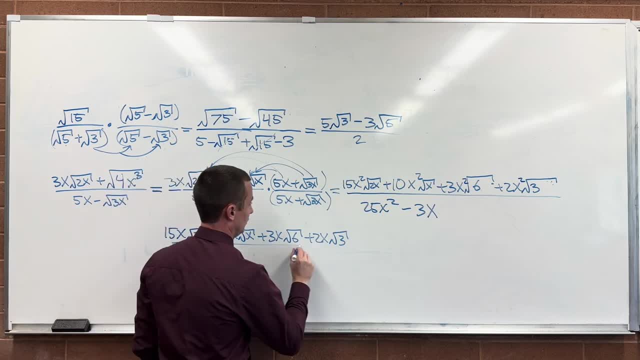 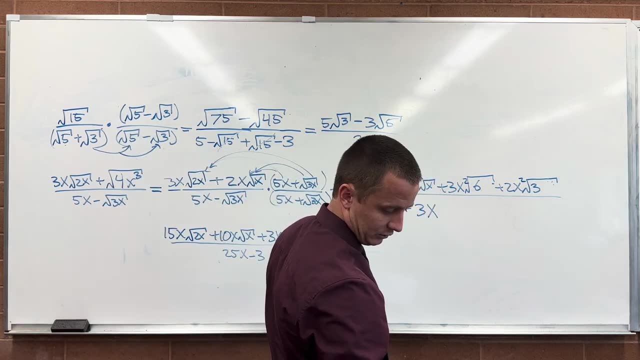 square root of 3.. All over 25x minus 3.. Good, And let's check the author's answer: 15x square root of 2x, 3x square root of 6,, 10x square root of x, 2x square root of 3,. 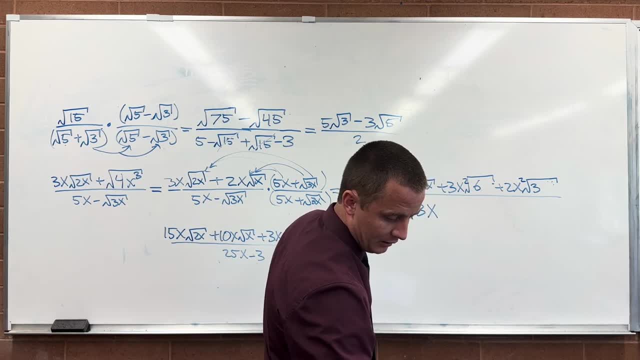 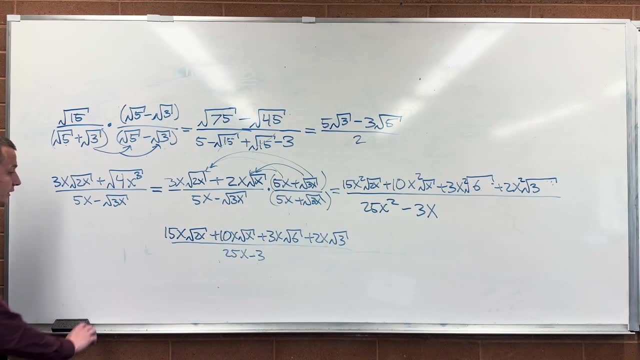 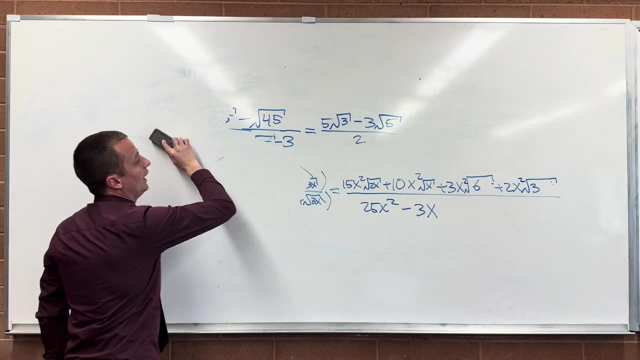 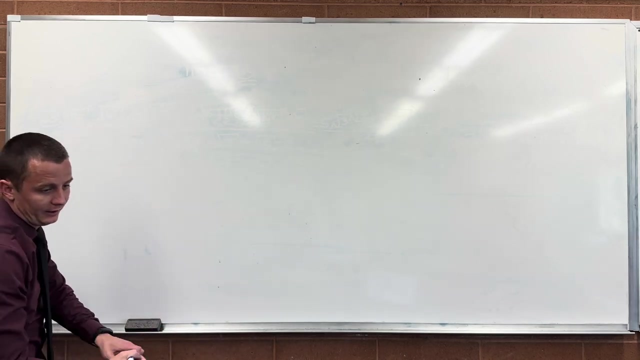 all over 25x minus 3.. All right, Got the same thing, And that concludes the first section. All right On to the next section. The next section is converting back and forth between using radical notation and exponent notation. So what do we mean by that? 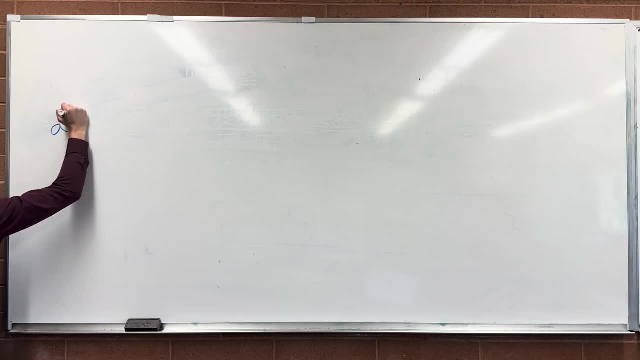 We mean by that that a to the power of n over m is the same thing as the mth root of a to the n. Let's see this in action. And if I told you I want you to calculate a to the two thirds, this would be the same. 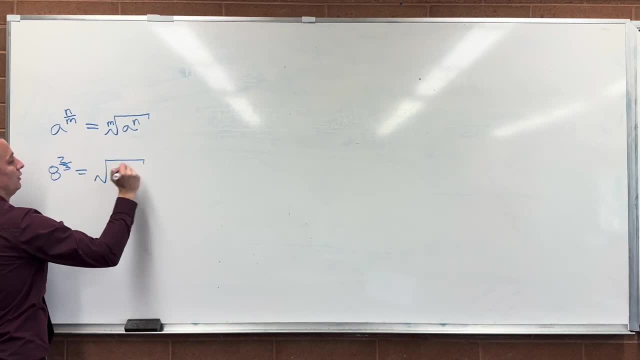 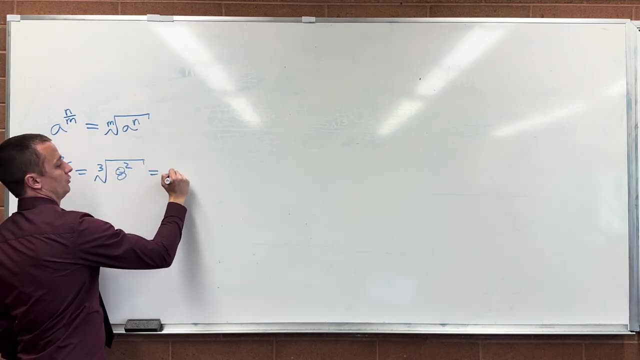 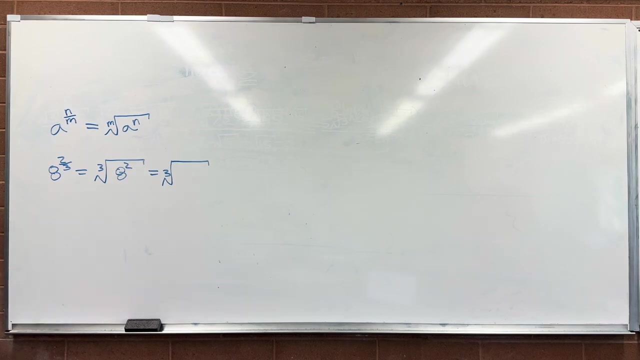 thing as calculating the cube root of a squared. So your denominator is what? So this? yes, Your denominator is what goes on the outside. Your numerator is what goes on the inside. 8 times 8 is 64, and what's the cubed root of 64? 4.. 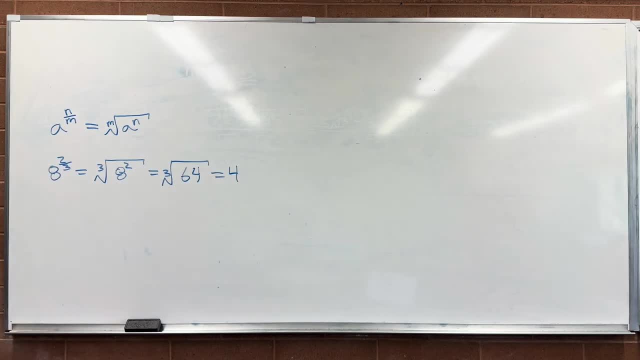 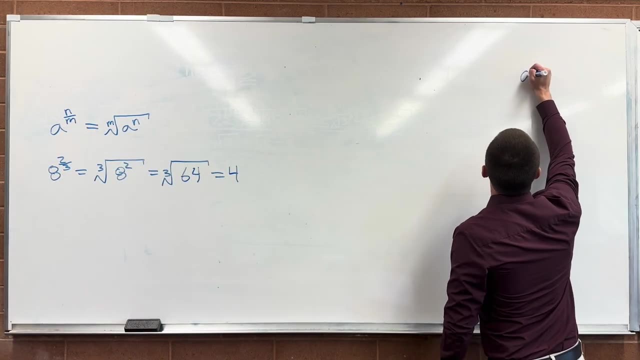 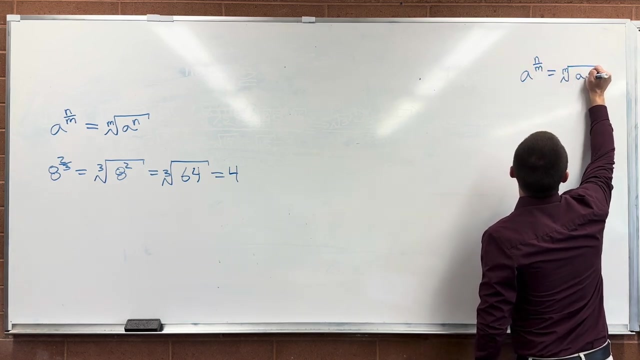 So 8 to the 2 thirds is 4.. So this is a principle we use back and forth. Let me write that over here because we use it a lot. So a to the n over m is the same thing as the nth root of a to the n. 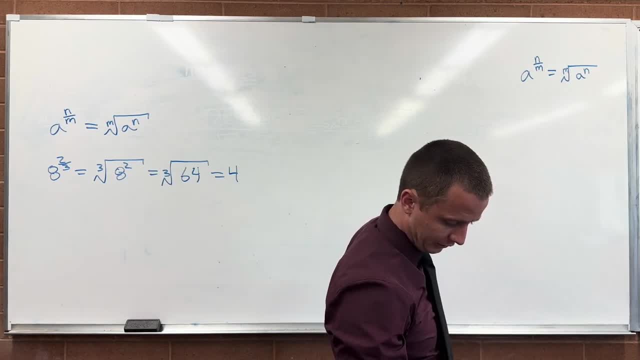 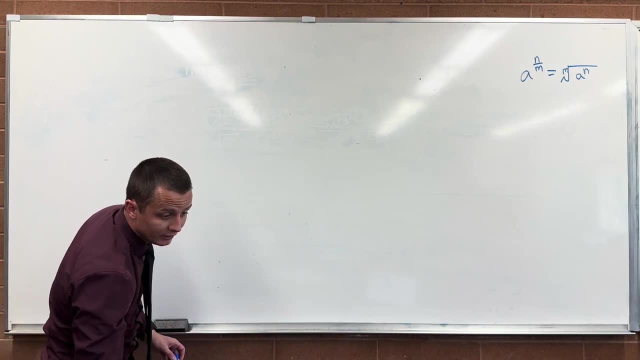 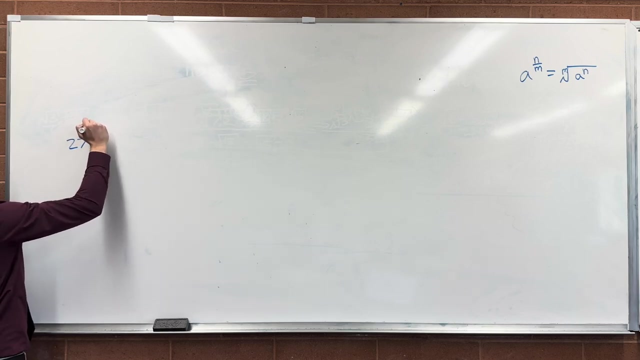 Okay, so let's work through some examples. So the first one: the author wants us to calculate 27 to the negative 4 thirds. So we're looking 27 to the negative 4 thirds, And he wants us to write this with radical notation. 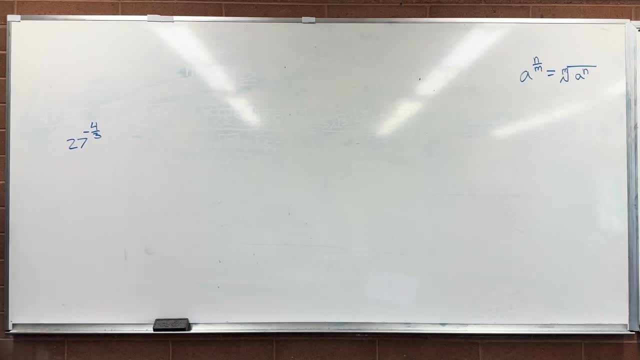 That's all he wants us to do. Okay, first off, it has a negative exponent. I hate negative exponents. What do I do with a negative exponent? to get rid of it, Put it in the denominator: a to the negative m is the same thing as 1 over a to the positive m. 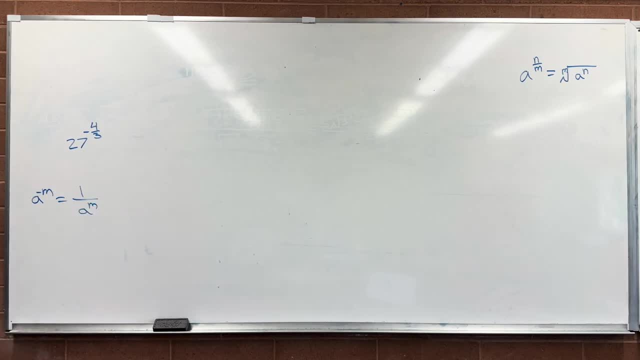 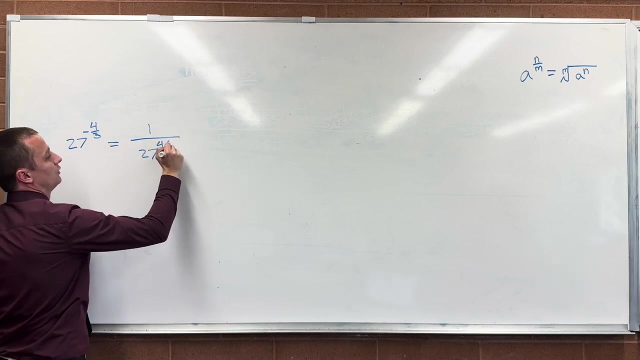 If you put it in the denominator, it makes the exponent positive. That's what I'm trying to say. Okay, so this is equal to 1 over 27, to the 4 thirds, Right, Okay. Okay now what do we do? 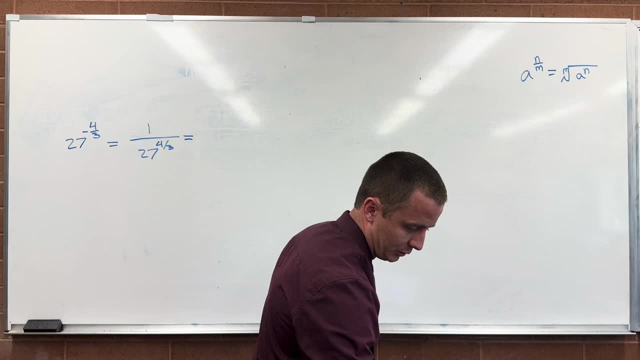 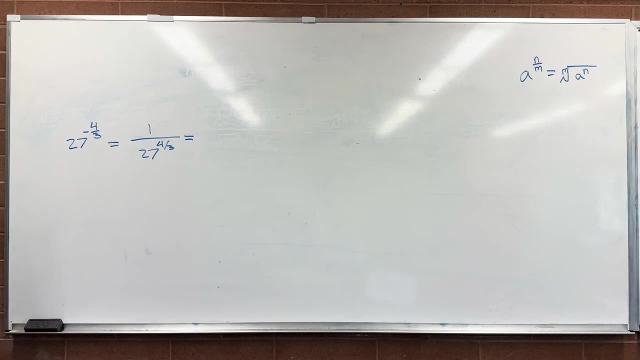 Right, we can use that same notation. I wonder if he wants us to actually just calculate this number. Yes, we can calculate the number. Okay, Now, 27 to the 4 thirds, this is 1 over. Two ways we can think about this. 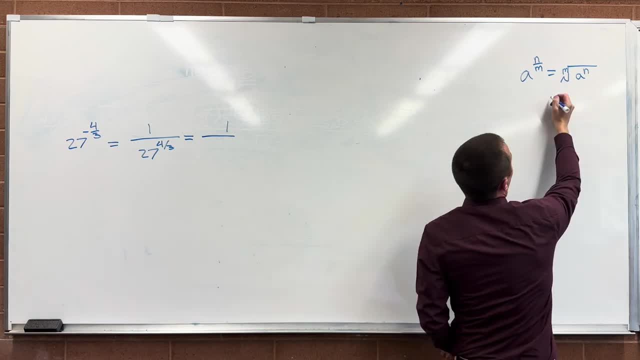 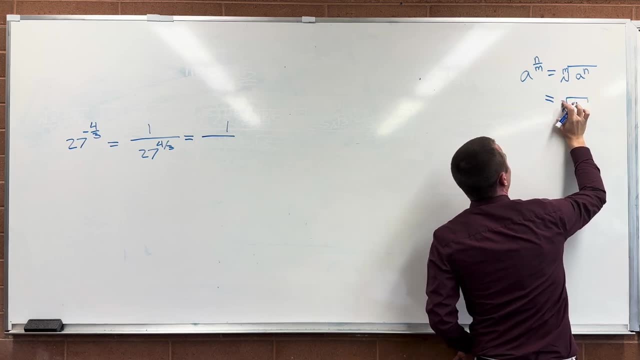 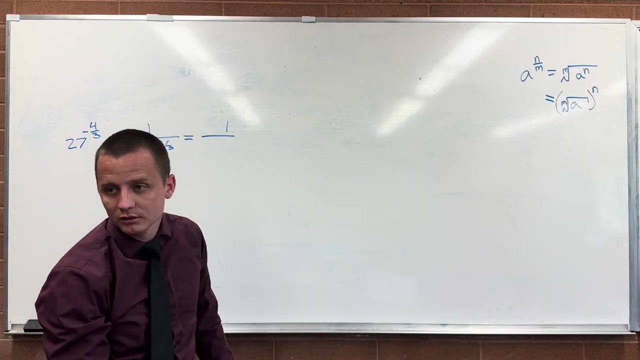 I can think about this as the nth root of a to the n. I can also think about this as The nth root of a- Sorry, The nth root of a all to the power of n. Those are logically equivalent. You with me. 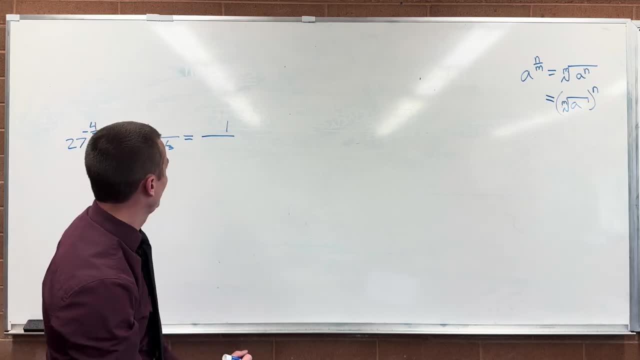 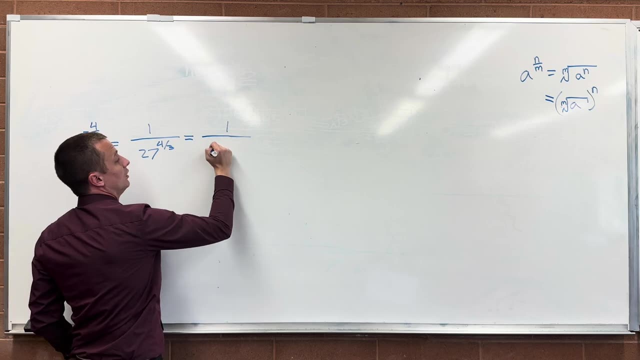 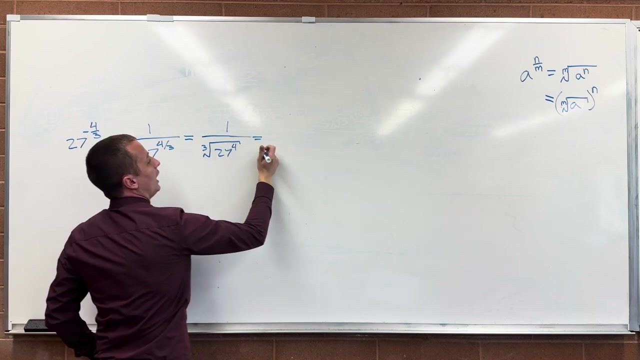 Mm-hmm. Okay, So 27 to the 4 thirds. I can either write this as I can say this is the cubed root of 27 to the 4. Or I can say I can say that this is. 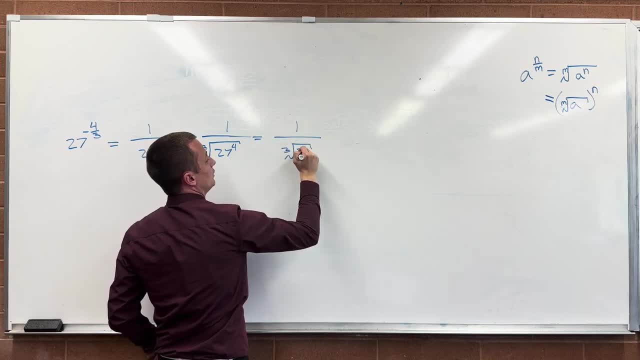 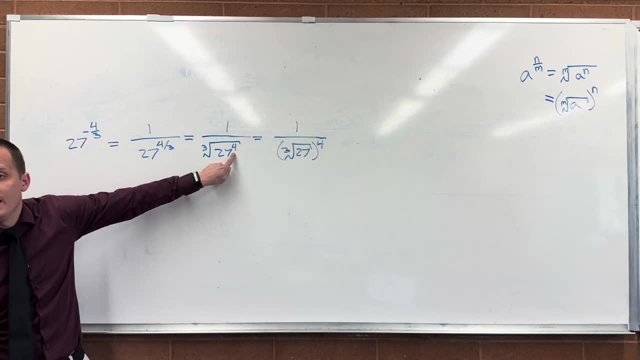 Take the cubed root of 27 and raise it to the power of 4.. What do I want to do first? Do I want to raise 27 to the power of 4 first, or do I want to take its cubed root first? 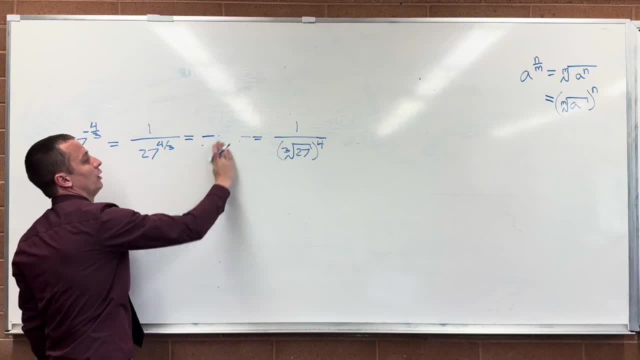 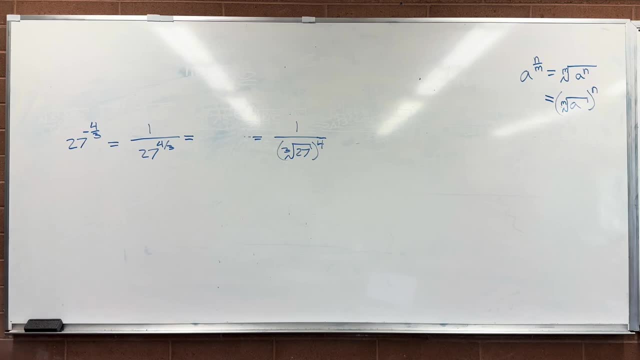 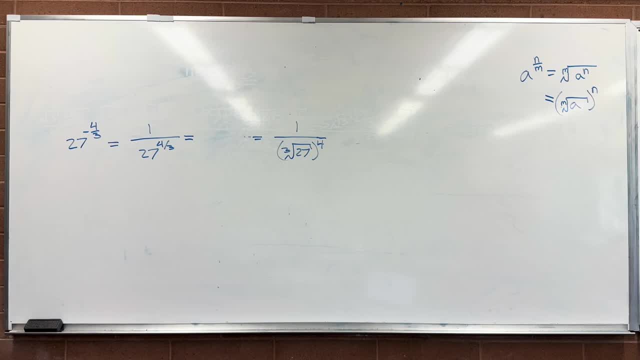 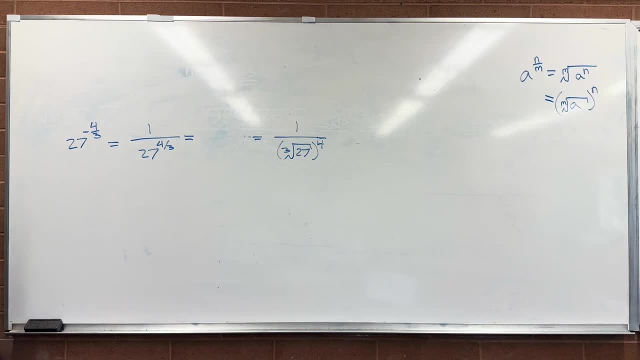 3.. Try again: 3.. 3 times 3 times 3 is 27.. So this is equal to the same thing as 1 over the cubed root of 27.. That's just 3 all to the power of 4.. 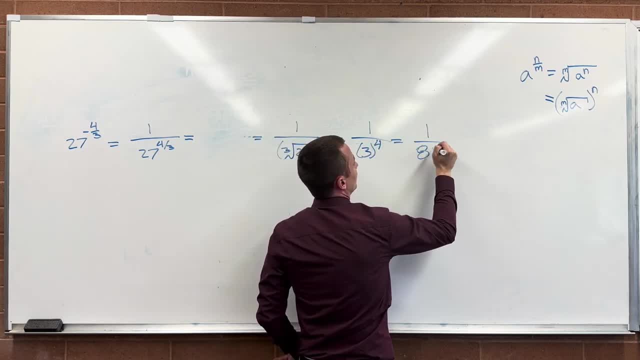 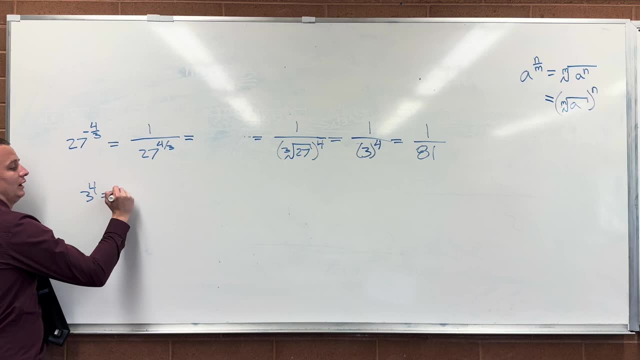 And now, what's 3 to the 4? 3 to the 4.. What's 3 times 3 times 3 times 3? 36.. 3 to the 4 is the same thing as 3 squared times 3 squared. 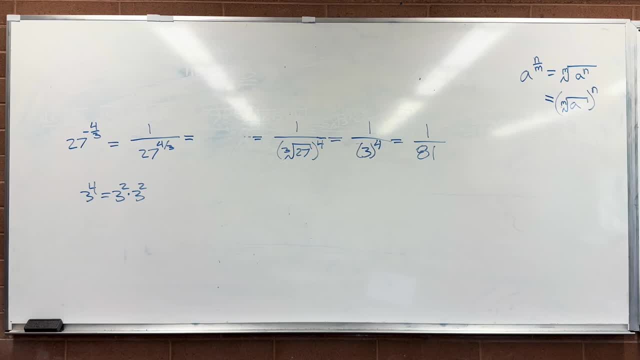 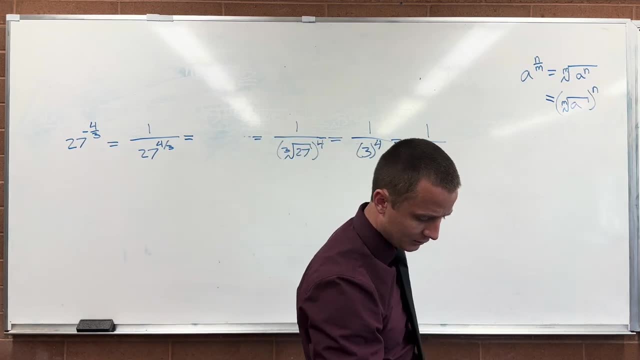 Just do 2 and then do 2 and then put it together. 9 times 9 is 81.. There you go. So 1 over 81 is the answer to what. that is All right, Let's It reminds you of all your exponential properties. 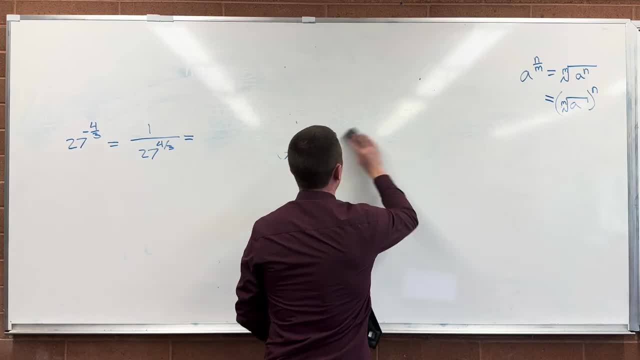 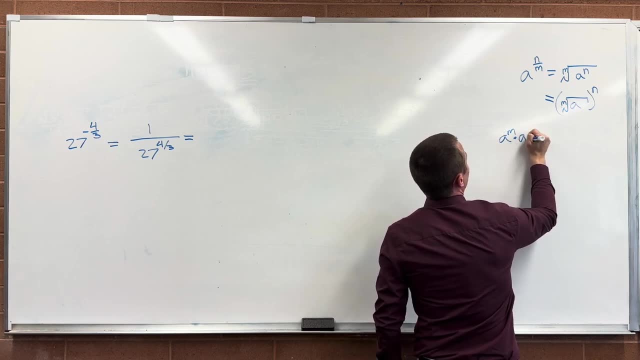 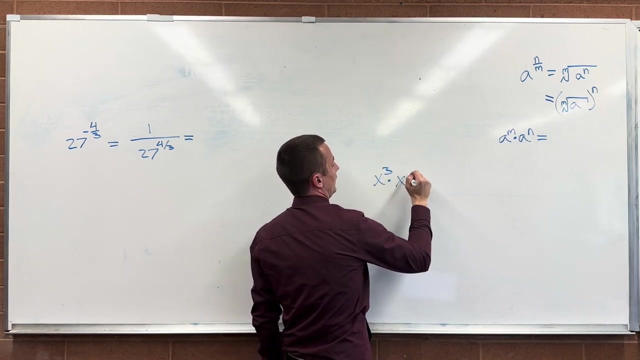 These are all things we've already talked about, but we can rewrite a bunch of them out. We'll just write them over here in the margin. So a to the m times a to the n is equal to what? If I have x cubed times x squared, what does that equal? 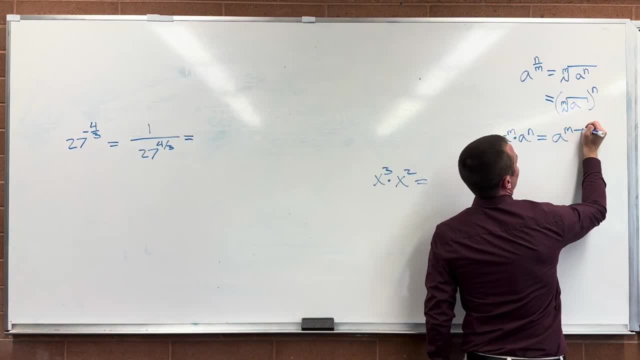 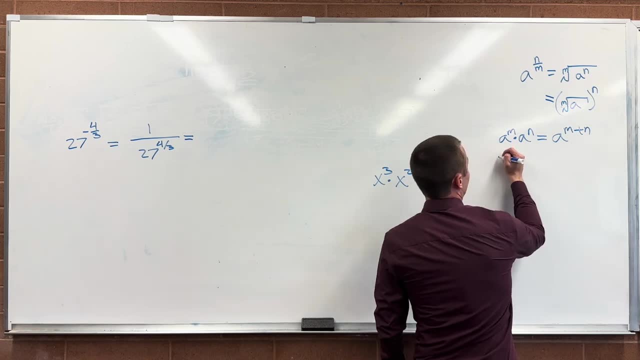 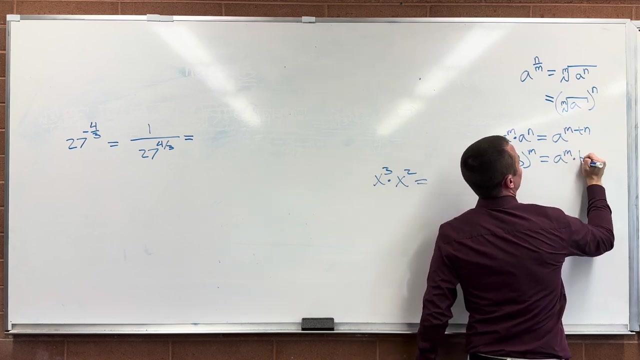 x to the 5.. x to the 5.. So this is just a to the m plus n. So when you multiply terms you add exponents. If I have a times b all to the power of m, this is the same thing as a to the m, times b to the n. 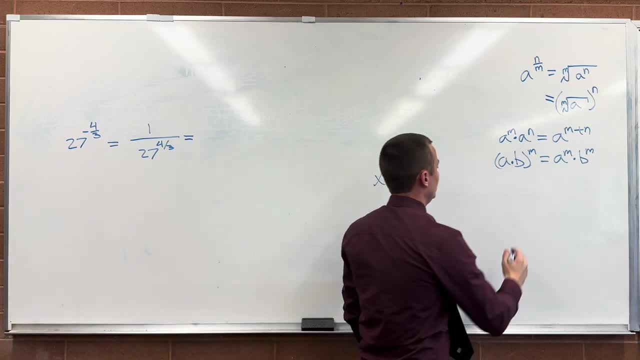 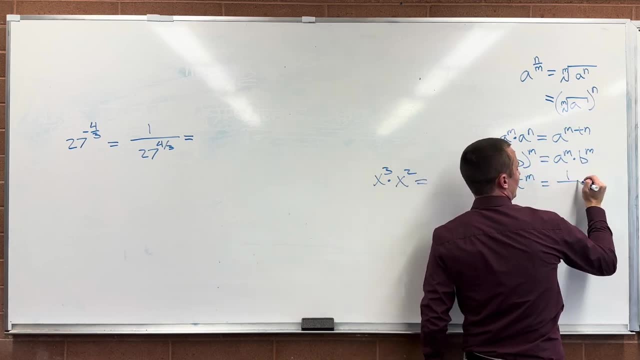 You have to raise both of them to that power. Next one: We already talked about this one: a to the minus m. Why do I keep doing threes? a to the minus m is equal to 1 over a to the m. 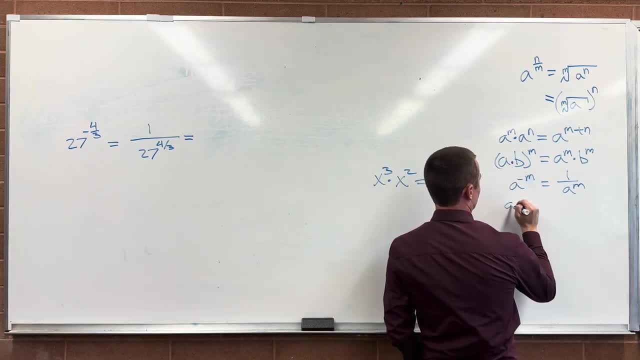 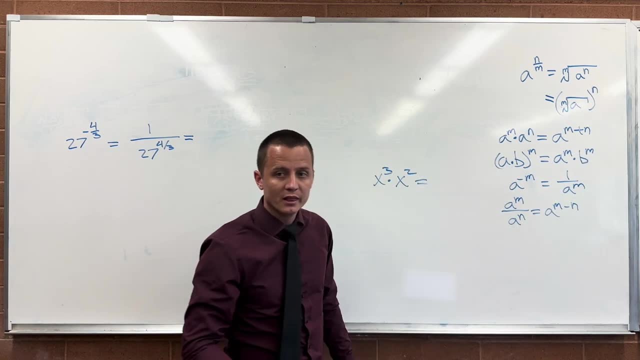 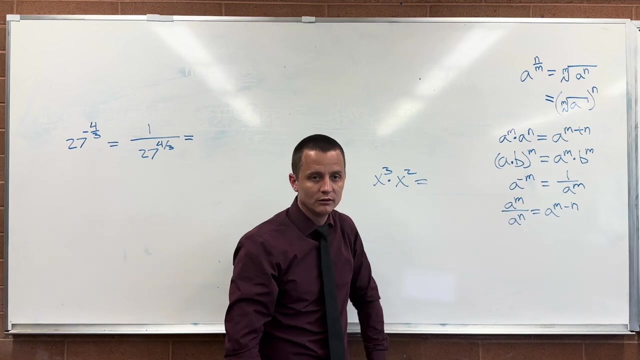 Next one: a to the m over m is just a to the m minus n. How do you get that? Remember, if I take the a to the n and bring it upstairs, it makes the exponent negative. and then just adding them together. 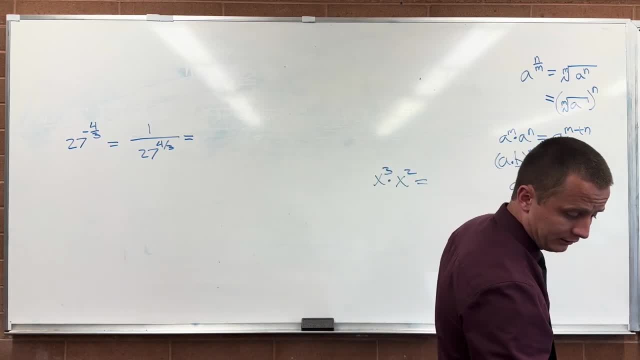 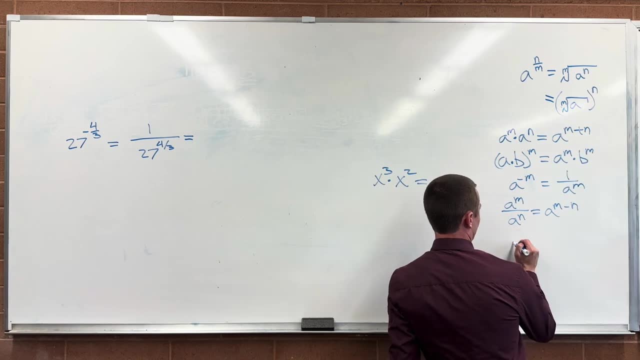 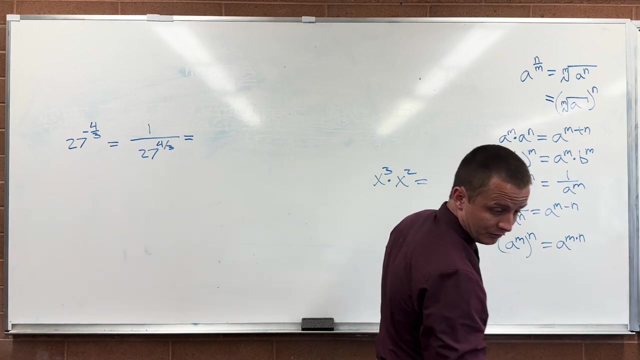 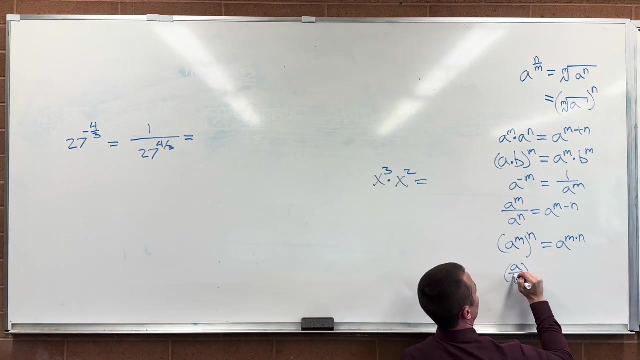 So this one's quickly proved. from this one, Let's see, We did that, we did that. Here's an important one: a to the m, all to the n again is a to the m times n. Another important one: a over b to the negative m is the same thing as. 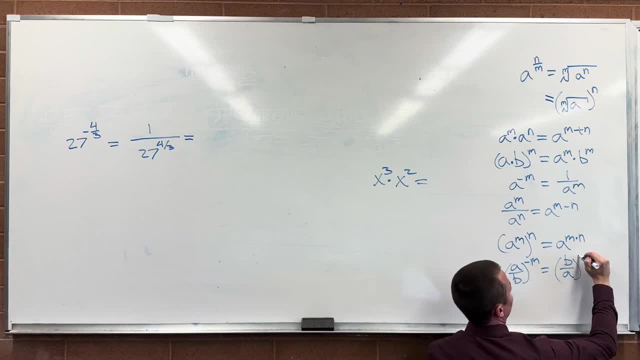 split the reciprocal b over a to the m Good. And then finally our last one: What's a to the power of 0, equal to 1. 1. Anything to the power of 0 is 1.. That's a little too gross. 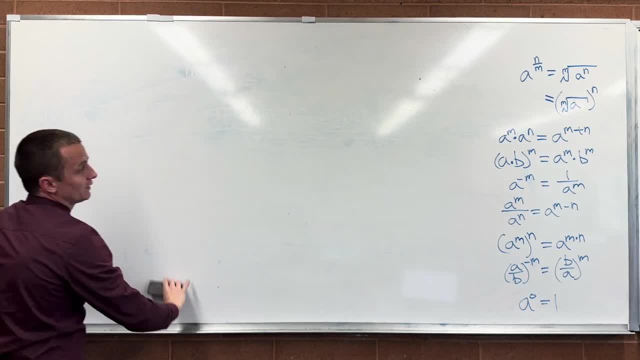 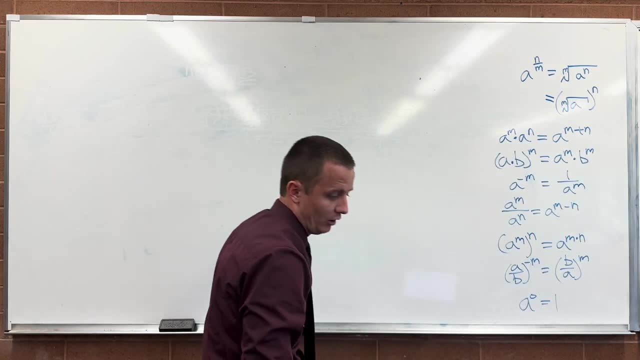 All right. So there's a reminder of the basic exponent rules we'll be using over and over again in this section. So now let's do an example with all this. So a to the 2 thirds. a to the 2 thirds. 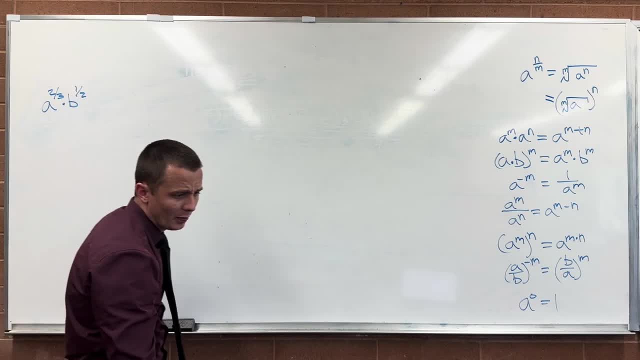 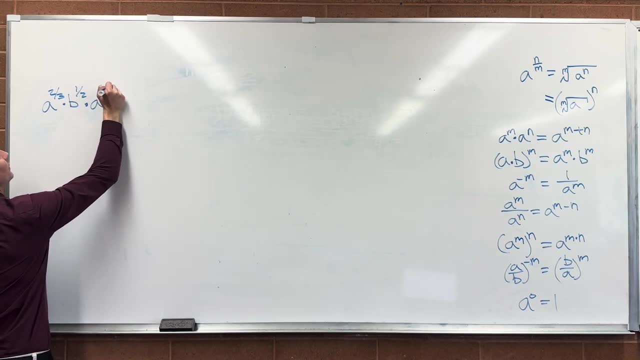 times b to the 1. half times a to the 1. sixth, b to the 1. fifth Times a to the 1. sixth times b to the 1 fifth. OK, When I multiply common terms, I add their exponents. 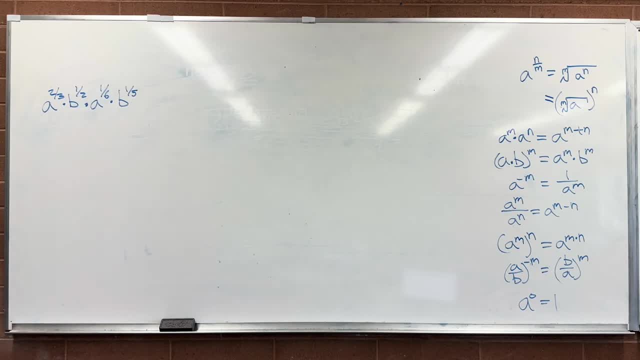 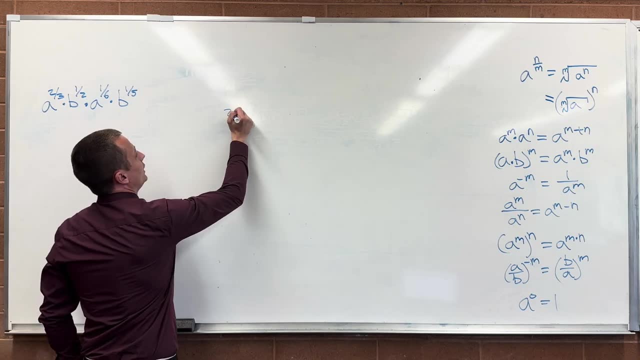 Yeah, So a to the 2 thirds times a to the 1 sixth. When I multiply common terms, I add their exponents. I have to add 2 thirds to 1 sixth. So a scratch work over here. What is 2 thirds plus 1 sixth? 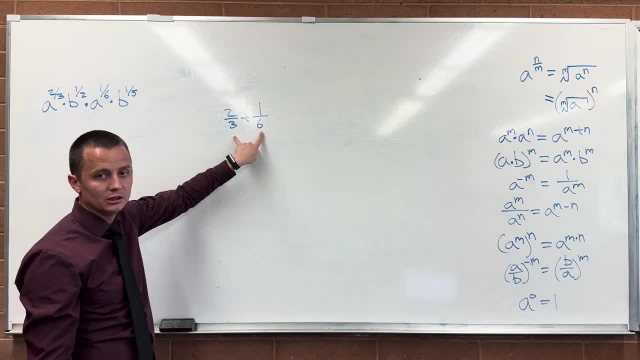 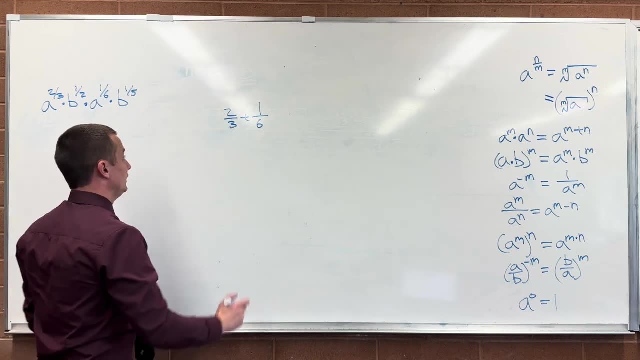 First, I need to get my common denominator. What's my common denominator going to be? 6.. 2. 6 is my common denominator. I need to multiply this top and bottom by 2 to get it, So you have the right idea. 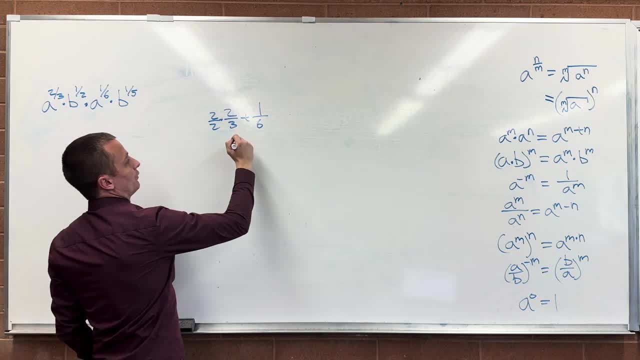 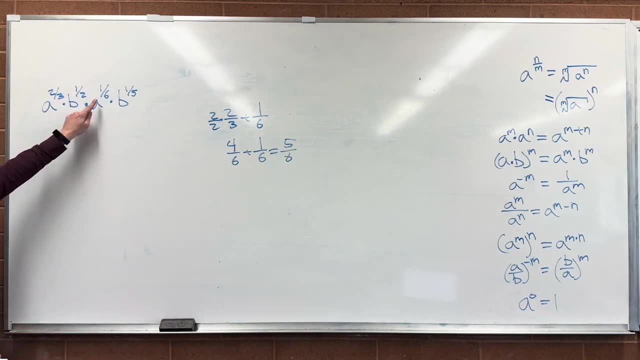 So multiply that top and bottom by 2 to get it. And so we're left with 4 sixths plus 1 sixth is equal to 5 sixths, 5 sixths. So a to the 2 thirds times a to the 1 sixth gives me a to the 5 sixths. 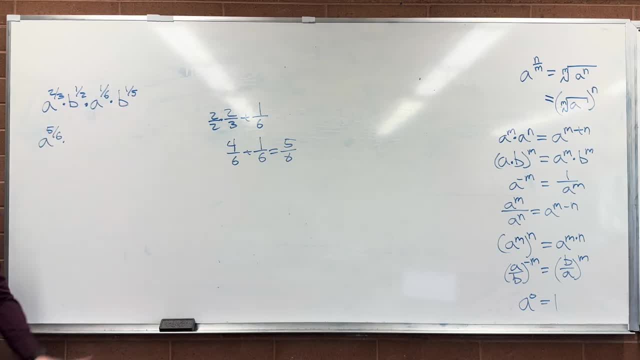 Now we need to combine our b's. 1 half plus 1 fifth is 1 half plus 1 fifth. Mm-hmm, 1 half plus 1 fifth. What is it? What's our common denominator? It's 10.. 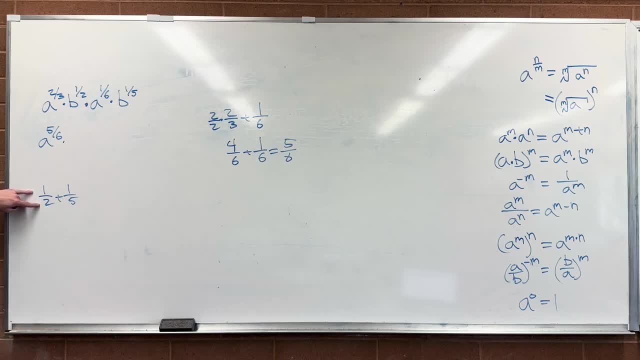 10.. How do I get this to have a 10?? 5. Multiply top and bottom by 5.. How do I get this to have a 10?? 2. Multiply top and bottom by 2. 6. 2.. 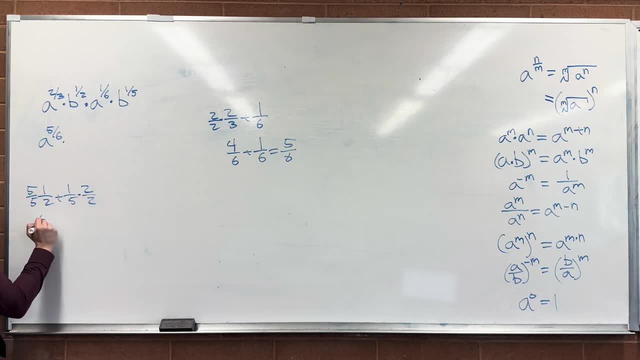 7. 7 tenths. Right, So 5 tenths plus 2 tenths is equal to 7 tenths. Another way you can ask yourself is: 1 half is how many tenths? 1 half is 5 tenths. 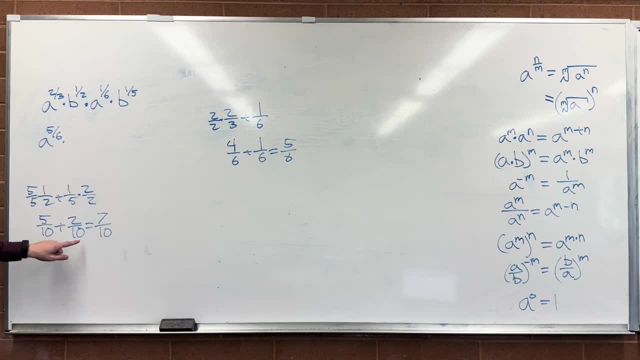 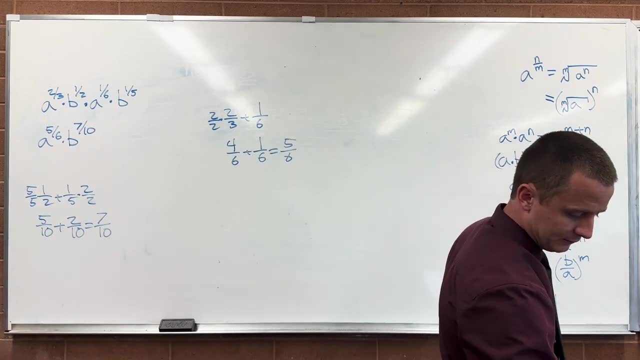 1 fifth is how many tenths? 1 fifth is 2 tenths, 5 tenths plus 2 tenths is 7 tenths. So this is times b to the 7 tenths And that's how you deal with, that's how you combine these terms with these different fractions. 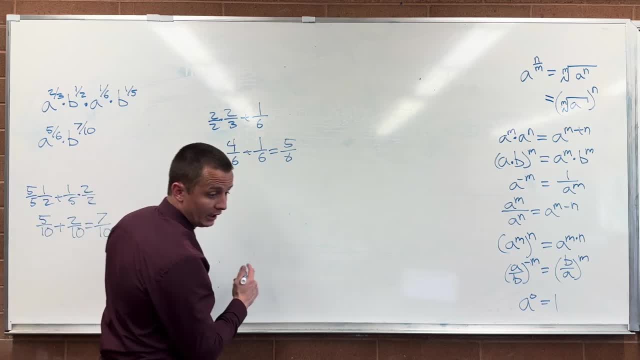 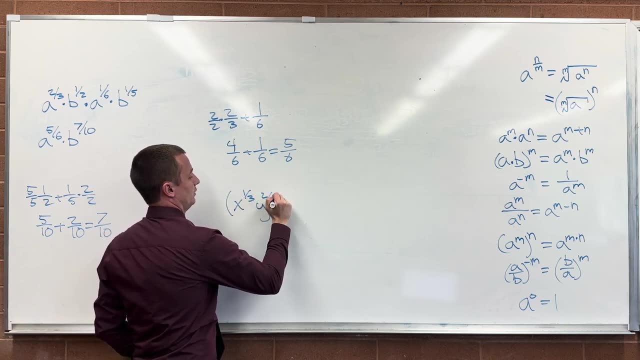 All right, Let's try another one. This one: we have x to the 1 third, y to the 2 fifths, x to the 1 third, y to the 2 fifths, And we're raising this whole thing to the power of 3 fourths. 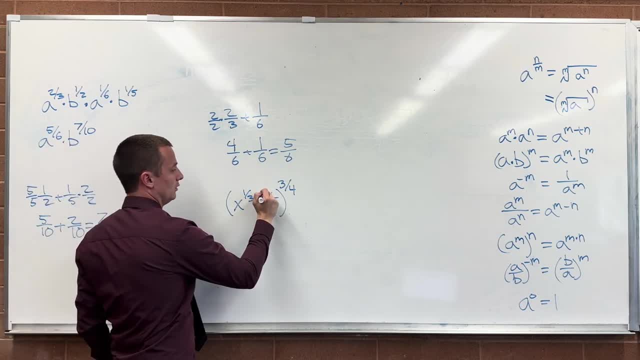 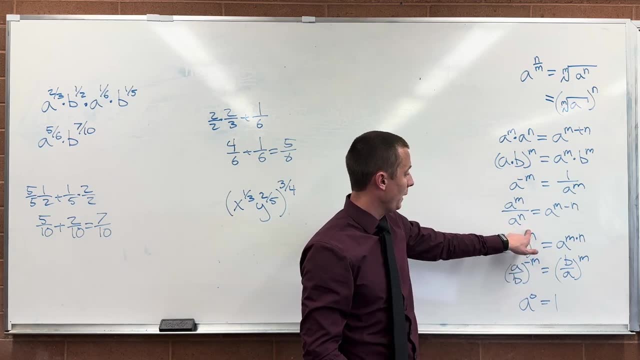 How do you do that? You just multiply. You just multiply. Where's the rule? It's this one: a to the n to the power of n is just a to the m times n. So you just multiply the 3 fourths to each of those exponents. 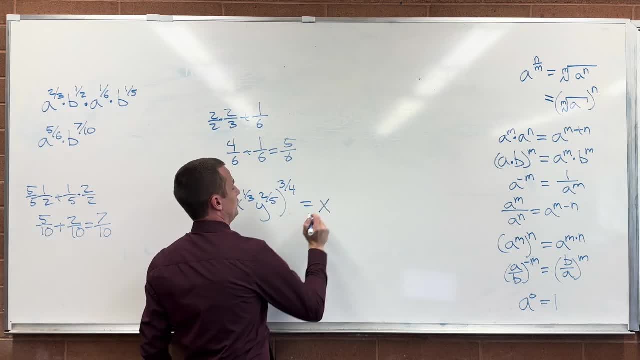 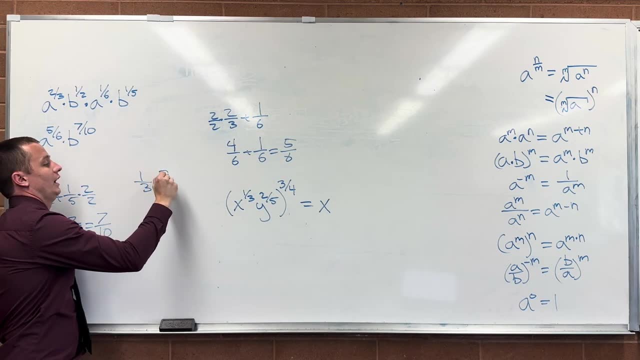 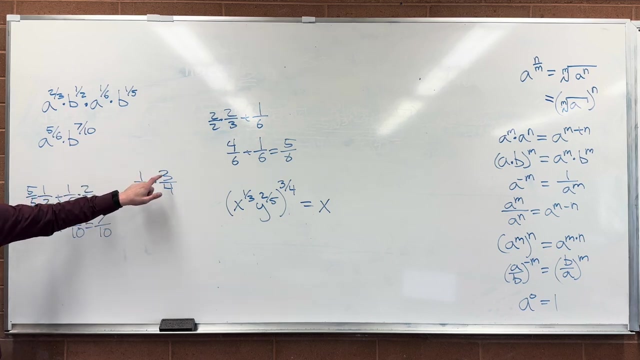 So 3 fourths times 1. third is 3 fourths times 1. third is 1 third times 3 fourths is equal to over thinking it. five. one third times three fourths is, oh, three twelves. I said: oh, there it is the threes. cancel out top of bottom, leaving us with 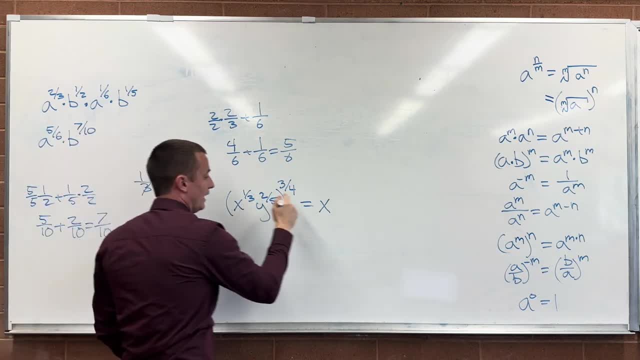 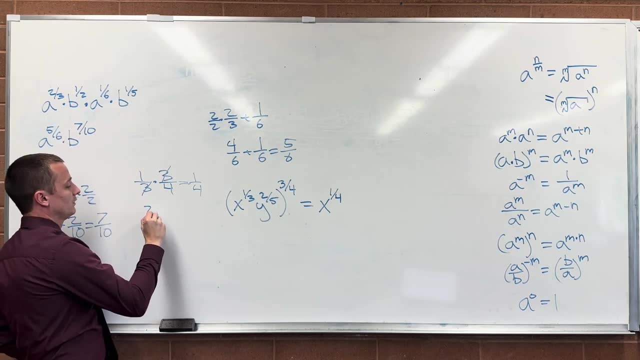 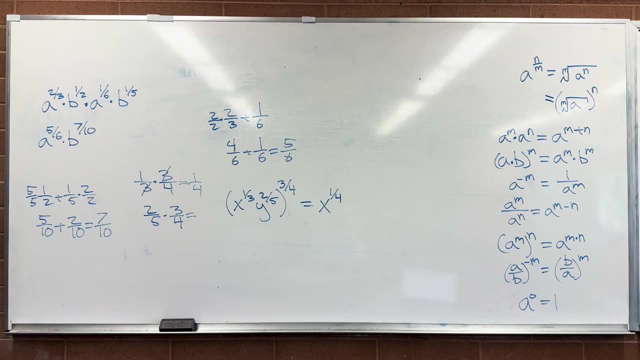 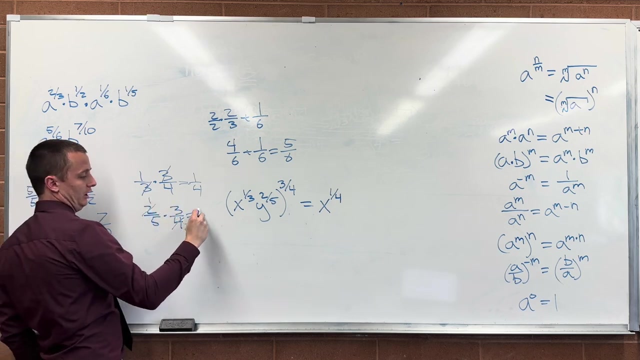 one or okay, so we have X to the 1, 4th. and now let's play this game again. what is 2 this times 3? 4th equal. first off, let's cancel out the 2 before you go nuts with it. that leaves a 1 and a 2 there. so multiplying across 1 times 3 is 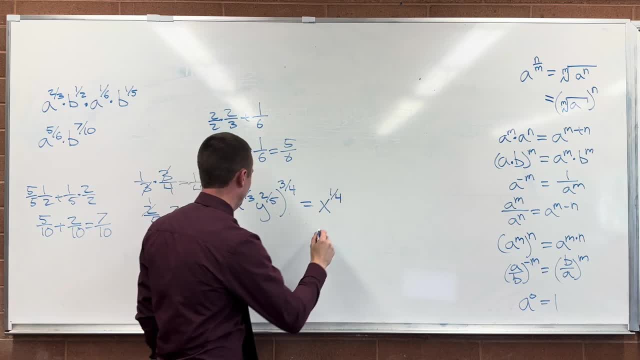 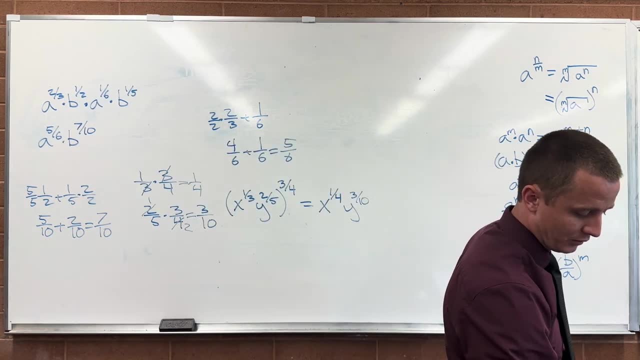 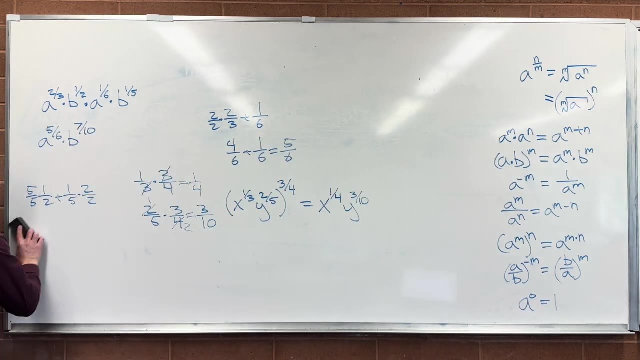 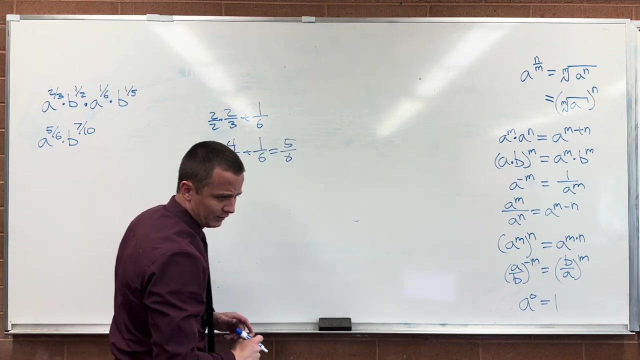 3, 5 times 2 is 10. that easy, right? okay, we definitely need you to do another one of these. actually, let's get this one because he's trying to trick you, and then I'll find another one where we have to multiply the exponents. okay, this one has an x. 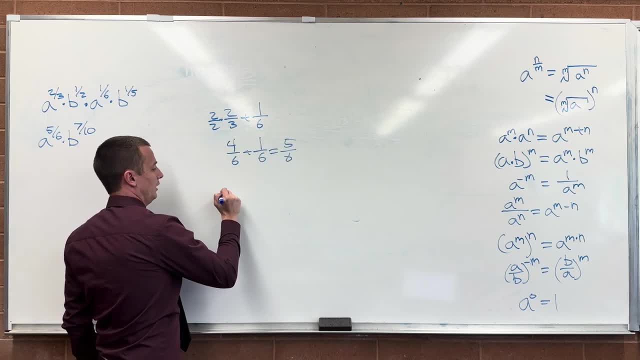 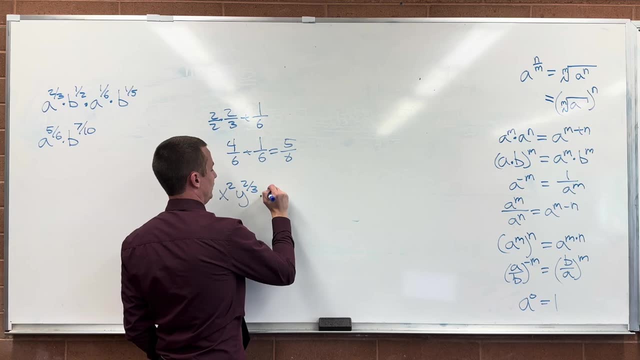 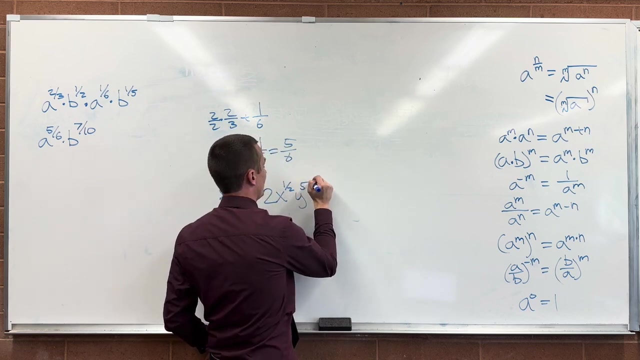 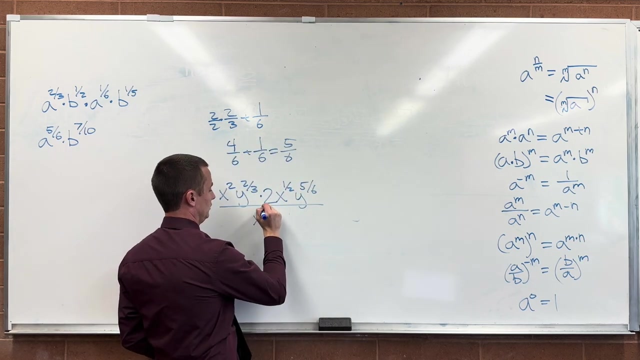 squared y to the 2 thirds. so we have an x squared y to the 2 thirds times 2x to the 1 half times 2, x to the 1 half, y to the 5, 6 all over, x to 7 halves, y to 0, now y to the. 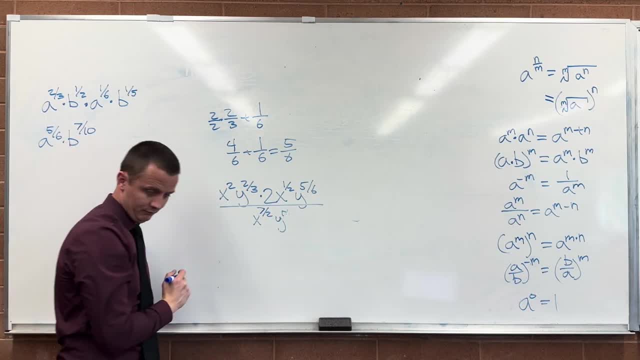 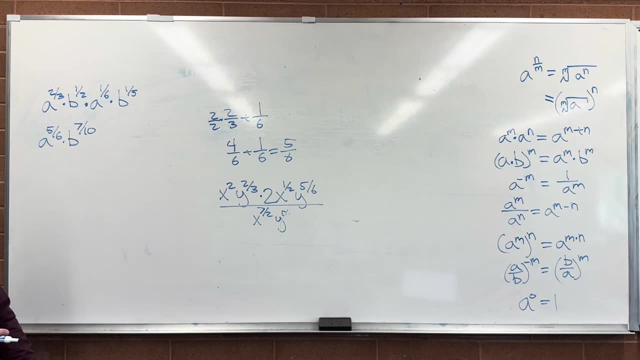 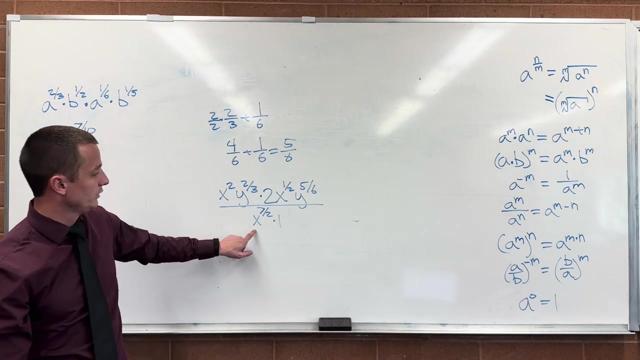 0 is 1, so we don't even have to worry about that. same as multiplying the denominator by 1. so that's going to be his first gotcha, so you just cancel it out. you can. y to 0 is the same thing is multiplying this by 1. what's when? I? 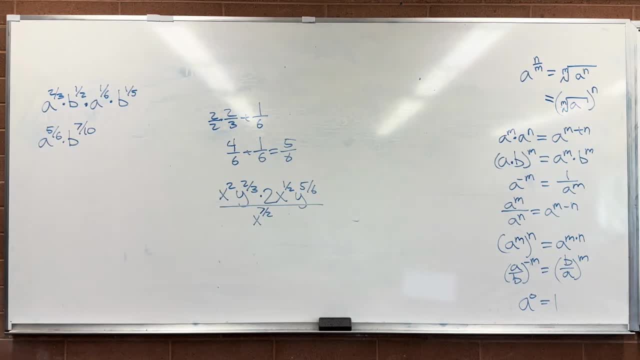 multiply by 1, I just get that number itself. so the y to 0 makes no difference here. okay, so now let's write this out in our numerator: 2 is just 2, that's, we can do with that. now. x squared x to the 1 half, which is what's 2 plus 1 half? we're. 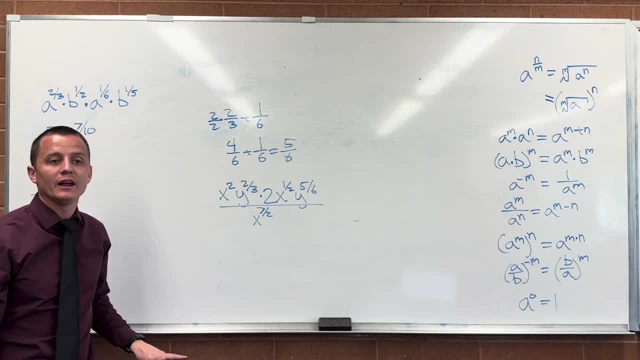 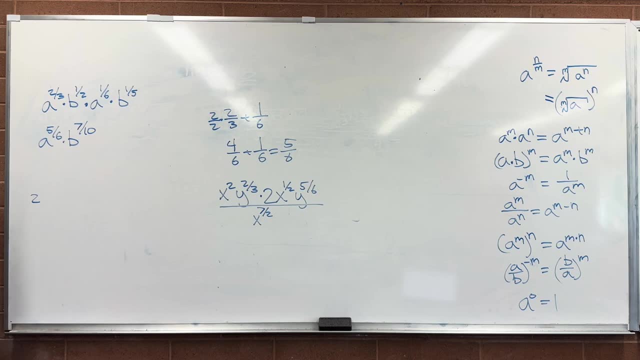 not taking a square root greater than you think we're. when you multiply like terms, you add the exponents. it's what? well, that's gonna be two over one. we're adding the exponents, so two and a half. say that as a fraction. five hats right. 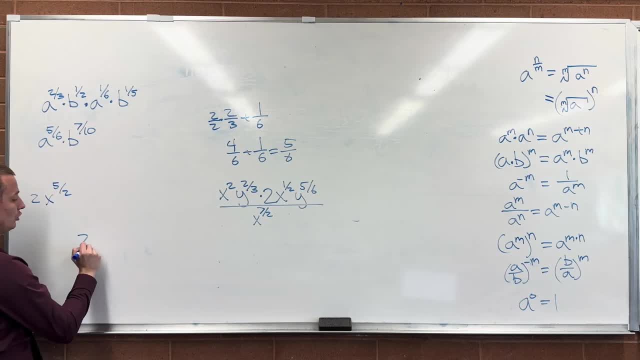 thanks to the five paths, we were doing two plus one half. what's our common denominator again be to multiply this, I top and bottom by 2. 2 over 2, 2 is the same thing as 4 halves plus 1. half gives us 5 pass. okay, why we have 2 3rds plus 5. 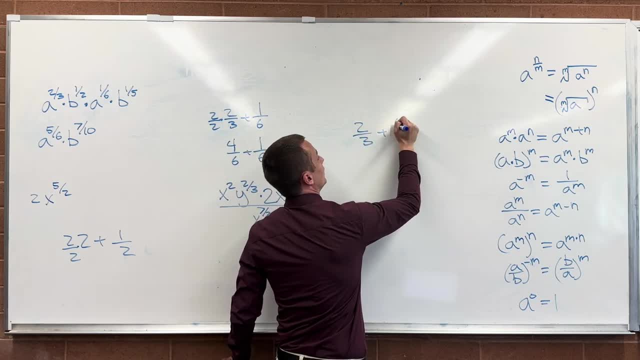 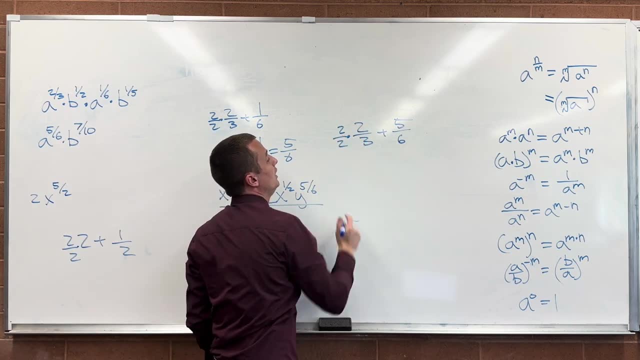 6- let's make sure we do that right- and plus 5, 6, what's my common denominator gonna be 6, so I need to multiply this one top and bottom, like to do, and so we got 4, 6 plus 5, 6 gives me 9, 6, 9. 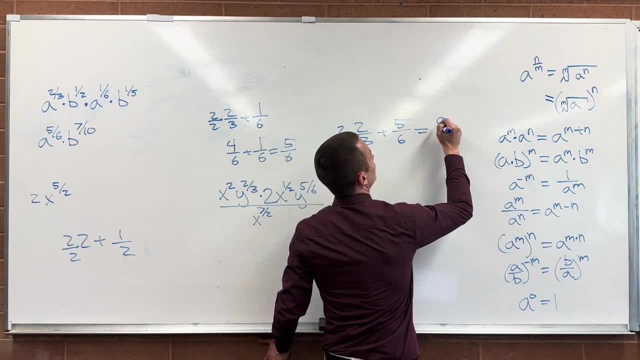 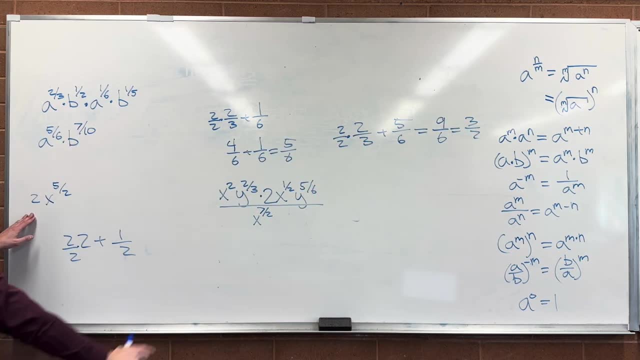 6 is the same thing as 3 halves. 3 halves Counts out of 3, top and bottom 3 halves. So this is what term? are we doing Our y's? So this is y to the 3 halves Now in my denominator. 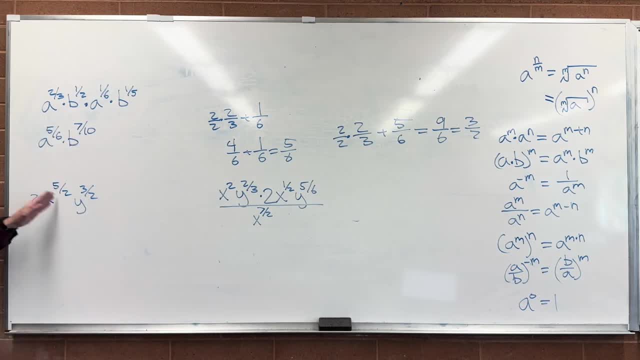 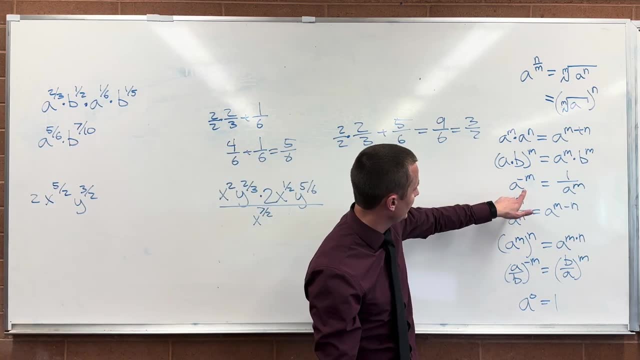 I have x to 7 halves, but I need to somehow combine it with this x, So I'm just going to bring it upstairs for a second to combine it. So I'm using this rule right here where if we flip it from top to bottom it just makes the x want negative. So I'm going to 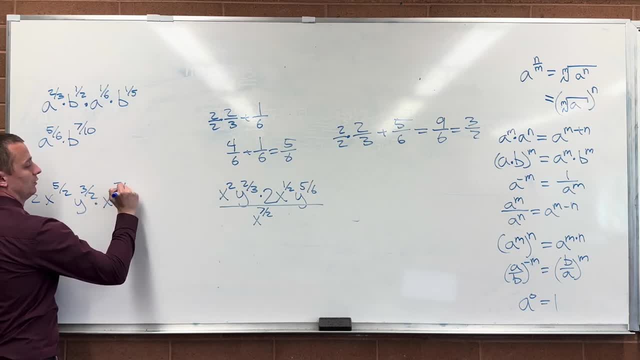 multiply it by x. now to the minus 7 halves. That was bringing this upstairs, just so I can combine it with this x. We'll put it back downstairs if we need to, and it's all set up. All right? what's 5 halves minus 7 halves: 1. 3. No, it's 2 halves, It's 1. Negative. 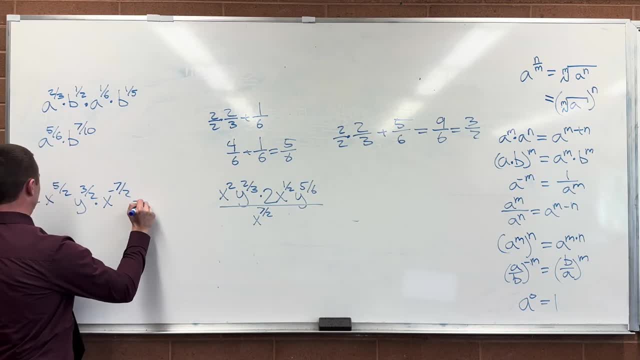 1. Negative 1. So this is now equal to 2x to the negative, 1. Y to the 3 halves. Now, finally, we're done combining like terms. Now we just don't want a negative exponent. So anything that was negative, put it down here. If you had. 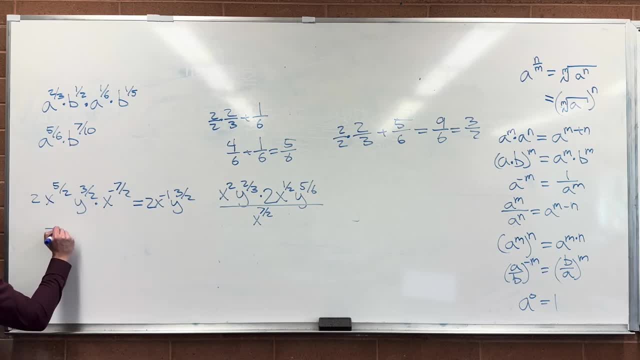 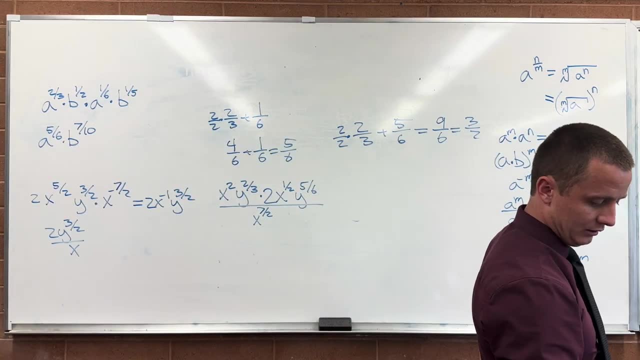 negative in the denominator, put it up here. So this is finally: 2y to the 3 halves all over x, and we're done. Make sense. 2y to the 3 halves, Okay, And one more monstrosity. 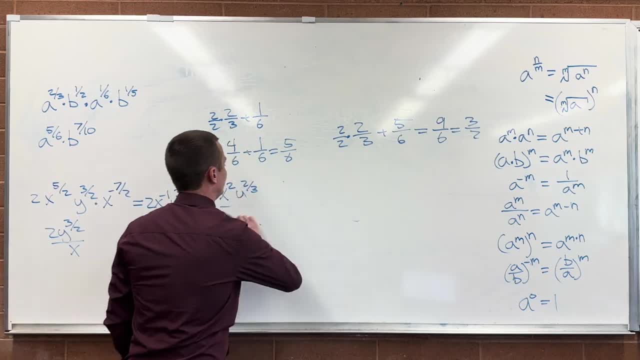 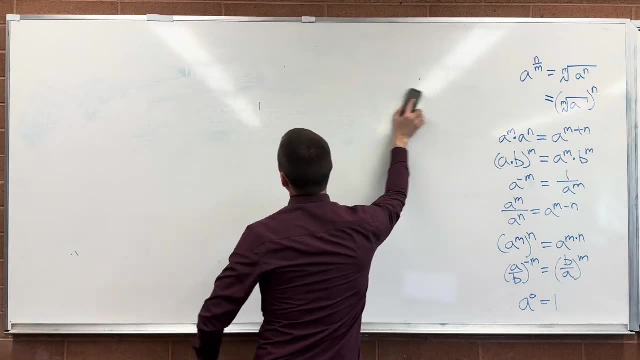 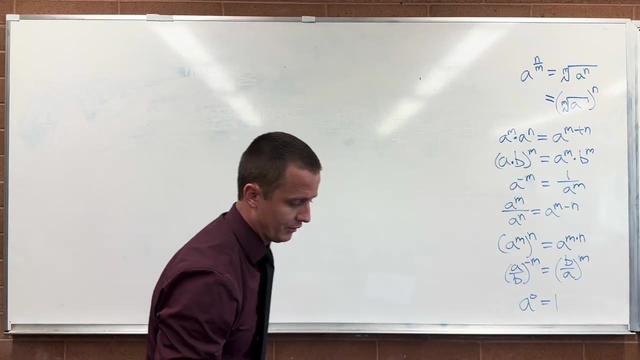 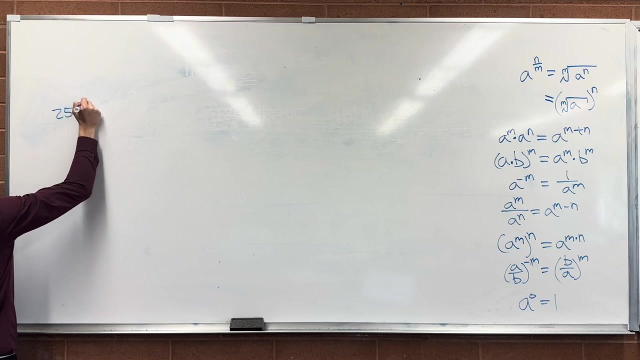 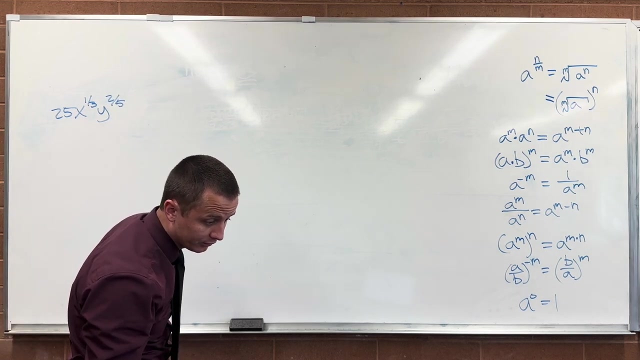 and then we'll move on to the next section, And this is another multiplying one, So should be good for you. Probably need a lot of space for this. All right, This one, 25x to the 1 third, y to the 2 fifths. So 25x to the 1 third, y to the 2 fifths, all. 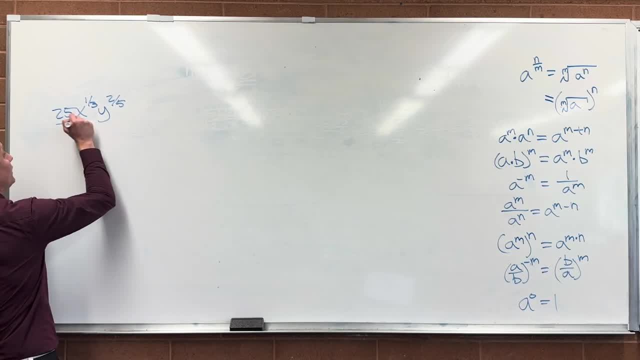 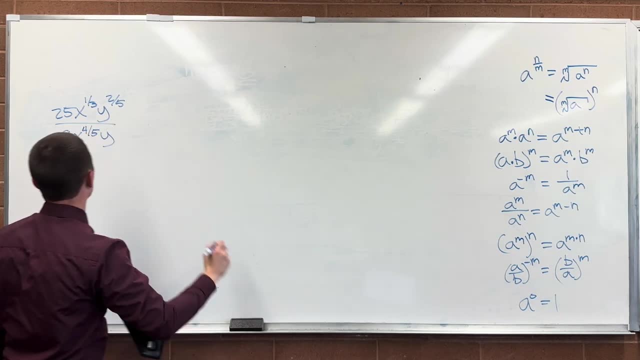 over 9.. 9x to the 4 fifths, 9x to the 4 fifths, y to the negative 3 halves, y to the negative 3 halves. And now we're taking this whole thing and we're rating it to the power of. 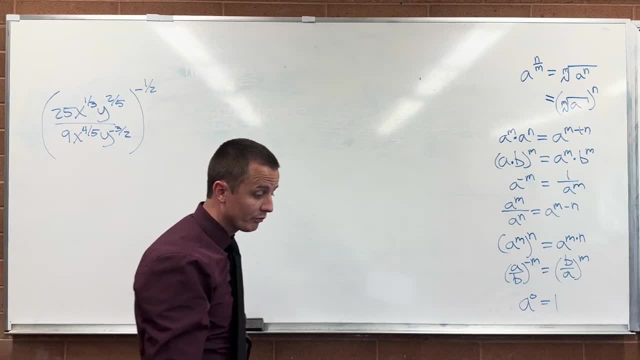 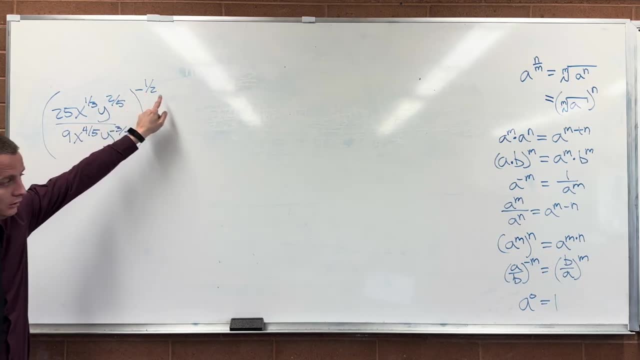 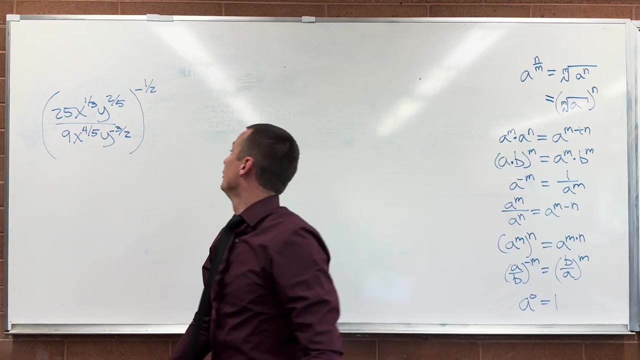 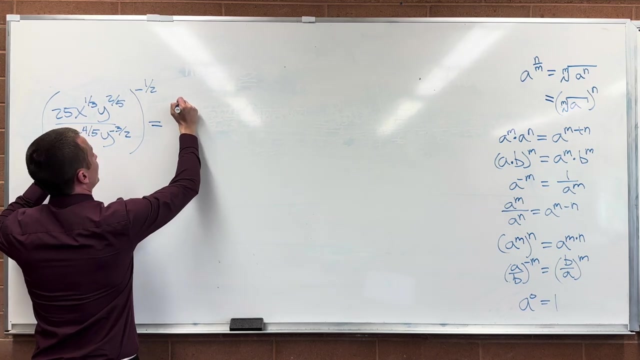 minus 1 half, So you can start with the inside first or, if you want to get rid of that minus 1 half, right out the door. we can use this rule: a over b to the negative m And the spacing is b over a to the m. Perfect, So we can start out by writing this as 9x to: 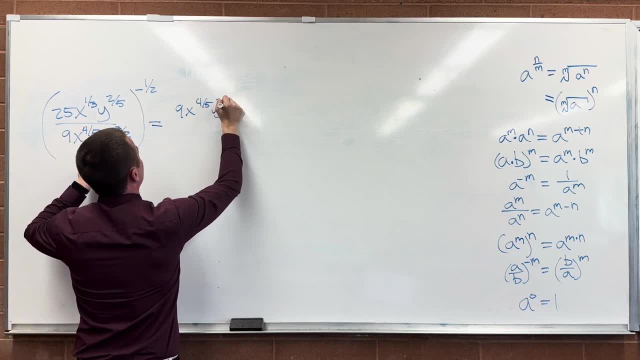 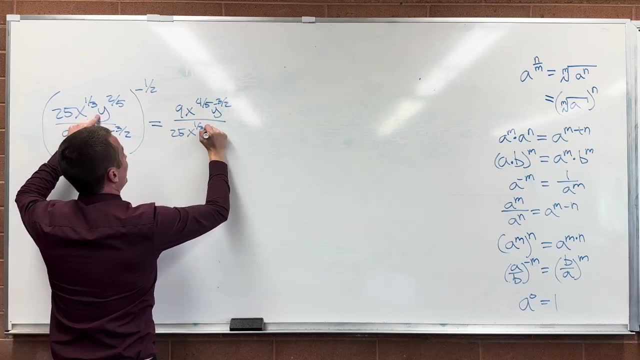 the 4 fifths, y to the 3 halves minus 3 halves, all over 25x to the 1 third, y to the 2 fifths, all raised to the 1 half. Okay, Now we're going to do this again. So we're taking this whole thing and we're going to 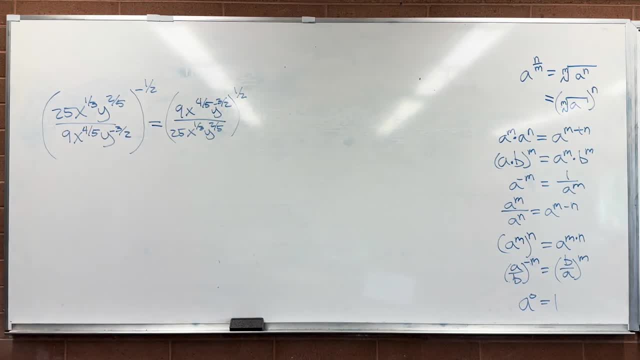 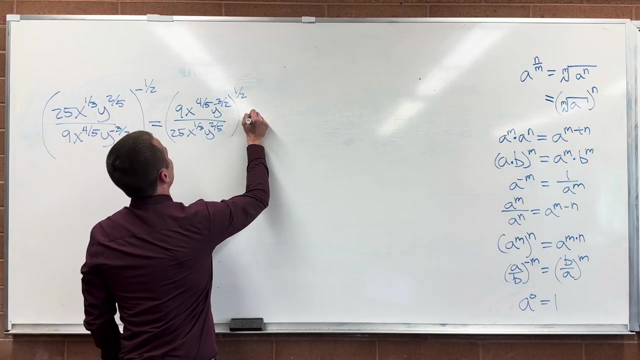 Now let's multiply in our exponent Or we can cancel out like terms first if we wanted. I'm going to multiply in the exponent first because it looks like he gave us numbers easy to take the square root of. Okay. so this is going to be equal to multiplying everything to the 1 half. 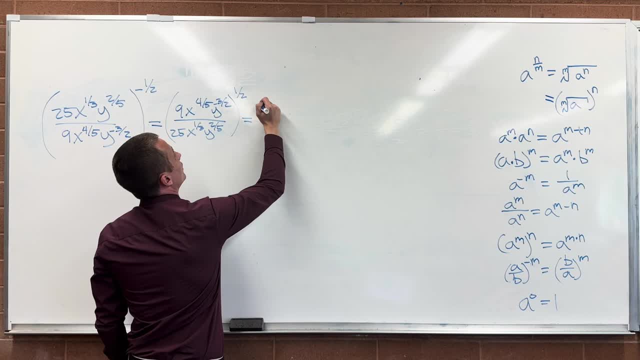 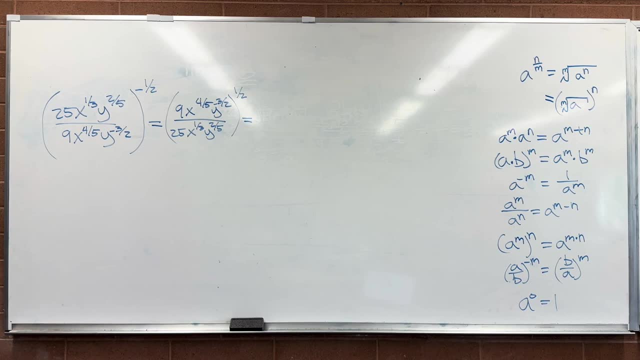 So 9 to the 1 half is 9 to the 1 half is Same thing as square root of 9.. 9 to the 1 half: square root of 9. 9 to the 1 half is 3.. 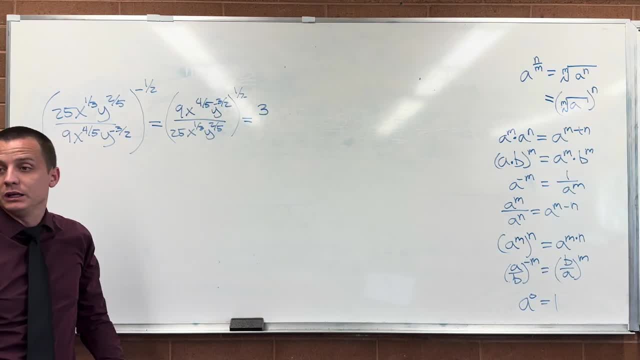 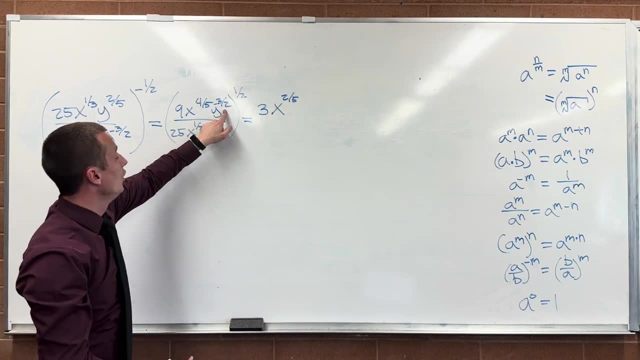 X to the 4 fifths times 1 half is going to be 4 tenths or 2 fifths, So that's X to the 2 fifths, Negative 3 halves times 1 half. X to the 2 fifths times 1 half is: 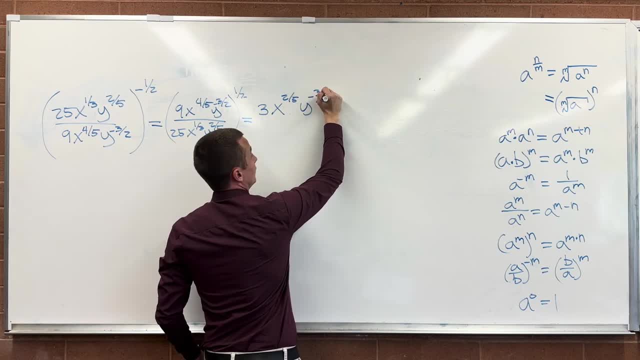 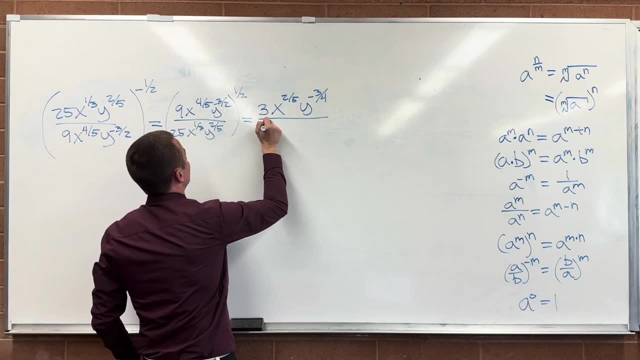 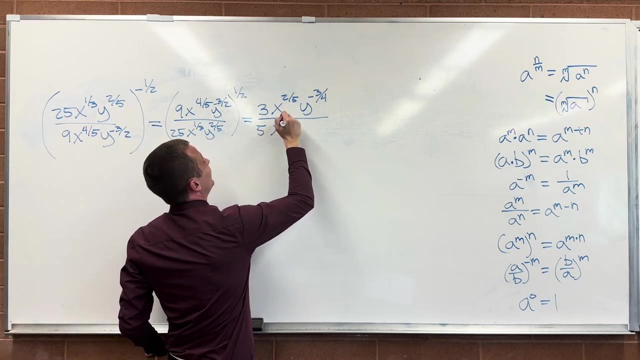 Negative: 3 fourths. All over in the denominator, we get 5. 20.. Good, 1 third times 1 half Is 1 sixth. 2 sixths: 1 sixth, 1 sixth. A third times a half is a sixth. 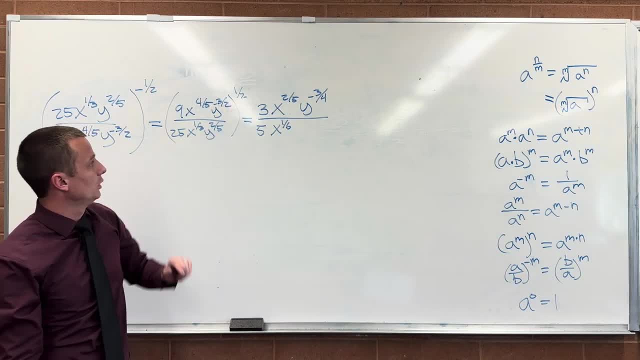 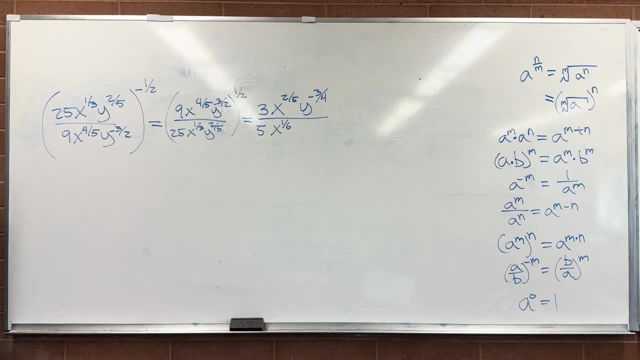 Multiply the numeric to the numeric denominator to the denominator: 2 fifths times 1 half is 3 tenths 10.. Multiply It's 10.. 2 tenths, 2 tenths or 1 fifth. 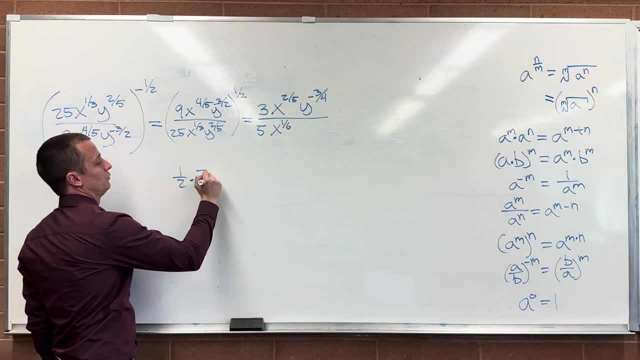 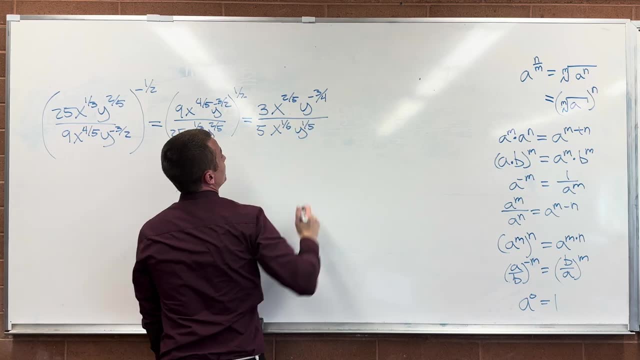 1 fifth. You had 1 half times 2 fifths, 1 fifth, Alright, so Y to the 1 fifth. Okay, Now I'm going to put all my X's upstairs and all my Y's downstairs, because I think that's going to help things. cancel out. 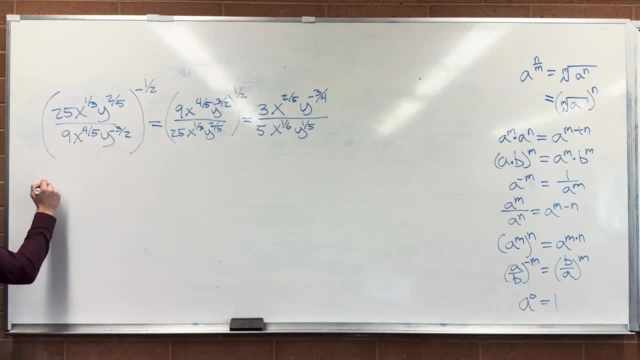 So that is going to give me, in the top, we're going to have 3X to the 2 fifths, And then, since I moved this upstairs, that's going to be X to the minus 1 sixth, And then, in the bottom, we're going to have 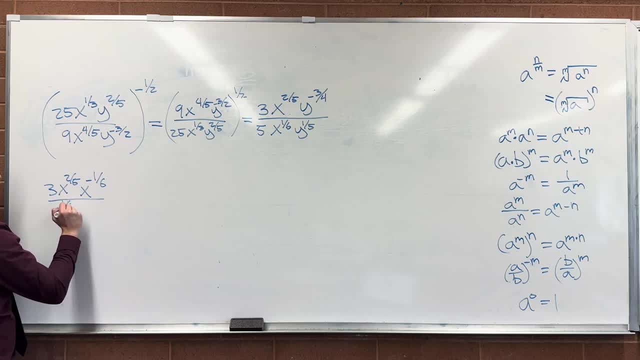 Y to the 1. fifth times. Y to the what. 3 fourths: Positive 3 fourths, Good, And now I just need to add these together, That's 3 fourths. You need your 5.. Oh, thank you, I lost my 5.. 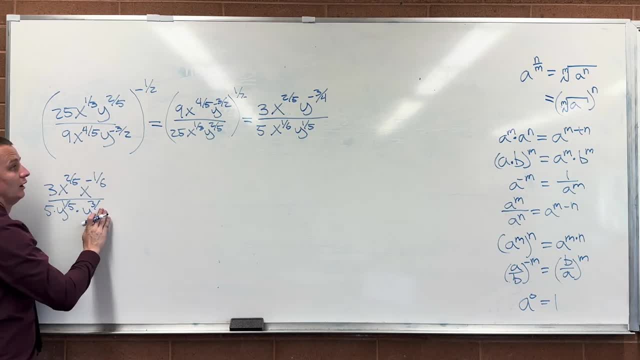 Okay, 3 fourths. Thank you, I looked at that Y already down there. 3 fourths- Yeah, don't let me lose track of any numbers. Don't want to have to rework this problem. Okay, So now upstairs. we need to do 2 fifths minus a 6.. 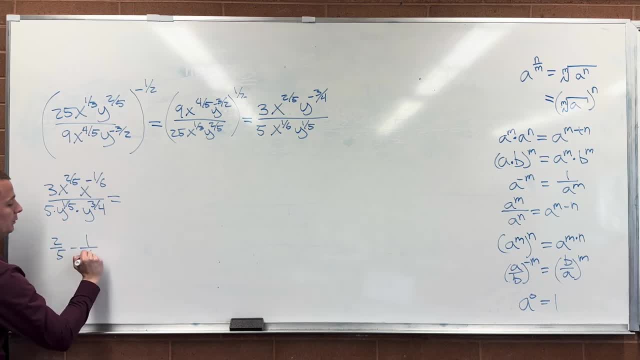 So we're doing 2 fifths minus a 6. What's my common divisor going to be 30. 30. So I need to multiply this one top and bottom by 6, and this one top and bottom by 5.. 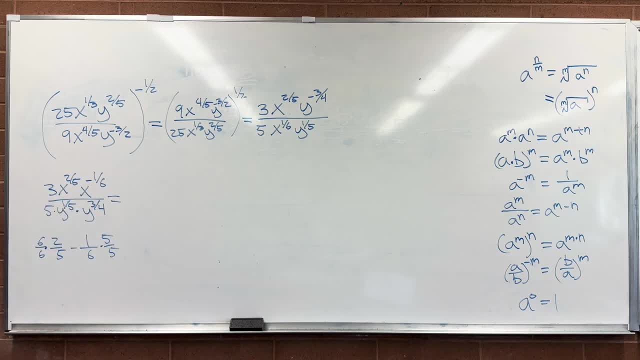 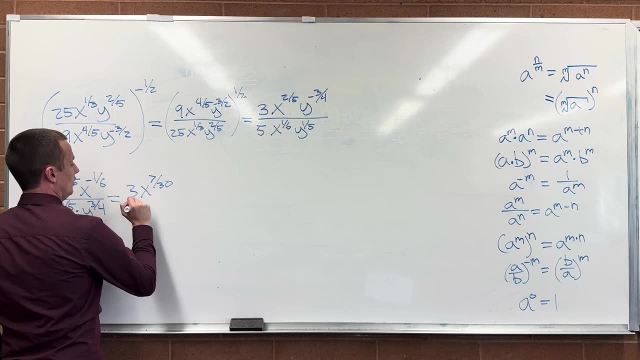 So I've got 12 minus 5 is 1 third. Oh wait, It's 7.. 7 thirtieths. So 3x to the 7 thirtieths, All over, 5y to the. 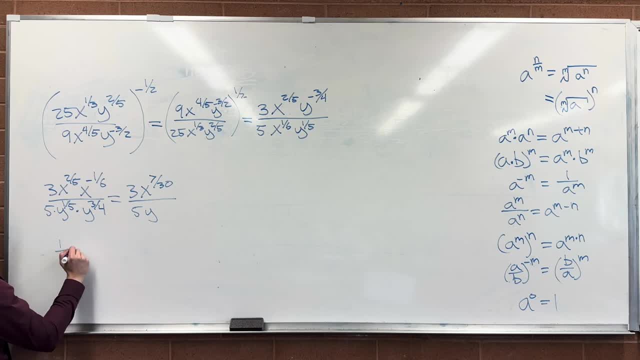 We have 1 fifth plus 3 fourths. What's my common divisor going to be 20. 20. So this one needs to be multiplied top and bottom by 5.. This one needs it by 4.. So we've got 4 plus 15 is. 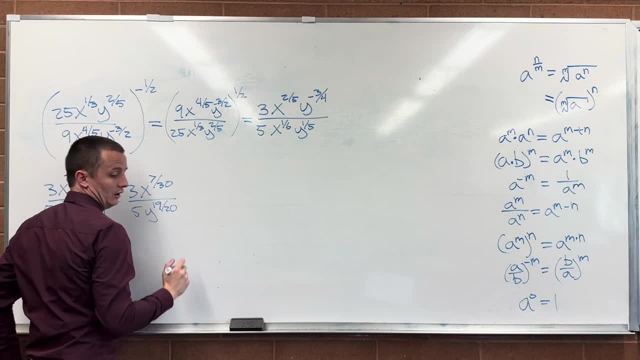 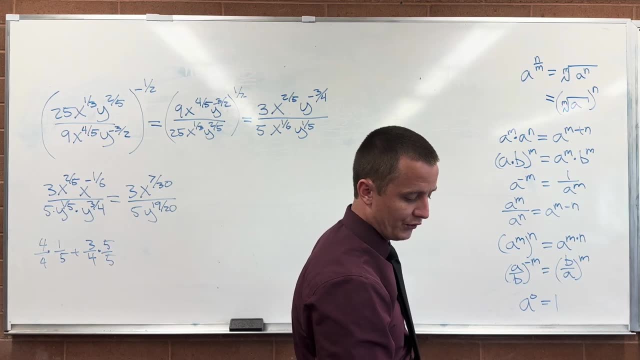 We're going to 19 over 20.. 19 thirtieths, All right, Let's see if we. Let's see if we Got even close to him. 3x to the 7 thirtieths. 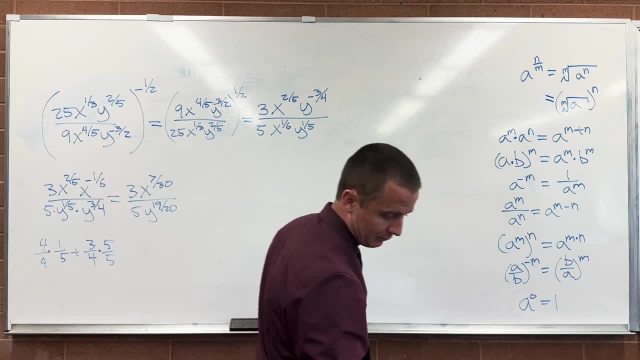 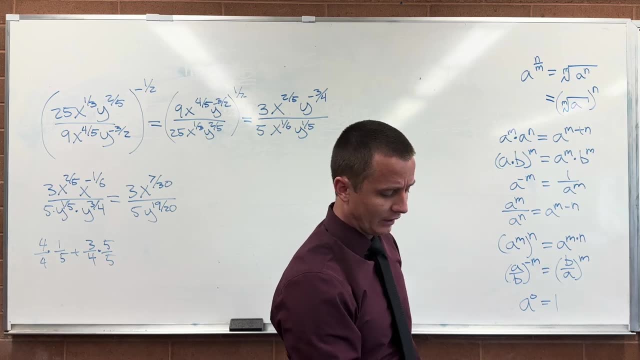 All over 5y to the 19 twentieths. All right, We nailed it Okay. Next section. The next section: same types of problems. He's just now going to give you radicals and exponents all together in one jumbled mess. 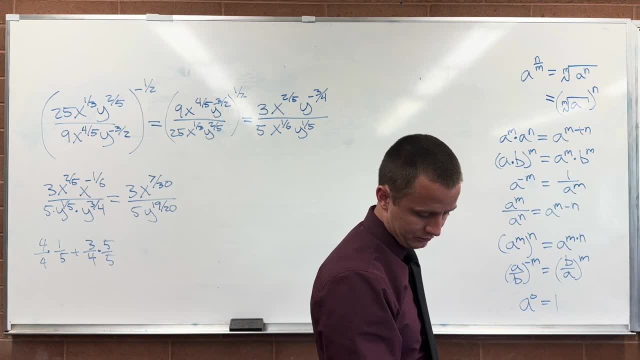 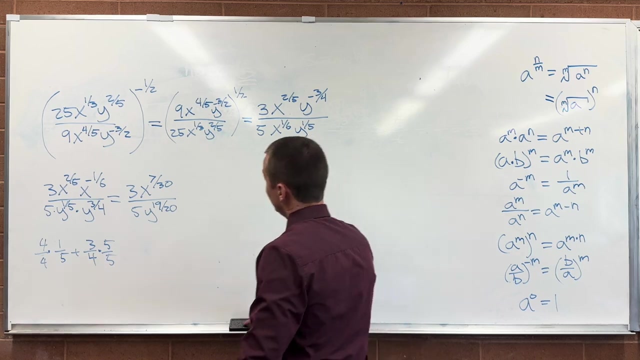 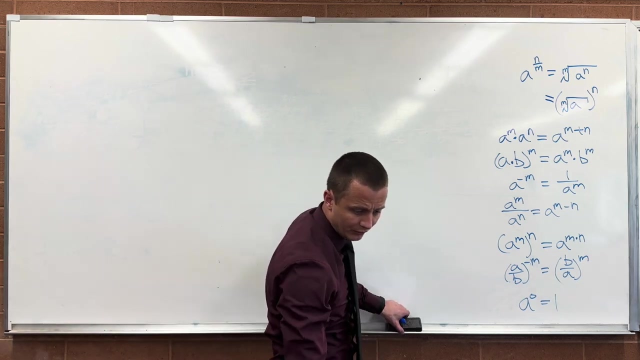 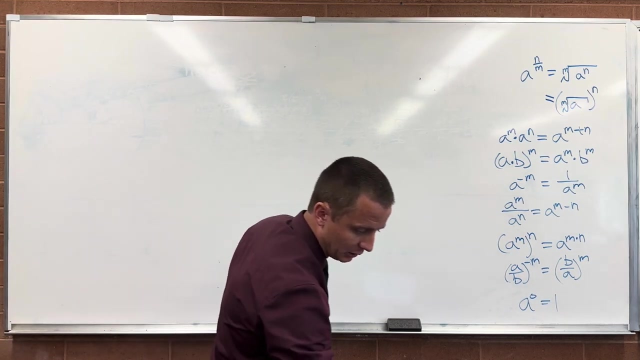 Rather than giving you all exponents or all radicals. So let's work through an example. So rewrite as rational exponent. Oh, that's not what the actual problem is going to be. The problem is going to be something like simplify. 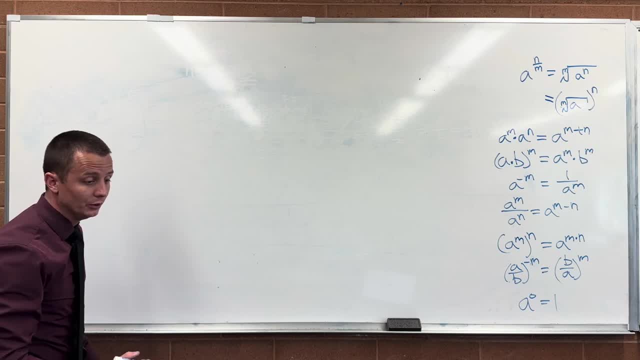 So he's going to give us a problem By calculating the 8th root. So we're going to calculate the 8th root of x to the 6,, y to the 2.. So we're going to start by giving us something like that: 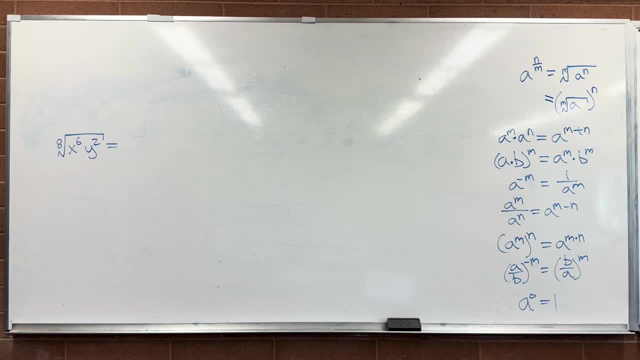 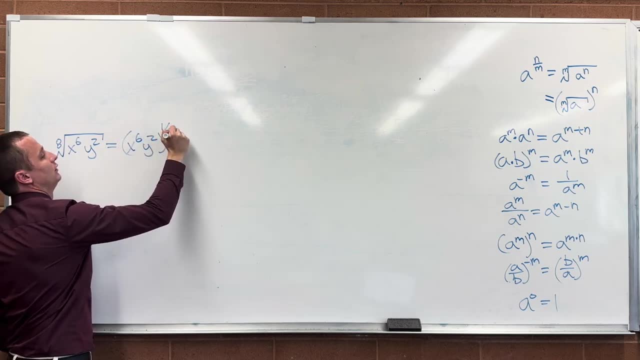 Now, first thing we're going to do is think about this in terms of exponents. So this is x to the 6, y to the 2, all to the 1 eighth Same thing. Taking the 8th root is the same thing as raising it to the 1 eighth power. 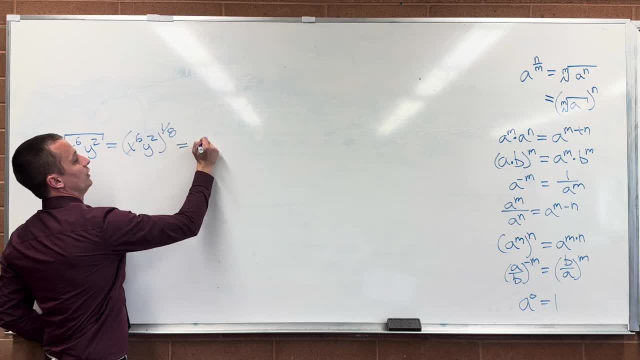 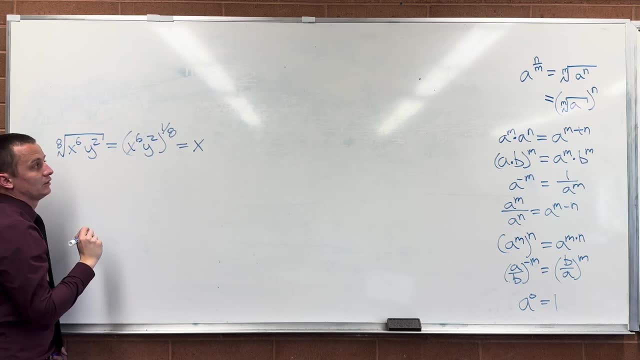 Okay, Now multiply 3 to our exponents, So this is x to the 6 eighths. You're just doing 6 times 1 eighth, 6 eighths. What is 6 eighths? Alright, we'll just write it for a second and then you'll see. 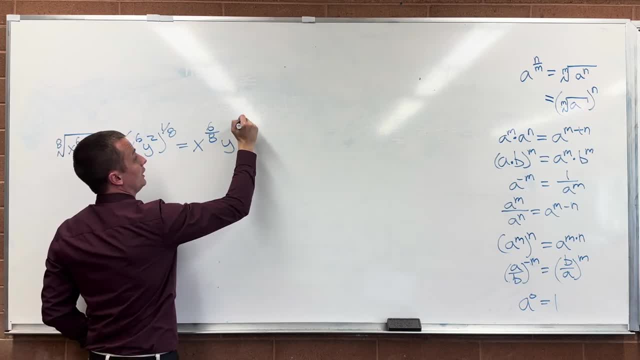 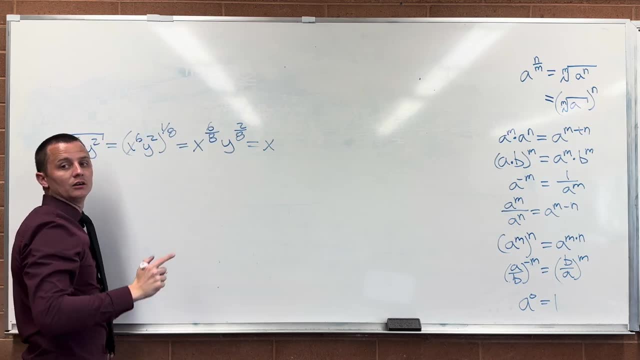 And y to the what? 2 eighths, 2 eighths. good, Now, 6 eighths is the same thing as 3 fourths, And 2 eighths is the same thing as 1 fourth. 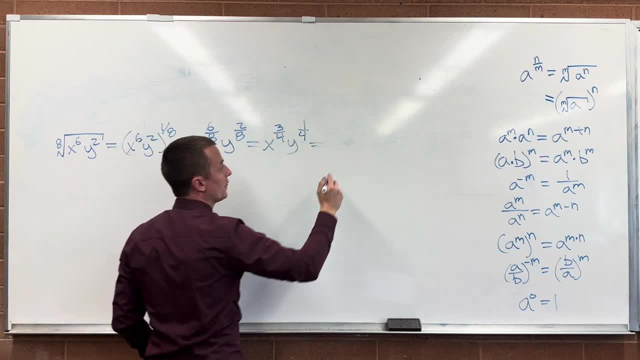 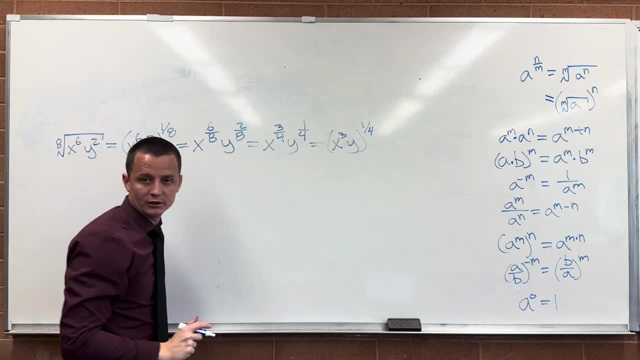 1 fourth. Now I'm going to pull the 1 fourth back out, So this is going to be x cubed y all to the 1 fourth. Wait, how did you get your x cubed? Because you took the 1 fourth out. 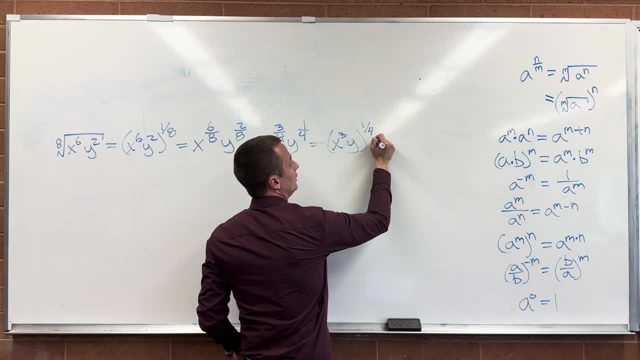 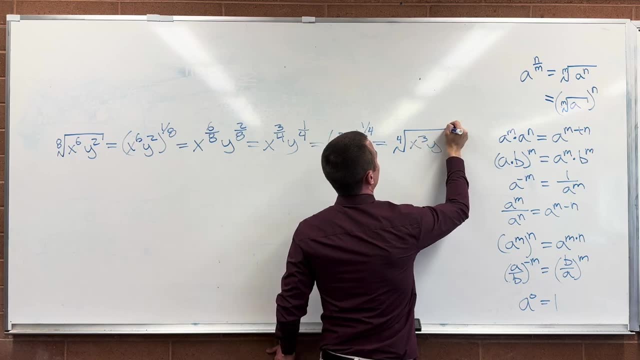 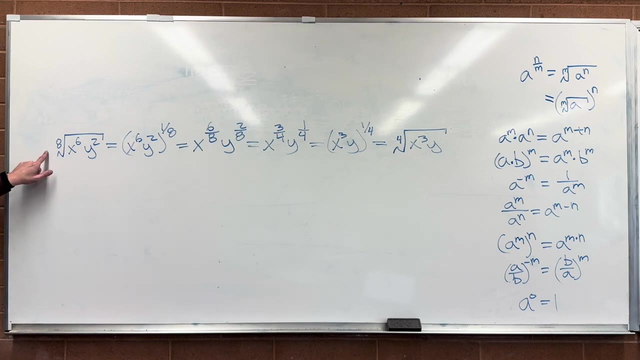 I took the 1 fourth out of both And then finally, this is the 4th root of x cubed y. So we just simplified. the 8th root of x squared, y squared is the same thing as the 4th root of x cubed y. 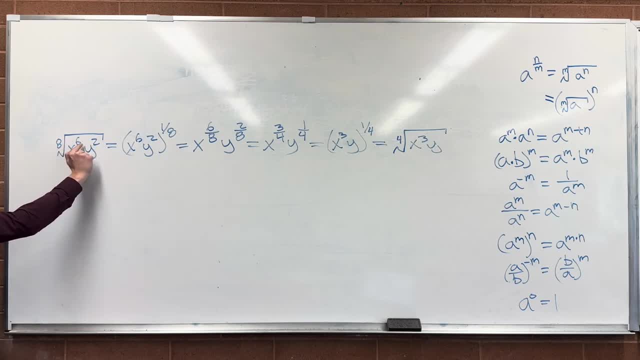 And you'll notice. what we did is we canceled out 2 top and bottom. We divided our numerator and our denominator each by 2 of our exponential fractions. Make sense? Yeah, So we don't want to have to write out this algebra every single time. 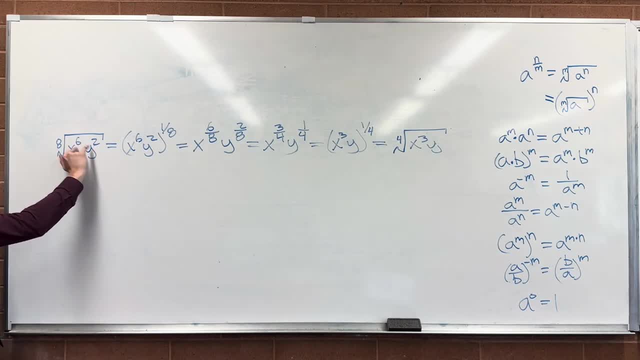 I want to be able to say to you: So notice that we can divide our numerator and our denominator of our exponents each by 2. And just go straight from this step to this step without having to show all the algebra in between. 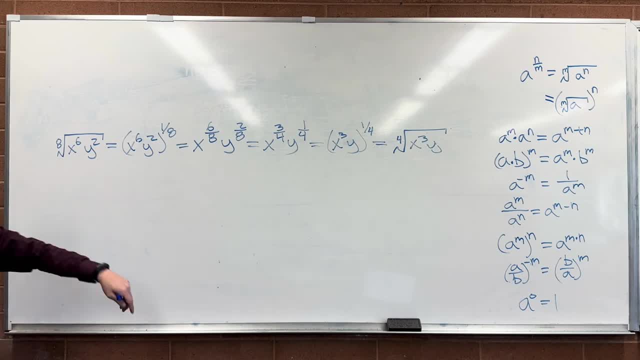 Because that's real tedious. I want you to just be able to see that Make sense, Yeah, So let's try another one, And this time we're not going to write out all the algebra, We're just going to see if we can see it. 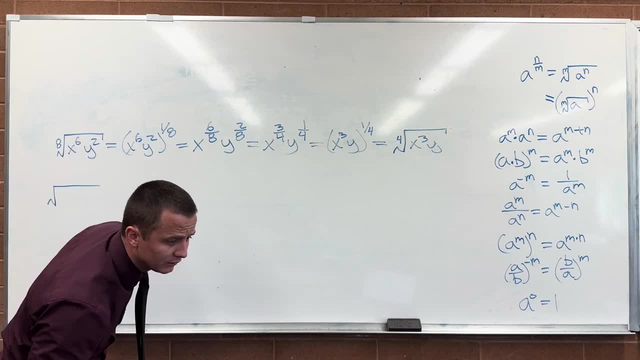 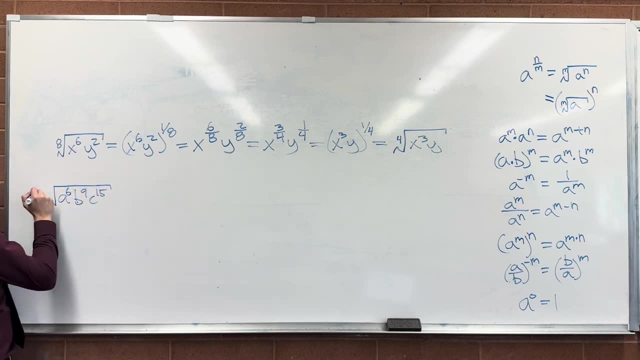 So I have a to the 6, b to the 9, c to the 15.. a to the 6, b to the 9, c to the 15.. And we're taking the 24th root of that. 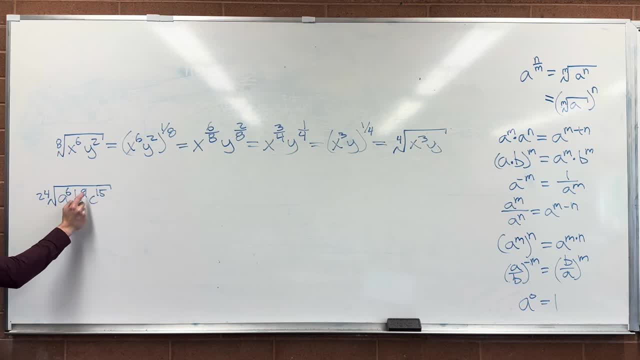 3. 3.. So you notice 3 goes into that, that, that and that. So I'm going to cancel out 3 top and bottom for my exponents, And so this is going to be the same thing as the 8th root. 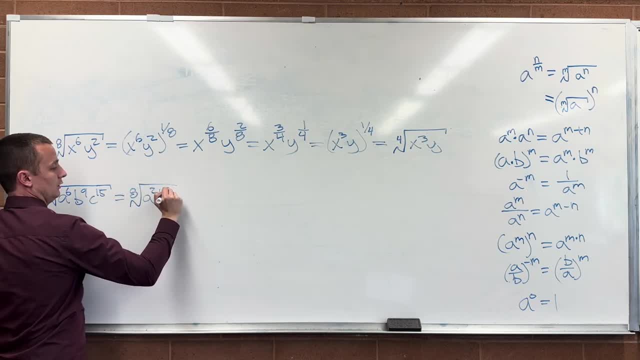 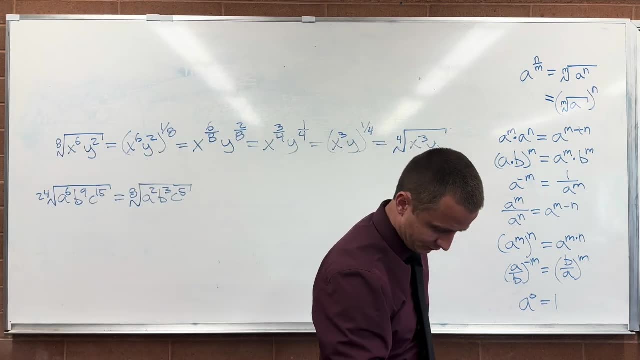 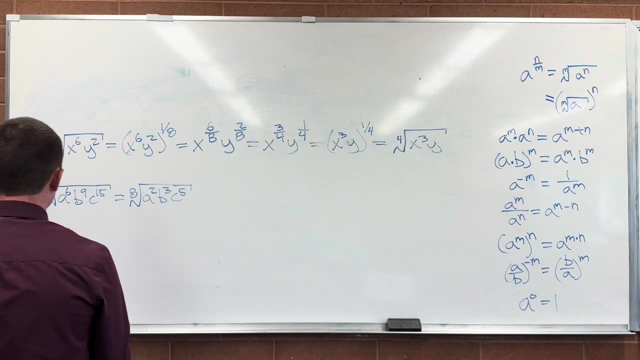 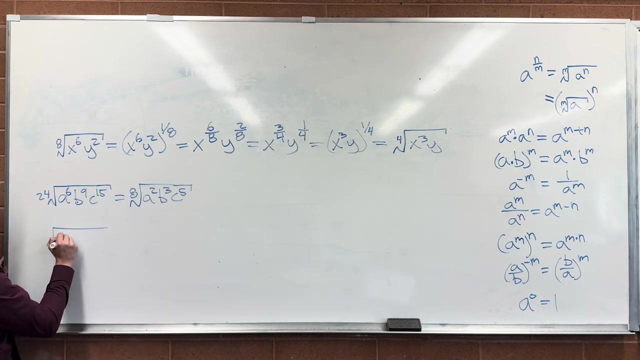 With a squared, b cubed and c to the 15. And that is exactly right. Cool right, How easy that was. Alright, let's try another one, One that has some numbers that might confuse you. So we are going to look at 8m to the 6, n cubed. 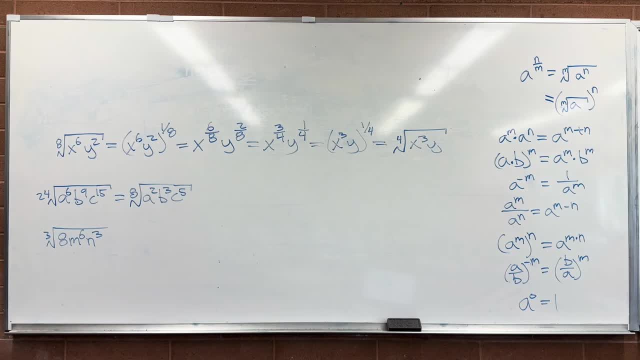 And we're taking its cubed root 3.. You see 3, except for that 8.. That pesky 8.. Is that 2?? No, it's 1.. But you have the right idea: 8 is the same thing as 2 cubed. 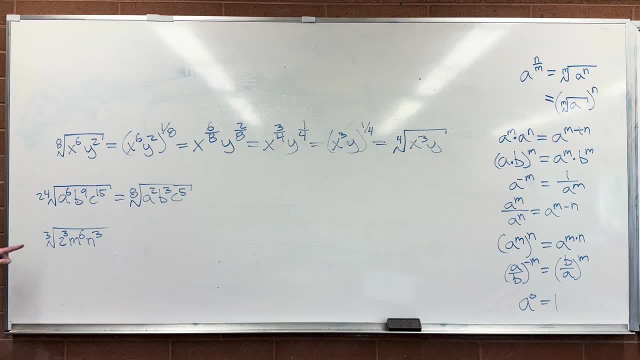 Oh, And so it is a cube. And so you see, each of our numerators can be divided by our denominator, And so this is the exact same thing as what? 3.. Isn't it 3, or just 1?? 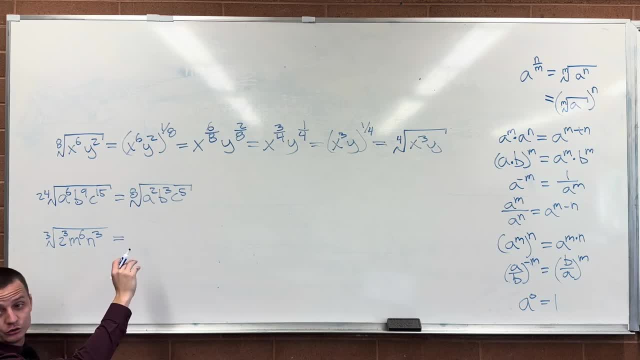 Because you're taking it out. You tell me What do I write? 3. Square root: 3. I'm not sure Up. So let's follow our rule. Let's follow our rule. We're taking the 3 out, top and bottom. 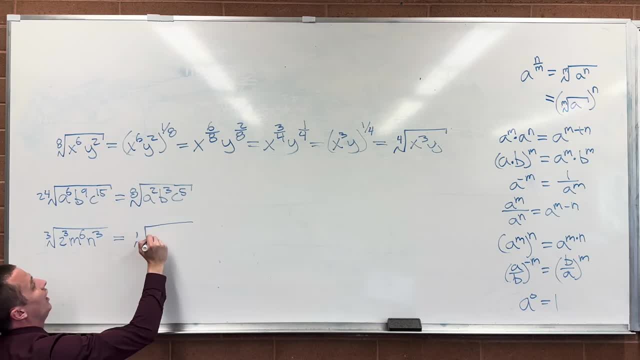 So we should be taking the first root of 2m squared n. Right, But we're taking the first root of it. What's the first root of a number? It's just the number. The square root is just a root. 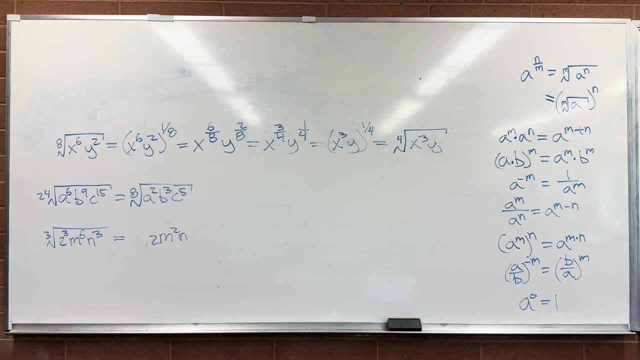 We don't even have a square root, We have a first root. So that's just the number itself. But notice that you could have almost guessed this one. Look, Take the cube root of 2. cubed That gets you 2.. 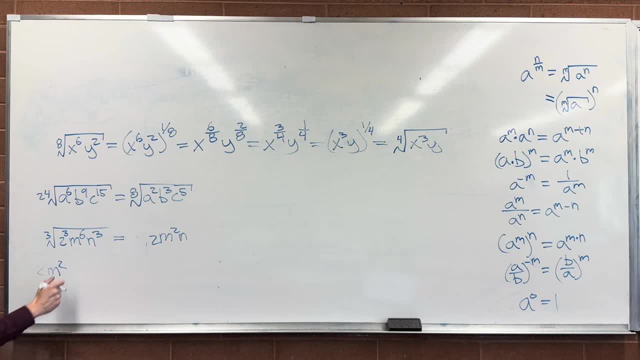 Cube root of n to the 6th. That gets you m squared. Cube root of n: cubed. That gets you n Using it the way you already knew how, So you can think about it as the first root of all those things. 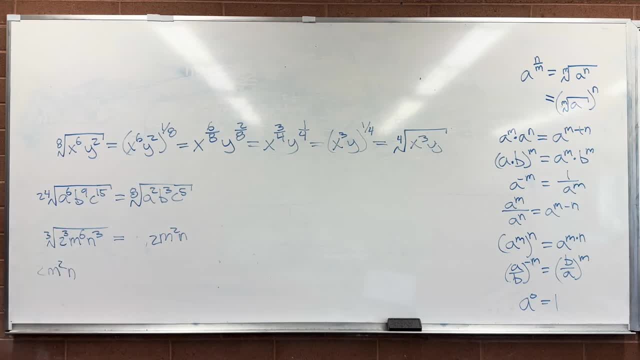 Or you could have done it the way that we did in previous problems: Same answer. So yeah, If you get it, If you get this, a 1 here, That same thing is just a number. Get rid of your racco all together. 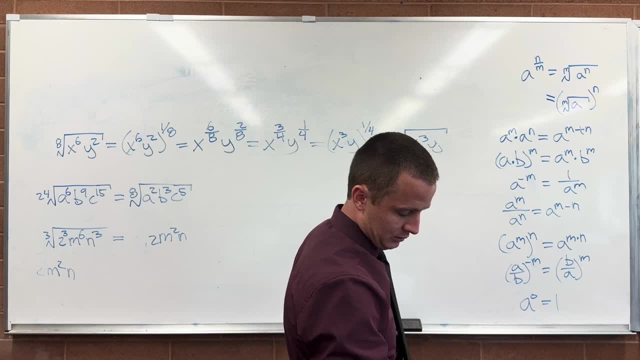 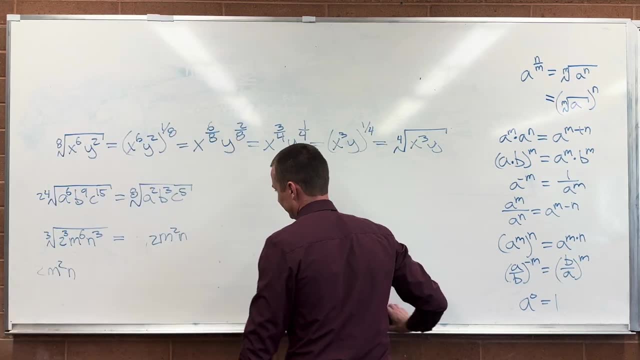 So that was a good problem. Oh, And part of it is I wrote the problem. That's not the problem the author gave us. That's not what we're doing. That's not the problem. The author gave us this problem. 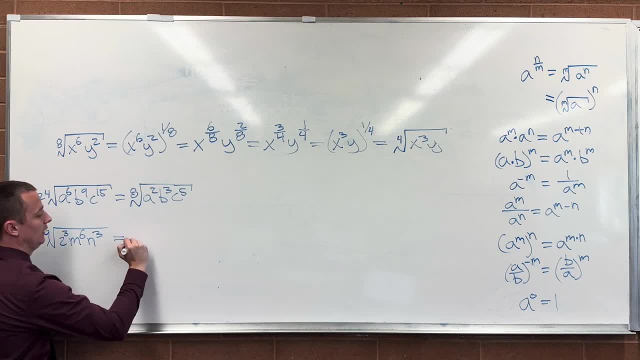 The 9th root And now divide the top of all by 3.. In this case, it's just the third root of 2 m squared n. Okay, So that's what he gave us, But if it came out like that, eh, good to cover anyways, just in case. 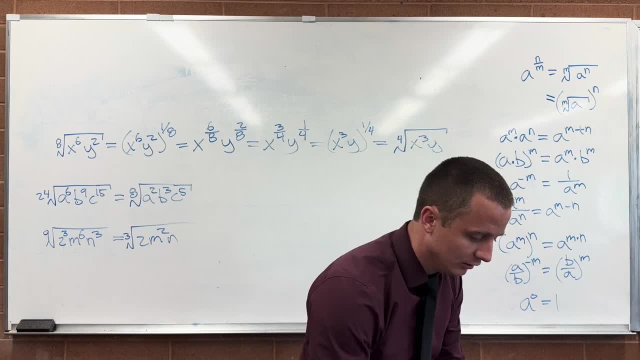 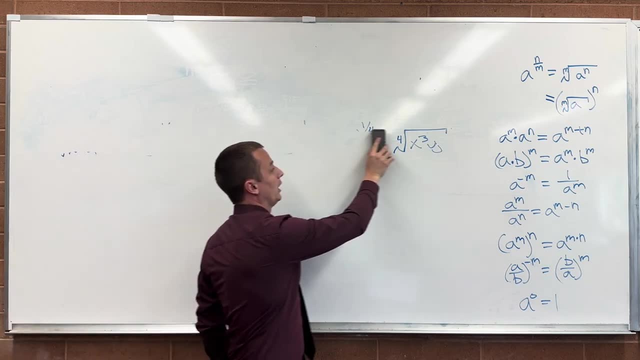 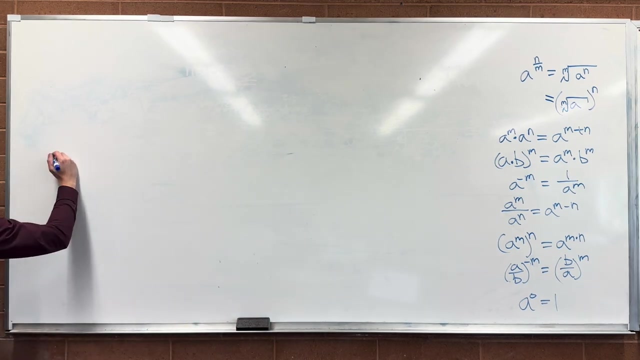 I was a little surprised that he gave you one that did that. That was a bit tricky. Okay, Slightly more convoluted one, One where we got to multiply some terms together and then simplify. So this one we have the fourth root of. 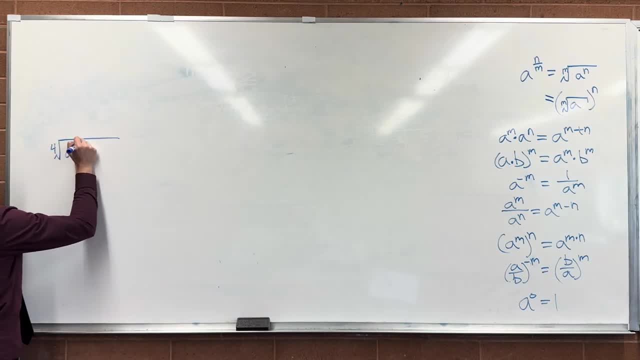 a squared, b cubed. a squared b, b cubed. And the radical All multiplied by the sixth root of a squared b. Okay, Make sure I got that right. Okay, So we have a squared. 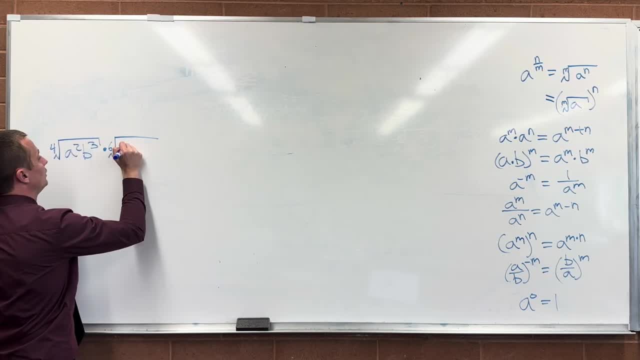 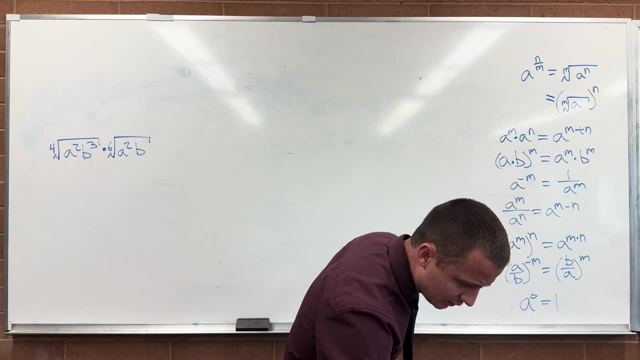 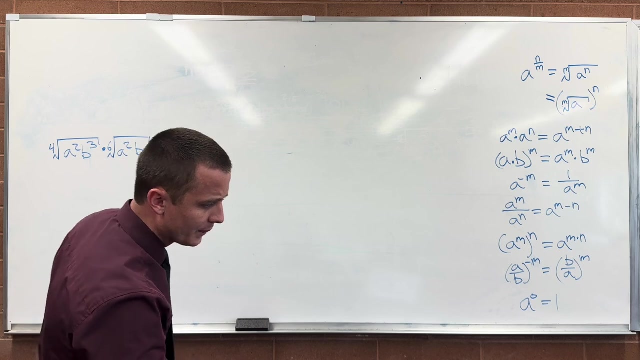 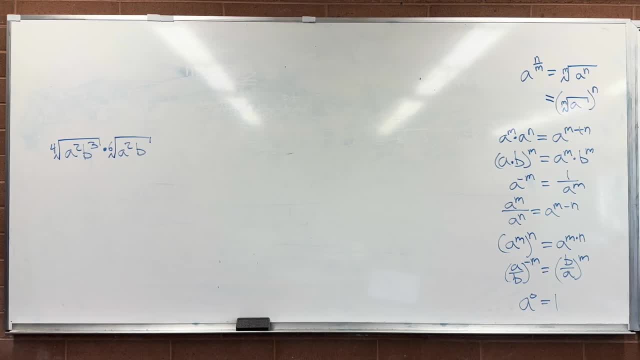 All right, How are we going to combine these together? We cannot just take this one fourth, this fourth power, and multiply it by the sixth power. We only know how to multiply when these are the same number. Okay, so then, make your square root the same, by making it a 2,, a 3, and a 2.. 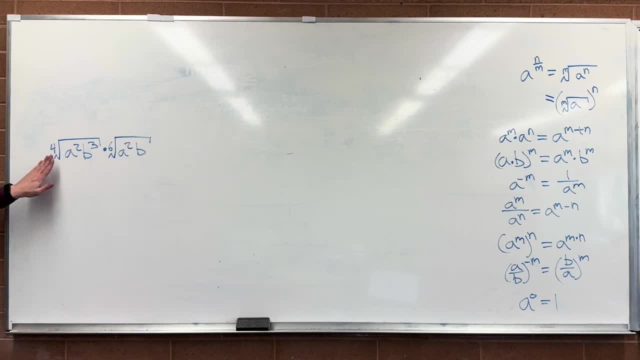 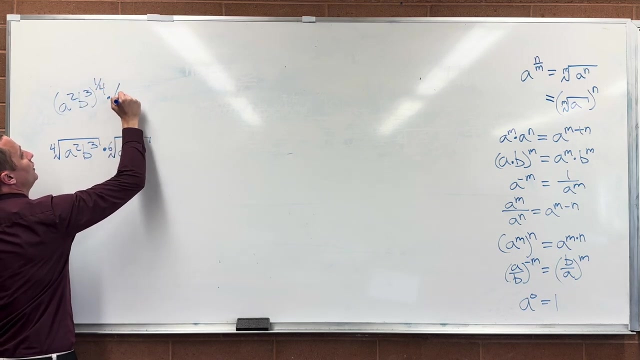 I don't know You might be onto something, So let me rewrite this and then this might help you. So I have a squared b cubed to the 1- 4th and I've got it multiplied by a squared b to the 1- 6th. 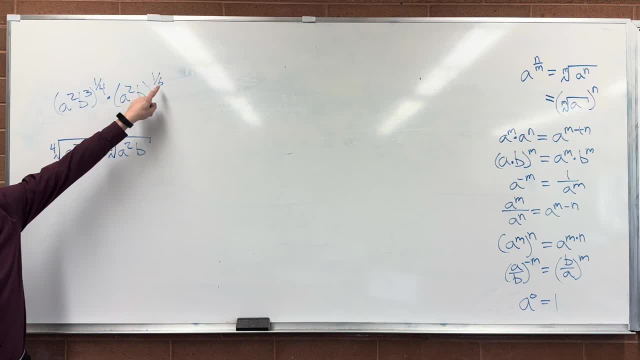 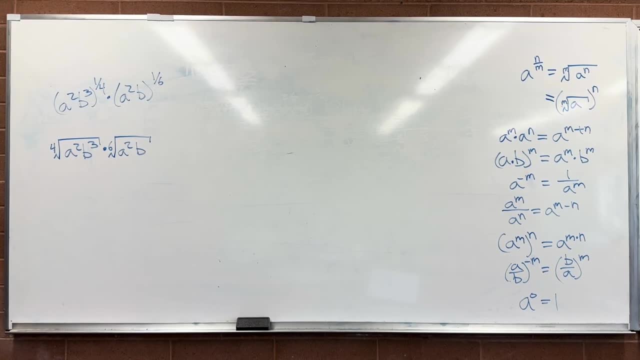 So I basically need to get a common denominator between 4 and 6.. How do I do that? What can I multiply? First off, what's my common denominator between 4 and 6? Common denominator If I asked you to add 1 4th and 1 6th. 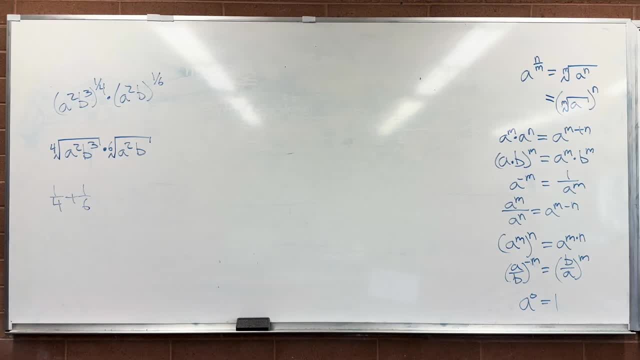 what would you have to use as your common denominator? You could use 24,, but 12 works Okay. Okay, so 12.. So what do I need to multiply this by to get the 12? 3. 3. 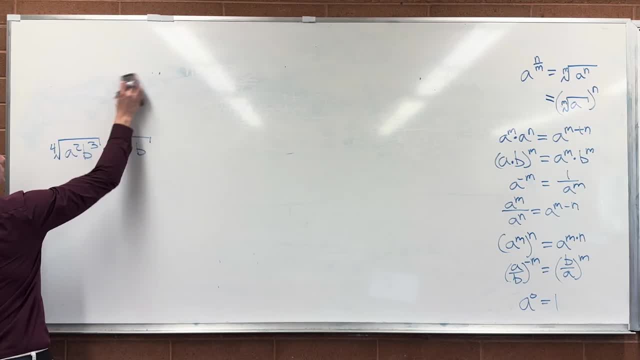 So I'm going to multiply this by. let me rewrite this with some space, Sorry, I wasn't thinking ahead. So this is a squared b cubed all to the 1- 4th. I'm going to multiply it by 3 over 3.. 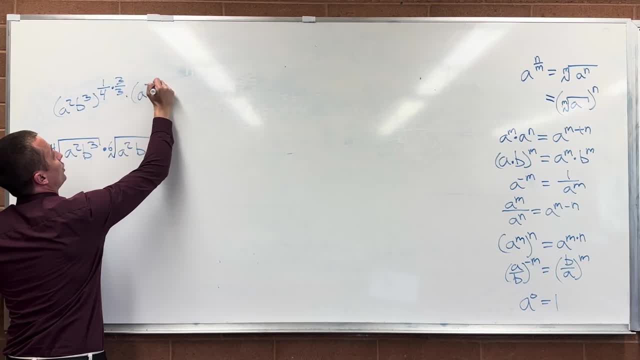 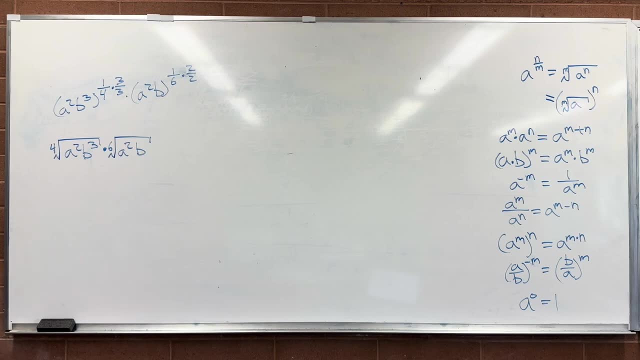 Similarly, this is going to be times a squared b to the 1, 6th and then multiply it by 2.. 2 over 2.. You with me? Now I'm going to take that cube and bring it in here. 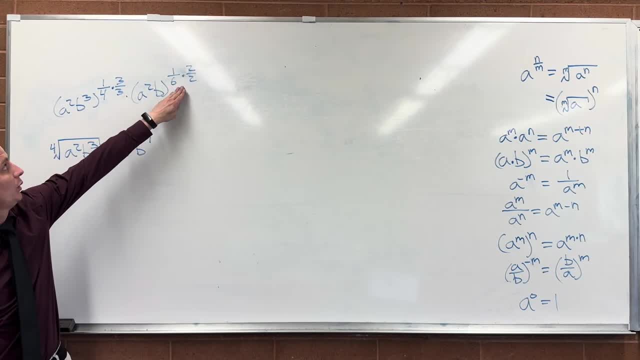 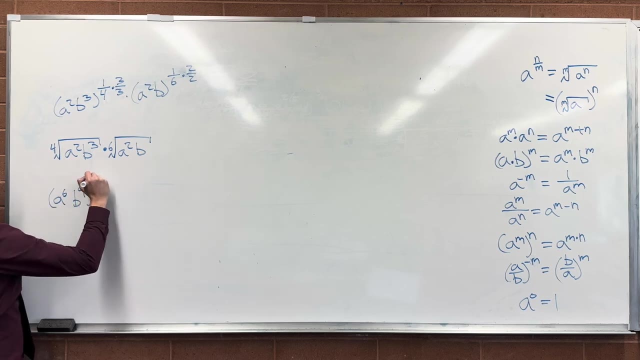 And I'm going to take that square and bring it in here and leave the 1 12th out here and the 1 12th out here. You see that. So rewriting this term, bringing the cube in, that is going to be a to the 6, b to the 9 to the 1 12th. 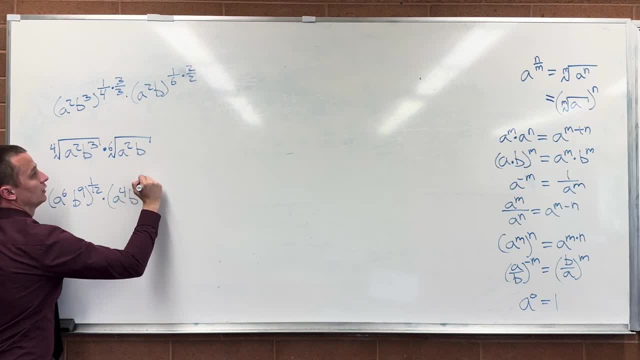 times a to the 4th, b squared all to the 1, 12th, And now I have the 12th root of this and the 12th root of this. So now I have the 12th root of a to the 6 times b to the 9,. 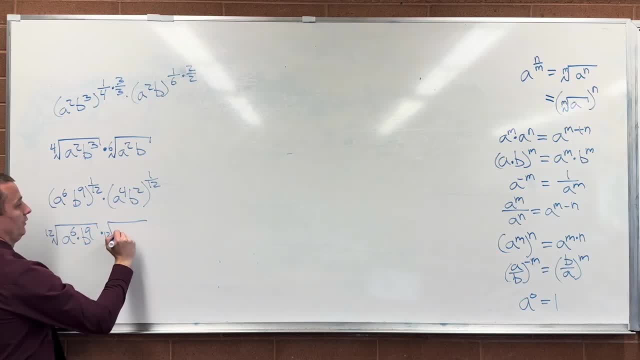 times the 12th root of a to the 4 b squared. So notice what I did Now, just going from here to here, because we don't want to have to go to that algebra again. I multiply top and bottom of this by 3,. 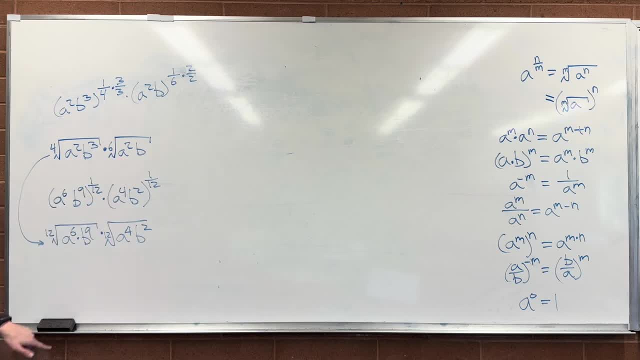 and I multiply top and bottom of this by 2.. That's how you can think about it. Remember that's a, b to the 1.. So take all the exponents inside, multiply by 2,. take the denominator 1,, multiply it by 2,. 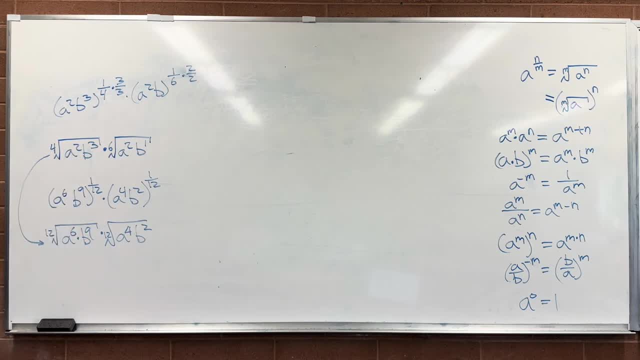 take the numerator 1, multiply it by 3, take the denominator 1, multiply it by 3.. That's all the algebra we just did. You're just trying to get you comfortable about thinking about these numbers as somehow the denominator for our exponents. 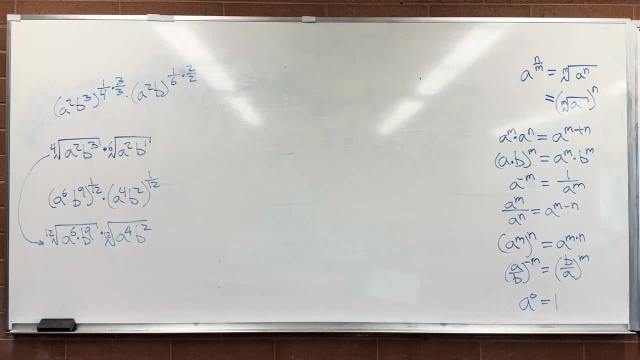 and these ones as our numerators, for our exponents, So that we don't have to go through all this middle algebra over and over again. And now that we have common roots, we can just multiply them the way we know them up. 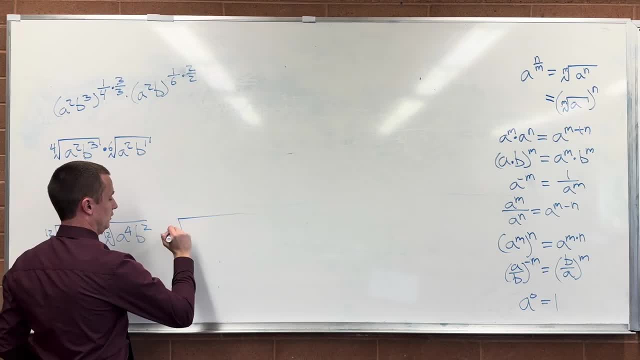 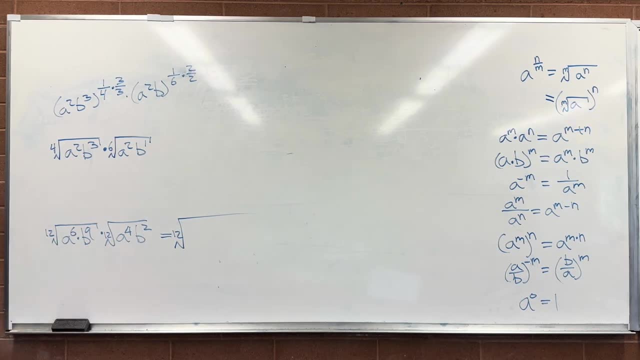 So this is just going to be the 12th root of When you multiply terms, you add exponents. You're going to be so tempted to get that mixed up left and right. It's going to be very confusing. a to the 10.. 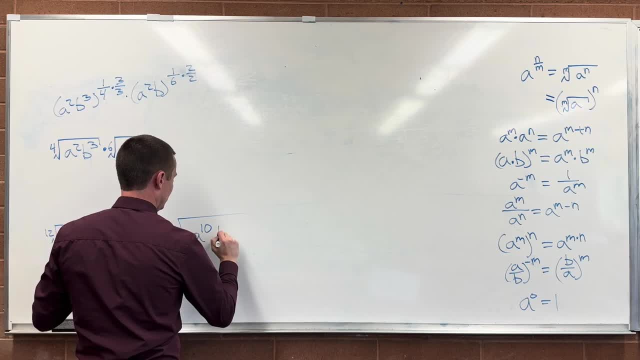 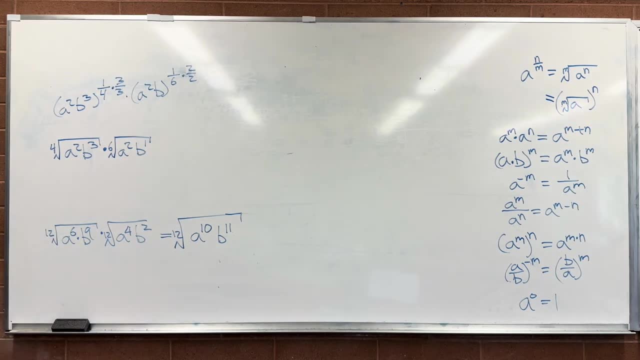 a to the 10., b to the 11. And b to the 11. 11.. And now notice that my numerator and my denominator have nothing that can cancel out. So I'm pretty sure that's going to be his answer. 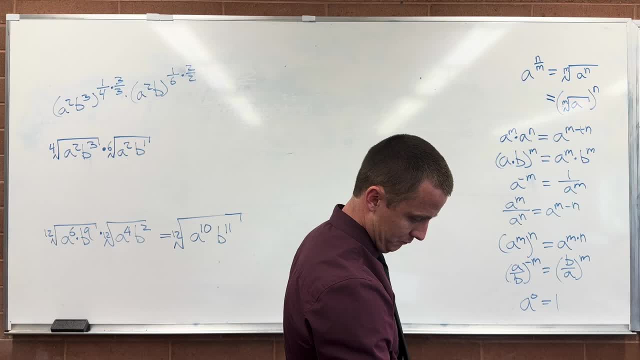 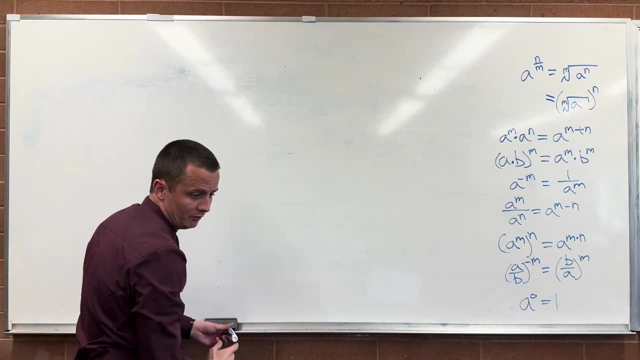 The 12th root of a to the 10,, b to the 11.. Alright, let's do one more like this And then I'll move on to the next type of example. So the next one he has is a fifth root. 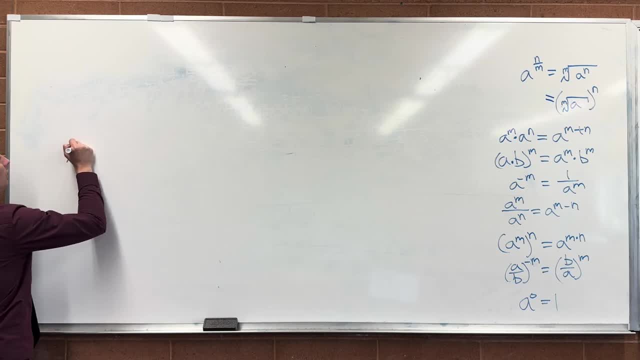 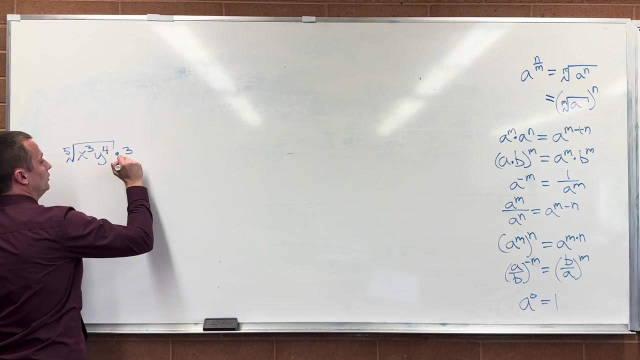 The fifth root of x cubed y to the fourth. So we have the fifth root of x cubed y to the fourth. All times the Lost, the problem. The cubed root of x squared y. The cubed root of x squared times y. 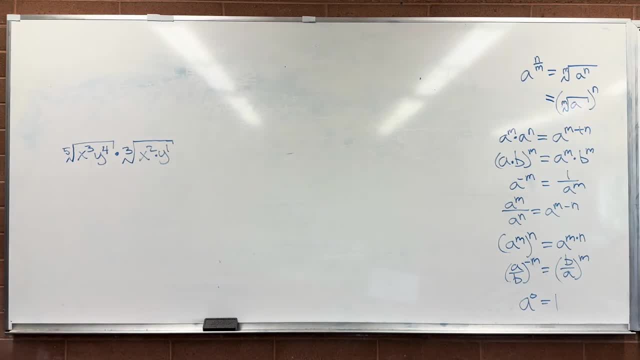 Think about that y as y to the 1.. Okay, I want a common denominator, so I need to multiply this by 3 and 3, and this by 5 and 5. And then I can put them all under my 15th root. 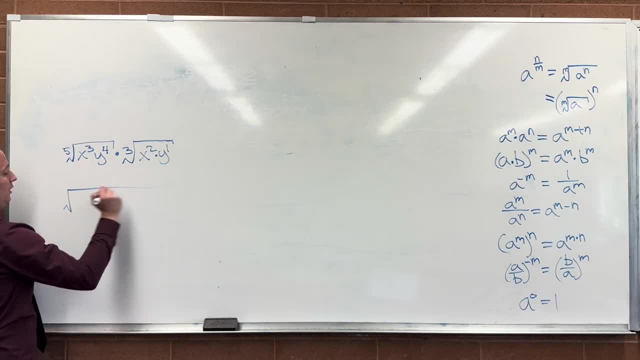 Yes, So this is going to be the 15th root of x to the 6. Multiplying this one by 3 is going to be x to the 9.. It's going to be really confusing when we multiply and when we add. 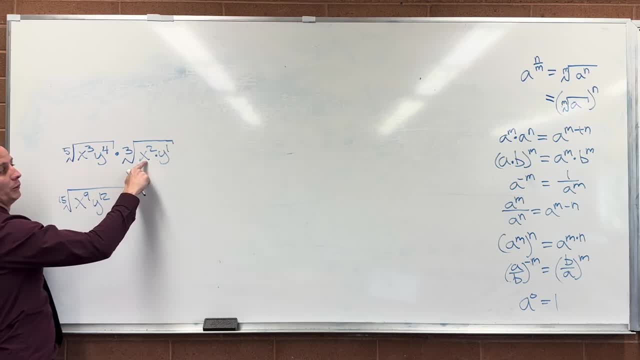 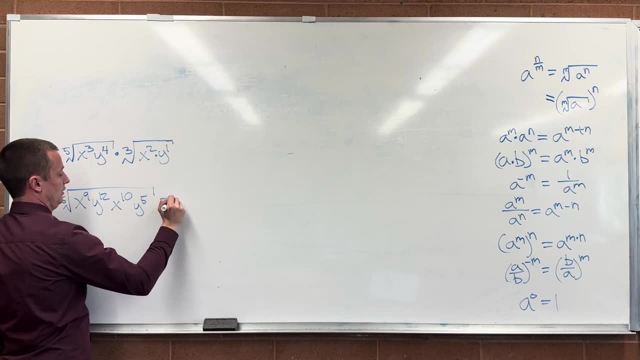 y to the 12.. y to the 12.. This one, we are multiplying it by 5, so that's x to the 10.. This one, we are multiplying by 5,. y to the 5.. Now, when you multiply terms, you add exponents. 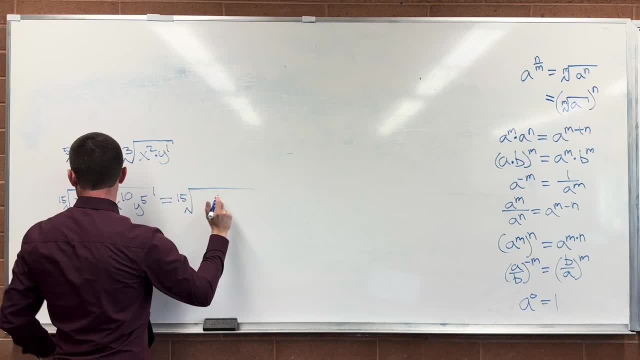 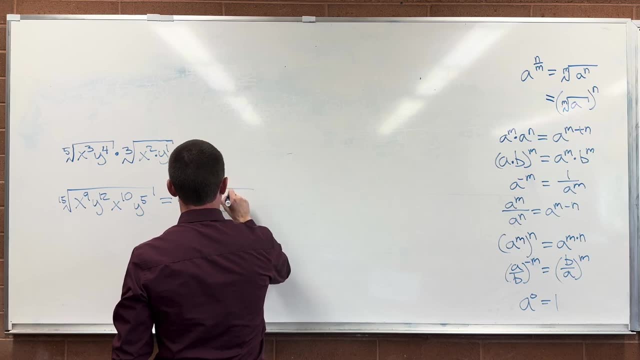 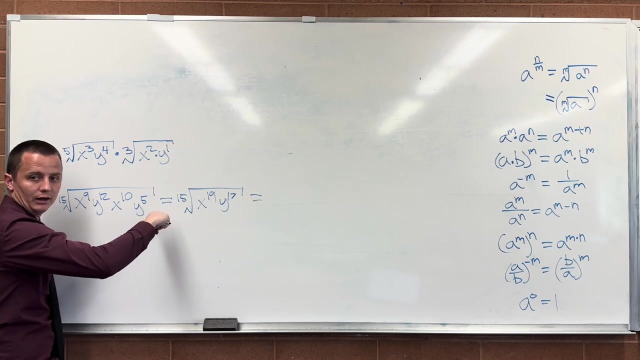 So this is the 15th root of x to the 19. Sorry, x to the 19,, y to the 17. 17. Now it takes 15 x's to get one out here, and it takes 15 y's to get one out here. 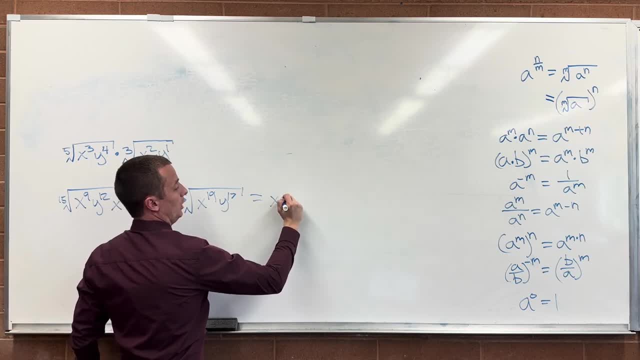 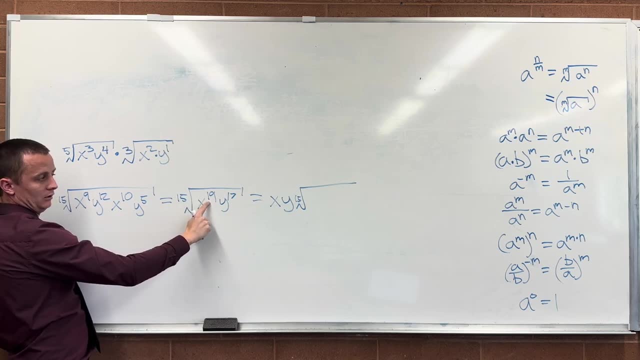 So I can pull out one x and one y and we're left with. if I pulled an x out inside, I'm left with. how many? 3., 4., x, 4. Because I have to pay 15 to bring an x out. 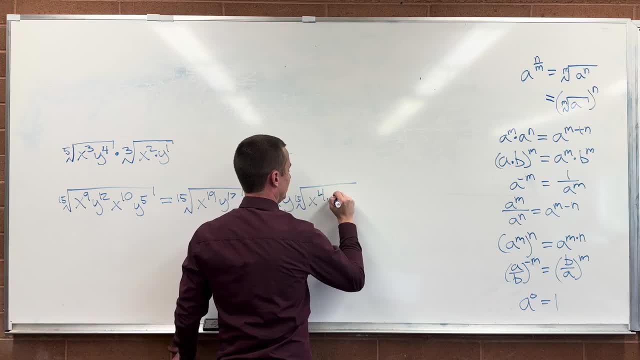 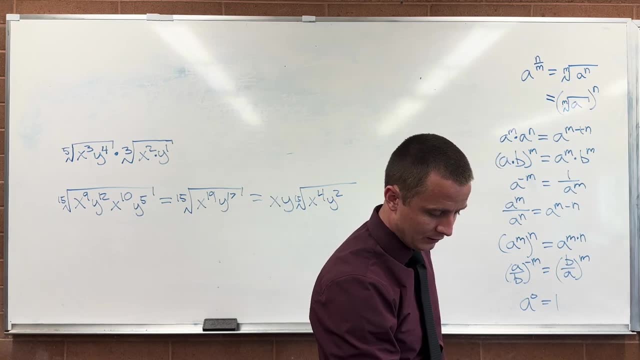 So this is x to the 4, y to the 2.. There we go, So x, y, 15th root of x to the 4,, y to the 2.. Okay, Which of these will be the hardest? 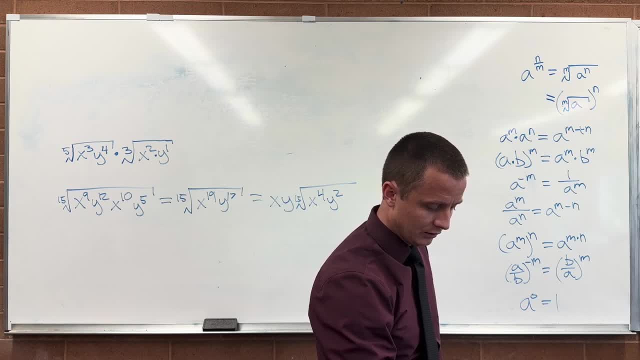 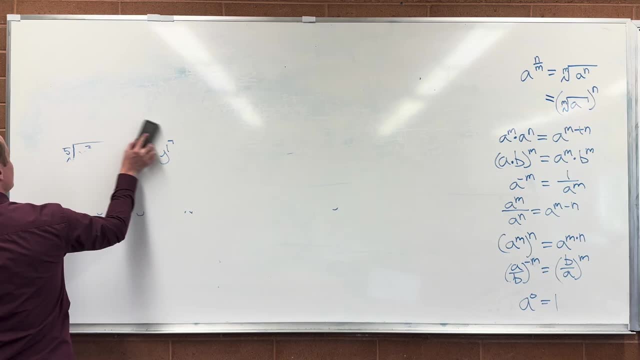 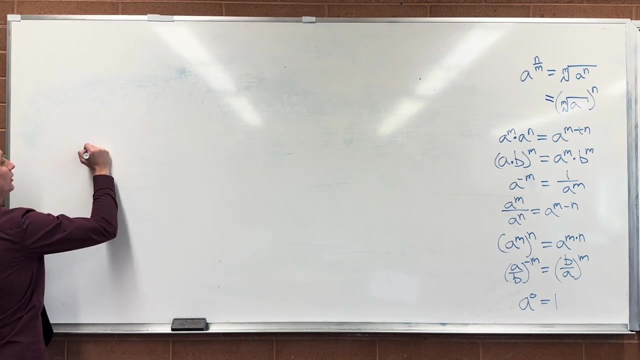 Let's do one with a fraction, because that might confuse you, Okay, So our last one that we'll do in this section is: we have got the 6th root of x to the 4,, y to the 3,, z to the 2,. 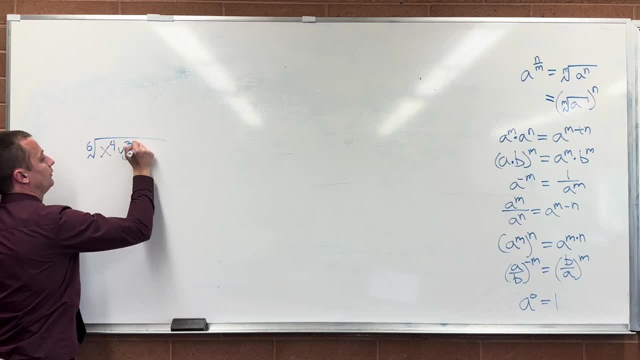 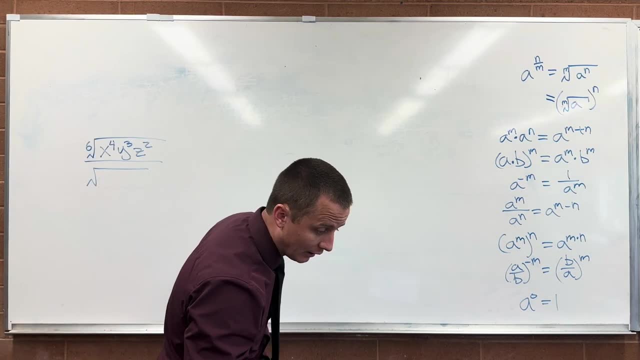 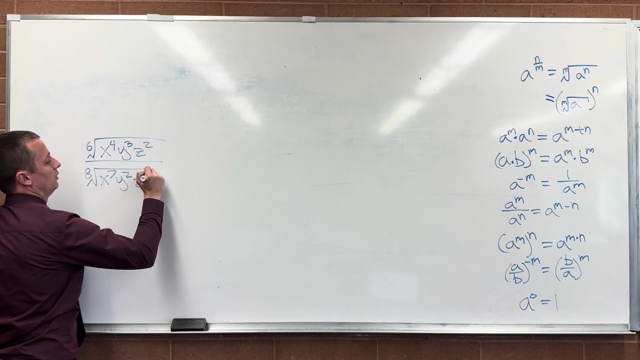 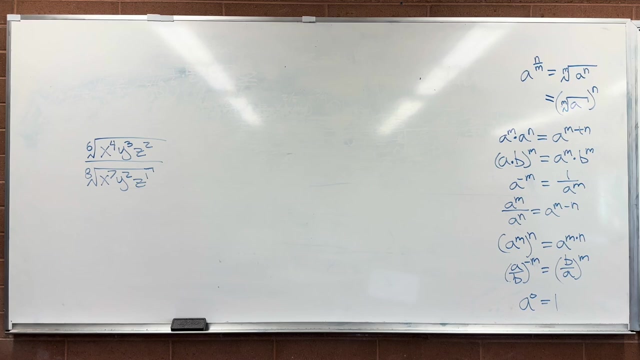 x to the 4,, y to the 3, z to the 2,, all over, all over: 8, 7, 2, 1.. 8, 7, 2, 1.. Alright, So now this time we're dividing them rather than multiplying them together. 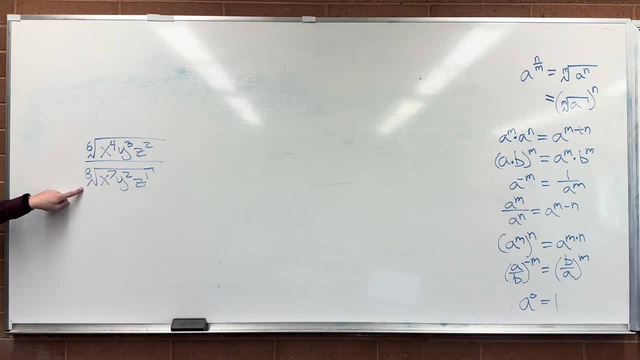 We still cannot divide these two things unless they have the same root here. So we're still going to do the same thing: Get our common denominator. So what's our common denominator between 6 and 8? going to be 48.. We can go smaller. 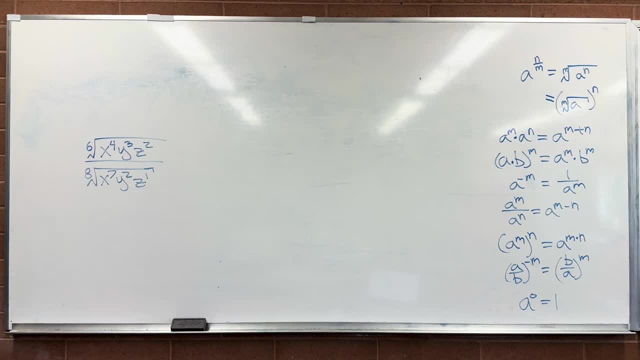 24. 24. 24.. So how do I get 6 to 24?? Times it by 4.. Times it by 4.. So I need to times all these ones by 4.. I need to times all these ones by 3.. 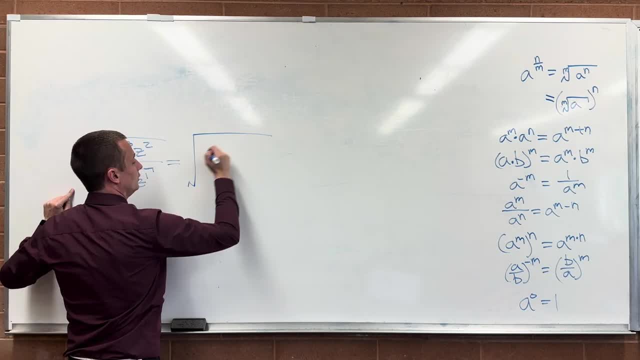 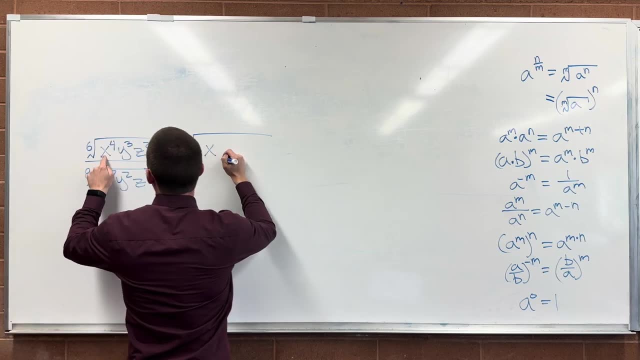 I'm going to write this all in one: big to the 24th radical. So taking the 24th root of, we were multiplying these ones by 4, so multiplying the x to the 4, x to the 16,, y to the 12,, z to the 8.. 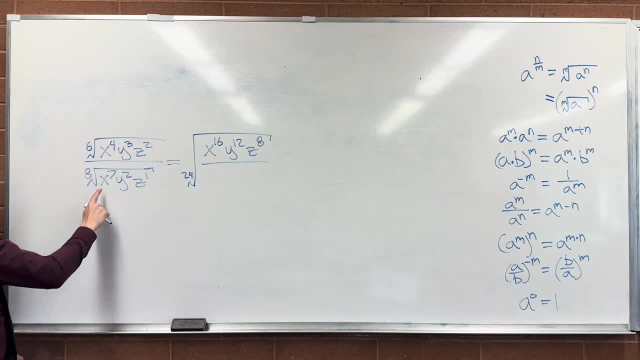 You're going to get confused by those over and over again. Down here we have x to the 21,, y to the 6,, z to the 3, right Now we need to combine these. So if I put them all in the numerator, 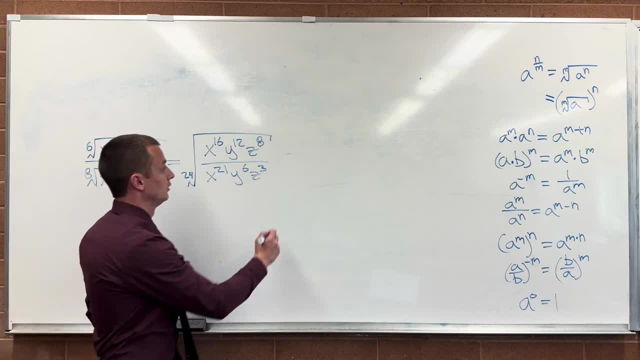 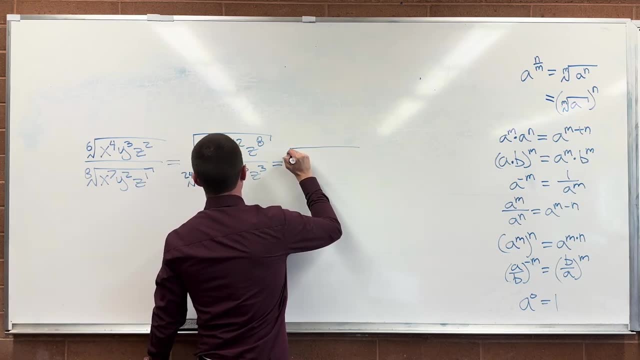 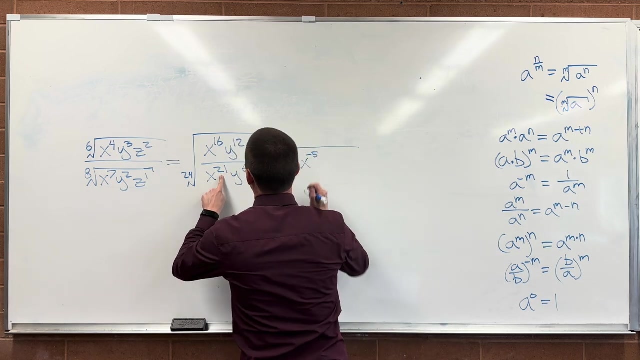 that takes all these ones and makes them negative. You with me. So this is going to be the 24th. root of 16 minus 21 is Minus 5. Minus 5.. 12 minus 6 is: 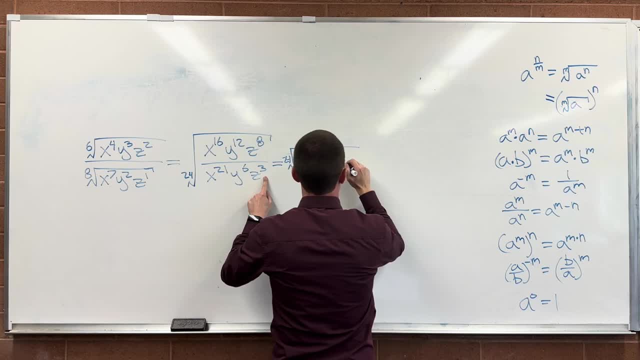 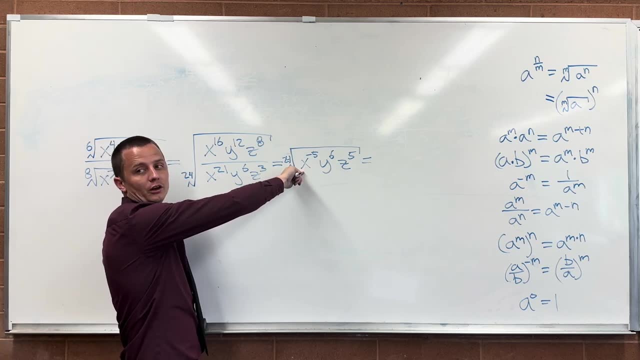 6. 6.. 8 minus 3 is 4.. 8 minus 3 is 5. 5.. And then finally we notice: OK, that's a negative exponent. It's all said and done. 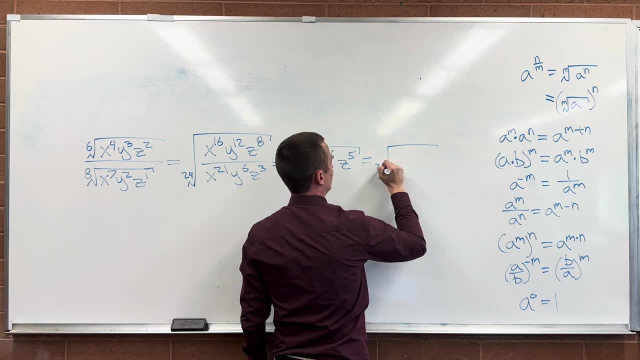 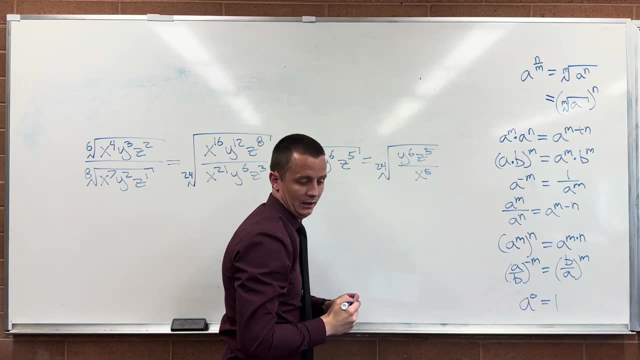 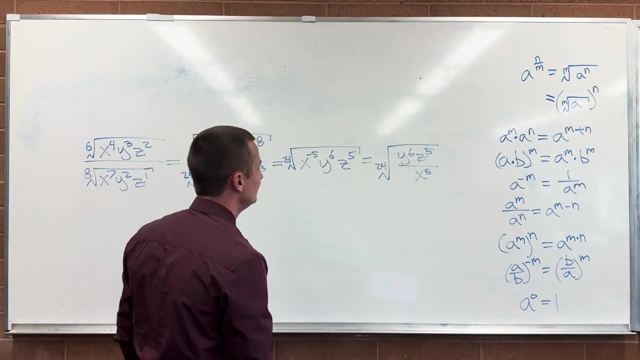 Let's put it back in the denominator. So this is the 24th root of y to the 6,, z to the 5,, all over x to the 5.. OK, Oh, Now it's not that we're still on track. 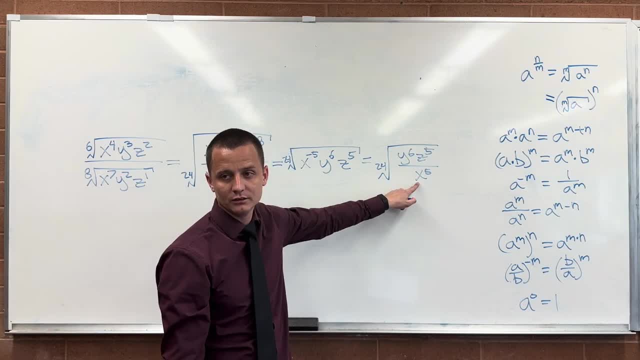 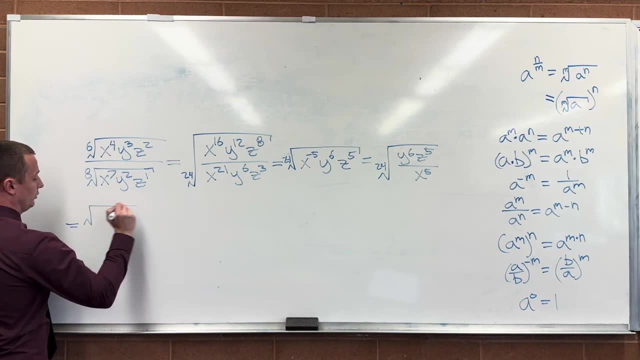 but this is not our answer, because we have a radical in the denominator Yeah. So let's finish up the process. Sorry, My bad. So this is the 24th root In the numerator. we still have y to the 6,, z to the 5.. 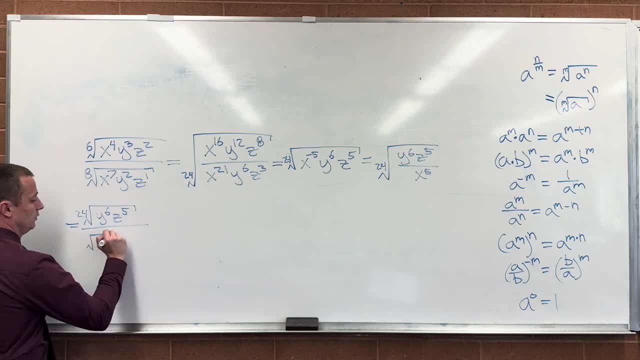 But in our denominator we also have the 24th root of x to the 5. Right Yeah, This is the same thing as this. We do not want radicals in the denominator. So how many x's? How many more x's do I need to have? 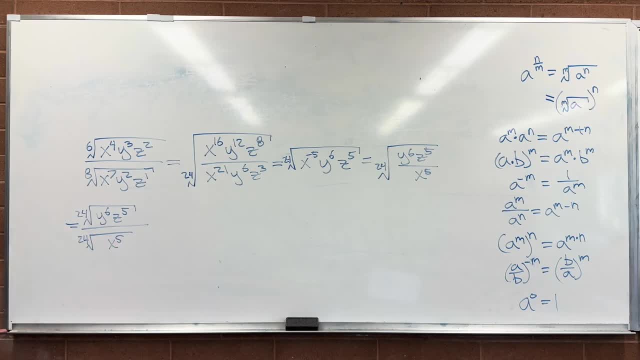 How many more x's do I need down here to cancel it out? How many x's would I need to have in here to pull it out? I need 24 of them. right, Right. The 24th root of x to the 24 is x. 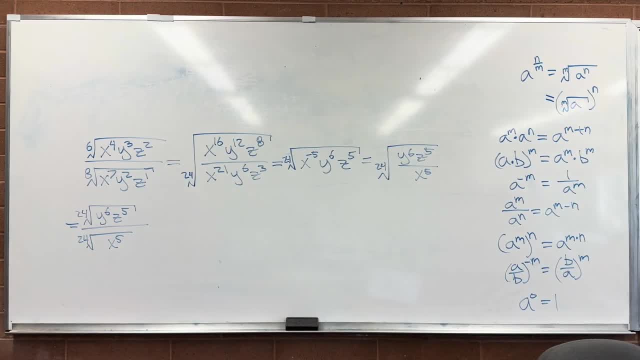 So that's how we can cancel it out, Or that's how we can pull out of the radical. So how many more do I need down here? I have 5.. I need 19.. So I need to multiply this top and bottom by the 24th root of x to the 19.. 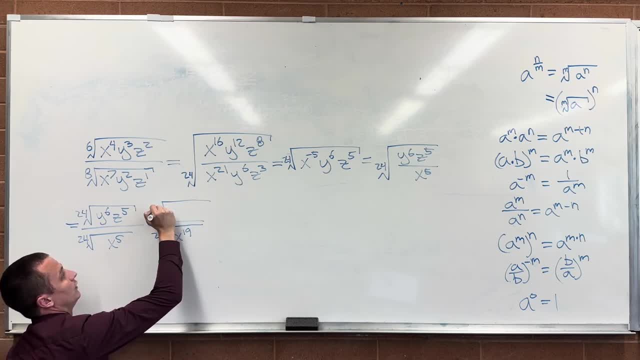 And the 24th root of x to the 19.. Oops, 19.. All right, And what does that leave us with? In the numerator, we have the 24th root of how many x's do we have? 19.. 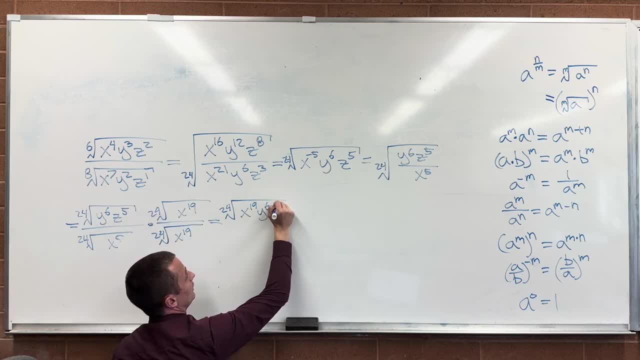 How many y's do we have 6.? How many z's do we have? 5.? All over, I have 19 here and 5 here, for a total of 24. 24. Take the 24th root and that leaves us with just x. 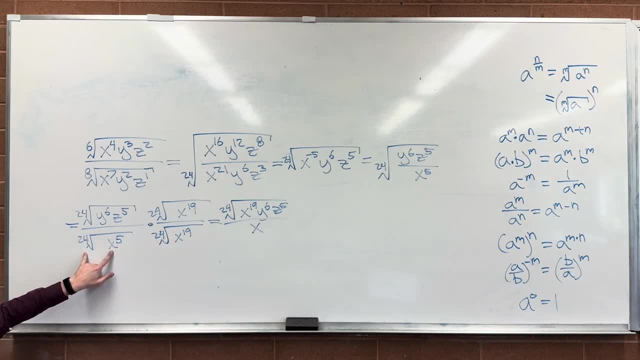 That's the whole reason. we did that right, Finding the number such that when we multiply it by this, we get just x. That's what we were after. Okay, And that is his answer. All right, Last section, And the last section is working with complex numbers. 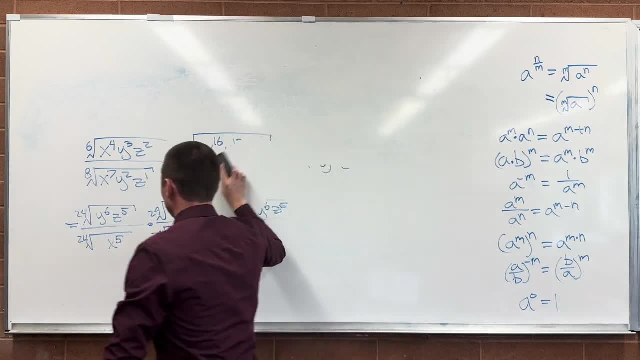 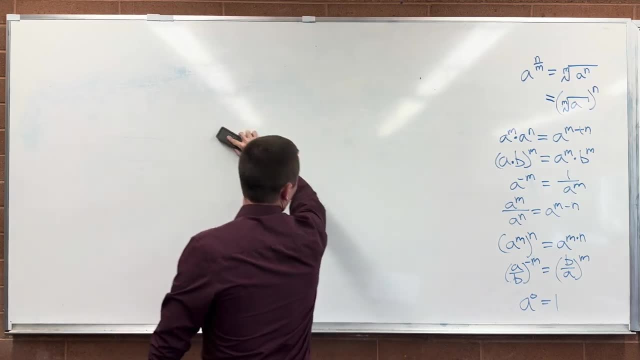 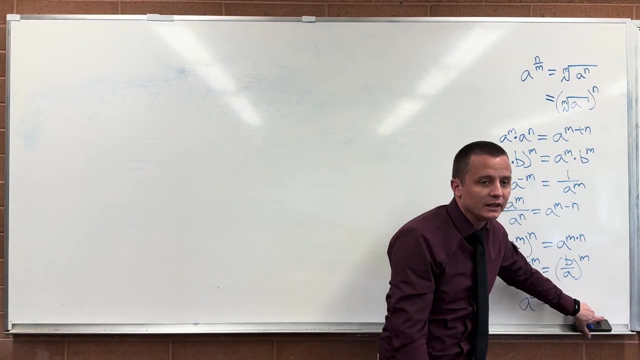 You ever come across complex numbers before? Yes, I think You think. Yeah, Let's kind of walk you through a little bit of history of this. Take you back to when you were in basic counting. I guess I'm a toddler. 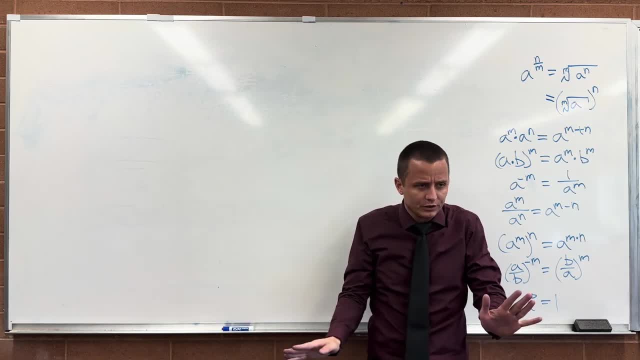 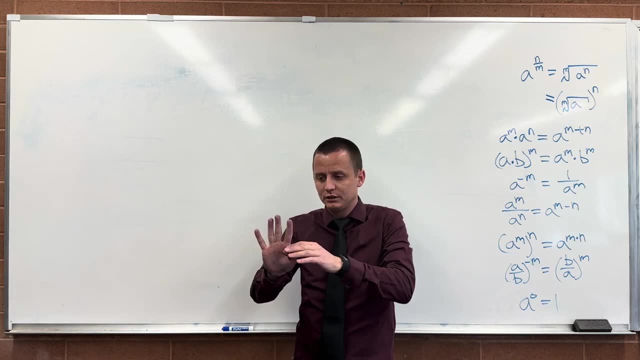 Right, And when I'm first teaching a toddler how to do arithmetic, I might ask the toddler: what's 5, take away 3? And what does a toddler know how to do? They start off with 5 and they say: put down 3 fingers, and they say it's 2.. 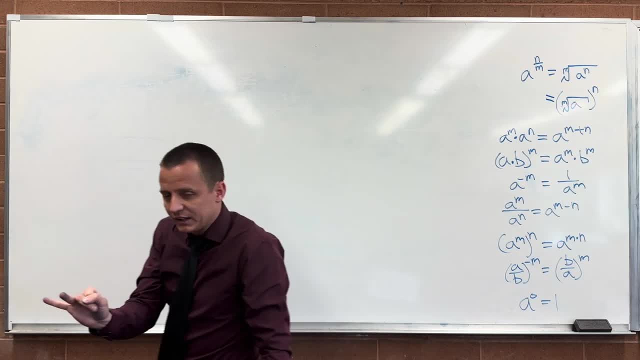 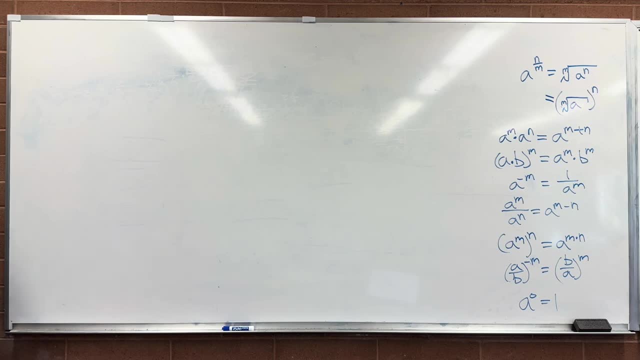 Right, And they can do that. Now, if I ask the toddler: okay, this time I want 3,, now take away 5.. And they'll say, okay, 1, 2.. You can't do that, It's broken. 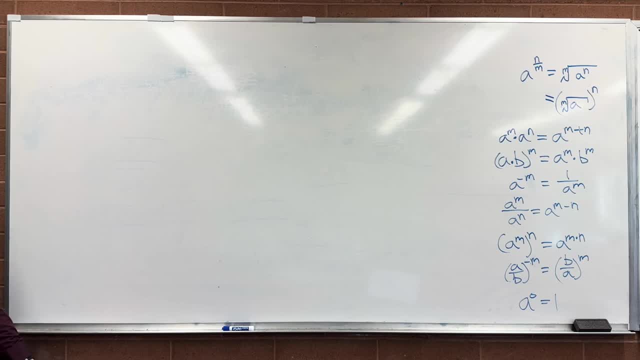 How can you do 3, take away 5? And you have to then explain to the child about negative numbers? See, there's nothing wrong with negative numbers. They're perfectly valid numbers And at first the child's going to be confused. 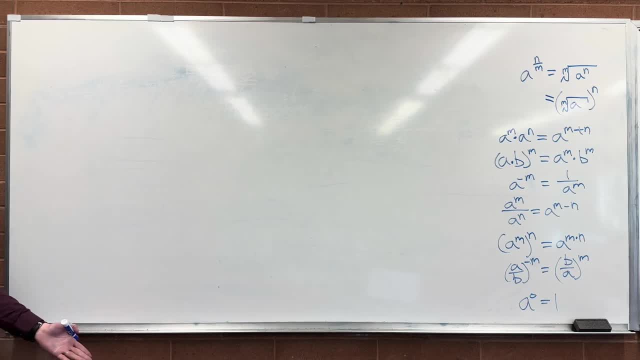 They'll say that's not a number. Show me negative 2 apples. What do you mean? negative 2 is a number And they're going to resist. And you didn't like going to that transition, But eventually you got comfortable with negative numbers. 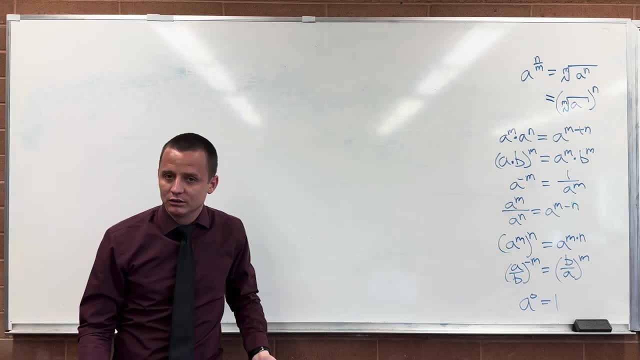 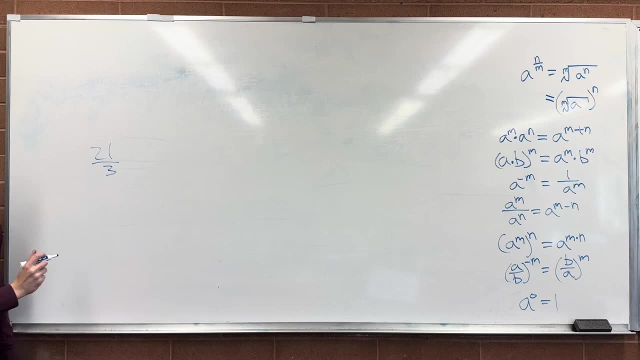 And you went a little bit further and you started doing division And you were asked to calculate problems like: what is you know 21 times? What is you know 21 divided by 3? And you came out with 7.. 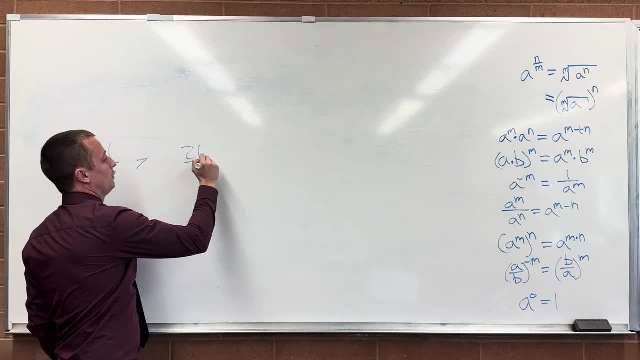 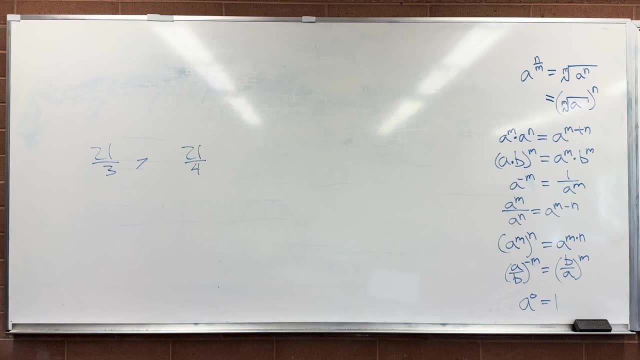 And then someone says, well, what's 21 divided by 4?? And you say, is it 5?? No, Is it 6? No, It doesn't work. And you say, sure it works, It's 21. fourths: 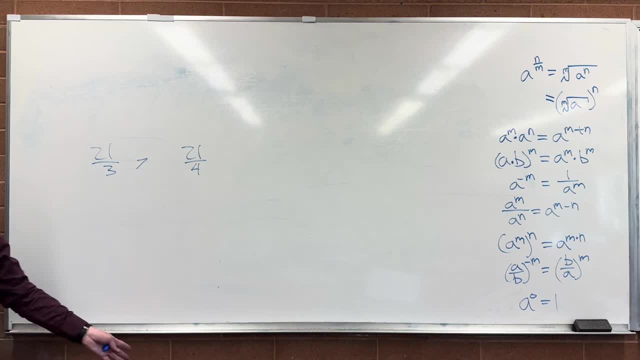 That's a perfectly good number, And then they kind of feel like you're cheating. You didn't solve the problem. You're just saying the answer is the problem. There's nothing wrong with that answer: 21 fourths. A little bit of time goes by. 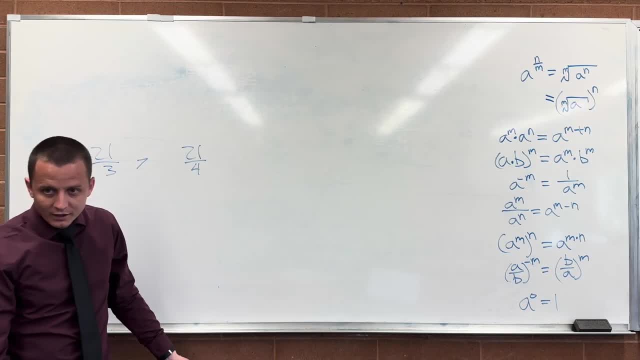 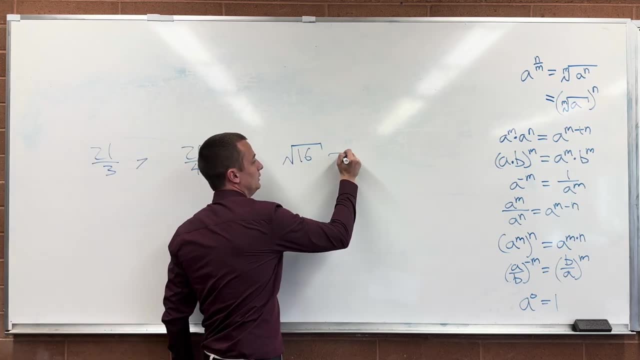 And you start being totally confused. And you're told to calculate radicals. And I might ask you to calculate something like the square root of 16.. And you calculate it And you say that's 4.. Yay, I say. OK, what's the square root of 2?? 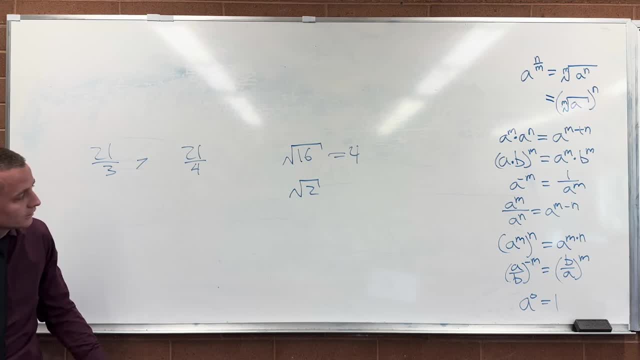 It doesn't have one. What do you mean? I say: yes, it does. What's the square root of 2?? It's the square root of 2.. That's what it is. It's a perfectly fine number. You say you're cheating. 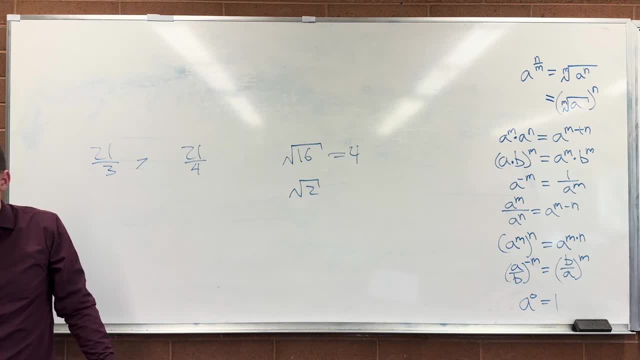 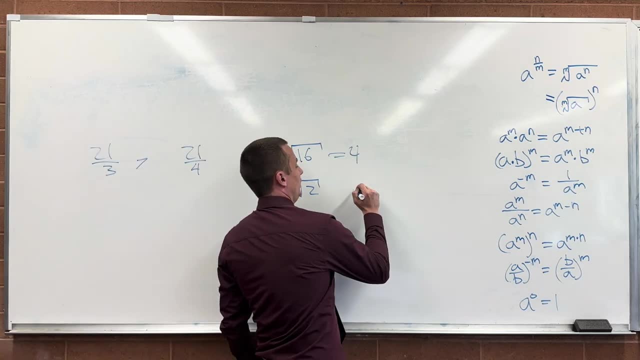 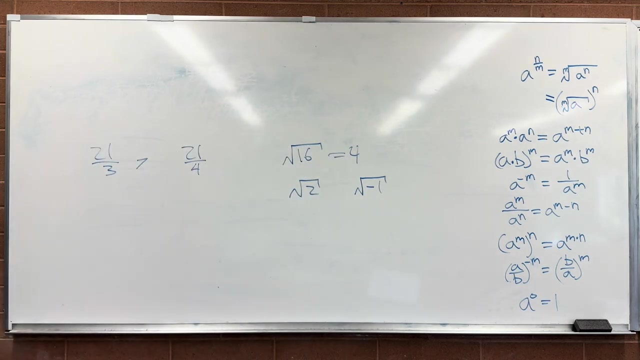 You didn't figure it out. No, That's it. That's what it is. Now we come to the next leap that you're not going to like taking. What is the square root of negative 1?? What times? what gives you negative 1?? 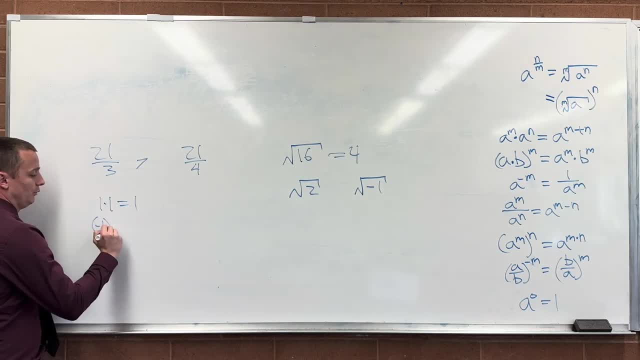 1 times 1 is 1.. Negative 1 times negative 1 is 1.. What's the square root of negative 1?? No, Negative 1 times negative 1 gives you 1.. It doesn't give you negative 1.. 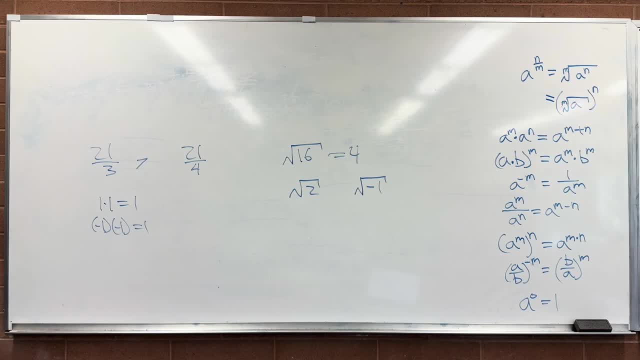 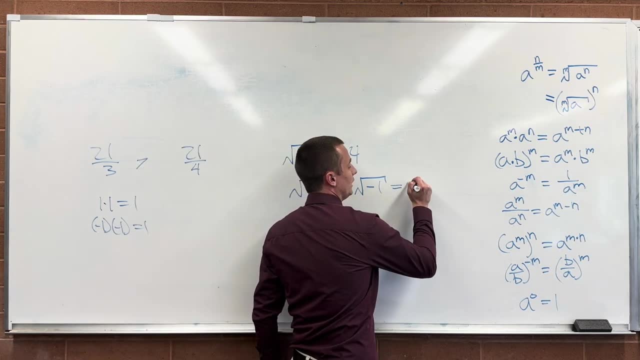 1 times 1 gives you 1.. Nothing, I don't know. Nothing, I don't know. The answer is the square root of negative 1, which we're going to start calling i. i we define to be the square root of negative 1.. 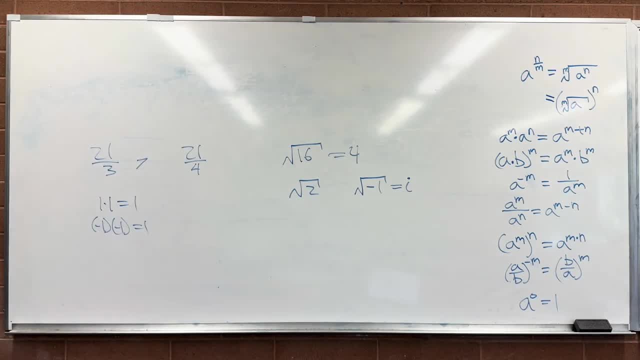 What's the square root of negative 1?? It's the square root of negative 1.. It's i, That's what. it is Perfectly fine saying it that way. Perfectly good number, And you're not going to like this. 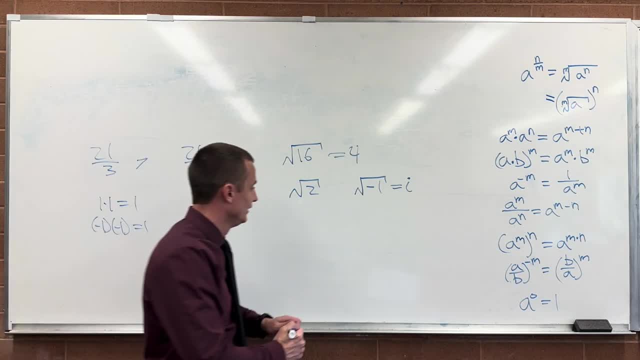 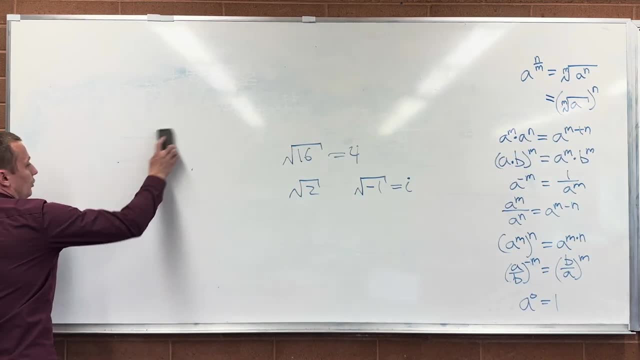 But it is OK. OK, So now we introduce i. i is the square root of negative 1.. Let's start getting comfortable with this. i thing Let's start tackling i to some powers. What's i to the power of 0?? 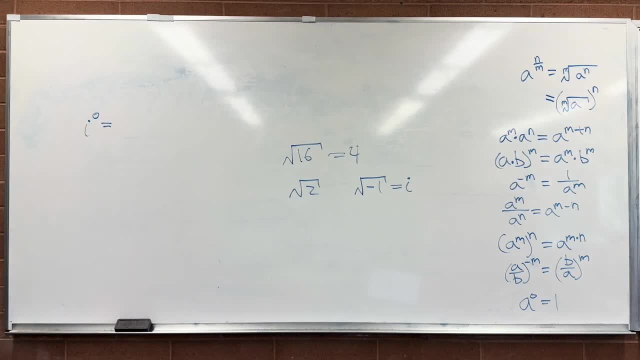 Negative 1. Anything to the power of 0 is 1.. 1. Right, What's i to the power of 1?? Negative 1. It's just i. Anything to the power of 1 is just that thing. 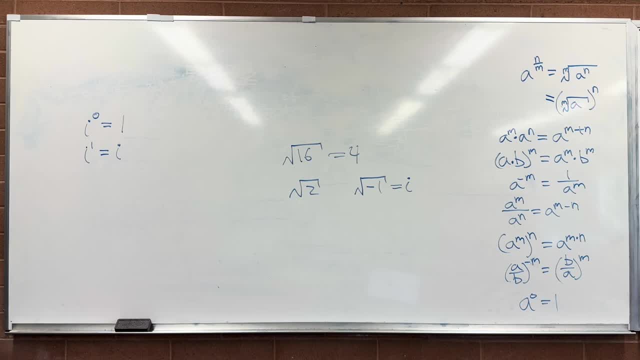 x to the power of 1? x 79 to the power of 1? 79.. 1 third to the power of 1? 1 third, Anything to the power of 1 is just that thing. Now, what is i squared? 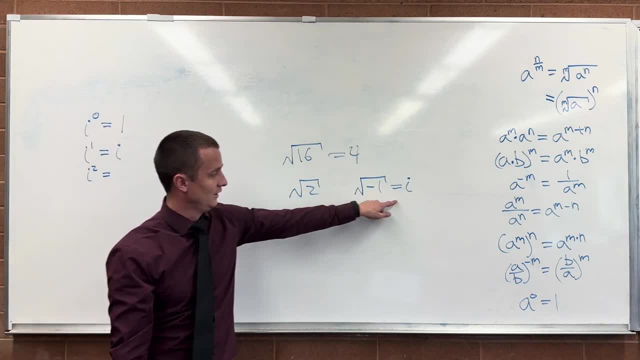 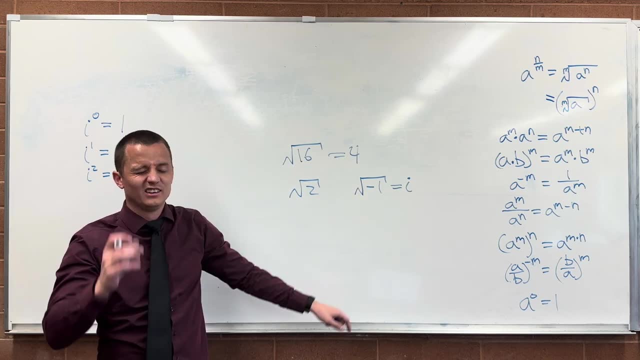 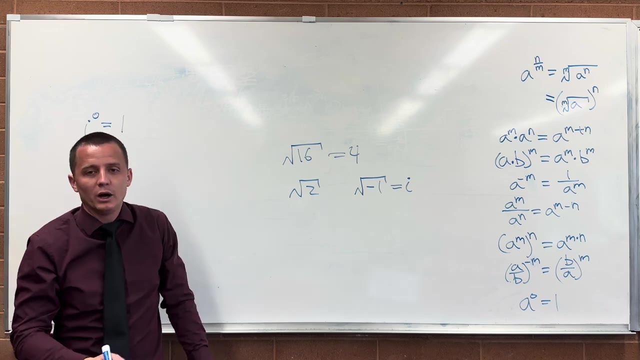 Negative 2.. What is i squared? 2. i, Negative 1., 2. i 2.. By definition, i is the square root of negative 1.. What is the square root of negative 1 times the square root of negative 1?? 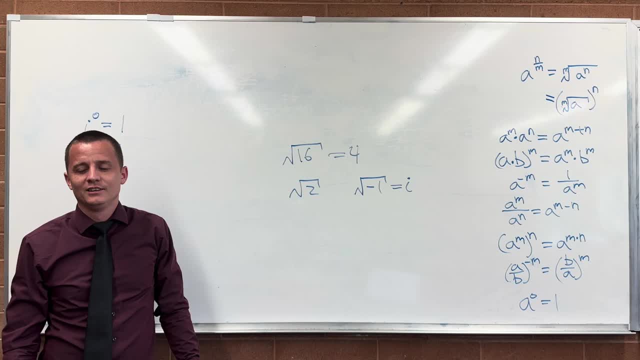 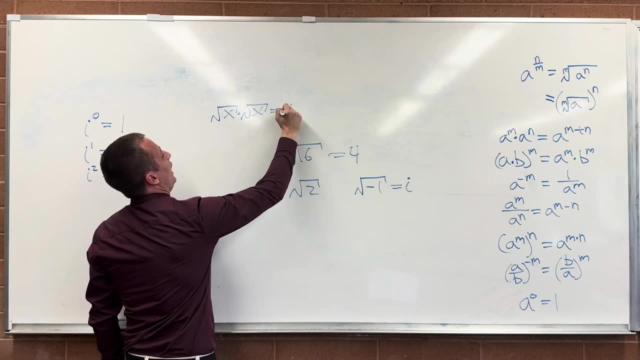 1. Oh, I don't know. What is the square root of x times the square root of x? Oh, x, x. What is the square root of negative 1 times the square root of negative 1?? Negative 1.. 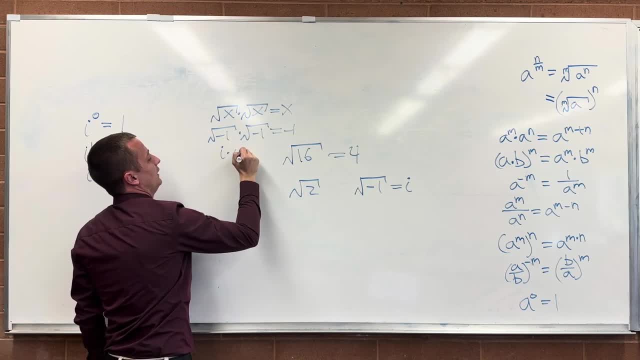 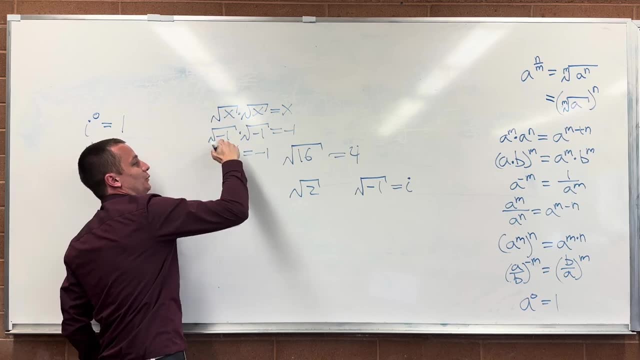 Negative 1.. What is i times i, i 1.. Oh sorry, Negative 1.. I is the square root of negative 1.. I just rewrote this exact thing twice. All right, Scan takes from getting used to. 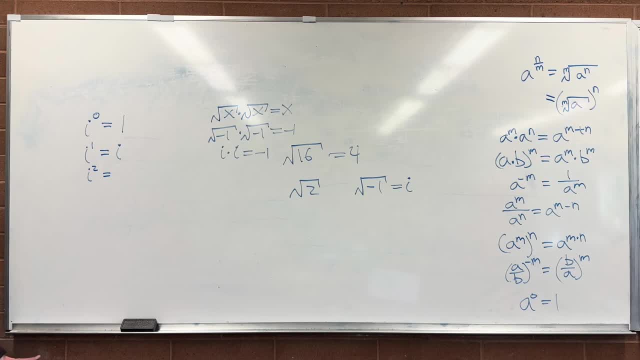 What is i? It's the square root of negative 1.. That's what it is, OK. So what's i squared? Negative 1., Negative 1.. We're getting there, Boom. OK, Let's calculate. i cubed. 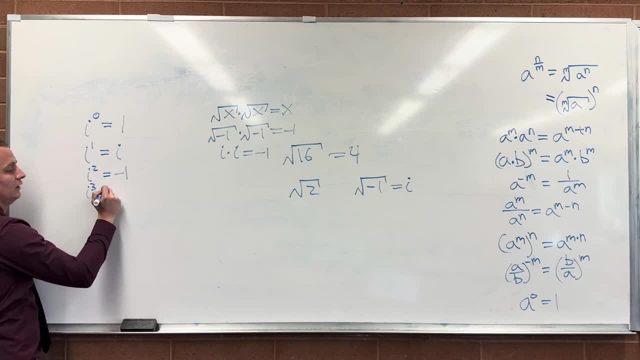 What does that equal? 1. No, it's. 2. It's i Negative? 3. No, because it makes: Look i cubed. 1. Is the same thing as i. 2. i, 2.. 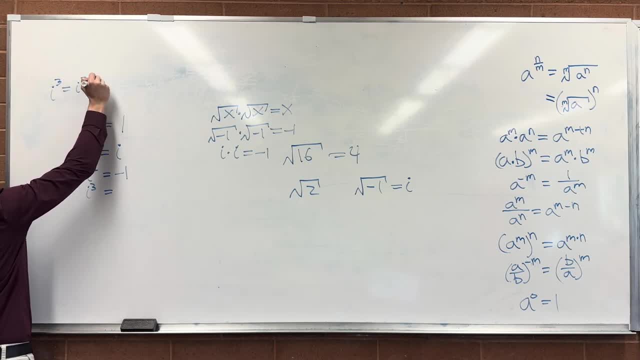 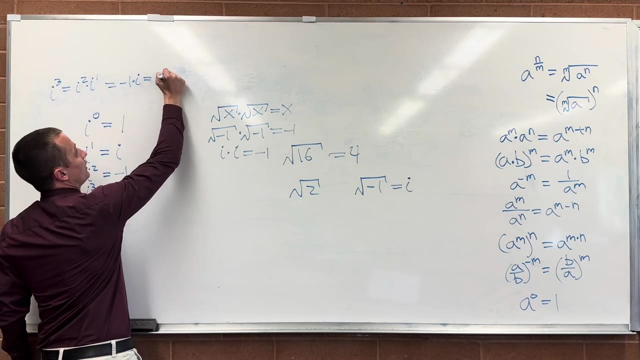 1. What does i squared times? i write Yes. What's i squared, Negative? 1. What's negative 1 times i? What's negative 1 times anything? 1. It's just the negative of that thing. What's negative 1 times x? 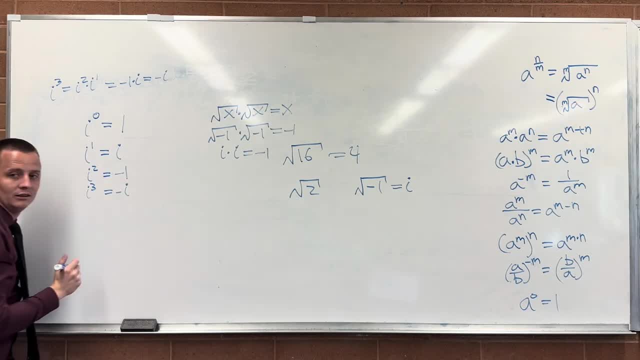 Negative x. So this is just negative i. Oh OK, That's retarded. Why is it retarded? It is It's I squared which is negative 1. It's just times I. You basically took this. times this: I to the 1, times I to the 2 gives you I to the 3.. 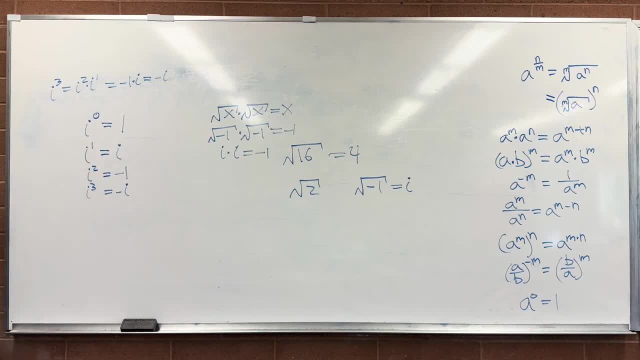 I times negative 1 gives you negative I Right. Okay, Let's do the really tricky one. What's I to the 4? equal to I to the 4 is 1.. 1!. How did you get that? Because I to the 4 is what. 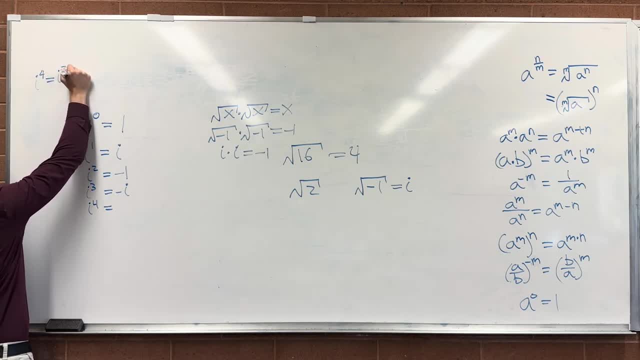 It's just negative. It's I squared times. I squared What's I squared? Negative 1.. What's I squared? Negative 1. Negative 1 times negative 1? 1. Positive 1.. So this was equal to negative 1 times negative 1,. 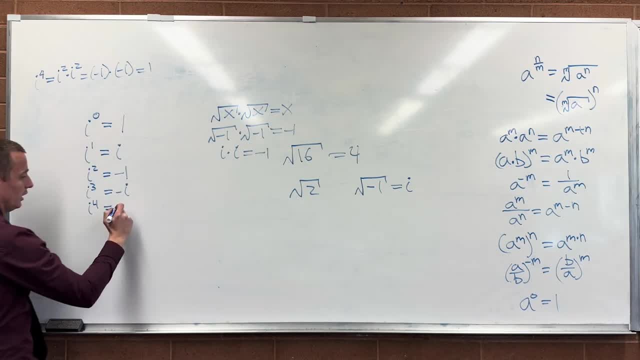 which is equal to positive 1.. So I to the 5 is positive 1. Or I to the 4 is positive 1. Or I to the 4 is positive 1. What's I to the 5?? Look, I'm taking the previous number and I'm multiplying it by I. 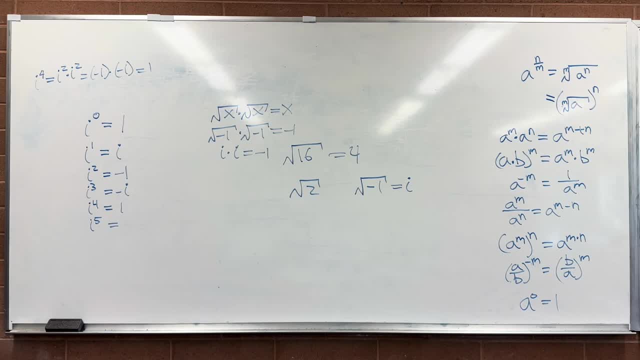 What's 1 times I? I Anything times 1 is just that thing. Alright, Now let's calculate I to the 6, which is just equal to the previous thing times I. What's I times I, Negative 1.. 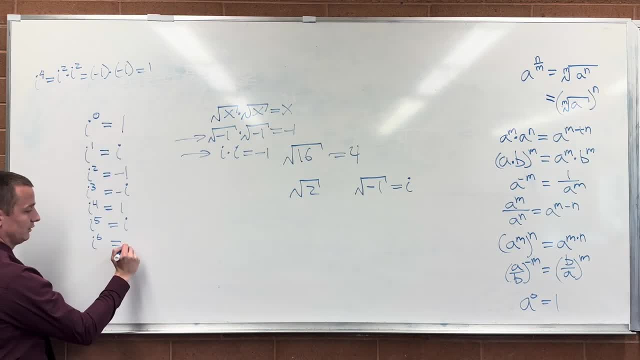 Negative 1.. This is negative 1.. What's I to the 7?? Negative I, Negative I. She's seeing it. Next one's going to be 1.. Next one's going to be I. I times 8 is going to be negative 1.. 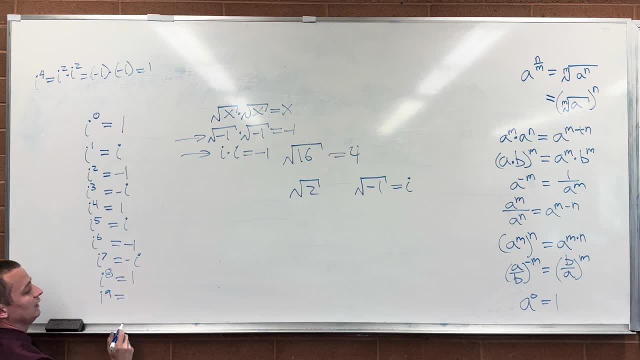 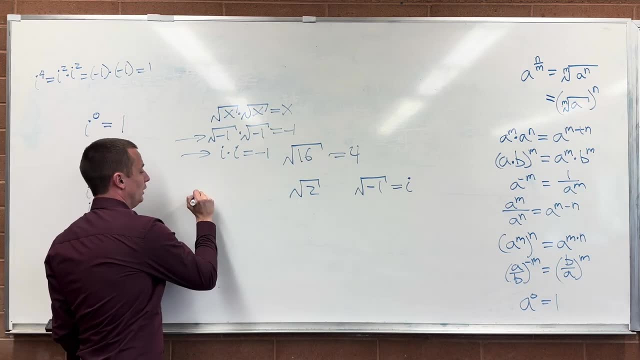 It's equal to 1.. I to the 9 is equal to I, I, And so on and so forth. Alright, Let's get tricky now. What's I to the 100?? 1., 1.. How did he do that? 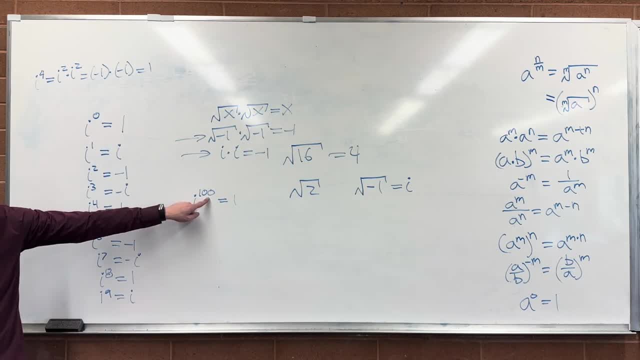 I don't know, Because 100 is a multiple of 4.. Oh, So this is I to the 4.. I to the 4 is 1.. It's I to the 4 25 times. Okay, Let's try another one. 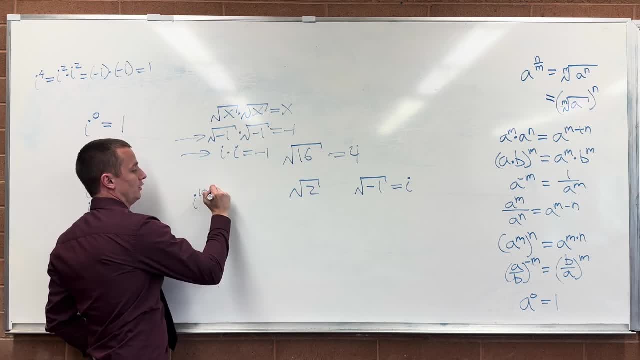 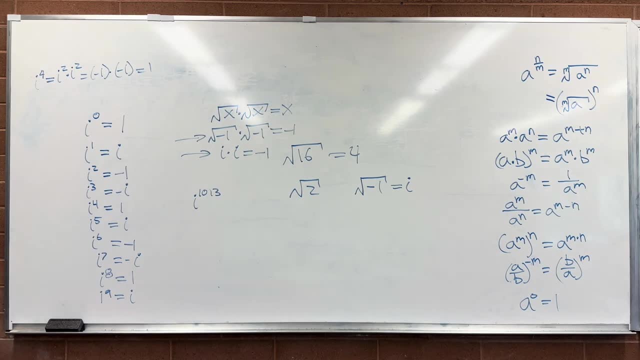 What's I to the 1013?? It's going to be negative 5.. No, You're just throwing out stuff. Yeah, What is the closest multiple of 4 to this? 4 and 9.. Oh sorry, I want to say 12.. 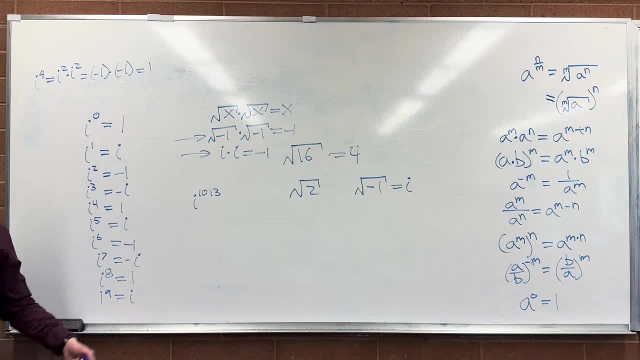 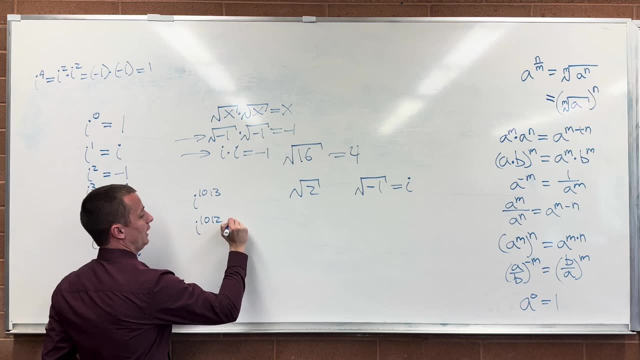 1,012.. 4 goes into 1,000.. 2 or 50 times 4 goes into 12, 3 times. So this is I to the 1,012 times I, That one's a multiple of 4.. 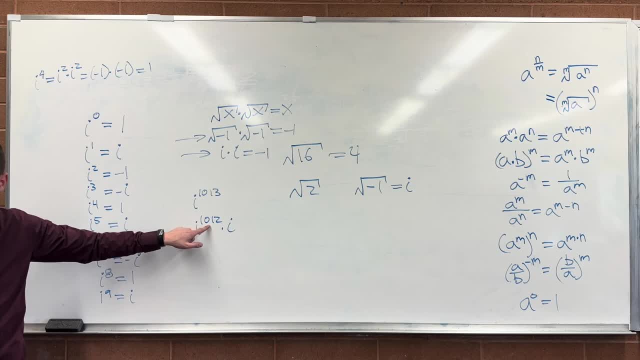 And I to any multiple of 4 is just 1.. 1 times I. is I You getting it? I think these are going to be some of your problems. It's going to say I to some really big number And you're going to have to work it out. 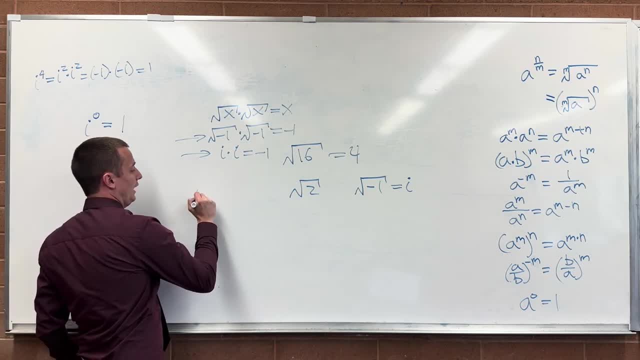 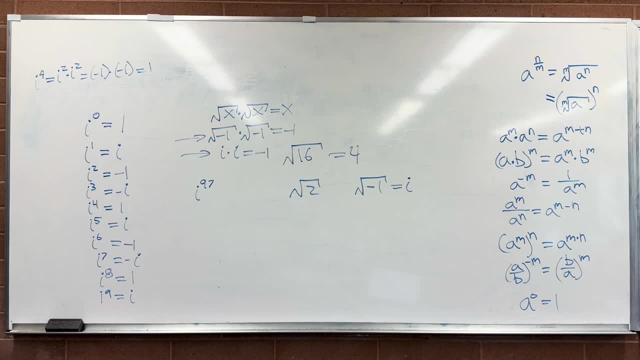 What is I to the 97?? What is I to the 97?? Well, you could do 96, which is why is it? You don't need to divide it. You just know 96 is a multiple of 4.. 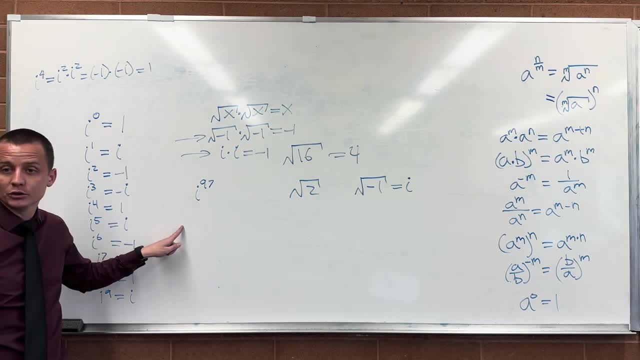 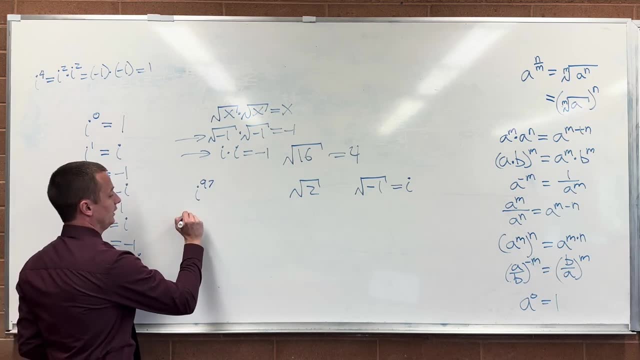 That's all you need to know. 96 is a divisible, So you have 96 as a multiple. So it's just I. 96 gets you to 1.. One more gets you to I, So this is I to the 96, which is a multiple of 4,. 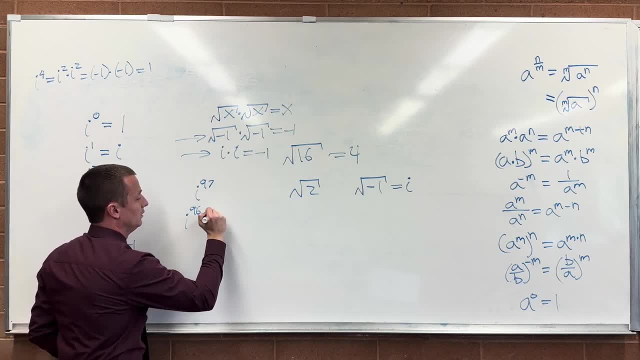 which, who cares? it's a multiple of 4, times I to the 1.. I to the 96 is 1.. I to the 96 is 1, times I to the 1.. You know, it's just I. 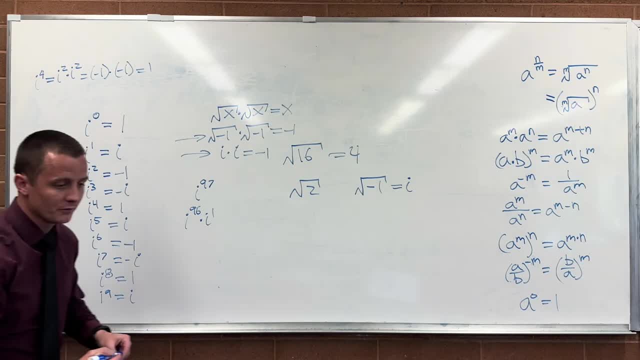 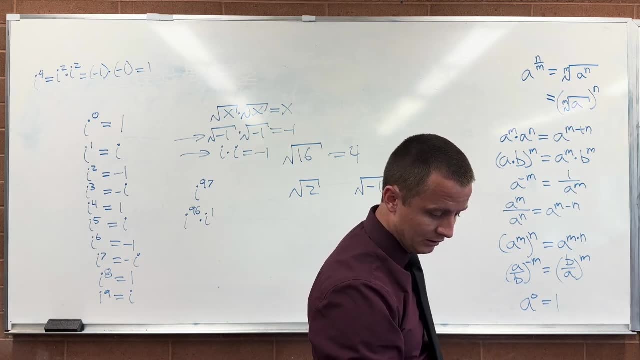 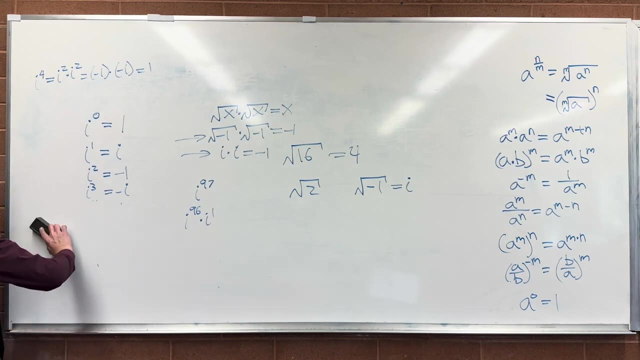 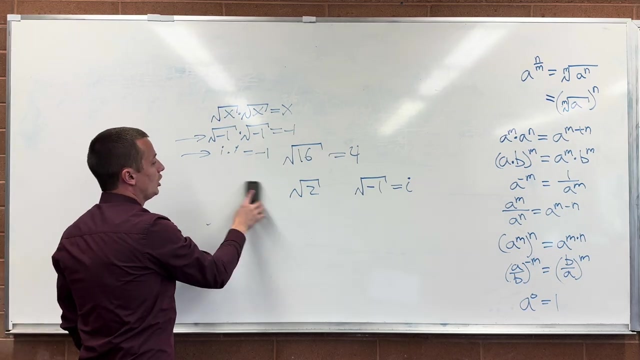 That's how these are going to work. OK, So a bit of a side note. Now let's get into complex numbers. What is a complex number? A complex number is a number that has a real part and an imaginary part. It does not mean that it's something that is imaginary. 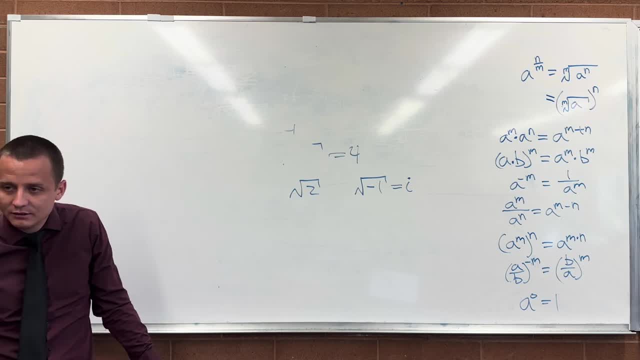 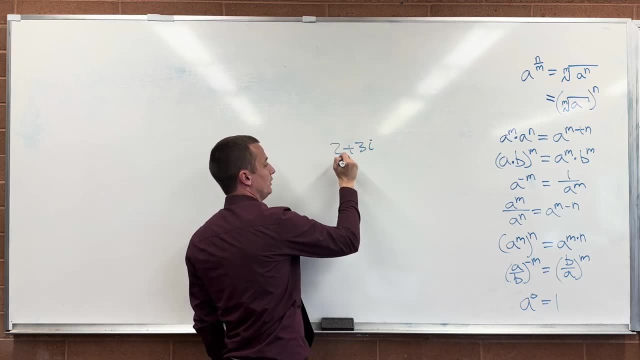 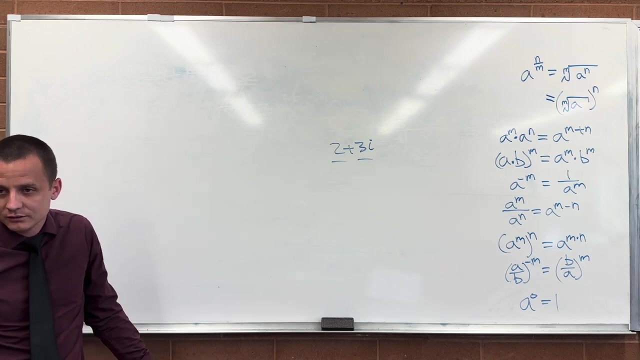 It means that it is some multiple of I. So an example of a complex number is 2 plus 3I. We call this the real part, This is the imaginary part, And together we call it a complex number, And you basically just treat the I's like they're their own variables. 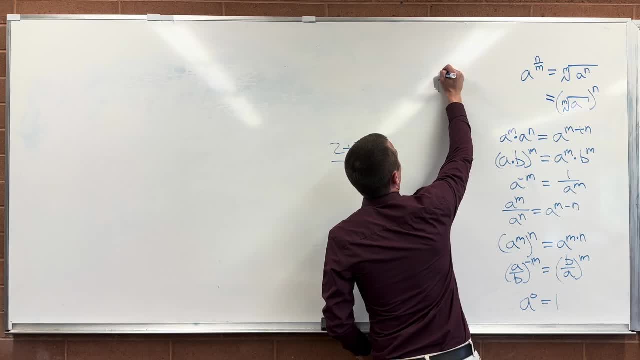 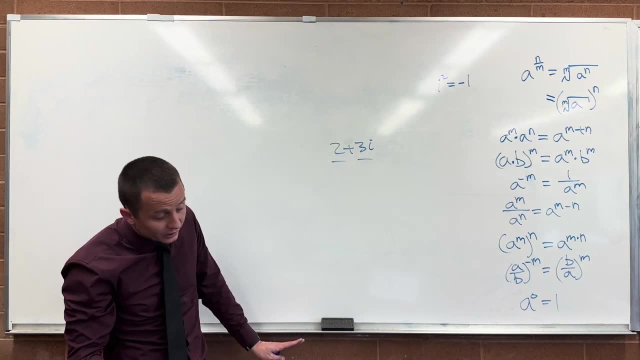 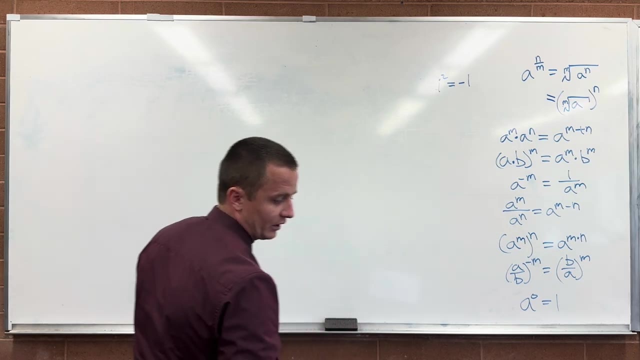 Just remember that, always and forever, I squared is equal to what Negative Negative 1.. And that's pretty much most of what you need to remember when you're working with these complex numbers. So let me give you an example. He's going to have you add two complex numbers together. 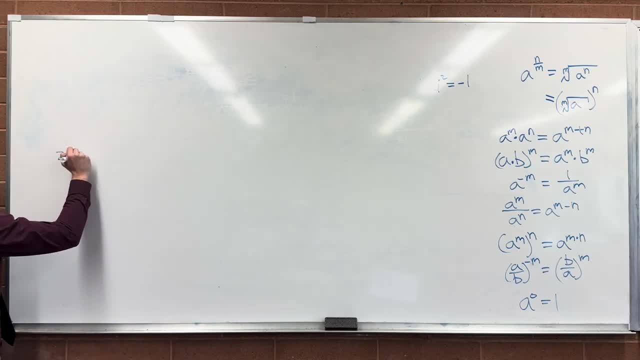 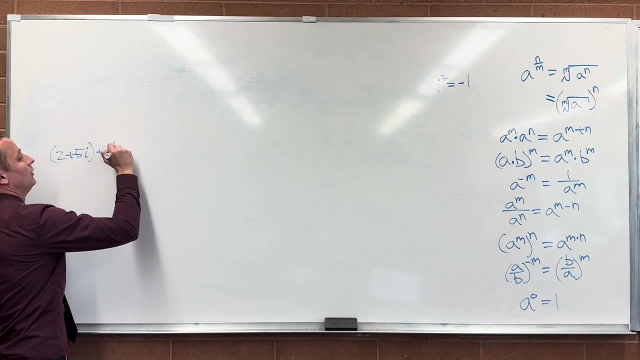 So you're going to take the complex number 2 plus 5I and you are going to add to it the complex number 4 minus 7I, And this works exactly the way you would have expected. Add up all the real parts. 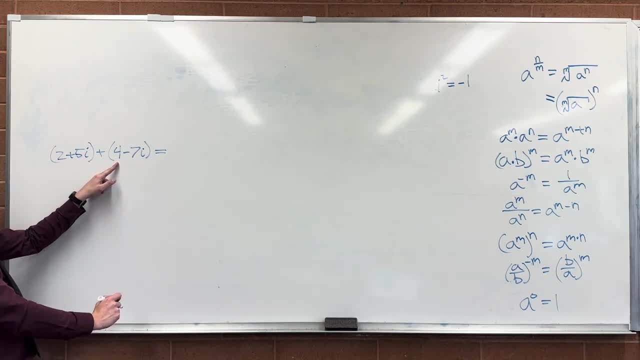 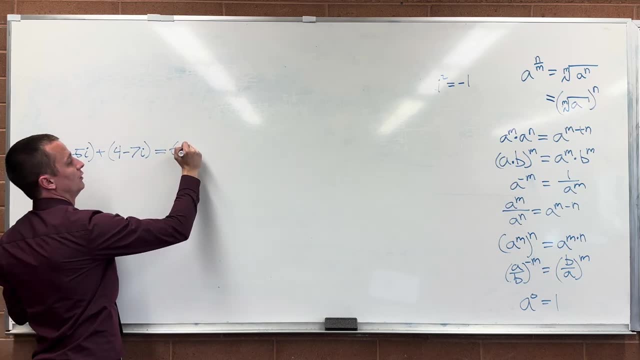 2 and 4 gives us 8. We're adding, not multiplying, 6., 6. And 5 and minus 7 gives us 3. Minus 2I- Oh, I'm such an unknown. 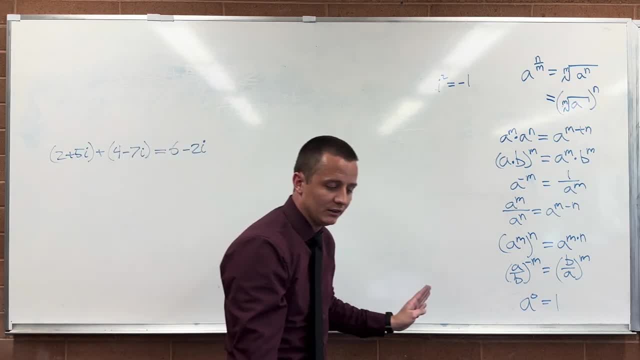 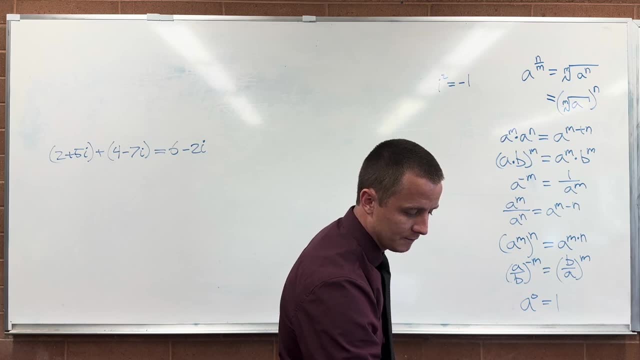 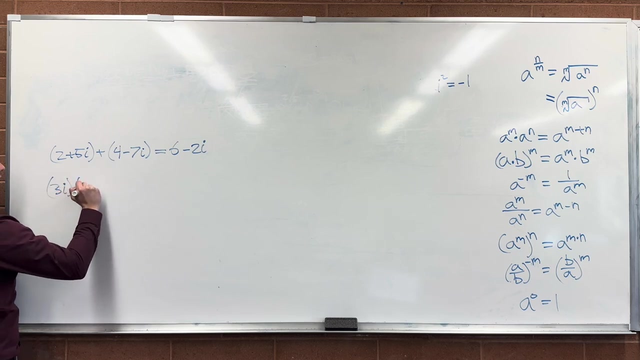 Right Yeah, So you just add the real part to the real part, the imaginary part to the imaginary part Works exactly the way you expect. Multiplying is where it gets more interesting, So let's try this one. We have 3I times 7I. 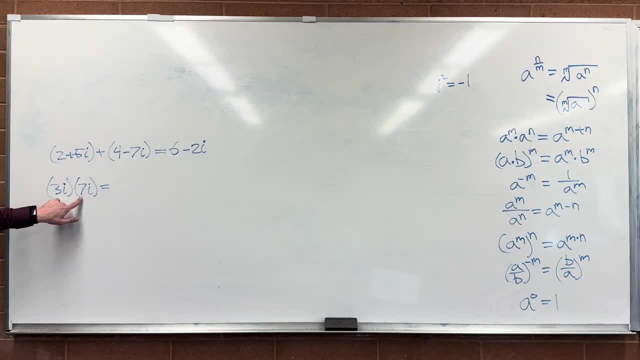 What does that give you? Do the real part first. Go ahead: 21I, 21I squared, Because you have an I times I, I, And what is I squared? Negative 1., Negative 1. So this is equal to. 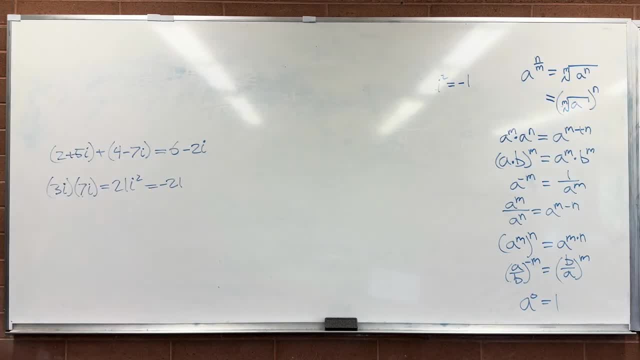 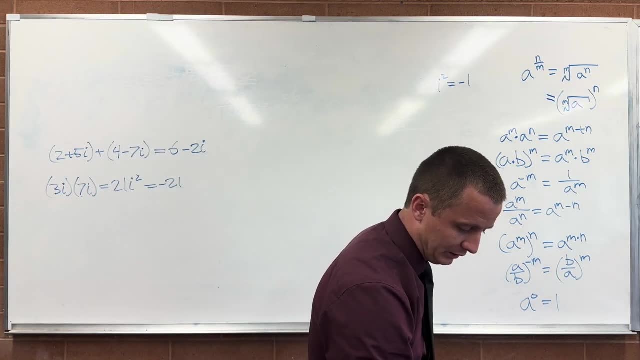 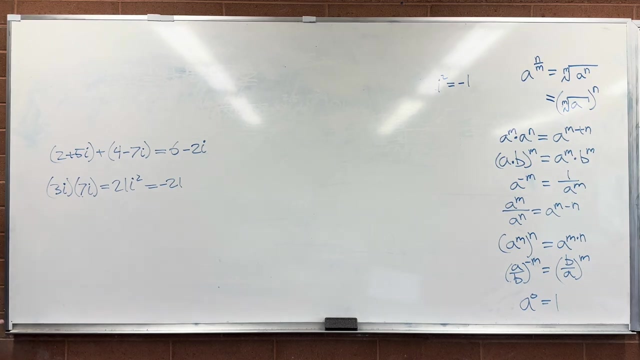 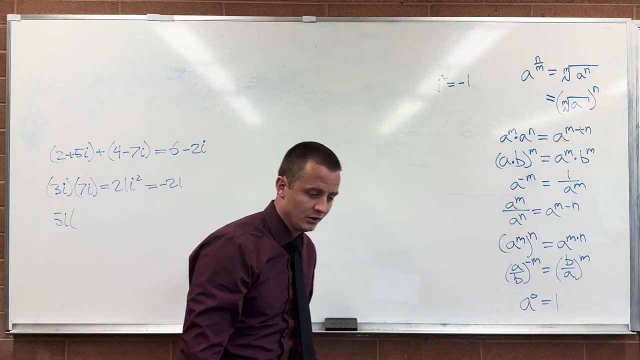 Negative 21.. Negative 21.. So 3I times 7I is negative 21.. Good, Got to get comfortable with these new numbers. Huh Yeah, Not the easiest stuff. Remember Getting close to through the book. 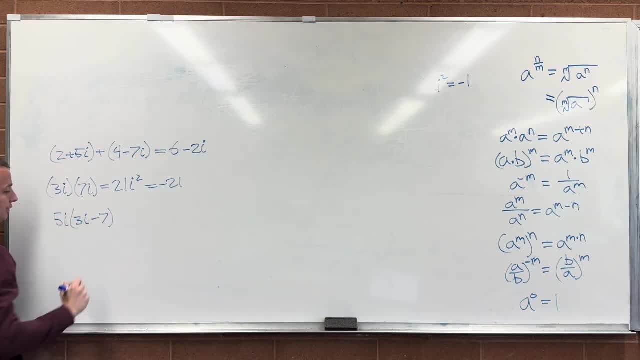 So chances are we're going to start getting into stuff you guys have never seen before, never come across for these last few chapters. Okay, Let's calculate this one: 5I times 3I minus 7.. So it's going to be 15I squared. 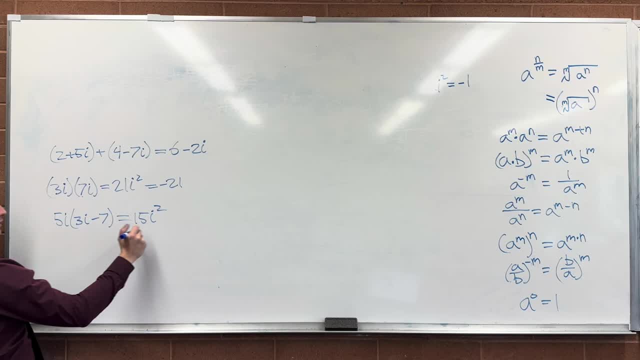 15I squared, Minus 35.. Minus 35I And 15I squared is the same thing as Negative, Negative 15.. Negative, 15.. Love the attitude. There we go, All right, Multiplying two complex numbers to each other. 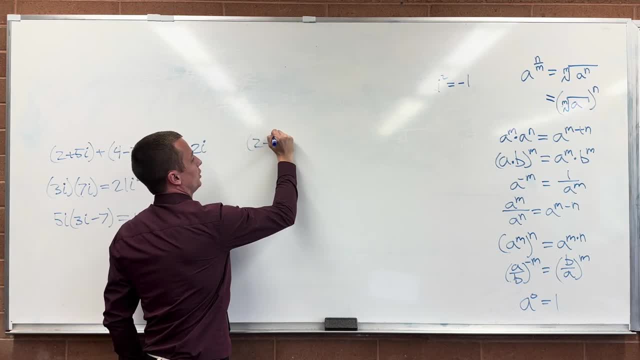 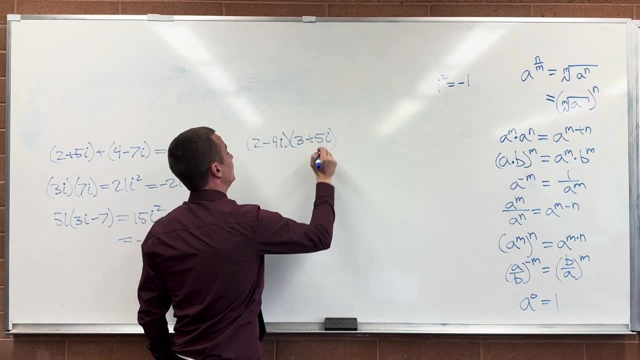 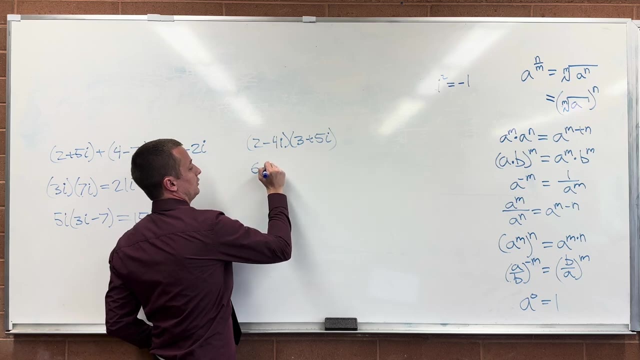 Again, it works exactly the way you know and love: 2 minus 4I times 3 plus 5I, So you just distribute each piece to each piece: 2 times 3 gives us 6. 6.. 2 times 5I gives us. 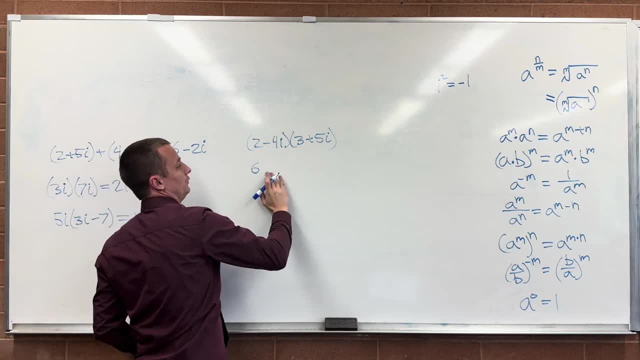 Negative 20.. Negative 20I: Oh, sorry, 20I. Oh, you guys want to do the? Okay, Let's do it your way. Negative 4I times 5I gives us 20I squared. 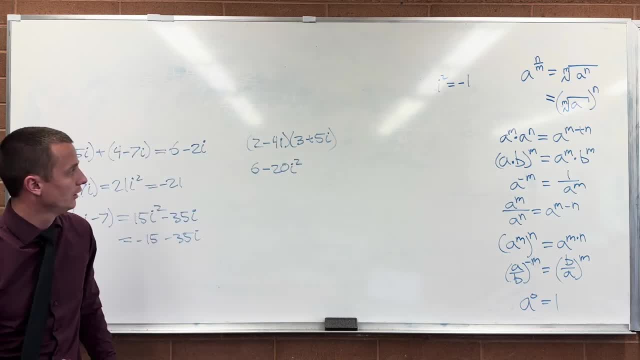 Negative 20I squared. Good, Okay, Now 2.. Wait, You guys are doing it weird. I can't follow your way of thinking about this. All right, Let's first do 2 to both of them and then the negative 4I to both of them. 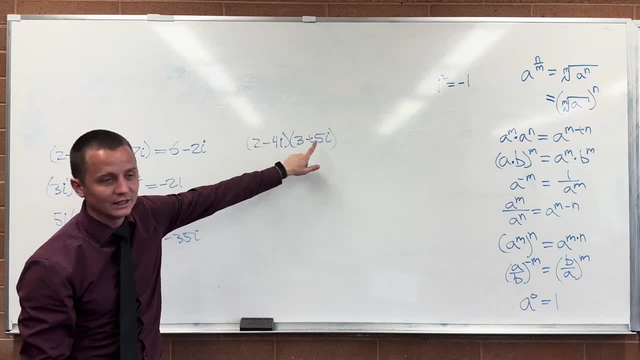 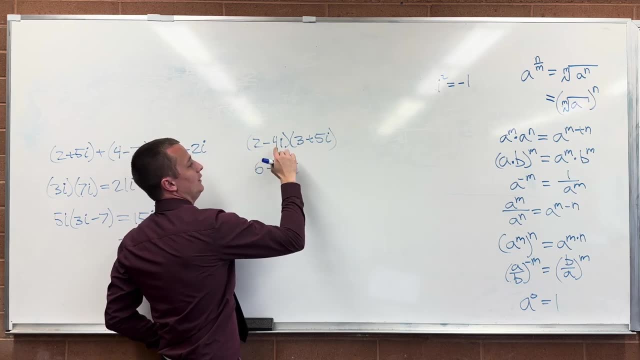 All right. 2 to 3 is 6.. 6.. 2 to 5I is 10. 10. 10. Negative 5I is 10I- 10I. Negative 4I to 3 is: 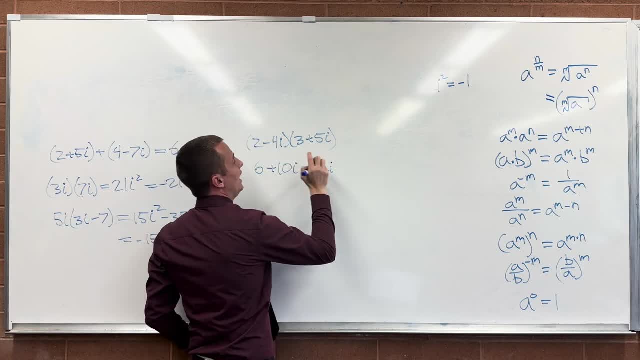 Negative: 12I. Negative 12I. Negative 12I And then negative 4I to 5I is Negative: 20I squared. Negative: 20I squared. Negative. 20I squared. Now negative: 20I squared is the same thing as 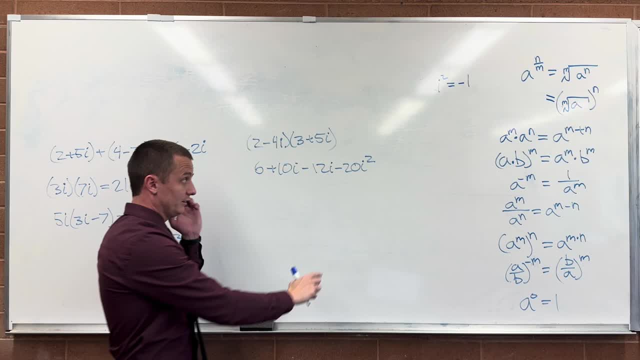 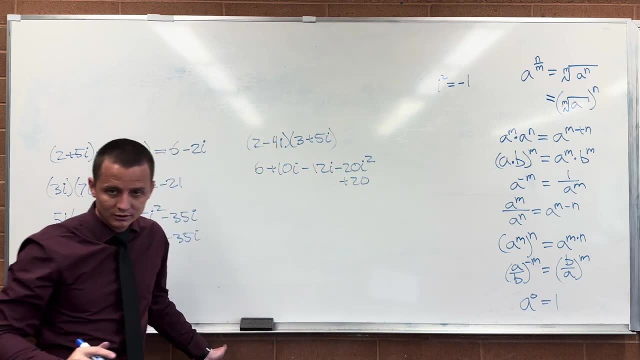 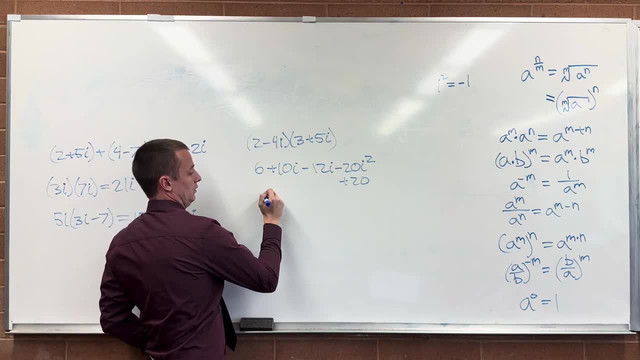 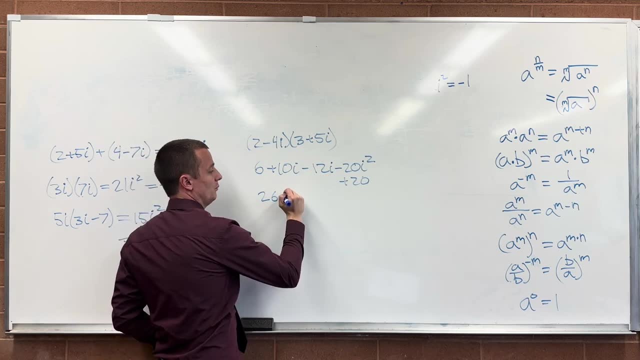 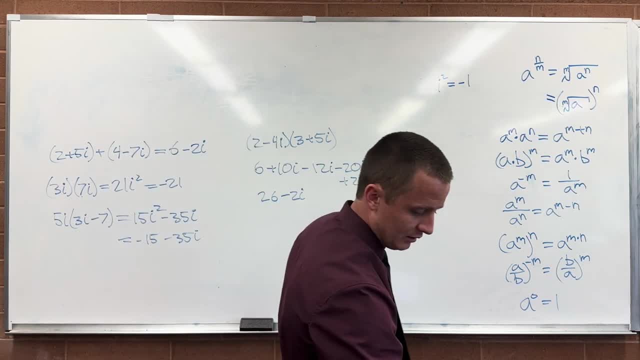 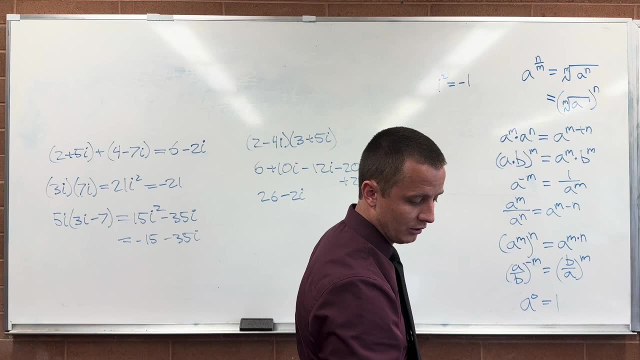 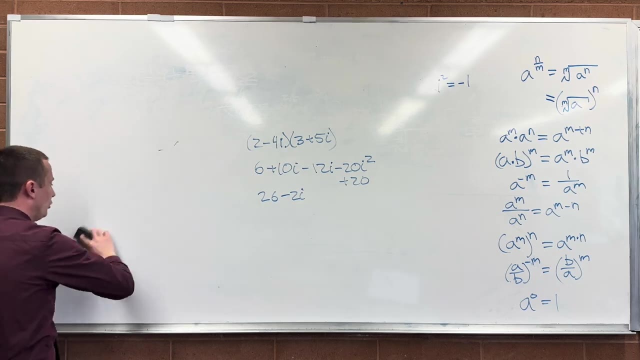 And there's our answer: Okay, Okay, this is a good one. The same way that we don't like having radicals in the denominator, we don't like having imaginary numbers in the denominator, Yeah, Yeah. So when we're told, to simplify, something like 7 plus 3i, 7 plus 3i, all over negative 5i. 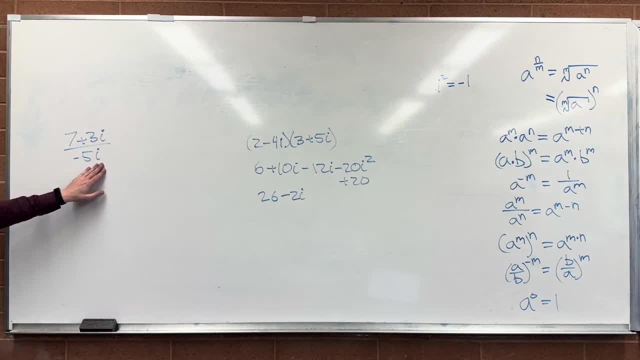 we don't like the i in the denominator. So how can I get rid of the i in the denominator? Just multiply by i, Because i times i is negative 1. So if I have one, i just multiply it by another i and it gets rid of it. 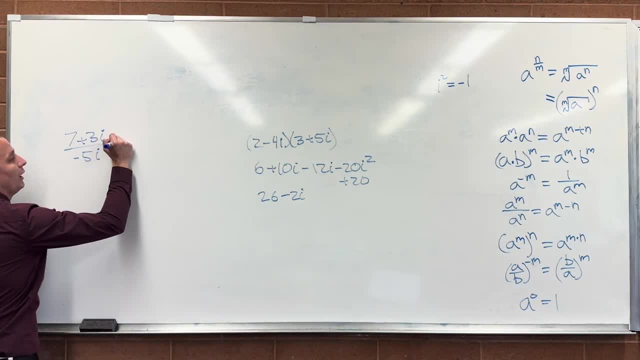 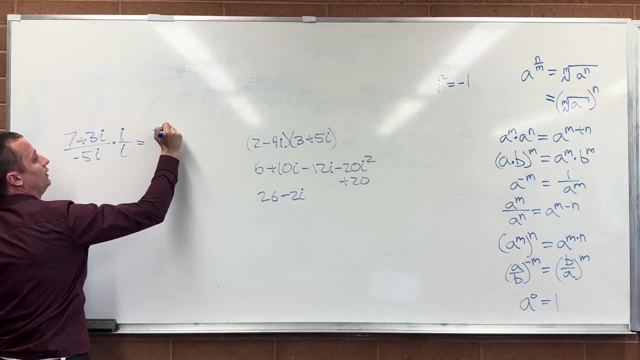 Right, Okay. So multiply top and bottom by i. In the top we get i minus 3.. It's plus 3i squared, which is minus 3.. Good, And in the denominator negative 5i times i is positive 5.. 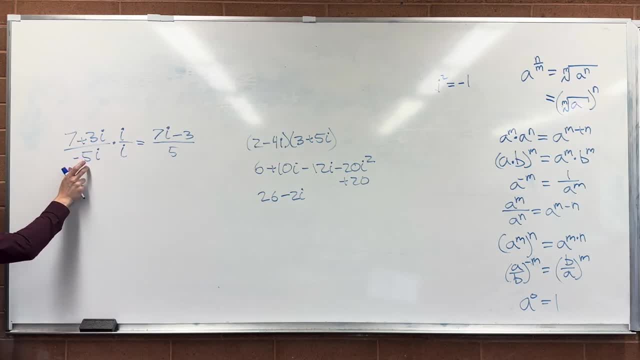 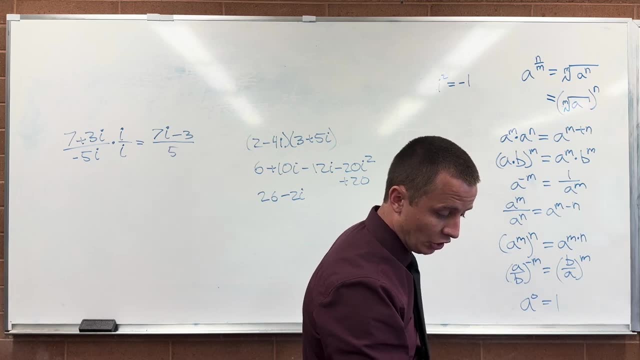 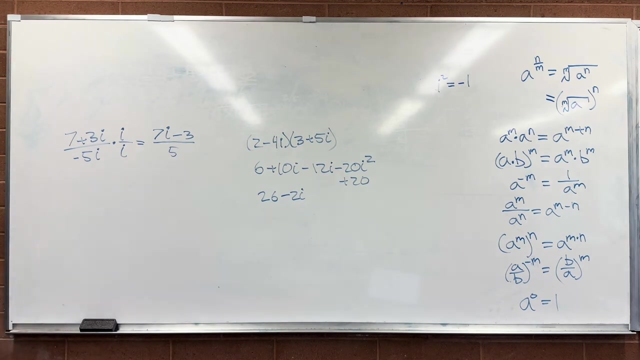 i times i is negative, Negative 1.. Negative 1 times negative 5 is positive 5.. And there's your answer, Right? Not bad at all. Now, the same way that when we had radicals in the denominator, we had to multiply by the conjugate. 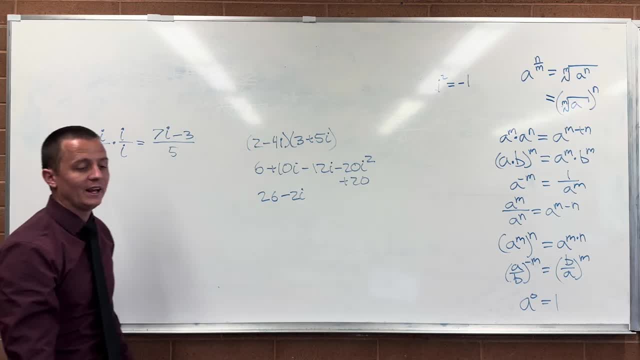 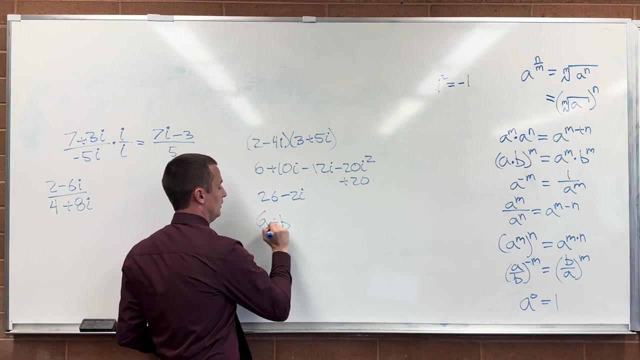 when we have a complex number in the denominator, we often have to multiply by its complex conjugate. So let's see an example of that. So this is 2 minus 6i, All over 4 plus eta. Again, we're going to use the fact that a plus b times a minus b is equal to a squared minus b squared. 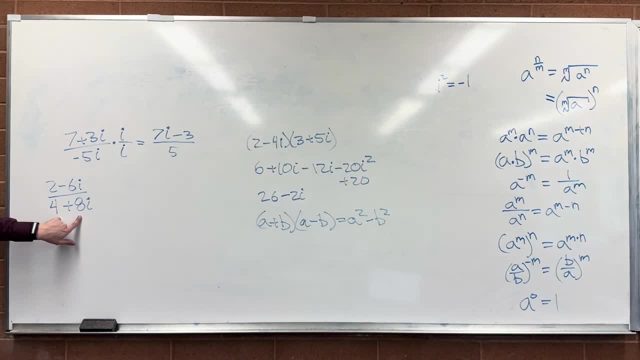 And so same thing here. We're going to multiply top and bottom by its complex conjugate, which is basically just swap the sign. If that was plus, multiply, Multiply by when it's minus. If that was minus, multiply when it's plus. 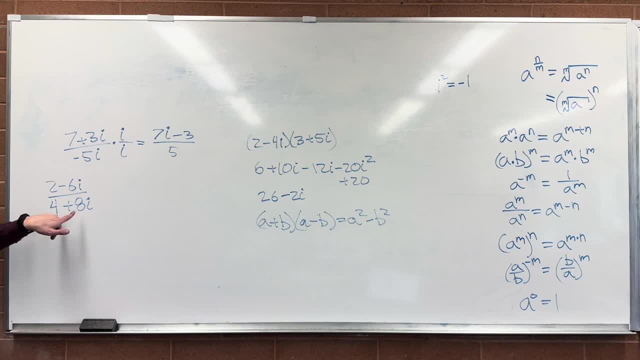 If you have an a plus b, here, you want to multiply by a minus b. If you have an a minus b, here you want to multiply by a plus b. You want, when it's all said and done, to have a squared minus b squared in your denominator. 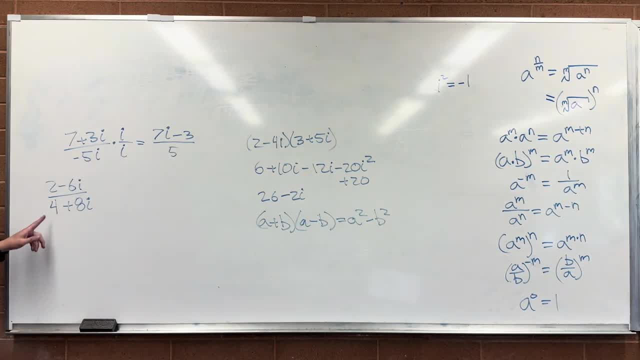 Since everything's squared, it's going to get rid of whichever term had your i's. If this had i's, it's going to get squared. If this had i's, it's going to get squared. And when you square your i's, you get rid of i's. 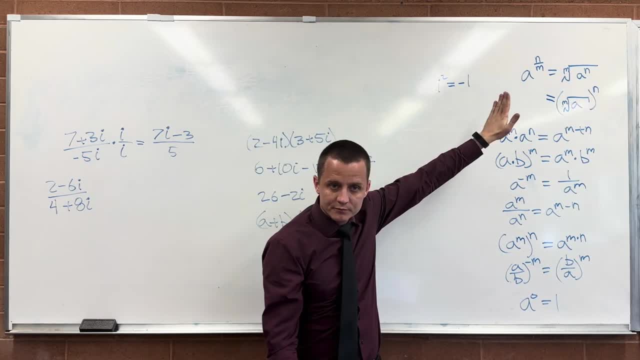 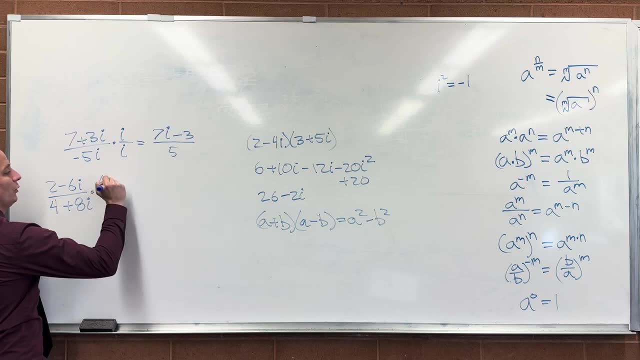 And you replace them with negative 1's. That's the idea. Good, Let's do it. So I'm going to take this one and then multiply top and bottom. by what am I multiplying? by 4 minus 8i? 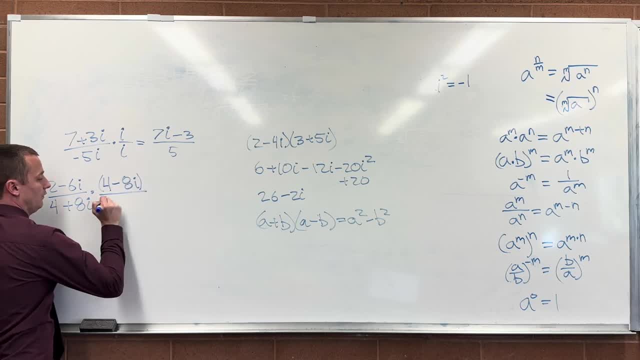 Minus 8i, Good, And again 4 minus 8i In the top. what are we going to get? Let's see ready some of this. We are going to get 8.. So multiplying it all out. 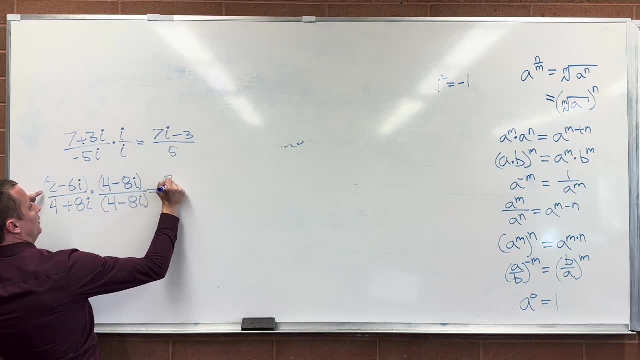 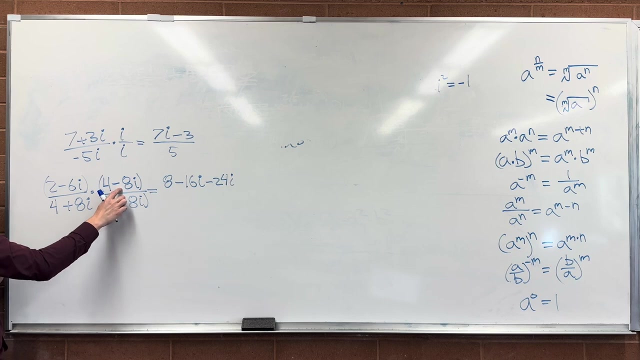 First I'm going to multiply the 2 to everything, So I'm going to get 8 minus 16i. Now I'm going to multiply the negative 6i to these, So minus 24i, And then negative 6 times negative. 8 is. 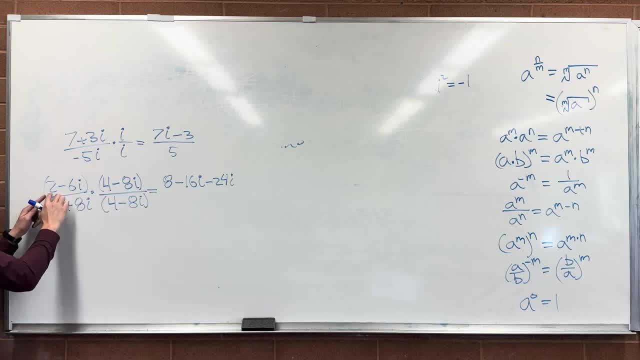 You need to do 4 times 2.. So I did 2 times 4 is 8.. I did 2 times negative 8i is that? Now I did negative 6i times that. Now I'm doing negative 6i times that. 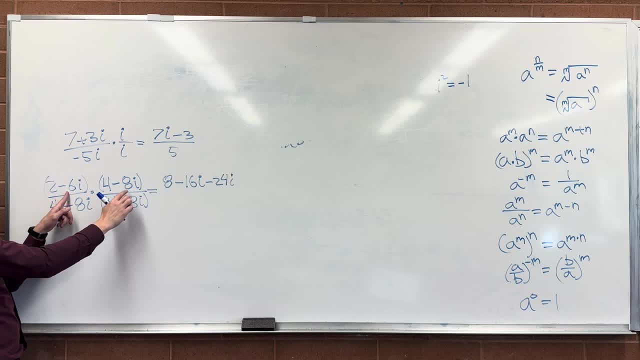 So negative 6 times negative. 8 is Positive 64i, Or it's 48.. Positive 48i squared. Sorry, positive 48i squared, So positive 48.. But then we have that i squared. 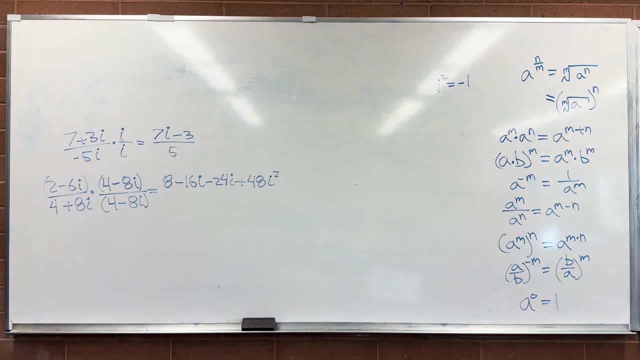 Which is going to make the whole thing negative. We'll catch that in the next round, But I just wanted to see it. And now we can multiply this all out and see that our i's cancel. Or we can remember that a plus b times a minus b is always and forever a squared plus b squared. 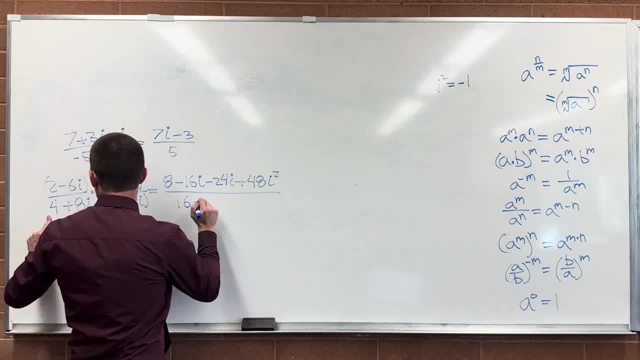 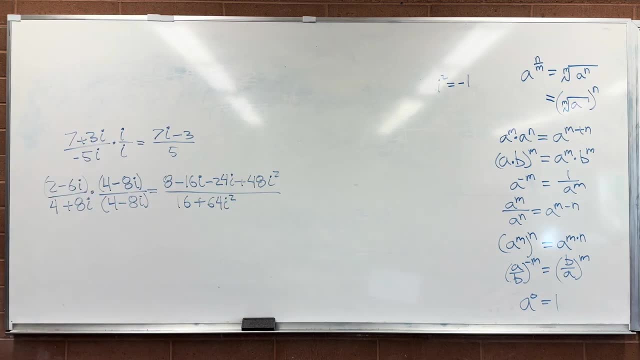 So this is going to be a squared, 16 plus b squared, which is 64i squared. Follow that. Okay, Now let's use the fact that i squared is negative 1 and start combining things. So i squared is negative 1.. 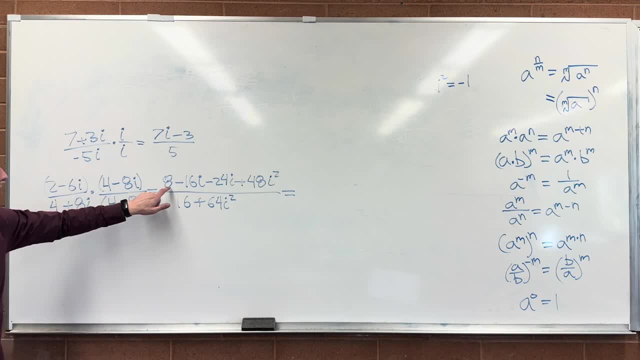 So this is negative 48. Negative 48 and positive 8 gives me 40.. Negative 40.. Negative 40. Good, So we have negative 40. How many i's do we have? We have negative 16 and negative 24 is. 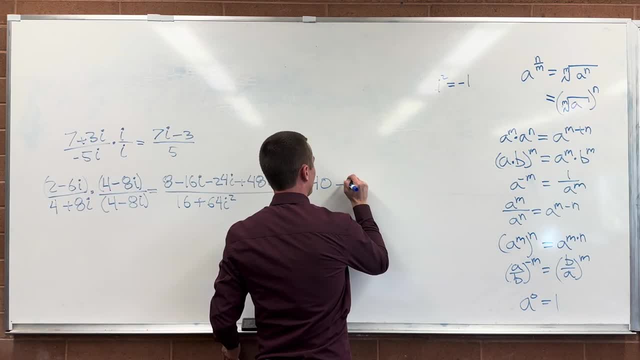 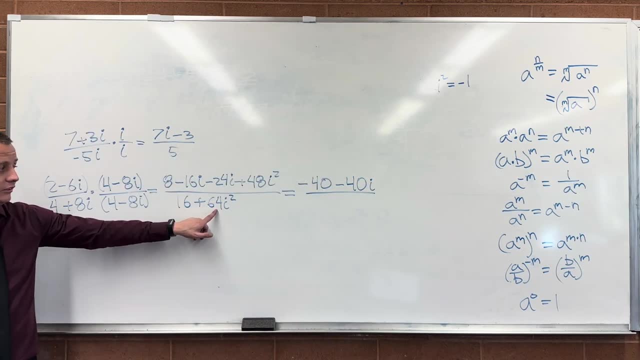 Negative 40.. Minus 40i All over in the denominator we have 64i squared is the same thing as negative 64.. Negative 64 plus 16? Uh, something like 40?, 44?, I don't know Sorry. 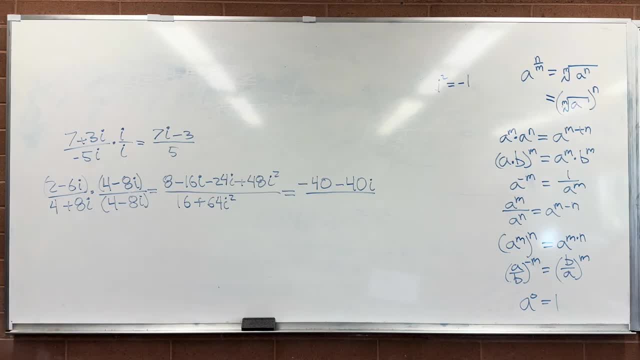 Yes, you got it right: 42.. No, not quite What Huh? It's 40 something. Yeah, it's minus 48.. Oh, 64 minus 16.. 64 minus a 10 gets us 54.. 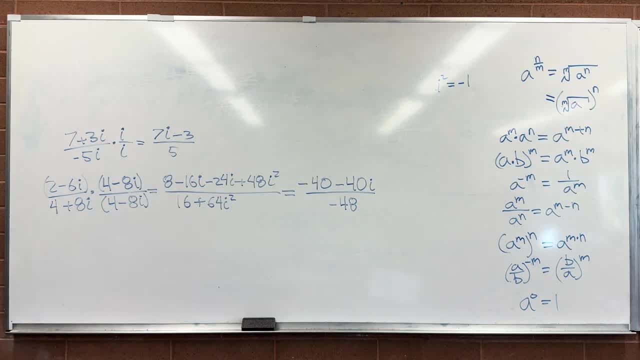 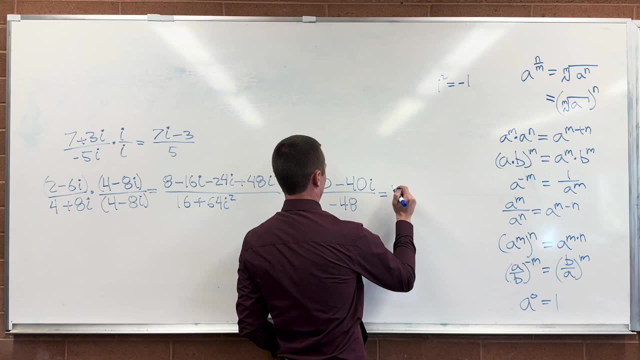 Now minus 6 gets us 48. Minus 48. Okay, We can for sure cancel out a 4 top and bottom. So that gives us. Let's see, we can take an 8 out of everything, right. 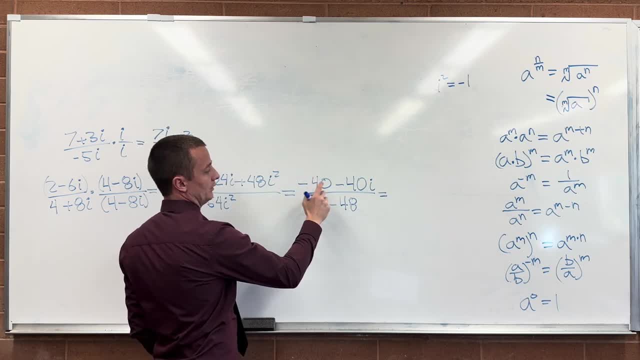 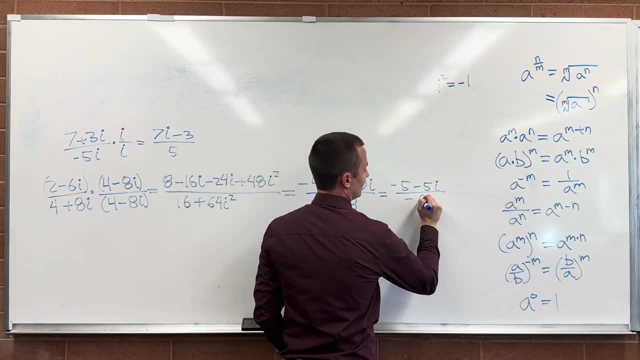 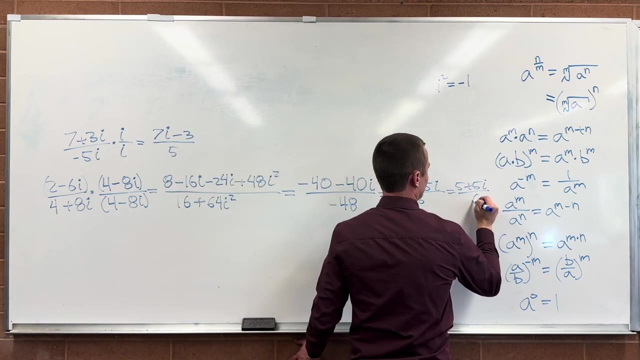 Yeah. So taking an 8 out of everything, that gives us a minus 5.. Minus 5i all over, Minus 6.. Minus 6.. Let's take the negative out of everything And that gives us 5 plus 5i over 6.. 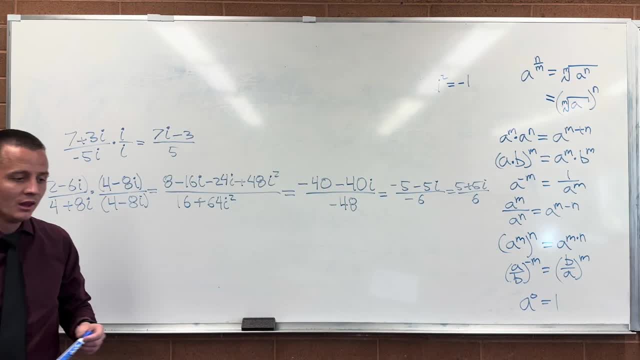 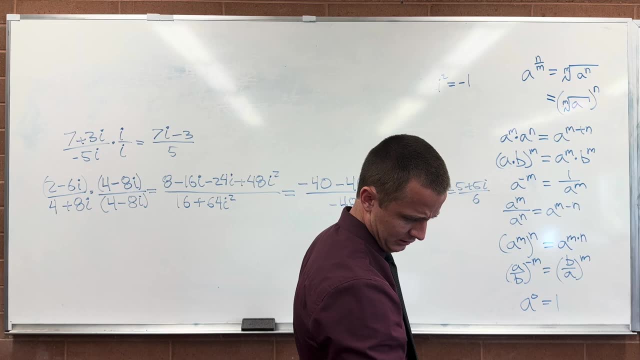 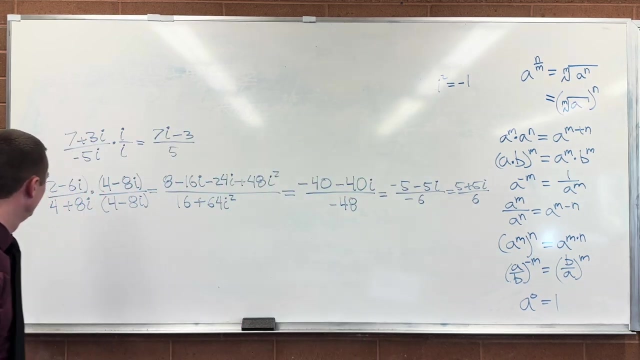 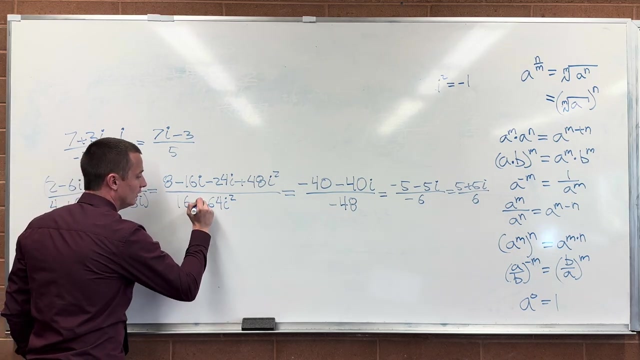 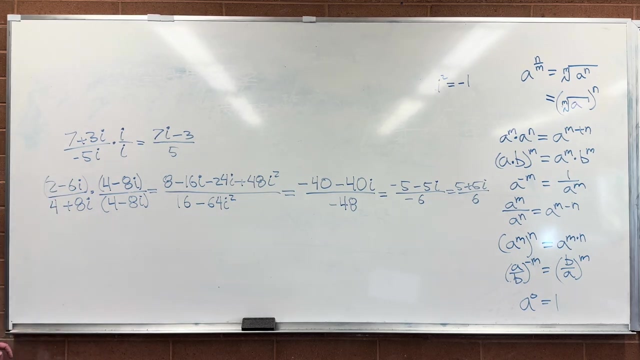 Right, And let's see his answer. Enter: Oh, Time to stop right here. a plus b times a minus b is a squared minus b squared. So it would be a positive 64.. So it would be a positive 64.. 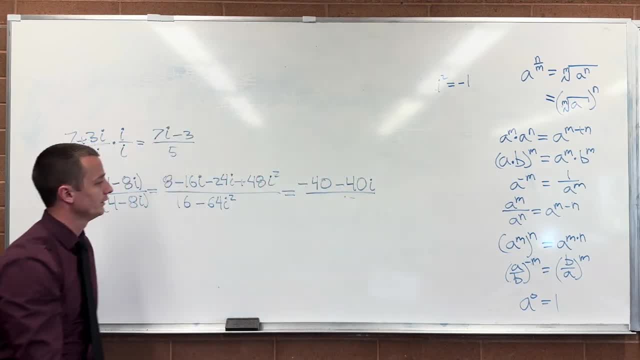 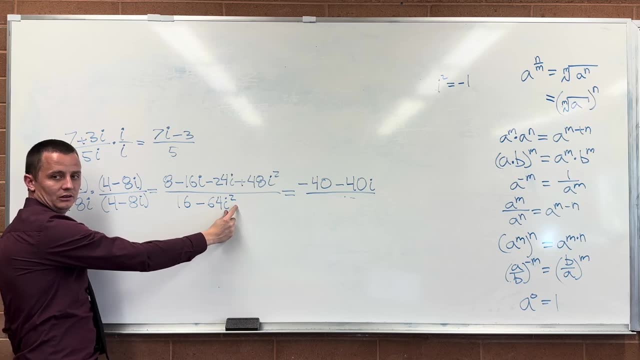 So we did our numerator right. This is our denominator that we did wrong. So let's work this out again: 16 minus- well, i squared- is negative 1.. So negative 64 times negative 1 is. 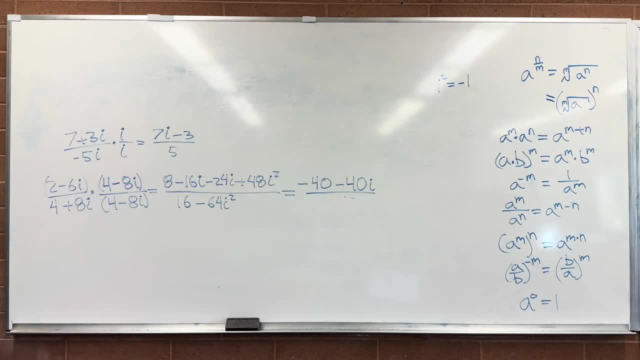 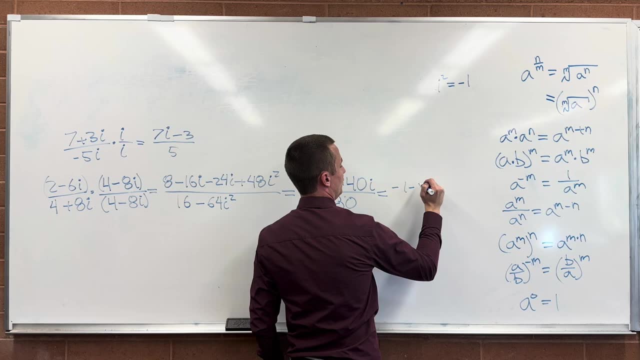 64. Positive 64. 64 plus 16 is 80. 80. And now we can cancel out 40 top and bottom And we're left with negative 1 minus i all over 2. Like that. 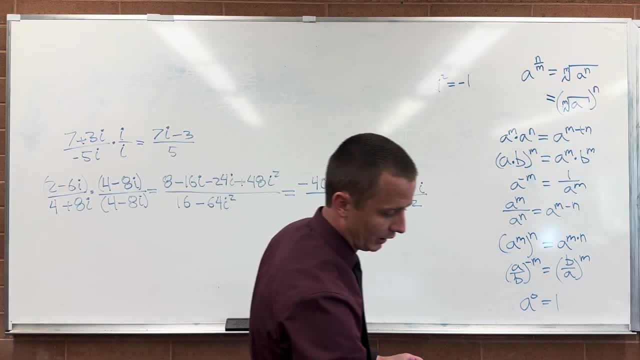 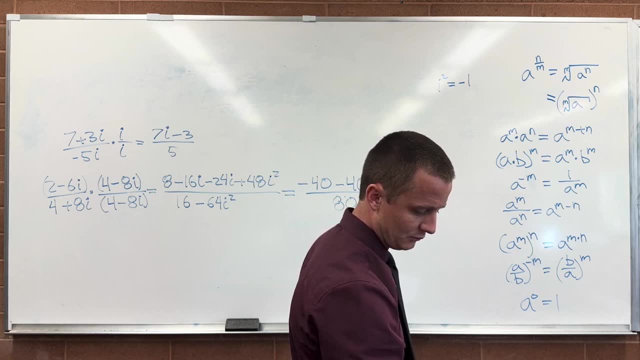 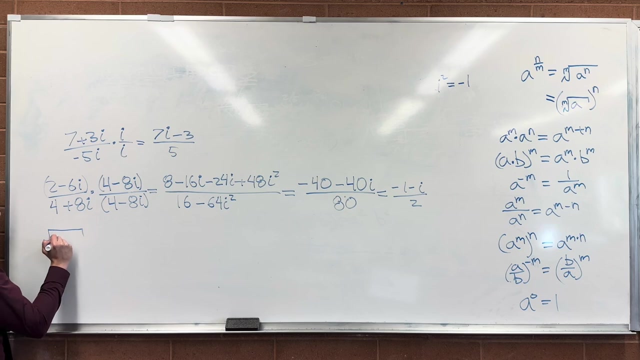 And that's what he has. All right, That's a good one, Nice, simple one, OK. So now we can calculate the square roots of negative numbers. So what's the square root of negative 16?? So I can pull 4 out. 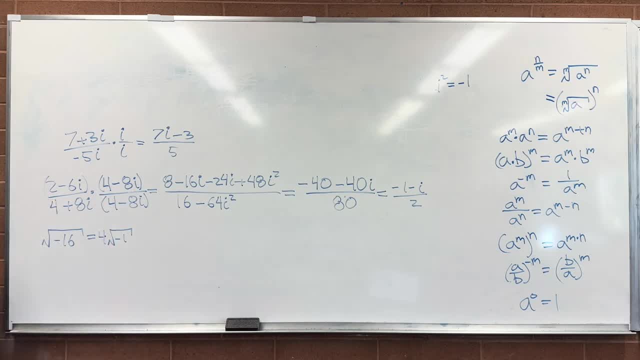 Mm-hmm, negative 1.. But what is the square root of negative 1? I, I is the square root of negative 1.. So this is just 4i, Or in other words, what's 4i times 4i, Negative 16.. Okay. 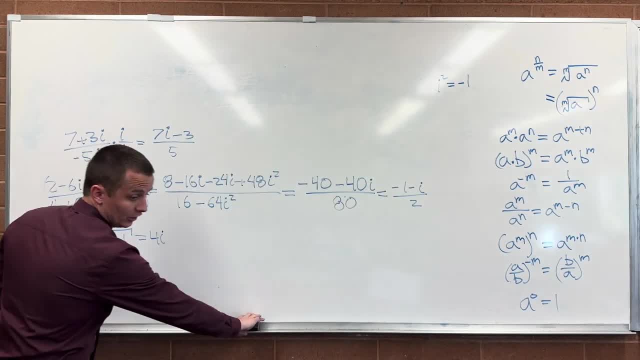 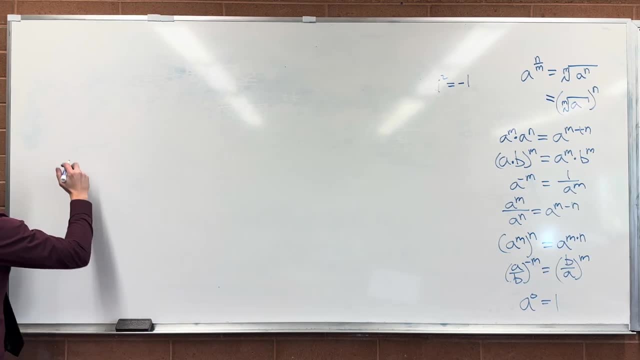 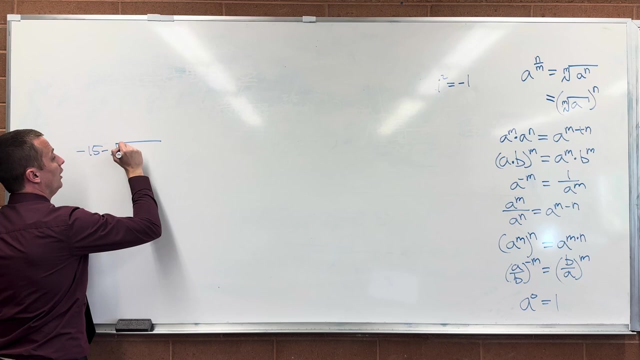 One more example, and then we'll be done with the material for today. So our last example: we want to do negative 15 minus the square root of negative 200, all over 20.. And see what that equals. Okay, So this 200, looking for. 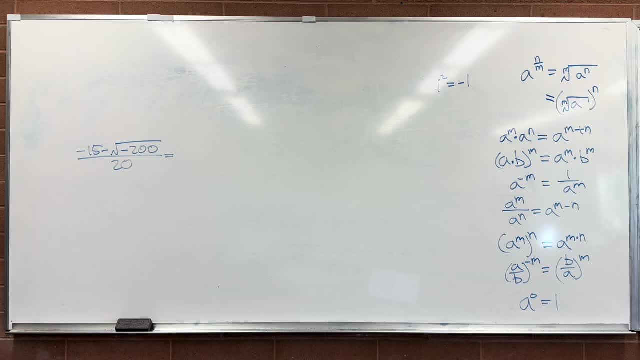 perfect squares in there. 4.. Say that again: 4. 4 goes in there. 3 and 8. I lied, Not 3 and 8.. All right, Let's keep thinking about this, So 200.. 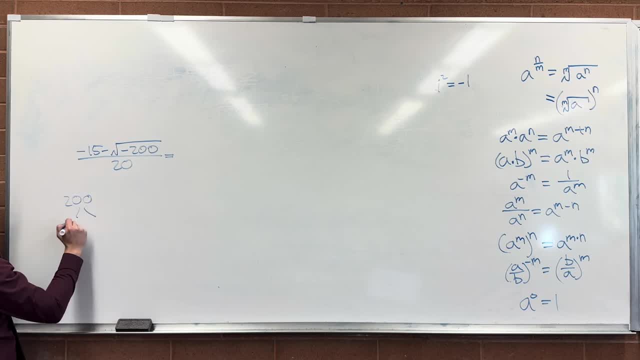 You already pulled the 4 out. If I pull the 4 out, what am I left with? 4.. 4 times what is 200?? Oh, 50.. 50. Okay, And then is there a perfect square in 50? Yes, What is it? 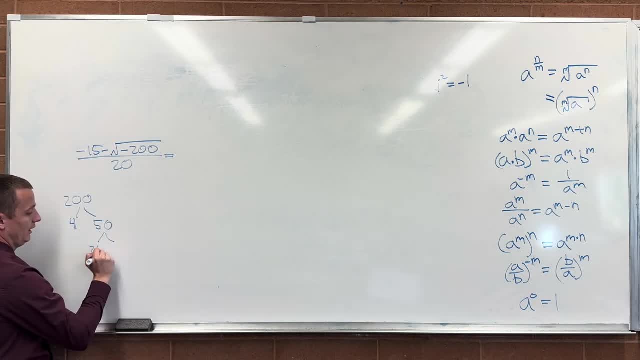 25.. 25.. Yes, 25 times 2.. All right. So 4 gave us a perfect square and 25 gave us a perfect square. So 4 times 25 will give us a perfect square, which is 100.. 100 is a perfect square 10 times 10.. 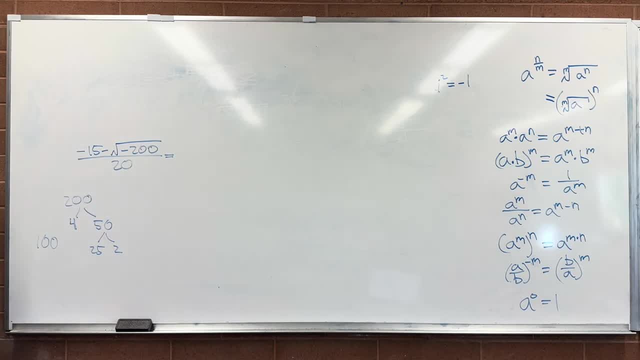 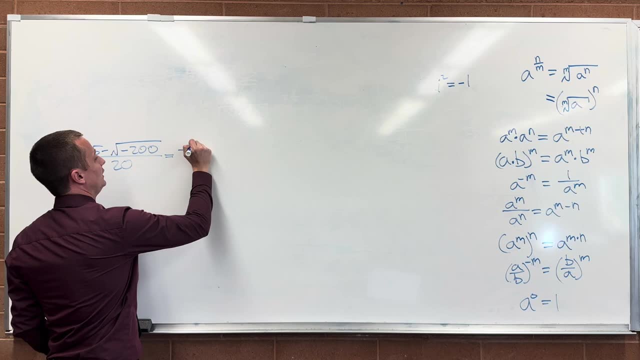 Whoa. Okay, So we're looking for a perfect square that goes to 200.. It's 100 and 2.. Oh, You see that. So this is negative 15.. I'm going to pull out 100, which turns it into 10..